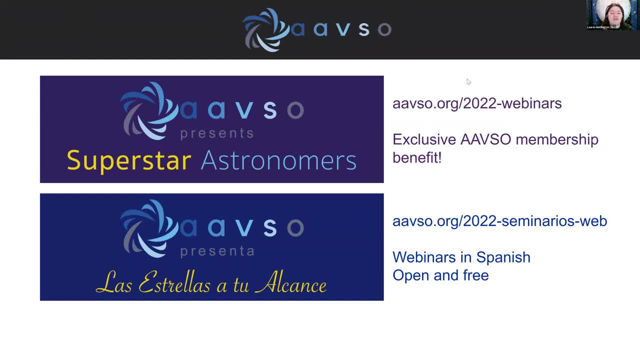 Superstar Astronomers is a members-only broadcast which features talks from the world's leading astronomers Coming up. later this month, we will be hearing from Dr Emily Levesque about a bird that mimicked a black hole and a telescope that got shot. Are you curious? what on earth that's? 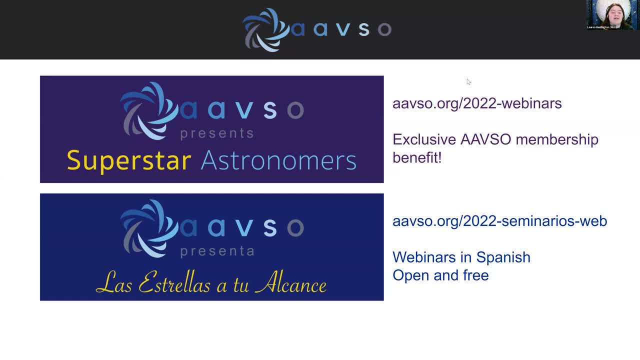 about Because I am. If you are just like me, please visit our website to register for the webinar and find out about it for yourself. Also new this year: our very own Sebastian Otero is hosting a very exciting webinar series in Spanish, So if you or one of your astronomy. 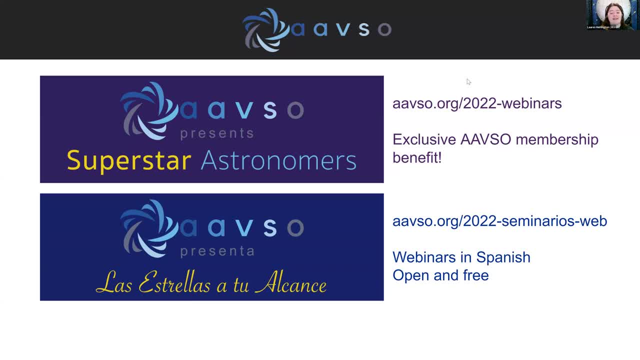 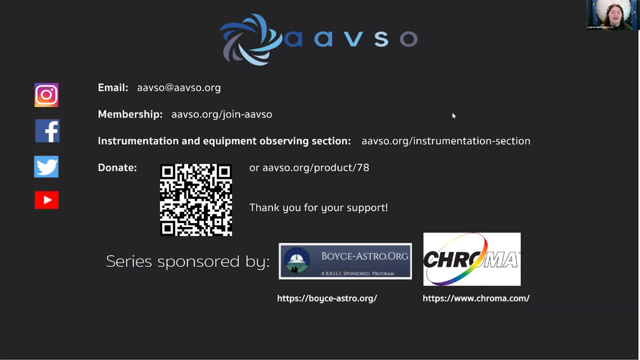 friends speak Spanish, please feel free to join us. The links to learn more about each of these webinar series are up there on the screen. Finally, we would like to thank and acknowledge our sponsors Boyce Astro and Chroma Technology, The Boyce Research Initiative and Education. 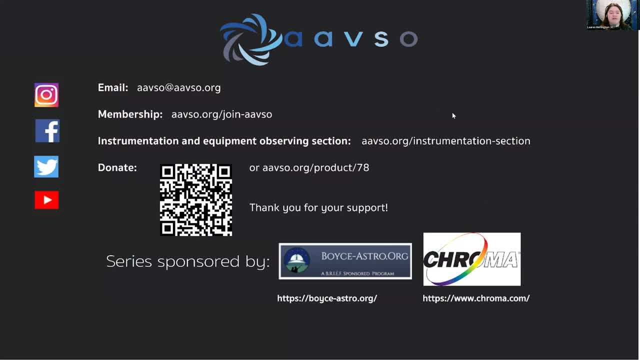 Foundation provides online astronomy education, observatory resources and research experiences to students who are interested in learning more about astronomy. The Boyce Research Initiative and Education Foundation provides online astronomy education, observatory resources and research experiences to students, student teams and schools, in order to 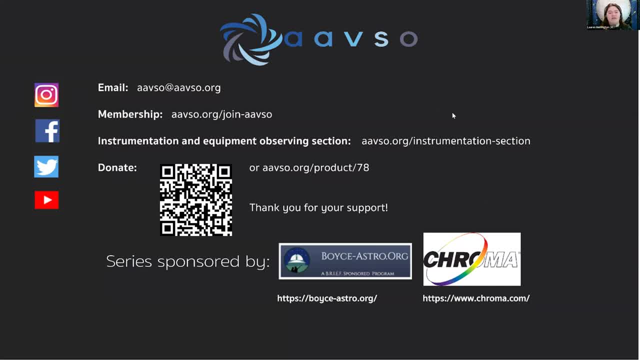 learn how to perform observations, conduct research and publish their results in scientific journals such as the Journal of the AAVSO. Please do check out their webpage to learn more about their work. Founded in 1991 as a 100% employee-owned company, Chroma Technology is a. 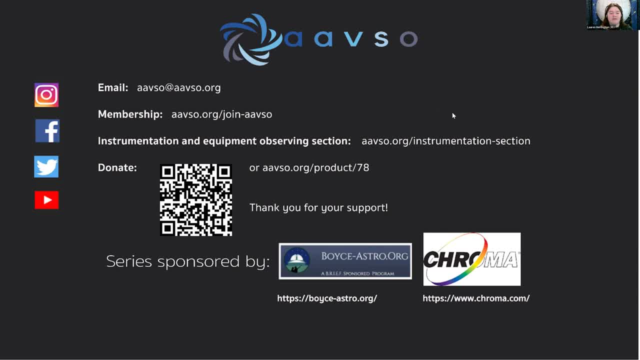 leading manufacturer and OEM supplier of highly precise optical filters using thin-film coding technology. Their reputation is built on dedicated customer service, including free clinical and application support. They remain committed to serving both the scientific and technical communities in their pursuit of the scientific endeavor Chroma's product. 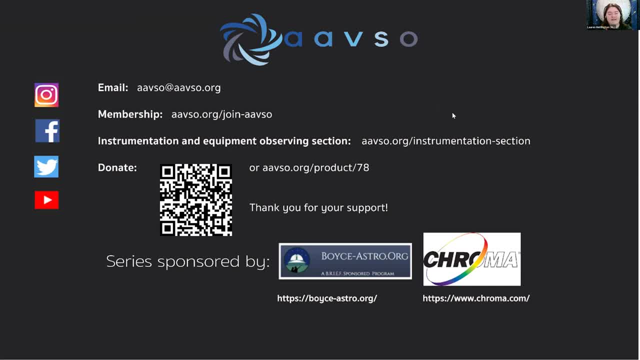 portfolio provides solutions for industries ranging from the life sciences and agriculture to manufacturing, inspection, security and aerospace. This broad array of applications served includes fluorescence, microscopy, flow cytometry, biomedical instrumentation and surgical devices, machine vision, multispectral imaging and, of course, our favorite, astronomy. 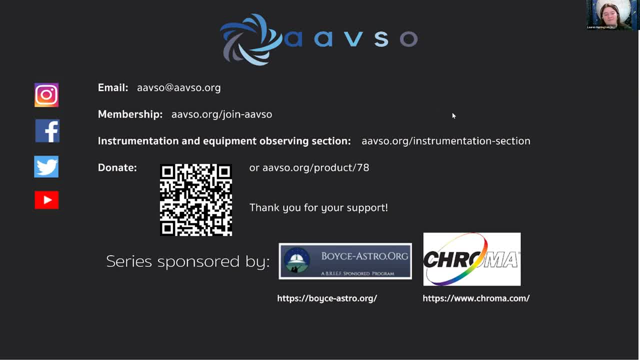 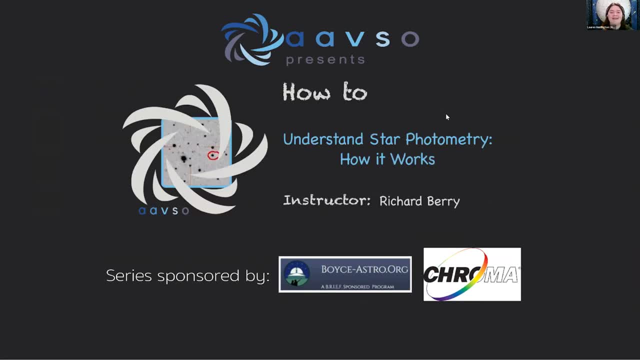 Thank you for your time today and I look forward to seeing you in the next webinar. Okay, now with that out of the way, allow me to introduce your instructor for today. It is my great pleasure to welcome back to this webinar series Richard Berry. Mr Berry. 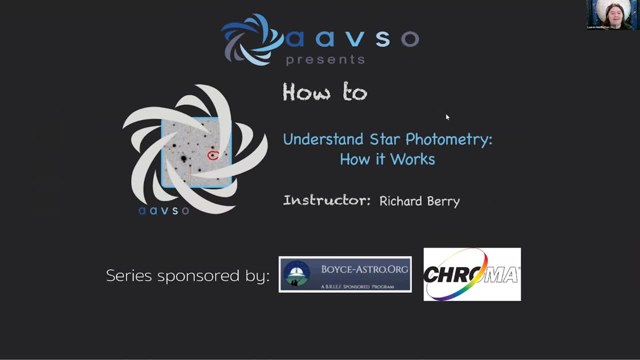 has been a frequent presenter at past AAVSO meetings and webinars, and it's really not hard to see why He has over 30 years of expertise in a wide variety of fields, from telescope making to observatory building to photometry, which he's been practicing ever since the 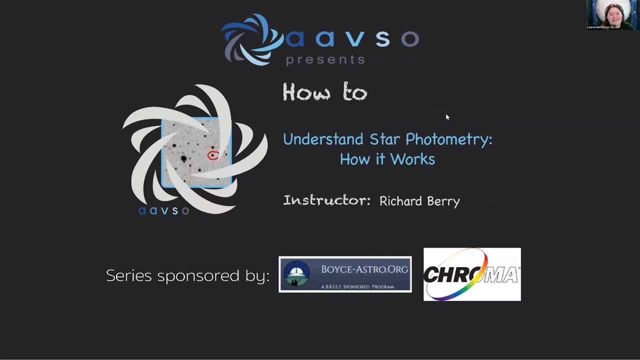 days of photomultiplier tubes. As if that weren't enough, he's also a software developer and the author behind the software Astronomical Image Processing for Windows, also known as AIP4Win. Between his observational experience and his experience literally writing the tools that the rest of us use, he's come 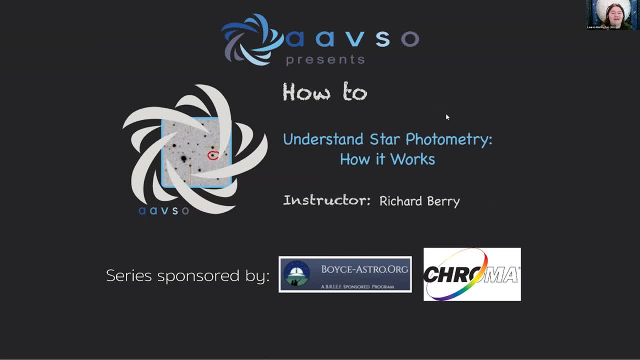 to be quite an expert on the topic of photometry- Not only how the data is recorded, but also how it's handled behind the scenes. Today, he's here with us to give us a glimpse into the nuts and bolts of photometry, and 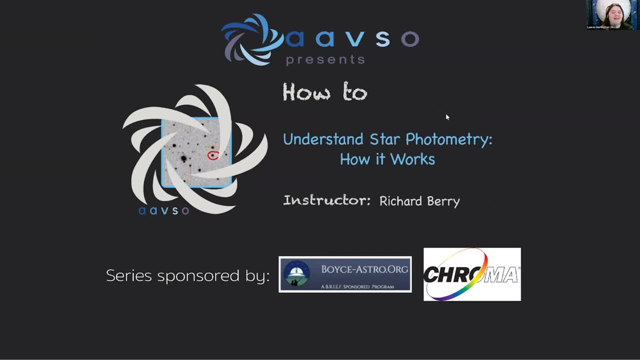 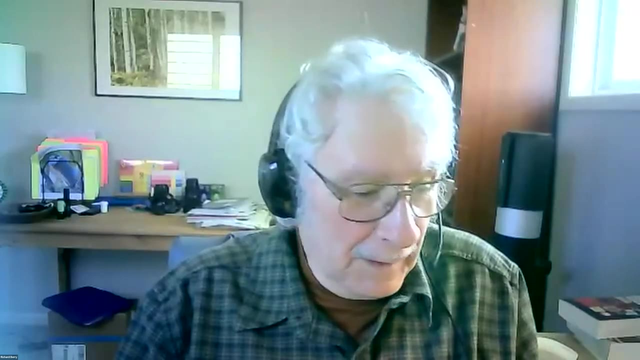 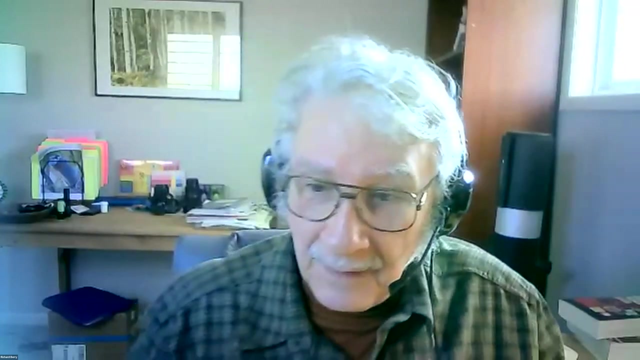 how, with a little bit of math, a bunch of pixels can be transformed into scientific discovery. Without further ado, please allow me to introduce Richard Berry. Welcome back, Mr Berry. Hi, Lauren, So what I'm going to do today is take you on a tour inside the computer. 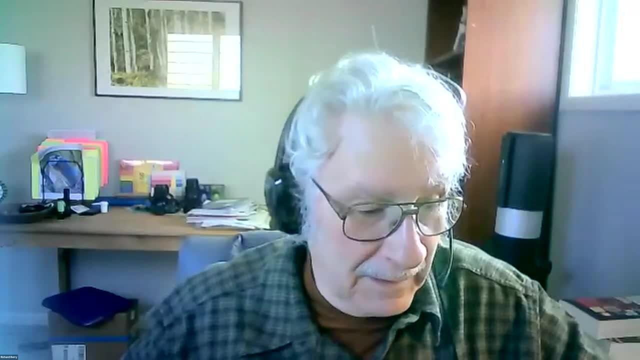 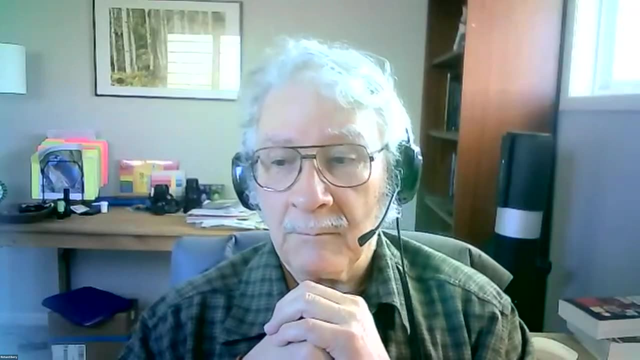 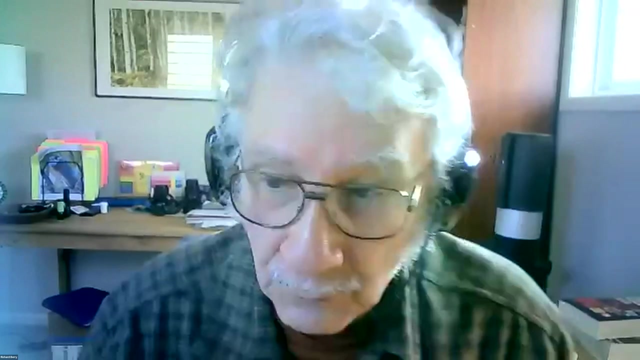 I'm going to show you a little bit of what it looks like inside, the way it works, And I will be using AIP4Windows as my demonstration tool. But basically all photometry, all aperture photometry, works pretty much the same way, So what I will tell you will probably apply. 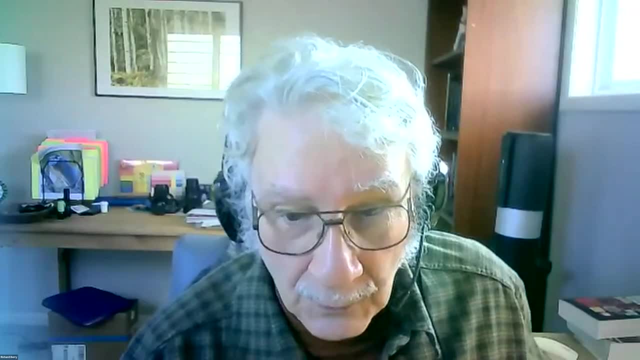 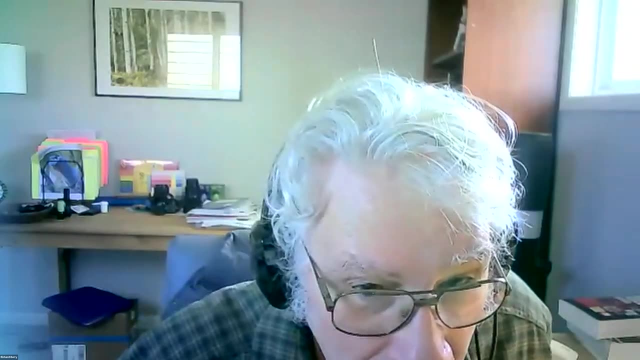 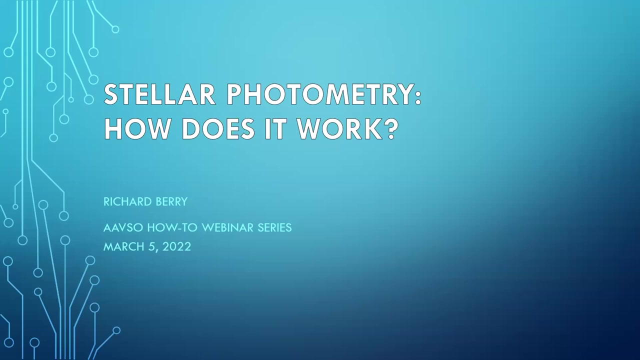 reasonably well to almost any software you may be using. So I'm going to share my screen And if we've done this right, Okay, All right. So we should be there Looks great, Okay And okay. So, and I'm using the presenter mode and if everything's working right, you. 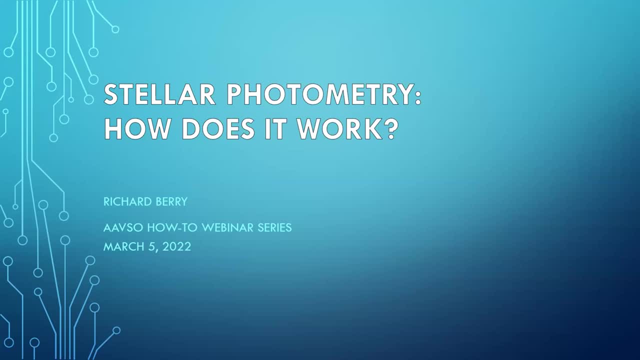 guys are still seeing the title slide. Yep, looks great on full screen and everything We practice and we're perfect. Okay, Thank you Great. So what's going on? Wait a minute. Oh, it's a very Windowsy thing. 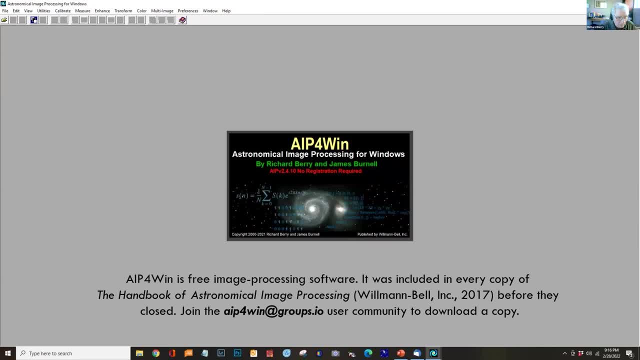 It locks out my screen. Okay, Okay, So AIP4Windows is free and that's by accident. My publisher went out of business and left my software orphaned on the Web. I did some quick hacks in it, some quick hacks in it, and created a groups IO called AIP, for when user community and you can download the software from there. it's free, it's open to everybody. 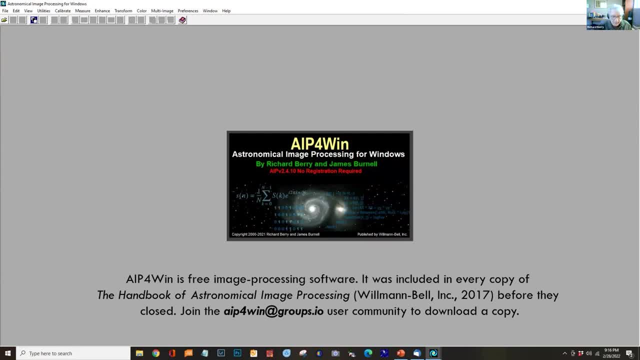 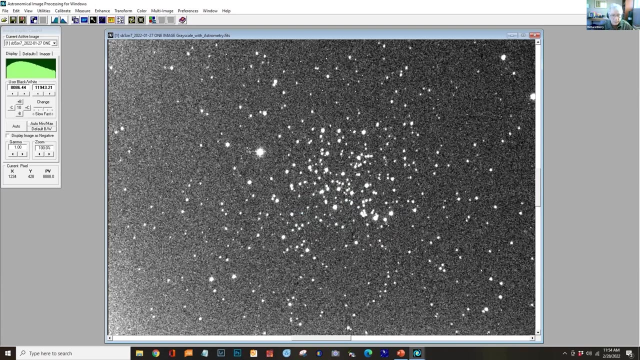 And, with all honesty, it does have some bugs, Because it was a quick and dirty job. So let's begin the software I'm I'm going to be working with today: two images of m 67, which is a cluster that's used for standardizing filters and cameras, because it's got a lot of stars whose standard magnitudes are well known. 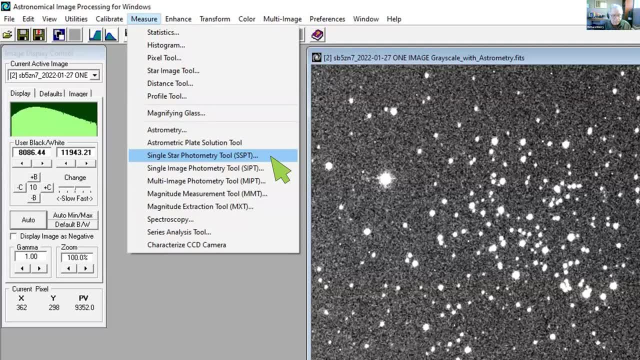 And I will be demonstrating today With the very simplest photometry tool in AIP for Windows, which is a single star photometry tool. This is basically written as a learning tool for beginners And I'm demonstrating with it because it's it's not complicated, It's easy to explain, So we click on that link. 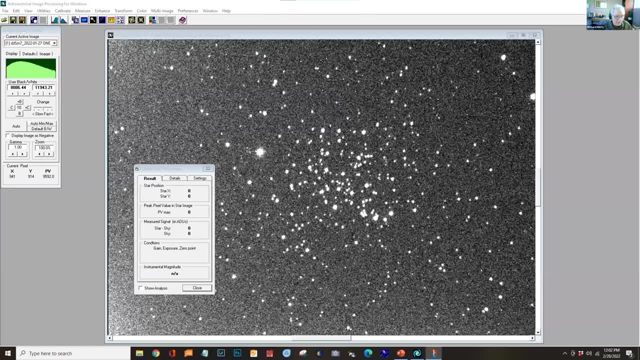 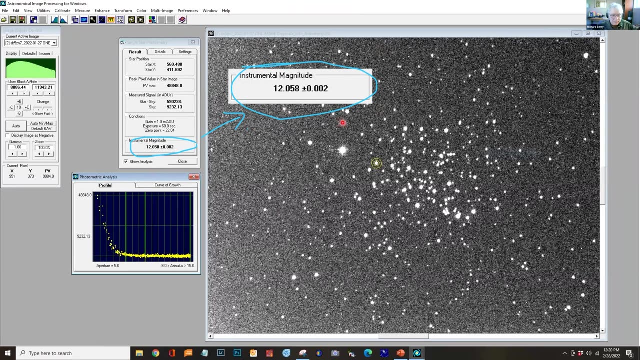 The tool comes up. you can, you can see it. Let me get my laser pointer. There we go. So there's the tool, very simple tool, And we go out, we click on a star and magnitude comes up. Aha, it's magic. 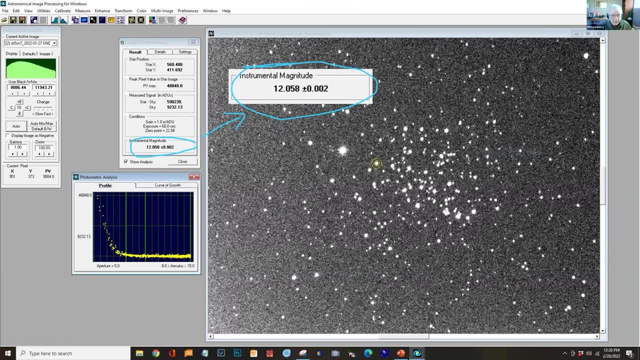 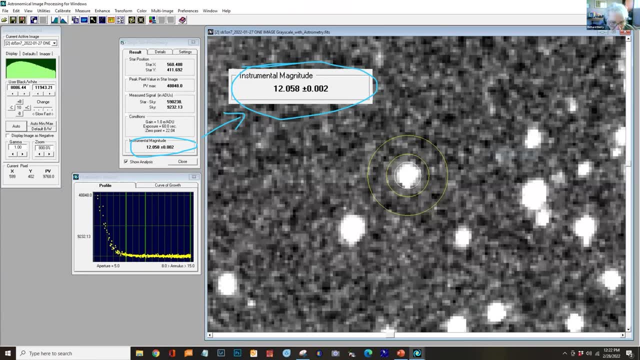 Okay. so what I'm going to be talking about today is how does that happen? And we're going to be moving in close and getting really up close and personal With the pixels and the star images. Now, this image is a four second exposure using a EV scope by uni stellar. 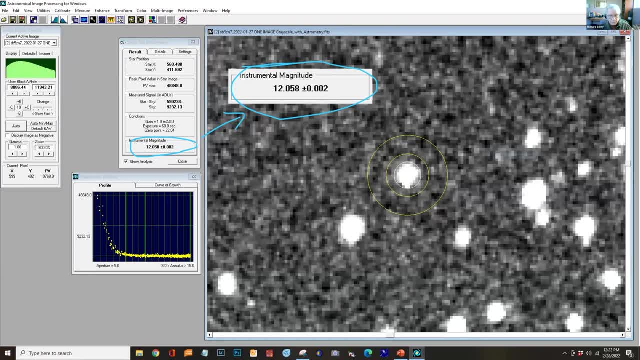 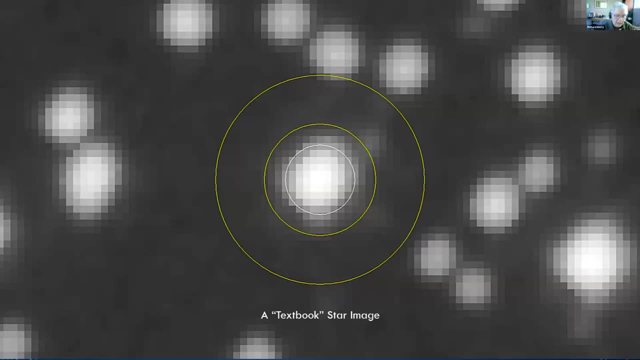 It's it's basic way of taking pictures, as it shoots a lot of four second exposures and then stacks them. The other image I'll be working with is a stacked image And it's made with 904 second frames And when you do that you get a beautiful textbook star image. 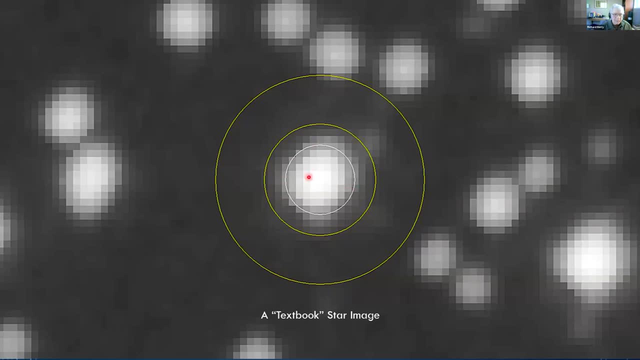 I mean, this is there's the star. it's nice and well sampled, You've got pretty clean. there's not much many background stars in it and you can see, because we're working in M 67. It's a very crowded field. 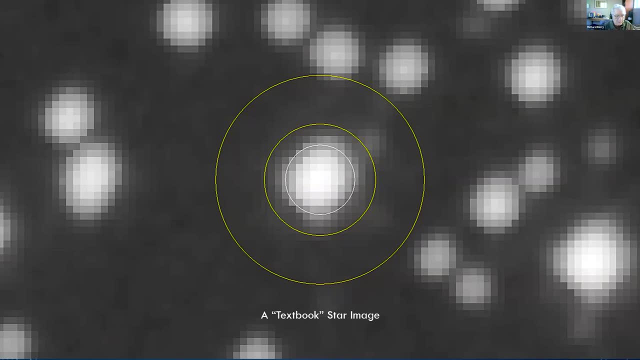 This kind of field. it kind of gives photometers connections, because if you go click and you want to do something with this star, Ah, you're going to have some competition with that star. but we'll talk about how that kind of stuff works. 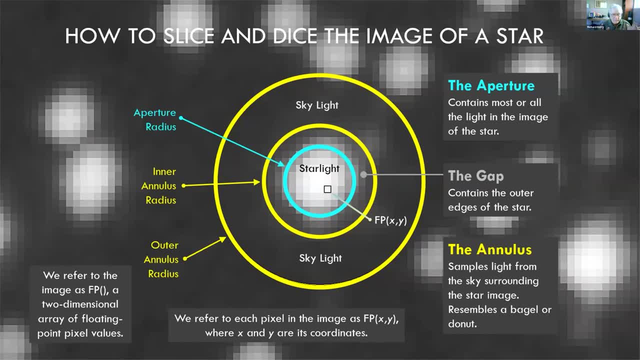 So here's. here's the basic piece of information that everybody does- photometry, aperture photometry- needs to understand. This is how we slice and dice the image of the star. This is how we slice and dice the image of the star. Okay, 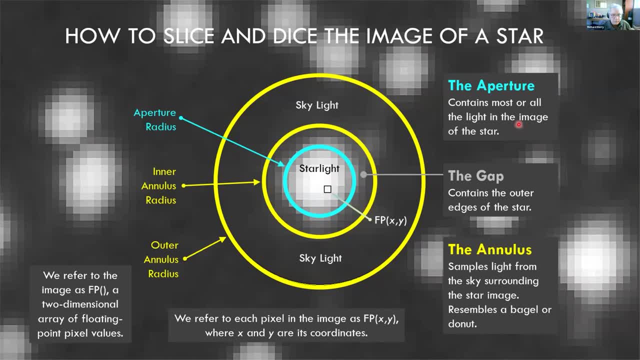 In the middle, closely surrounding the star, is what's called the aperture. aperture is the Latin word for window, Okay, and it contains most or all of the light in the, in the star image. Then we have a gap, And the reason we have a gap is that the star image usually has some extension. there's light out here. 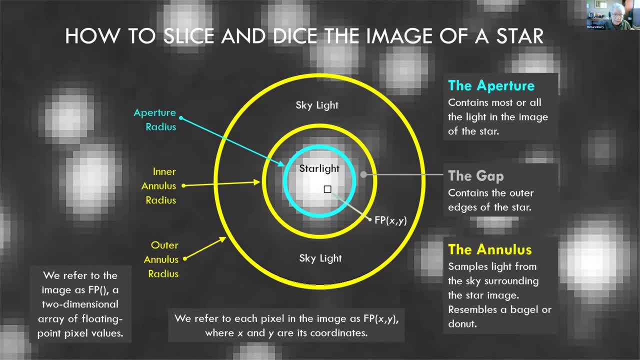 And it turns out- this is interesting- that the most efficient photometry actually does not quite use all of the stars light. As we begin to add more pixels to try to get all the starlight, We're adding noise from the sky background. And then, finally, we have the annulus- a donut or a bagel- you can call it either one if you want- to which we're going to use to determine. 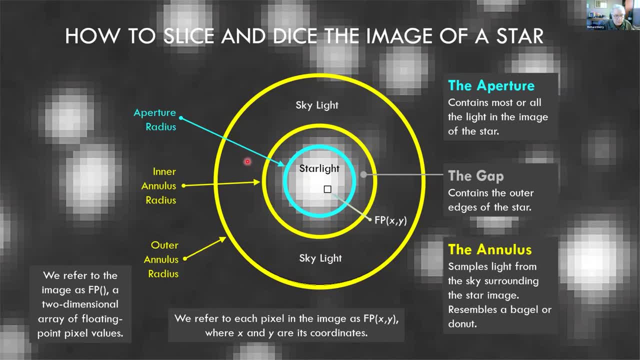 Which we're going to use to determine How much light is coming from the star that is adding to the light in the star. So the definitions: this is the aperture radius from center out, This is the inner annulus radius and this is the outer annulus radius. 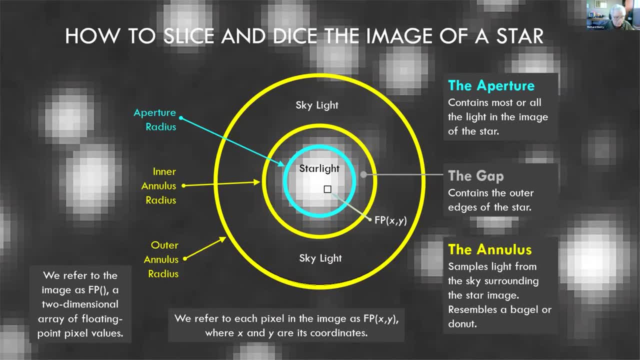 And because we're going to be talking about software code And if you're, if you don't do software programming, You're going to get technical, But you will see code, Don't let your eyes glaze over. It's to make a button. It's basic. Okay, so it's basic software. 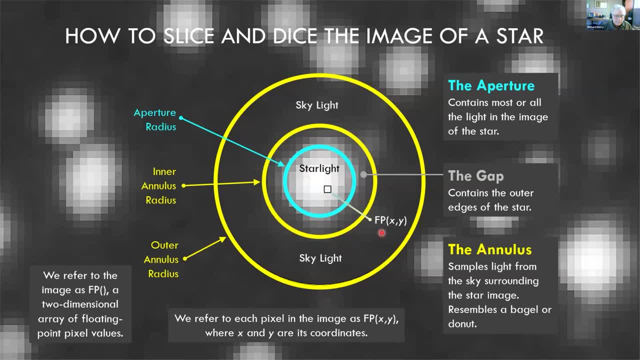 We call any given pixel. The terminology we use is FP. FP is an array of floating point values And X, Y is. it's X, Y coordinates, So X and Y axes, So the image itself is X. FP Meaning this notation means it's an array. 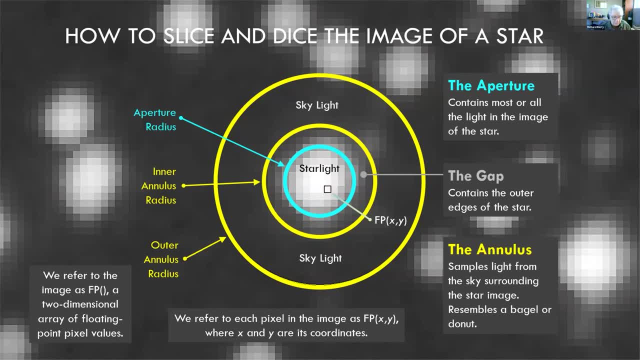 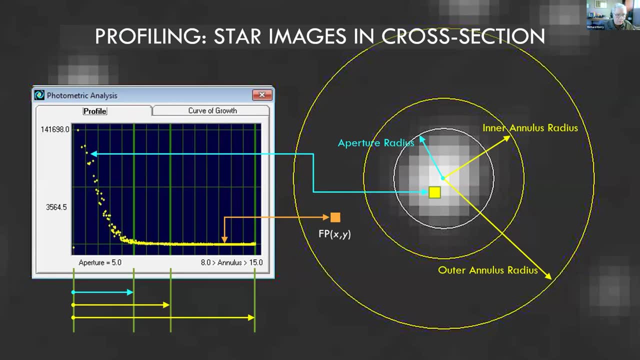 And X. Y tells us which pixel it is, And we'll also be looking at another way of looking at the star image, which is to create a profile. Okay, And in the profile, what we do is here's. here's our aperture, inner. Okay, And in the profile, what we do is here's: here's our aperture inner. And in the profile, what we do is: here's here's our aperture inner. And in the profile, what we do is here's our aperture inner. 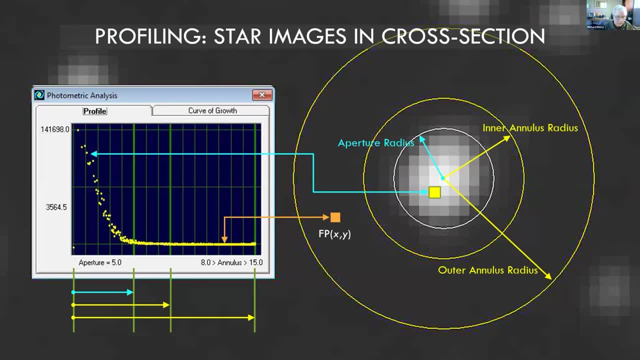 And in the profile what we do is here's our aperture, inner and anulous, in and outer annually, And these in this graph we're moving radially outward and plotting each pixel. So this pixel here, which is it about radius of two, gets plotted here. 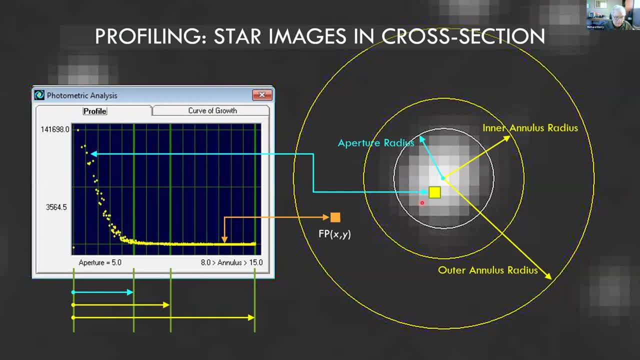 Okay. So if you look at the lines, it'll be like one and a half or something like that. So, And then a pixel out here which is quite far from the the center of the star image. it will get plotted out here somewhere. 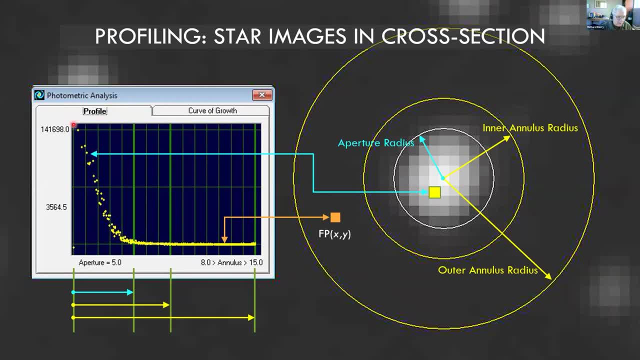 And you can see then that the star has a profile- Okay, and that profile is characteristic of every image in the star, And you can see out here that the annulus- it's clean as a whistle. This is absolutely beautiful. We love it when there's no other stars hanging out here to mess up our measurement of the background sky. 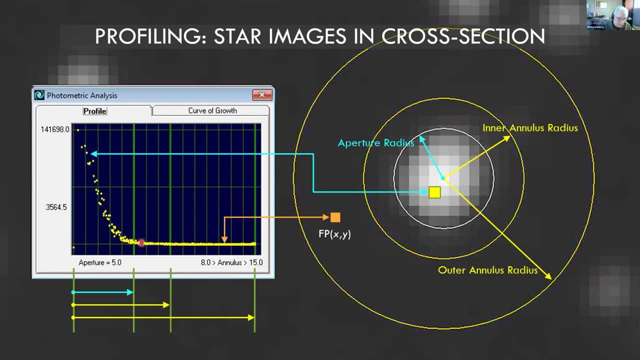 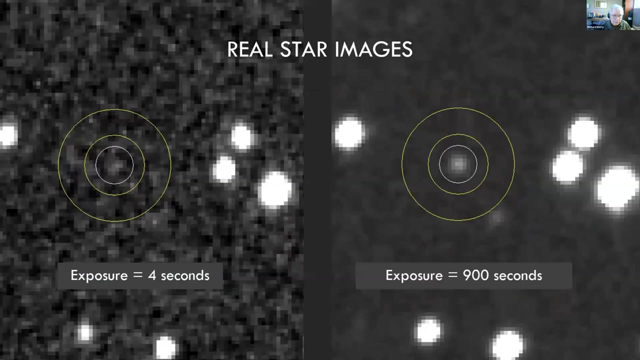 And you'll notice, if you look carefully, that there's still a little bit of starlight out here in the gap. Okay, and you can see that too. You can see these gray pixels. So we will be using The profile as a diagnostic for whether we're getting good photometry. 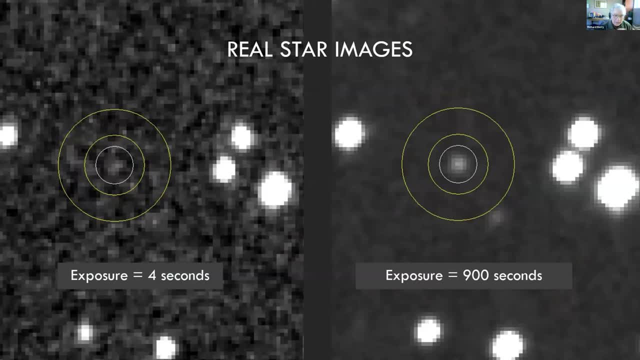 So i'm going to start out. Okay, if you do photometry, you've all seen this kind of stuff. Okay, here's your 4 s exposure and there's a star, And here we have integrated for 900 s And now you can see. 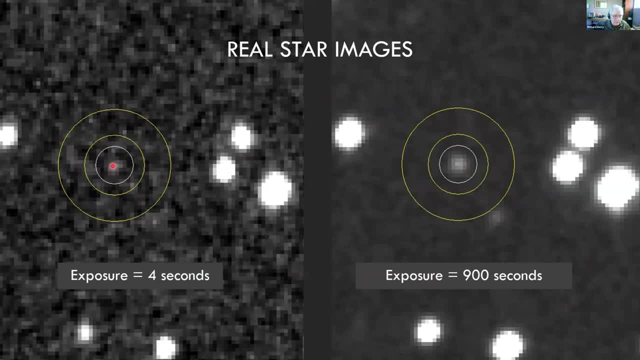 Yeah, this star is really there, Okay, and you can see that. the other stars in the 4 s exposure- These guys look pretty solid. and the 900 s exposures- These guys are really, really solid, because we've averaged so many photons together to create this image. 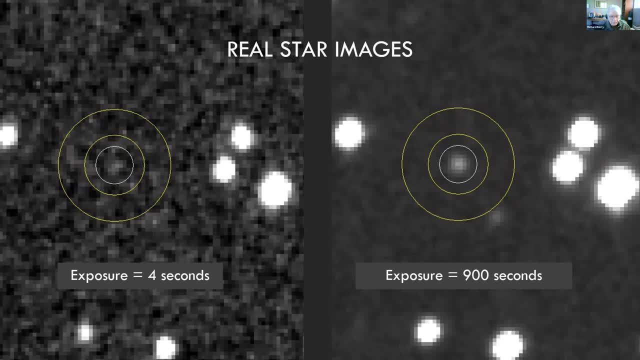 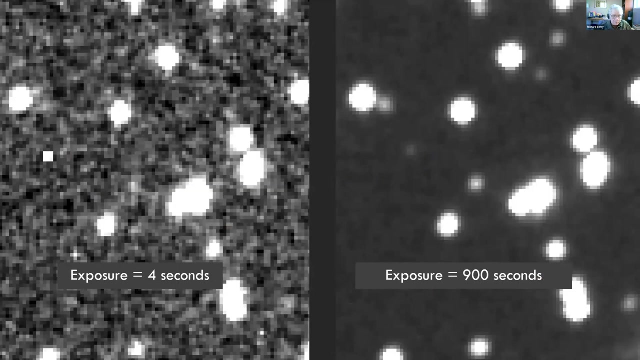 You can see the sky. background is almost noise free. It's really, really nice if you can integrate for long periods of time, And then i'm going to show you a couple more Cases of how star images develop. Okay, here's. here's a comparison of a 4 s exposure and a 900 s exposure. 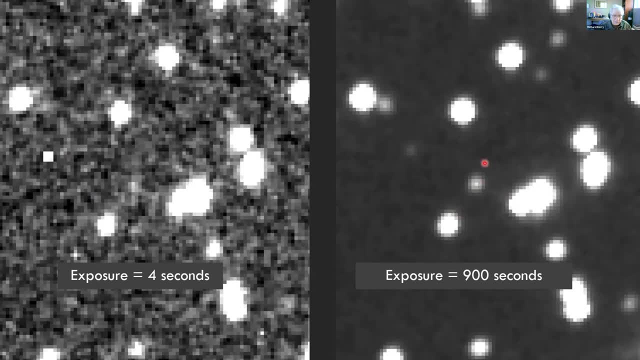 Okay, this guy here, which is nice and solid in 15 s, You can't be sure it's really there. You look at something like this and you say: What's that? Well, that could be a cosmic ray, It could be a hot pixel, It could be anything. 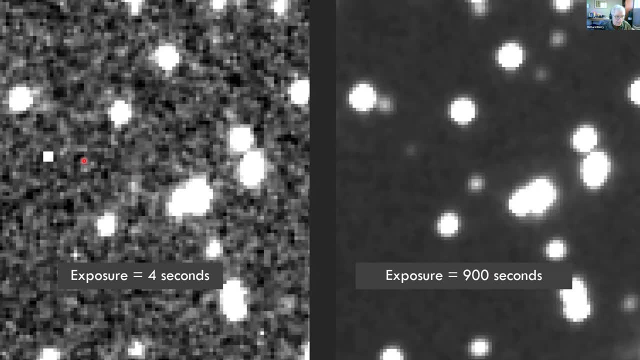 When we look at it after 900 s exposure it's not there. But this image here, which is probably this little cluster of pixels, is there and we can see another faint star and how it develops. It's useful in learning photometry to play around and compare. 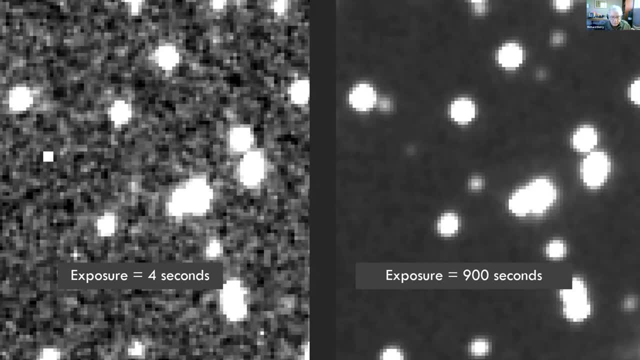 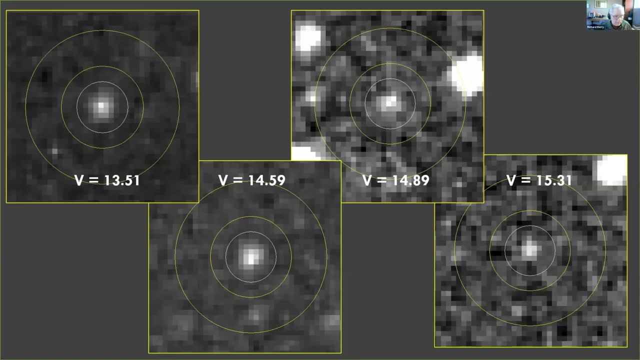 What kind of images you get with different kinds of exposures. So you get to to know, at a sort of a gut level, What good photometry looks like. So here is a thirteenth magnitude star. Here's a 14 and a half magnitude star. 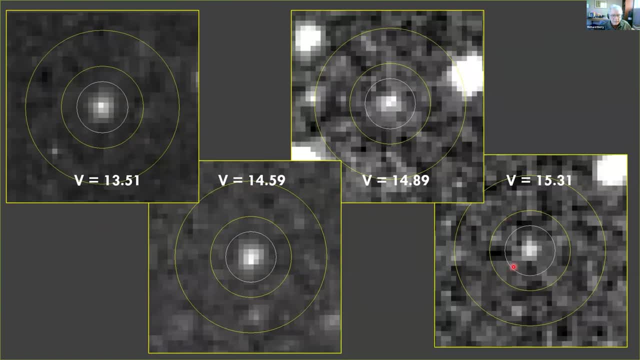 Here's what the star looks like as we're getting down to fifteenth. and here we are down, halfway down fifteenth magnitude. This little telescope which is has an aperture of 114 mm. You can work reasonably well to fifteenth magnitude and in a pinch you could be going down to sixteenth magnitude. 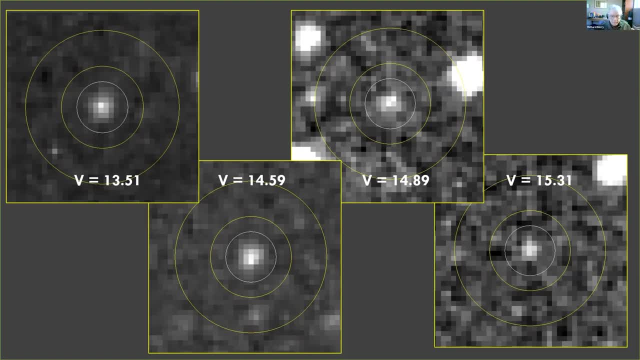 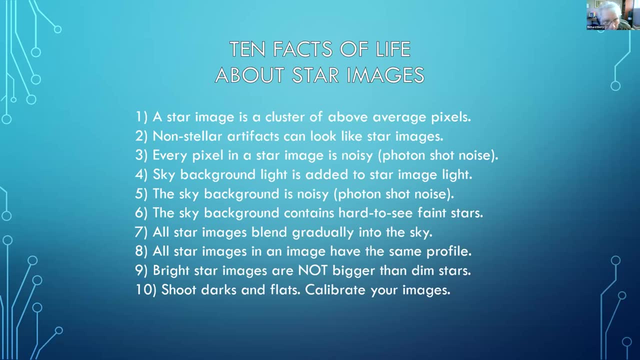 So we we've looked at some stars now and i'm going to talk about the, the facts of life when it comes to talking about star images. This is a birds and bees of stars. Okay, Start, and this will sound maybe a little overly academic. 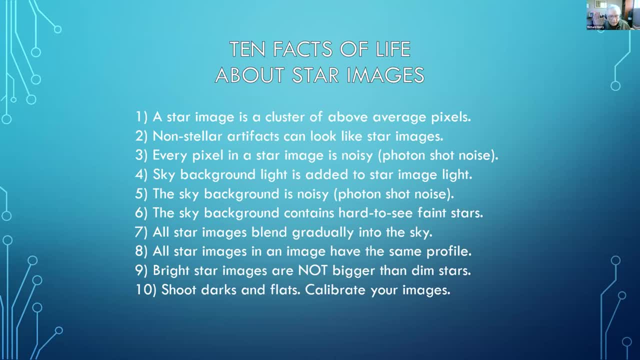 But when you're a computer programmer, you don't look at the start at the image and say that's a star. Okay, it's a cluster of pixels that are brighter than the average of the sky. That's all they are. And remember, pixels are just numbers in an array and that's how we're going to treat them. 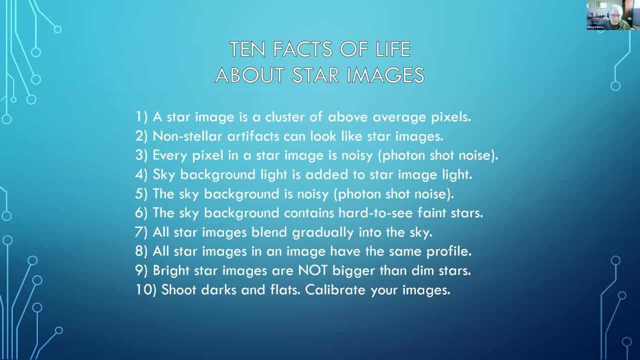 Okay, Non-stellar artifacts can look a whole lot like star images. You always have to be aware that there's cosmic rays, that there's beyonds flowing off of the cover glass on your Ccd. There's all kinds of of things that can make things that look a lot like a faint star image. 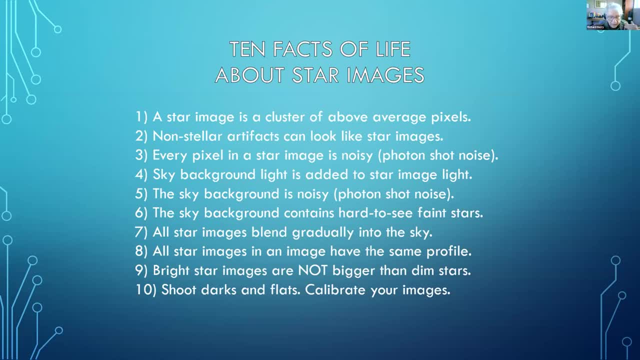 Every pixel is noisy. Okay, Because it's not just a magic number that happens. It happens because photons flowing in randomly vary and it the variation is is uncertain by approximately the square root of the number of photons that it happened. So if you have 10,000 photons coming in, it's going to be 10,000 plus and minus 100 square root of 10,000.. 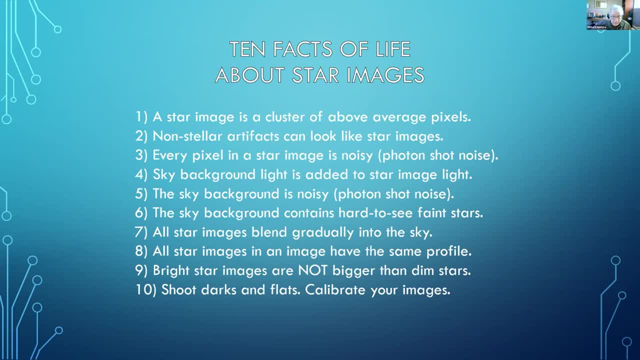 Okay, The sky Background light is added to the sky Star light. Okay, The sky background itself is noisy. It's again photon shot noise, And when you look at these images you always see those that randomly look. If we brand a movie of a series of frames like that, it would look all swarmy. 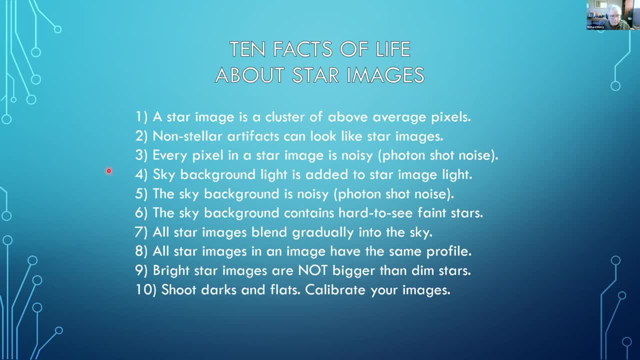 It would look varying up and down crazily. The sky background always contains faint, hard to see stars. Okay, There's always parasitic stars in your background And what they do is they make the background brighter. Now you can say: well, on the average, there's going to be a faint star underneath your bright star, which is perfectly true. 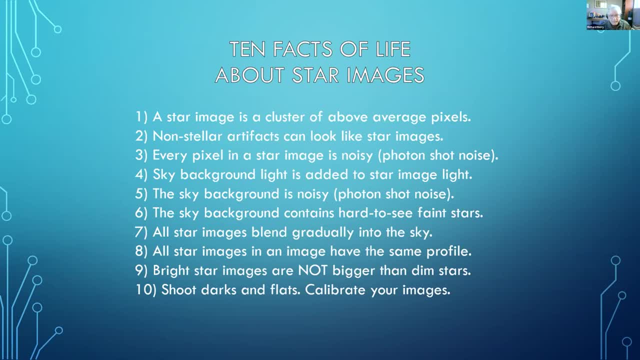 But you're going to be. every time you do photometry on that star, you're going to include that faint star in it. What we don't want is to have a faint star in it, Okay. What we don't want is to have the light of the sky background included every single time. 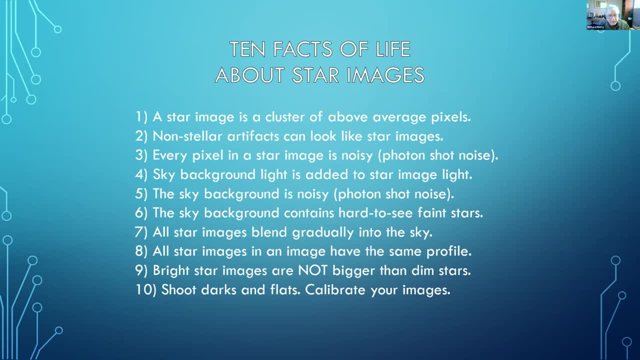 Okay, All star images blend gradually into the sky. They do not have hard edges. Okay, They fade away And if you do a really long exposure, you can find star pixels out 10, 20 pixels away from the center In any given image. all star images have the same profile. 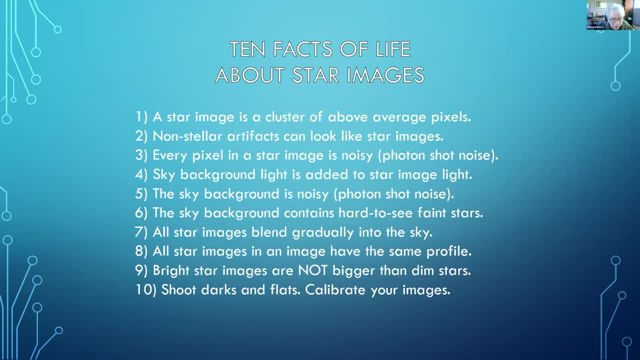 Okay, This is contrary to what your visual. the way you see it visually, It looks like bright stars are big, faint stars are little. They all have the same profile. In other words, a bright star spreads out quite some distance, So do the faint stars. 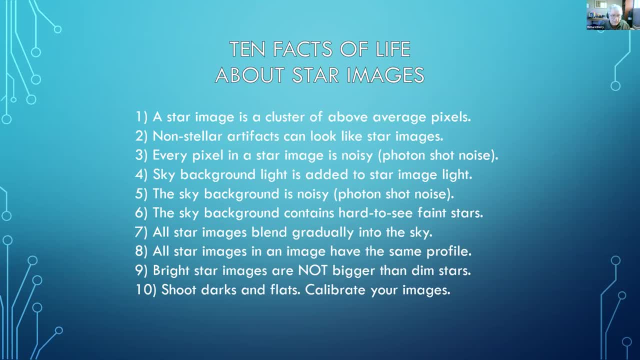 Bright star images are not bigger than your dim stars And when you're doing photometry, shoot your dark, shoot your flats. calibrate your images because you like at least to get your pixels all normalized to the same sensitivity and you'd like to get rid of hot pixels. 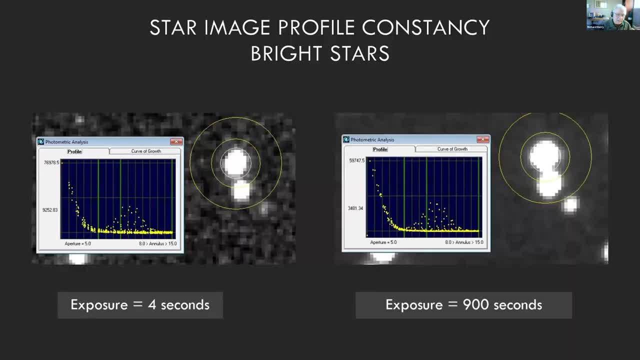 So I'm going to, you know, beat on this a little bit. This is star image profile constancy. I'm going to use my. Here's my four-second exposure, Here's my 900-second exposure, And I've got this little trio of stars. 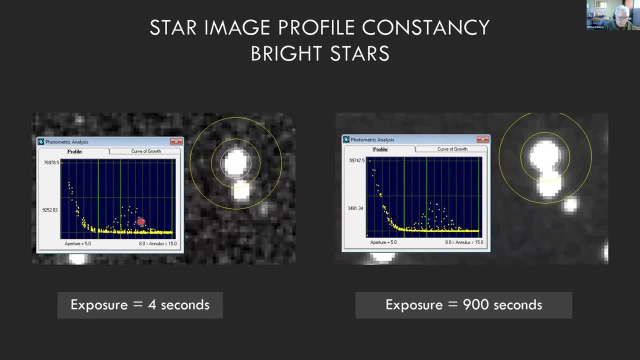 And they begin to show you how you work with the profile too. Okay, So here's your profile. It comes down In the four-second exposure it looks like this. In the 900-second exposure, it looks like that. the takeaway lesson here is that, whether it's a four second exposure or a 900 second exposure, 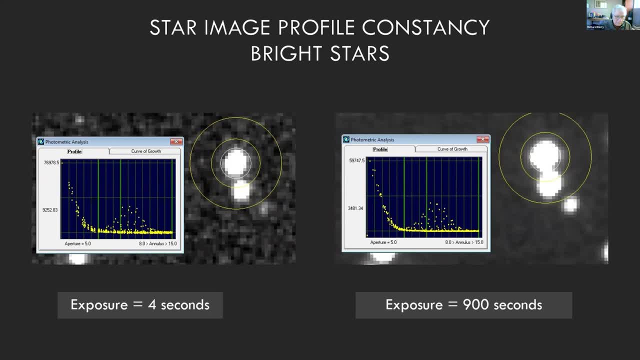 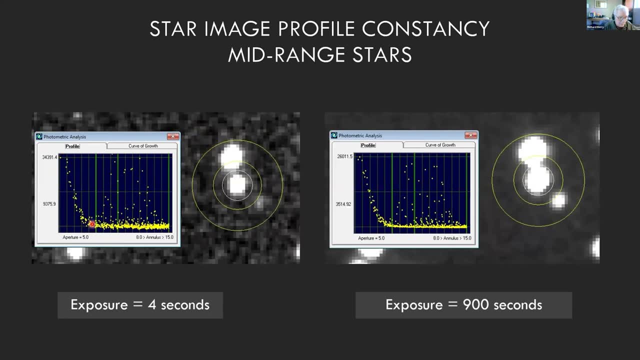 the profiles are the same. now that's a bright star for a medium bright star. once again, the profile is here, the profile is here and now this guy- he's picking up that guy and you can see the annulus is is um, highly compromised. it's got a lot of background star light, but if you look at it, that star is only maybe 10 percent. 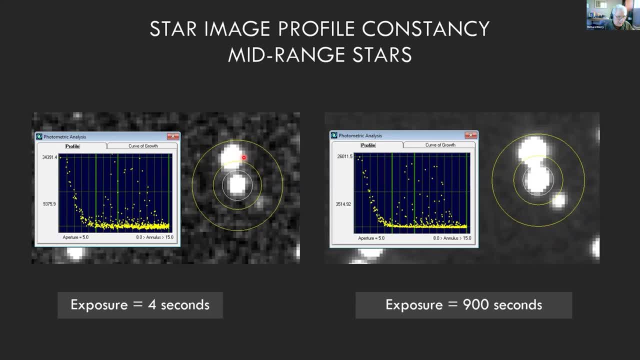 of the total amount of light that's coming into the annulus. if we can figure out some way to get rid of those, we'll have an accurate level, background level, that we can subtract. now here's, here's our, our gap again coming in handy and you can see that there's some light in that gap. 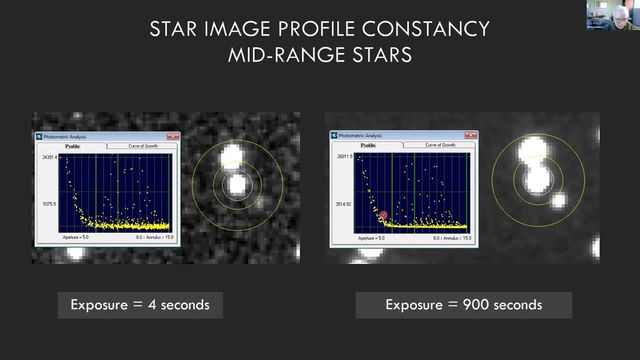 but look at this carefully and you can see, uh-huh. we have chosen our aperture radius so that we get very, very little parasitic light, and that's what we want to do, and it should be perhaps obvious by now. a corollary is of this: is you're going to shoot your bright? 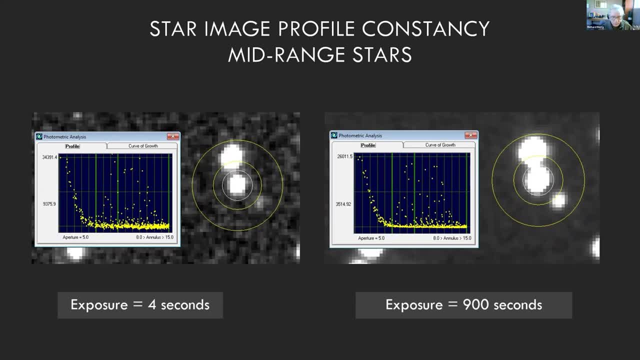 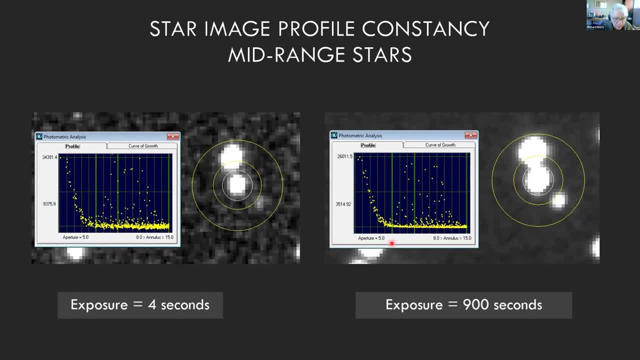 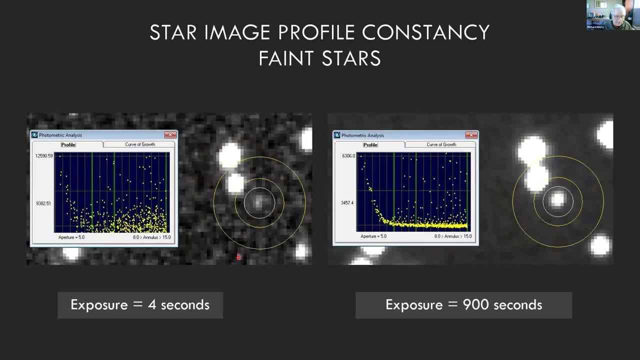 be getting more or less light from that star and you're going to be more or less light from parasitic sources. and then look at this, this faint star. okay, well, here is your profile again. okay, here it is in the four second exposure. it's messy. and here it is in the 900 second exposure and you can see now. 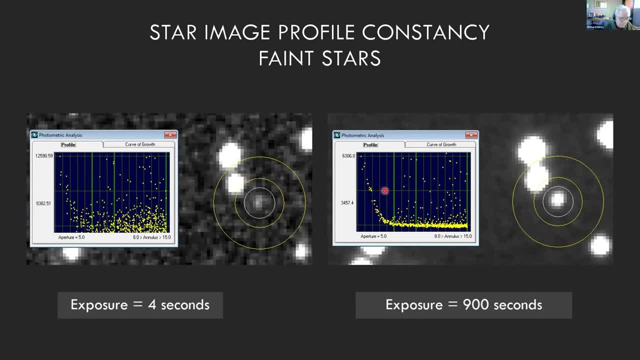 you got the the parasitic light from this guy and you've got the parasitic light from this guy and you can say, well, but that profile is there. and this is why you want to keep that constant, because you're trying to make your photometry the same regardless of the exposure. 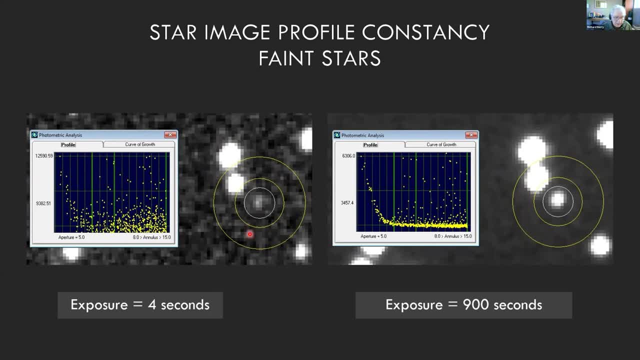 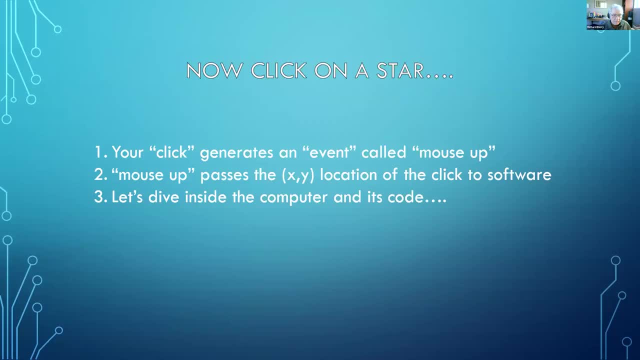 because, even though it doesn't look that way, when you analyze it technically, it turns out to be that way. so we're going to click on it. we're going to walk through the process now of what happens when you click on the star. so i've i've talked about stars and i hope that, uh, you will, you will bring up your. 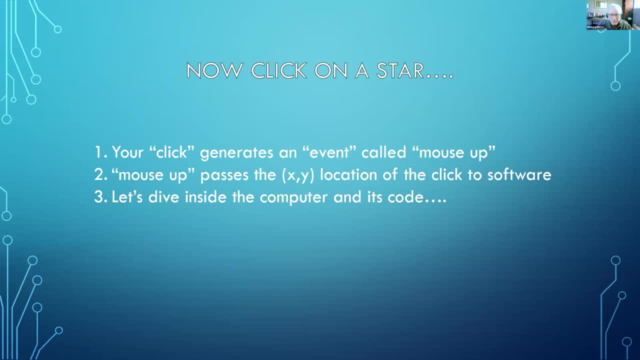 star images and blow them up to 800 or 1000 or 1600 percent and look at your stars carefully so you begin to understand it's dead. it's down at the pixel level that photometry happens. so we're going to click on a star. 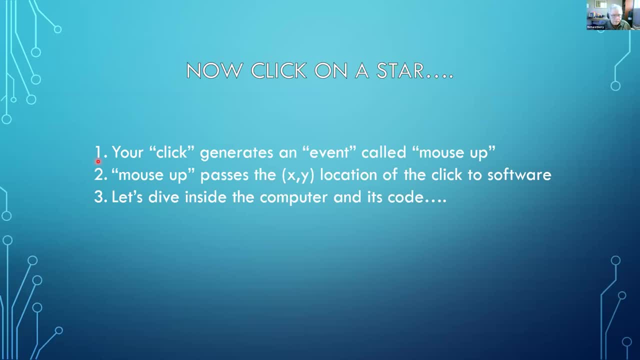 and in computer lingo my click generates an event. in gui type programming it's called mouse up, it all. actually, it creates a mouse down and then a mouse hold and a mouse up event. okay, we're going to trigger on the mouse up event and the mouse in the mouse up event. 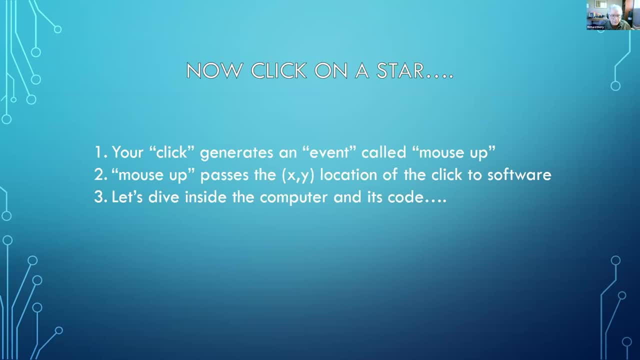 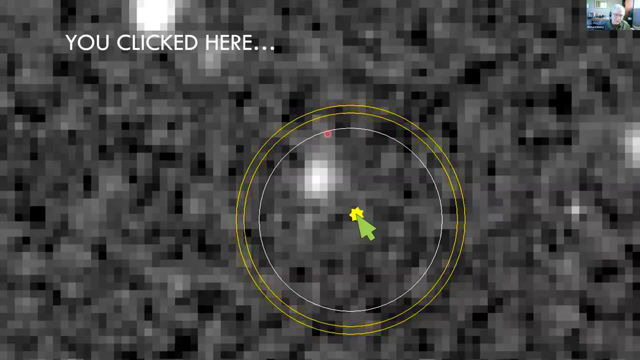 we grab the xy location of where you clicked. now we're going to dive into the software and bingo, you click there, click, okay, here's the star. you want a photometer, but you know, your hand shook a little bit. or the software which is looking at 500 images in a row and 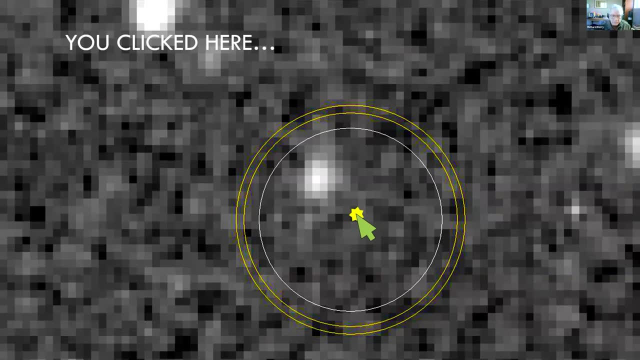 the stars are moving around a little bit or your tracking wasn't perfect. you're going to have to follow that star. so the software thought in the 399th image that the star was here, but in the 400th image the star had moved over to there. 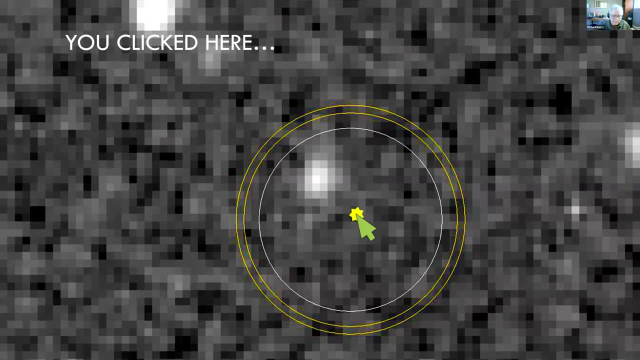 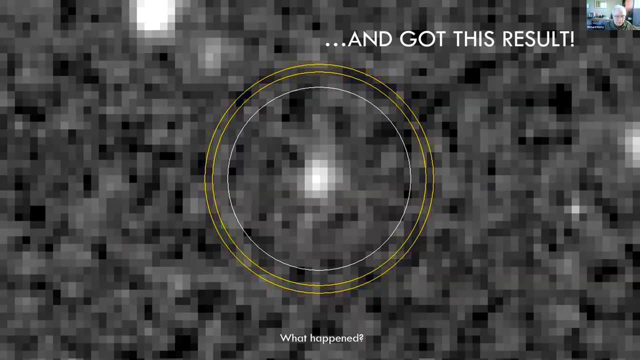 okay, so this was your starting point. you went click and here's what happened. the software figured out where the darn star went. well, this is really handy because you know you try to put your your mouse on the right spot and click there. you can do that pretty well. 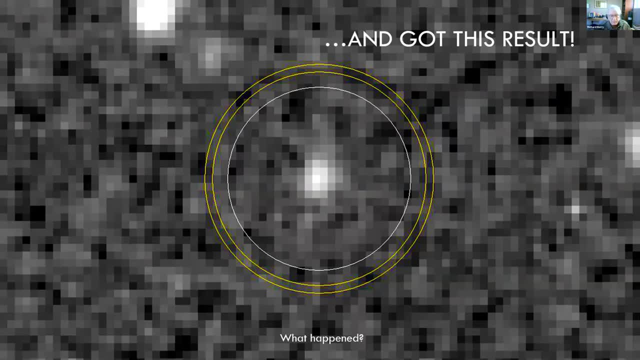 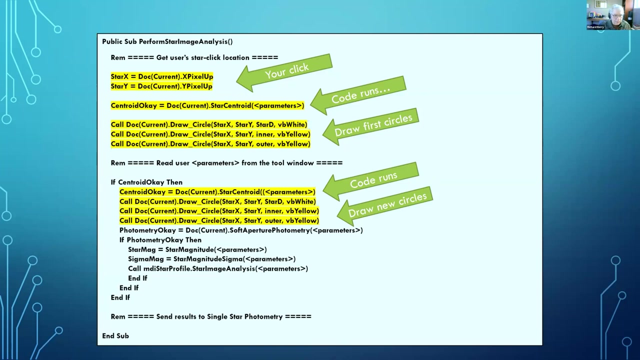 but you can't do it at 100 typically. you really do need to magnify it the way we've done it here. okay, now we're going to dive into computer code and i've done a this very slightly kludgy stuff here. because of the code i'm showing you and the code that was generated, that image is not exactly. 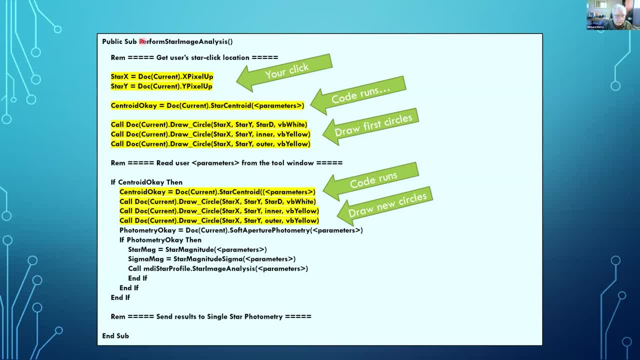 the same um, okay, but you can see that it's called a rpv. if you're allergic to computer programming, you know. i'm sorry, but this is the. this is. you know, it's like lifting the hood and looking at the carburetor and the distributor and the battery and the radiator and all that. 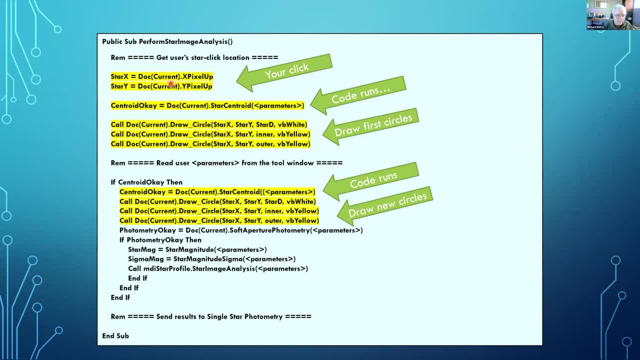 that stuff that's under the hood. so this is the code that generates this is my click and we get an x and y value and we then run code that determines where the center or valley is when we find itモ run code that determines where the center of light is and it draws the circles. so it draws. 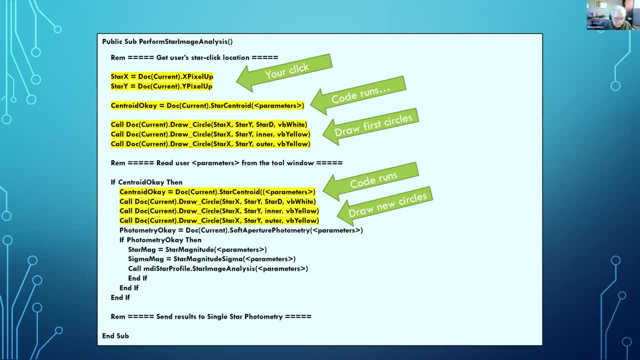 a white circle and two yellow circles. okay, so there's the white circle and there's the two yellow circles. then the the code here says: okay, i've just figured out where the center of the star is, and then it runs it again. okay, this time. on this, on the result that has come out of this, 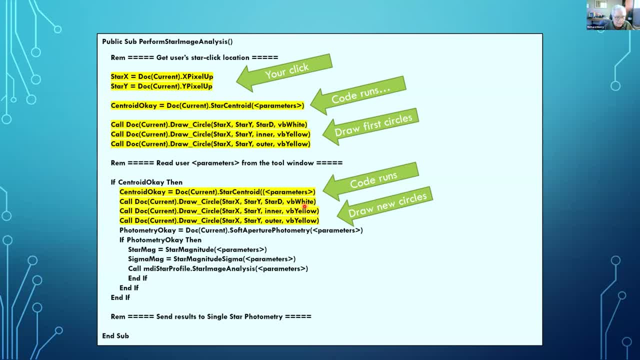 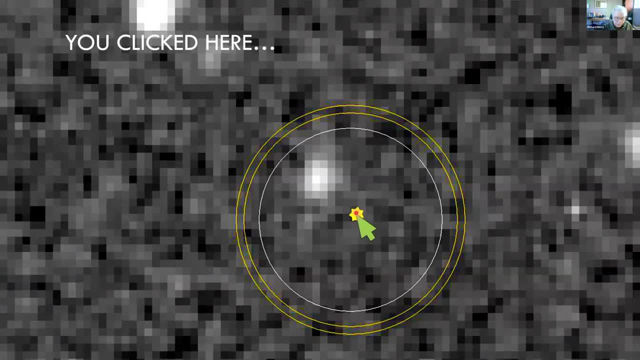 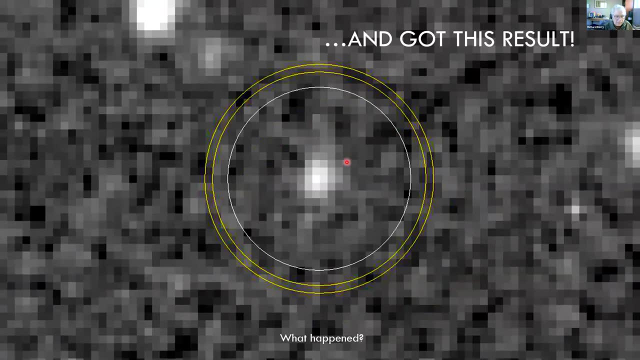 first centroid effort. so now we run it again. now we're centered and it draws them again. so this is your first time that piece of code runs right. it just draws the circles for the click. then when you get that second one, it zeros in on this guy. now where i've 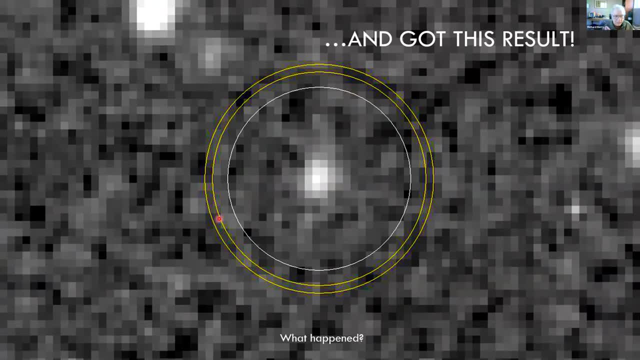 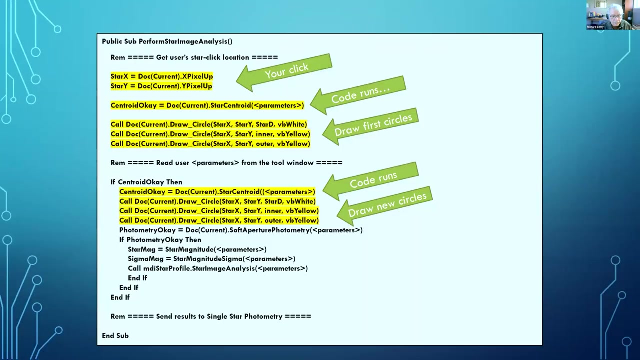 clued a little bit is in this drawing. i don't show it, but we, sneakily, are going to change. we change, change the aperture. so the aperture is actually here. it's smaller. we're looking at a smaller area, okay, so now introduce another programming concept. if you're not familiar with code. 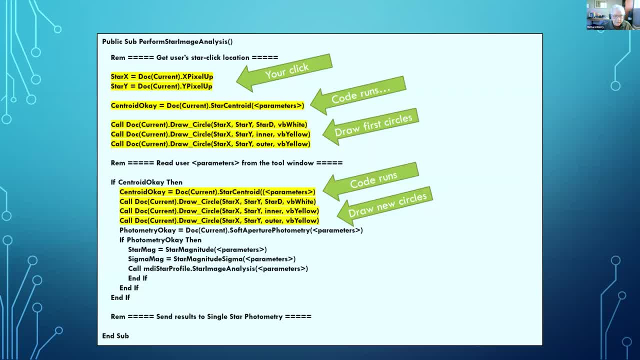 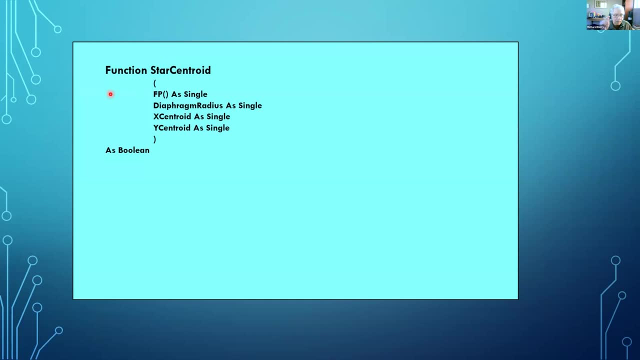 and that's called a function. okay, and that's what we did here. this we we called in the current document, we called the function star centroid and the code is here and the first thing it does it says: okay, these are the things that i'm going to put into my computation first. 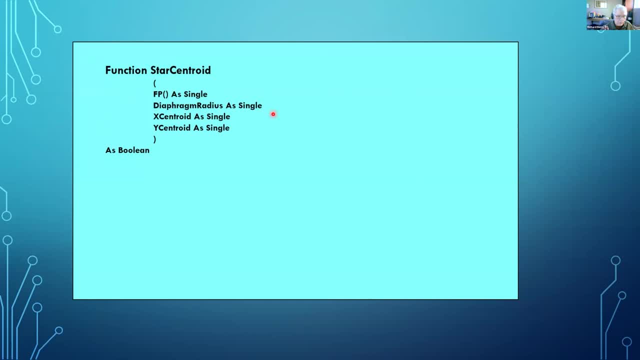 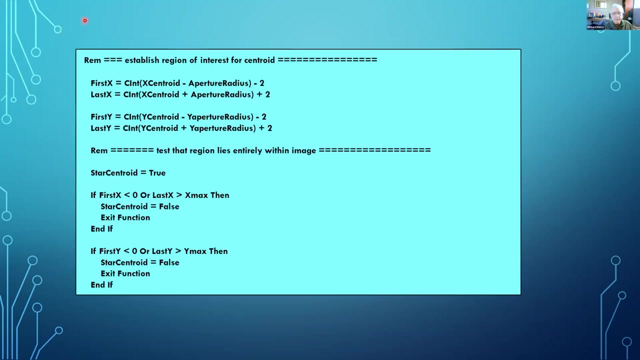 of all, i'm going to put the image in, then i'm going to put in the diaphragm radius, that is, the aperture radius, because we use, okay, and i'm also going to put in my click value for the centroid. and then, remember we, the software does not know where that click came from. okay, it doesn't know. 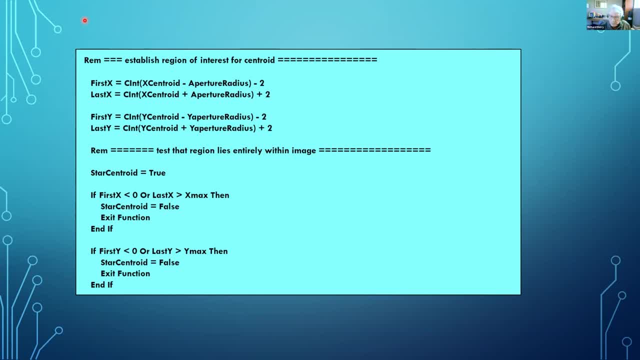 whether there's even a star there, because we don't use the centroid function only in this instance. we may be using it in some sort of automatic tracking routine. so the first thing we want to do is we want to map that screen. so this is where the start point is and the end point is, and this is where 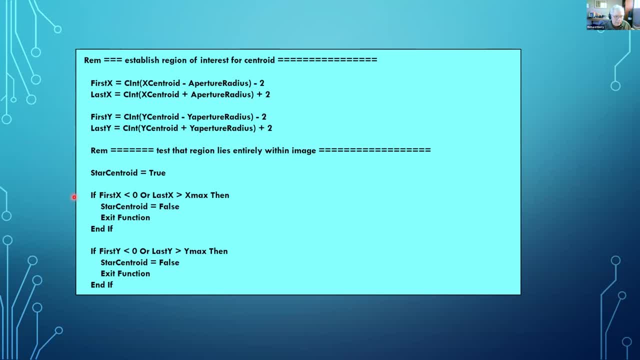 the end points comes from, and the first asset within that last asset is function action, and that would show if iition stands and the last action point in the list, control. okay, and so what we're gonna look at here is the our feature of function action being limited, because 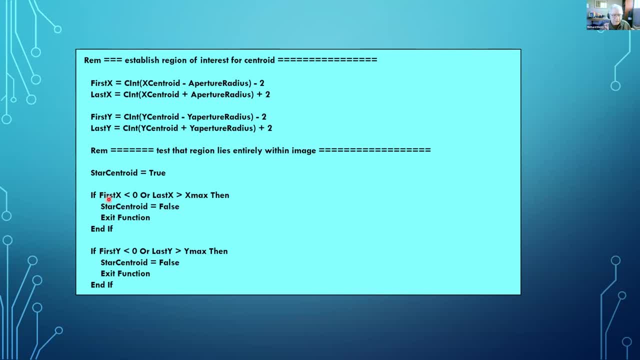 citizen access data only allows the detection of the motion, whereas an action is money wasted, as you can imagine. but at the IT component, it's really important thatuno retrip, as you can imagine, you're trying to find the function to keep those. if you go to space with you, it all has to и y max and red somethiq to бу jz that yaum ai. 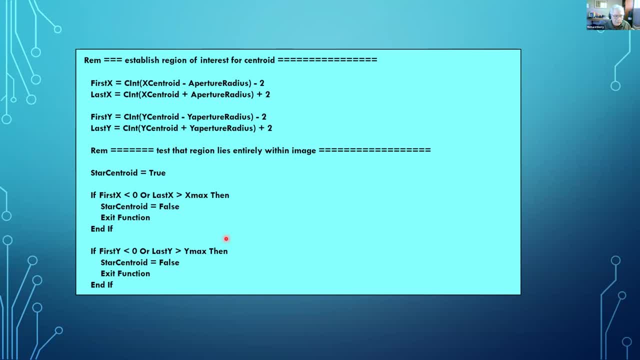 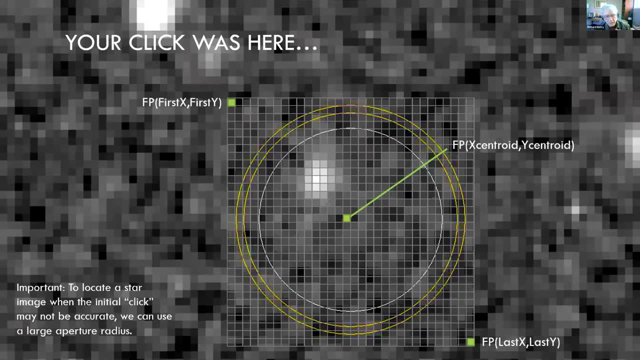 Steven Linthicum A. Sorry, let's get this right, Steven Linthicum A. It goes from X min to X Max and so forth. in other words, it's inside the image. that's a check. it's a necessary check, because if you don't do it right, you can get horrible things like divide by zero and boom, the software crashes. so 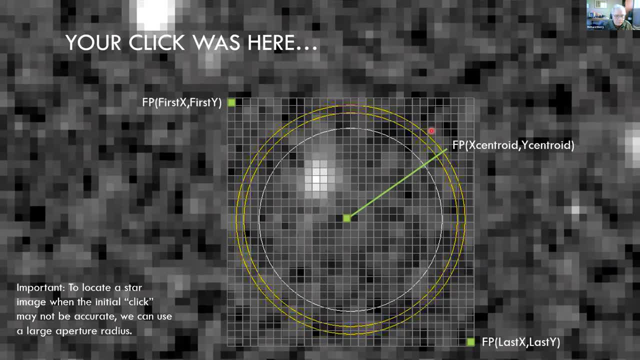 Steven Linthicum A. My click was here: Steven Linthicum A. The code runs and it defines this region from Steven Linthicum A- fp first x to fp last x. now i've sized this region to be bigger by a small amount, by, in this case, two pixels than the aperture that i'm going to be looking inside. Okay, and this is where my, this is where my click went in. 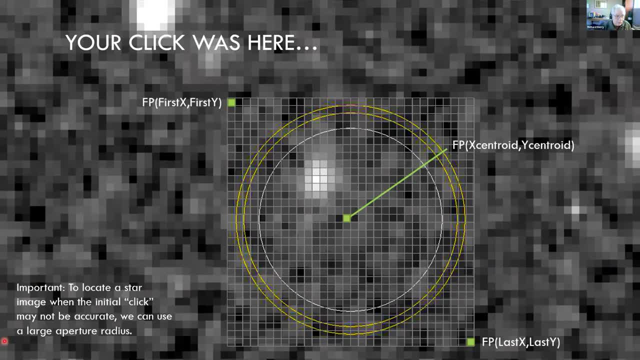 Steven Linthicum A And it's useful. you don't. for this to work well, the initial click does not have to be accurate, but it's useful to be able to see the Steven Linthicum A Accurate. that's why we're doing the centroid stuff, because we, when we're going to do the time atry, we really want to know exactly where the star image is. 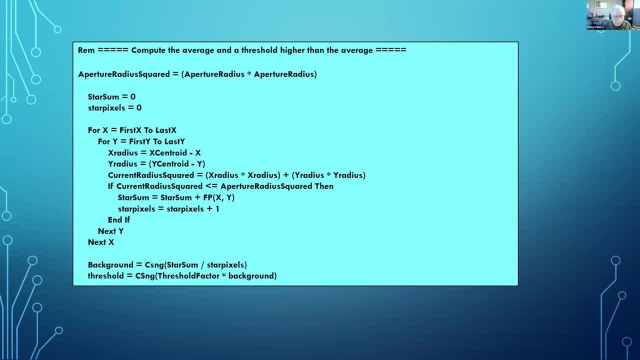 Steven Linthicum A. So the next thing we do, Steven Linthicum A. Let me back up a little bit. Okay, whenever you see if a structure like this, for X equals first to last, and you'll notice this, for for X equals, and then there's a next X. 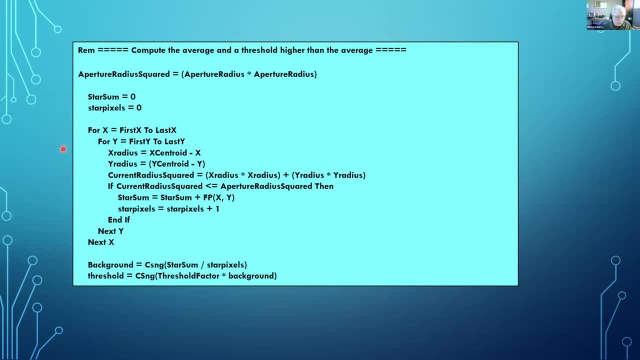 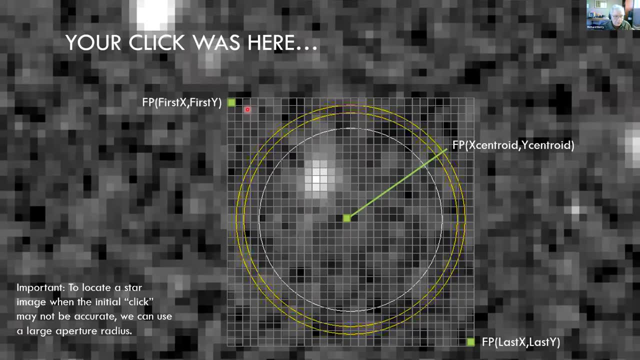 Steven Linthicum A. This is a loop, so the software is going to go around and around Steven Linthicum A And it's going to do this routine inside for each one of those. so what it's doing is it's scanning down the image and checking and it's doing a calculation: is this pixel inside or outside? if it's inside, we're going to add its value. 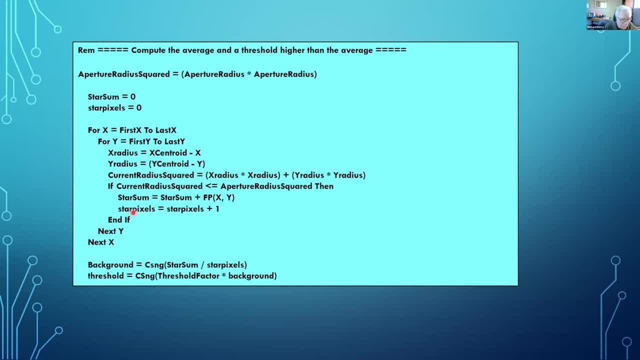 Steven Linthicum A To the total, and we're going to add the number of pixels we're going to. we're going to increment that by one. so what i'm doing is i'm computing the total, Steven Linthicum A, The average value of the of the background, the star sum divided by the number of pixels, and then i'm going to compute a threshold value. 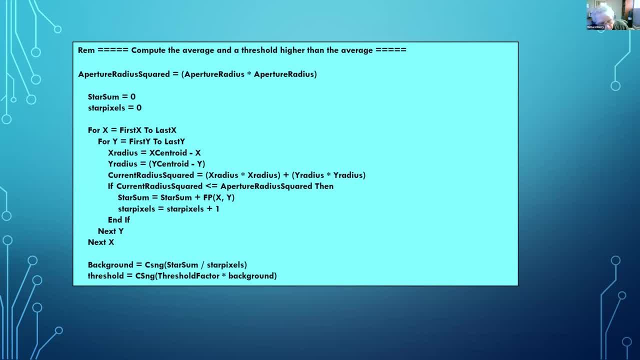 Steven Linthicum. A Something that's a little bigger than the background might be 20% brighter than the background, or, you know, 2% brighter in the background. this is something that the programmer determines by trial and error what gives good results. so this is: 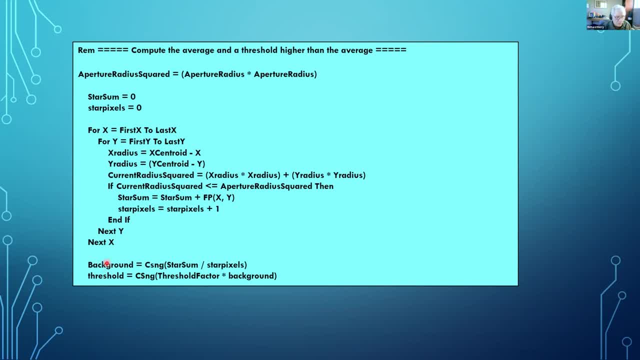 Steven Linthicum A secret number. that's Steven Linthicum A, hidden inside the code. so we're going to get a background and we're going to get threshold. so that's what this routine done. it did. it produces these two values. 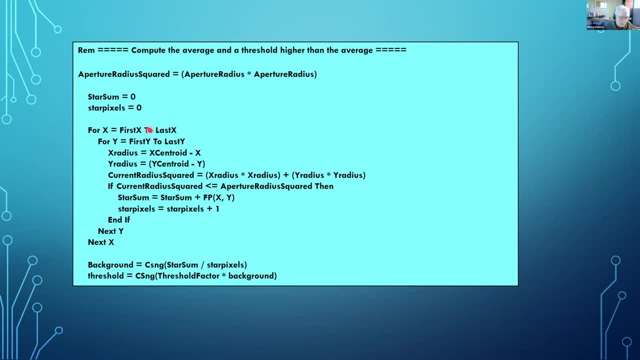 Steven Linthicum A. Okay, now programmers in the audience, you're going to say like wait a minute. you know you have this loop again and again and again. that's very inefficient way to code this kind of work. Steven Linthicum A. And the answer is: this code was written to be very easy to explain to myself. 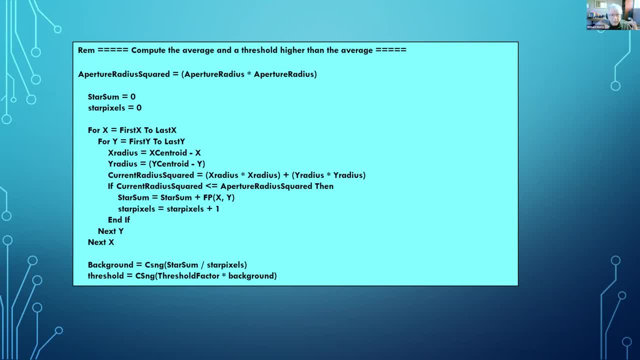 Steven Linthicum A. So I could Steven Linthicum A- be sure as I was when I was writing this- that actually did what I wanted it to do. and you say, wait a minute, you're writing it, you should know what it does. 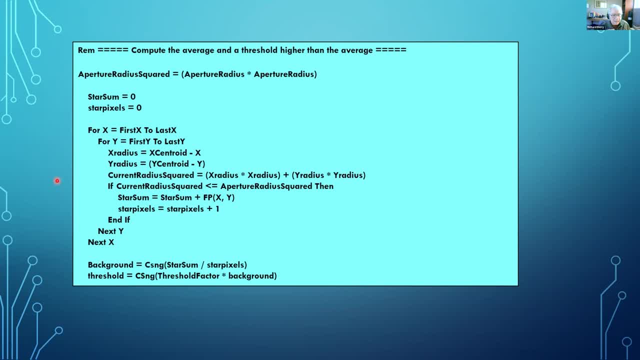 Steven Linthicum A, that's called bugs. okay, it's very easy to get clever and end up doing something like computing a background or a threshold that are not right. Steven Linthicum A. Every programmer knows that. they don't like to admit it. you make mistakes, so this code. 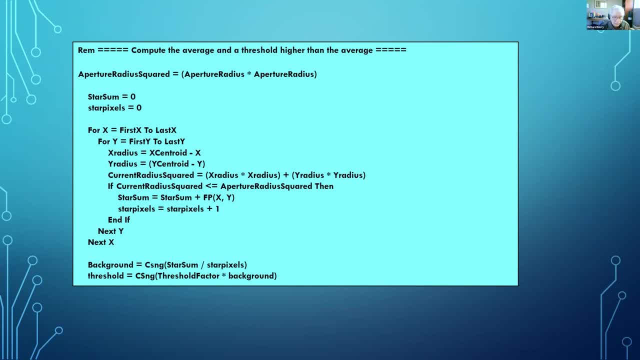 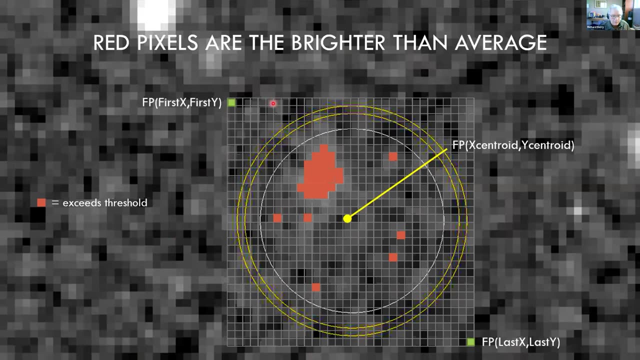 Steven Linthicum A, Which is very easy to explain to myself, is also relatively easy to explain to non programmers. so i'm doing something that's redundant and slow, and my excuses. Steven Linthicum A, there's like 250 pixels here. it did that in in. you know, literally microseconds. you know the human beings timescale is the 10th of a second. so you don't see the fact that i've written very, very. 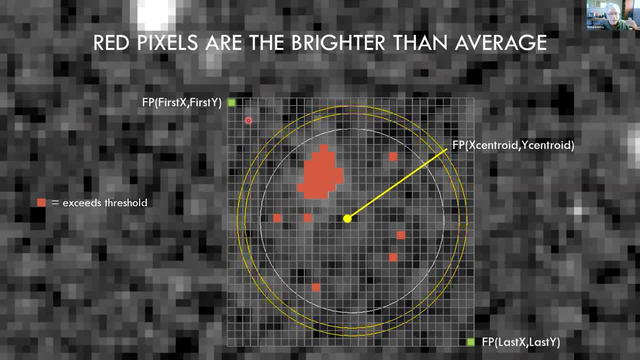 Steven Linthicum A. In effect, Steven Linthicum A In Steven Linthicum A- inefficient code. Okay, so what i've done here, just to clarify what what's going on if a pixel exceeds the threshold, i've colored it red. 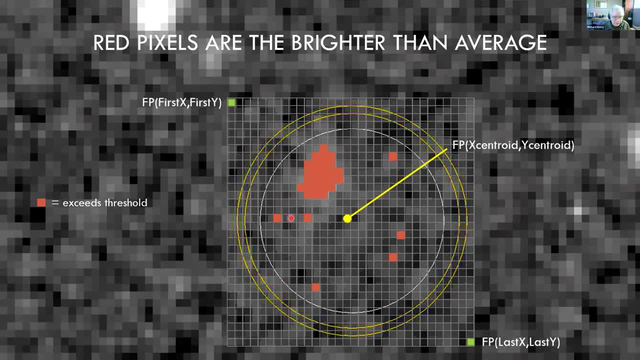 Steven Linthicum A. Okay, so here's the star image. remember him, okay, and you'll see that there's a bunch of other pixels that exceed that value, and here's what the here's what the centroid value was. so i've scanned this whole region. I found these guys that are bigger the threshold. 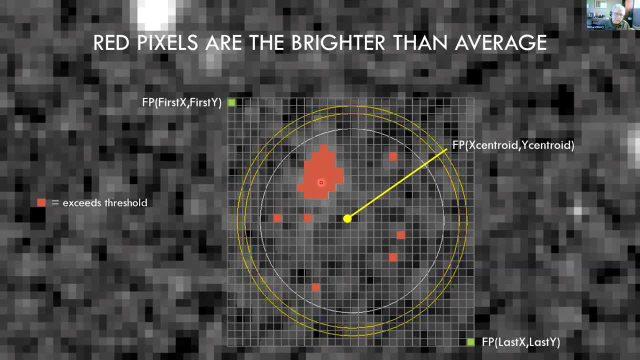 Steven Linthicum A And now Steven Linthicum A. You know we're going. we're going to take an average of these ones that exceed the threshold and say, well, that's where the real Center of the stars, but these guys that are out here hanging around, 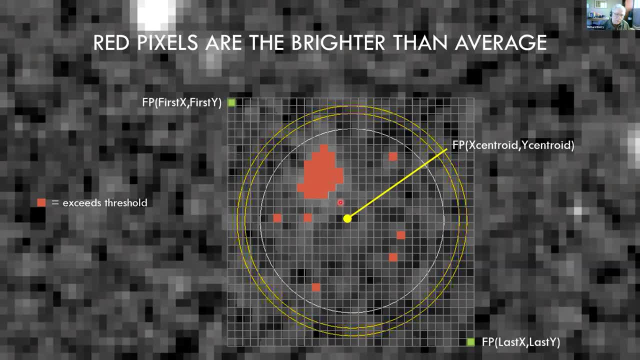 Steven Linthicum A. they're going to throw my value off by quite a bit. they're going to move it somewhere in this direction. I don't want that to happen, so i'm going to apply a test which is called the neighbor test. 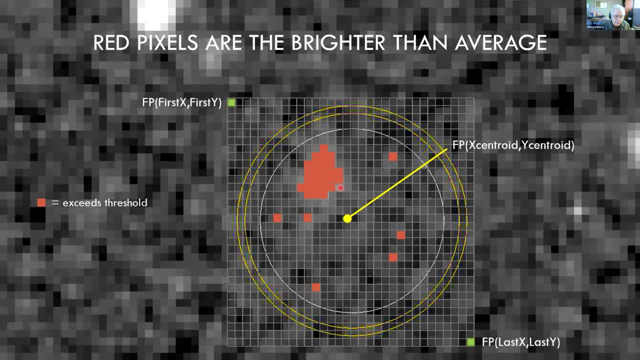 Steven Linthicum A, Which is Steven Linthicum A? How many Steven Linthicum A Plus Steven Linthicum A? Other pixels in the star image? does each pixel touch? okay? well, these guys are above value. so. 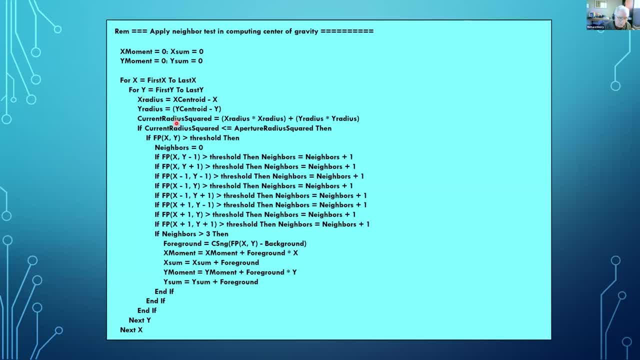 Steven Linthicum A. Okay, here's. here's what that looks like. once again, we're going to scan through the whole thing. we're actually going to do that test again. Okay, so we got Steven Linthicum A A computer standpoint. you know we've got a lot more numbers to crunch, but again, computers are so fast today. 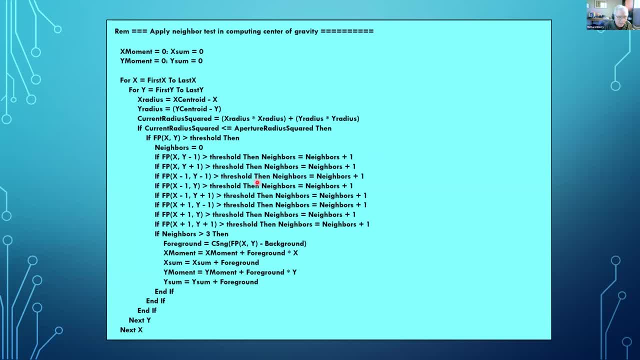 Steven Linthicum A, And for each pixel, Steven Linthicum A, we're going to check and see how many neighbors it has. so we're going to look at pixel X, Y and we're going to look at the pixel below it, above it, to the left, to the right, diagonally, and we're going to see, say, if it has more than three neighbors counted in. okay, measure, two things: one is it's, it's. 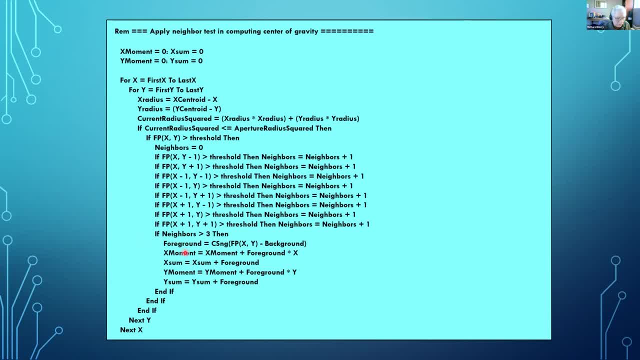 Steven Linthicum A. it's distance: Steven Linthicum A and it's Steven Linthicum A value: it's pixel value. so this is where we we do that and we're subtracting the background skylight off. 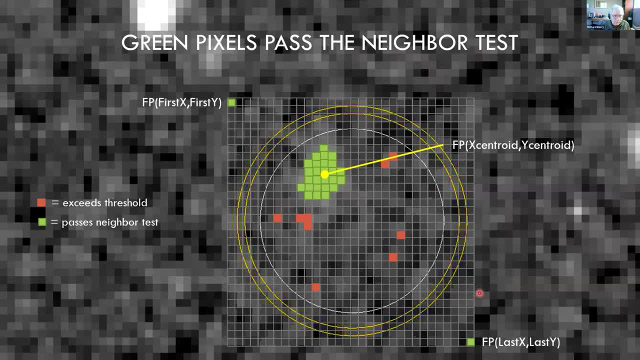 Steven Linthicum A. So if a pixel can pass the neighborhood neighbor test, it's going to be in this cluster. remember, I said star image is a cluster of pixels, Okay, and what we've done is we've said, ah, these guys are here, these guys do not pass, and I 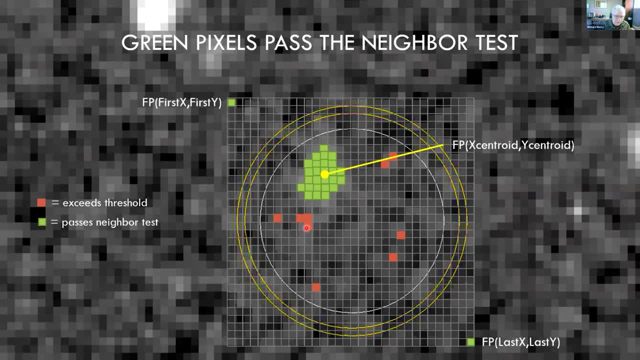 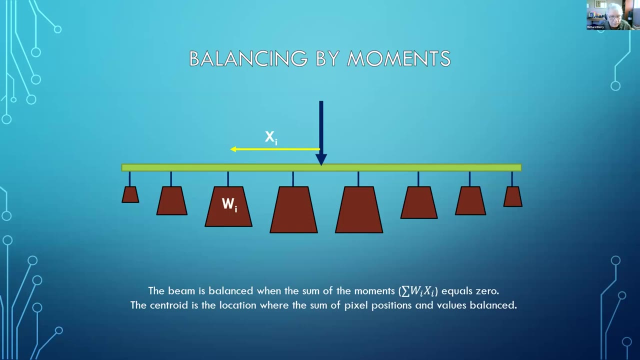 Steven Linthicum A added a couple samples here to show you. each one of these guys has two neighbors. Steven Linthicum A. They don't count, they're not part of the star image. Steven Linthicum A Now. Steven Linthicum A, An aperture of time atry. we find the centroid by balancing by moments, that is. 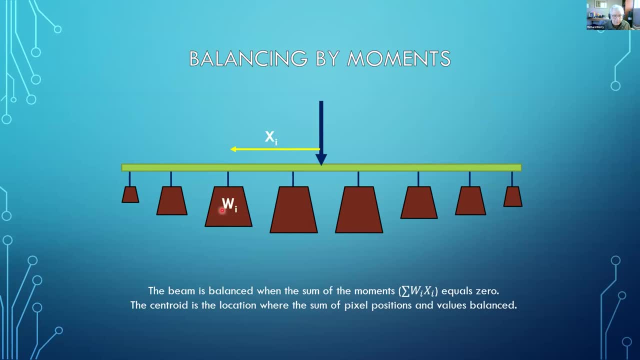 Steven Linthicum A. You multiply the weight of the pixel is pixel value. times is radial distance. Steven Linthicum A From the Center, Steven Linthicum A and Steven Linthicum A From that you can solve: where is this balance point? okay, that's what we're going to be doing here. 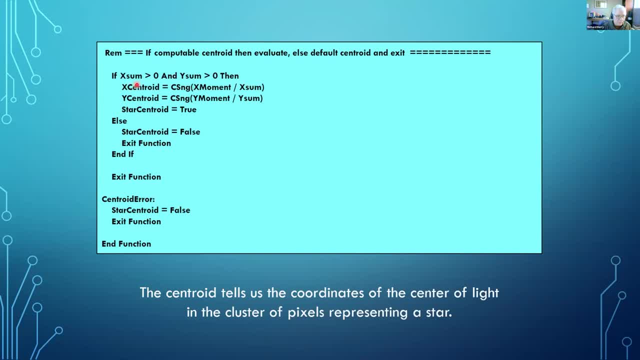 Steven Linthicum A. So we're going to take the moment divided by the sum and that will give me an x centroid, my wife centroid, and we're going to set the value of the function. star centroid is true, Steven Linthicum A. If it's not true, we're going to jump out of. 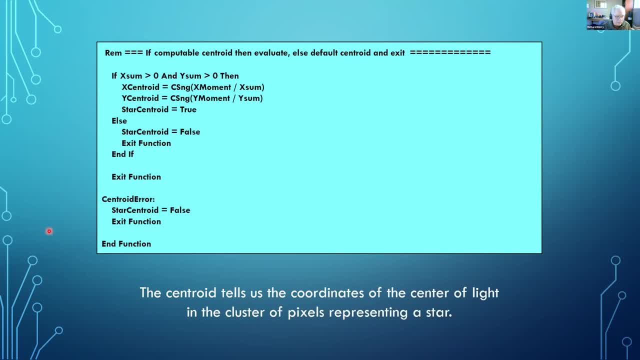 Steven Linthicum A The thing and say, yeah, we failed and if there was an error called, we're going to exit the function to. what the centroid is doing is it's telling us the coordinates of the light, of the, of the, of the Center of the light in the cluster of pixels that represented the star. 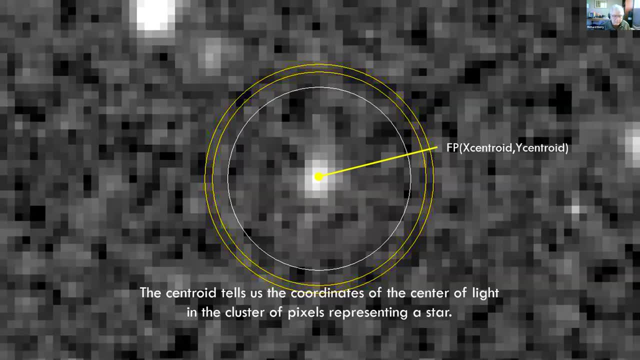 Steven Linthicum A. So here we go. this is the Center of the light. okay, Steven Linthicum A, And it won't be a whole number of pixel, it'll be some kind of fraction. Steven Linthicum A, A good centroid routine. 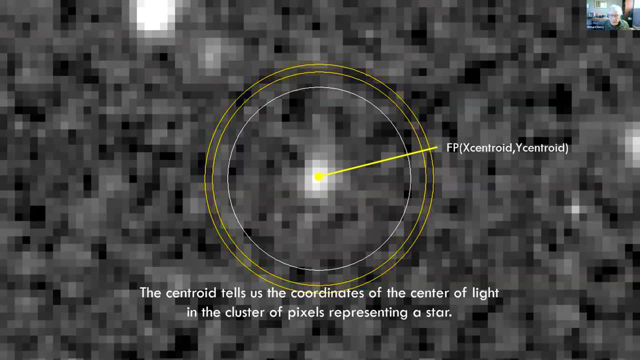 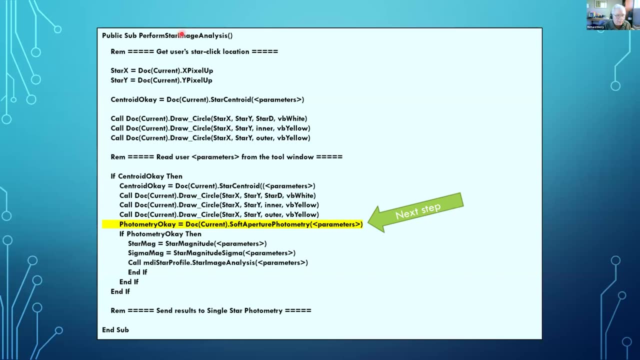 Steven Linthicum A will find the Center of the light, even a mess like this, to better than a 10th of a pixel. Steven Linthicum A. So we're going back to this, this Steven Linthicum A- routine, and saying, well, where are we now? 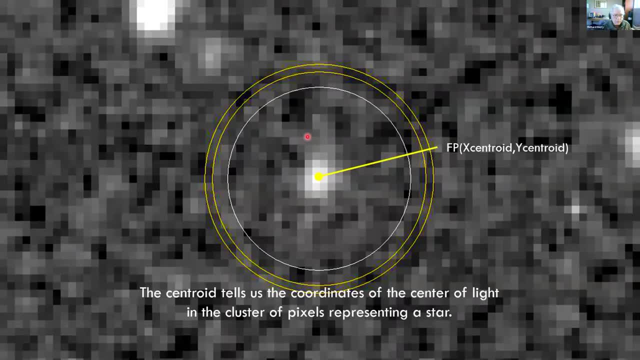 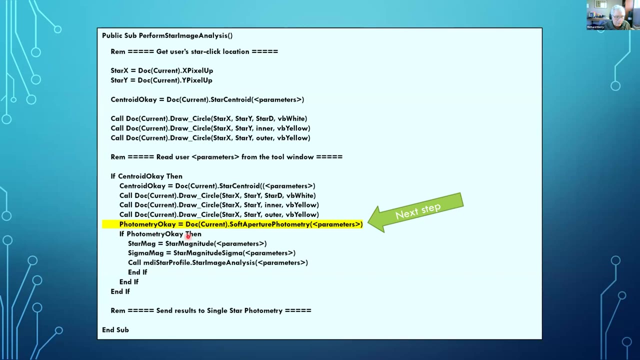 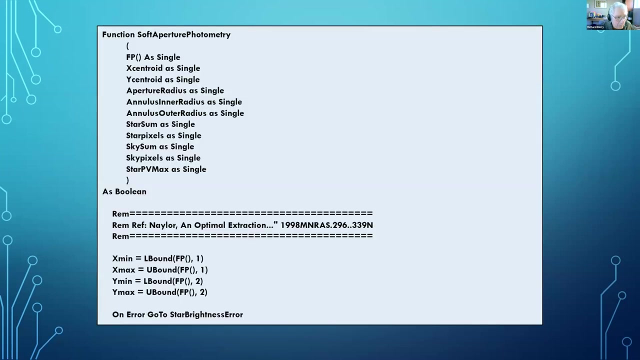 Steven Linthicum A, Because we're distrustful. we're going to run the centroid routine a second time, Steven Linthicum A, To make sure that we got it right the first time. Steven Linthicum A. Okay, and we're going if, if that works, if that, if the time, if the centroid was okay, then we're going to go and we're going to now try to do photometry. so this is what 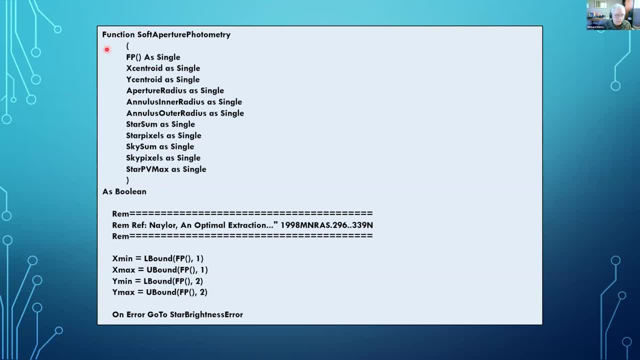 Steven Linthicum A routine called self soft aperture photometry does. the reason I call it soft is we're using an algorithm that Steven Linthicum A uses partial pixels- Steven Linthicum A- To try to find out where the edge is. 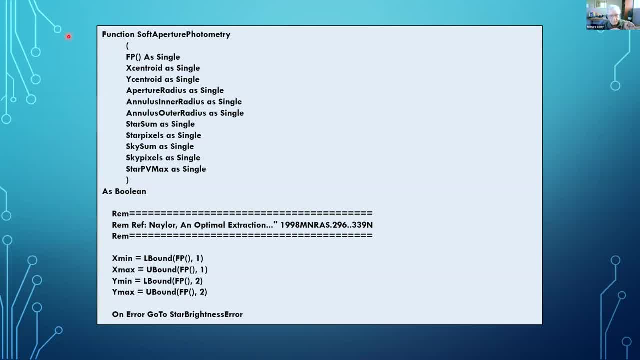 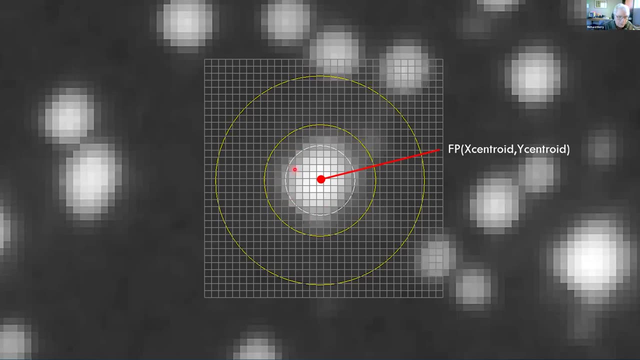 Steven Linthicum A. If you think about Steven Linthicum A, That the star image Steven Linthicum A is not smooth and continuous Steven Linthicum A, As as we would like to think, Steven Linthicum A. Okay, see, it's all broken into. it's a cluster of pixels, so there's going to be pixels at the edge which has starlight in them, which can be either in or out. okay, 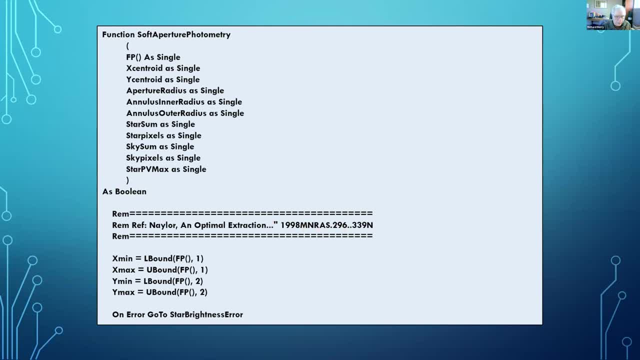 Steven Linthicum A. there's a paper in monthly notices that Royal astronomical society back in 1998.. Steven Linthicum A That I picked up and used for this, and when we define this function, these are the values that are going in. we're going to put all these values back out again. this is the way we wrote this particular code. so 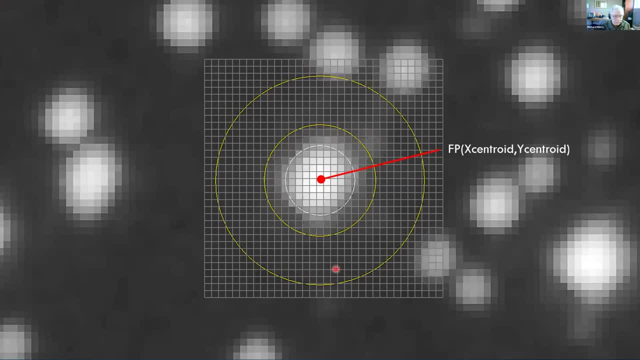 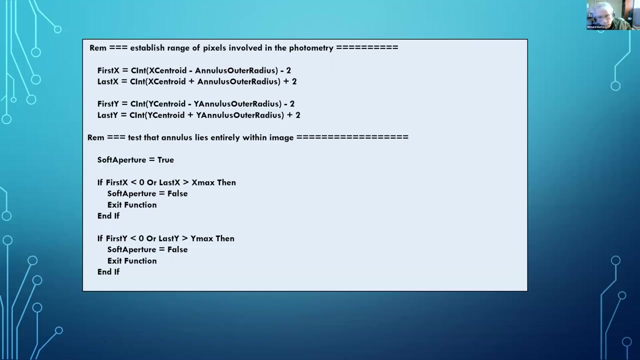 Steven Linthicum A. Here we are again. okay, here's our first and last, and we're ready to scan this and I for this, them for this talk. i've used the much better quality image rather than the the ready looking one, Steven Linthicum A. So, once again, 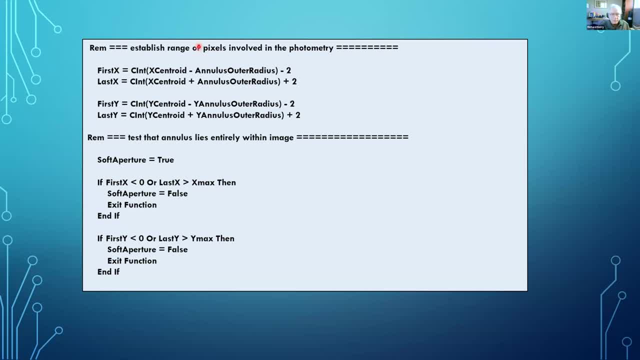 Steven Linthicum A. We don't know where that centroid came from. we don't know there's really a star there. so the first thing we do is we define the region. we're going to be looking. Steven Linthicum A. We set the value of the of the 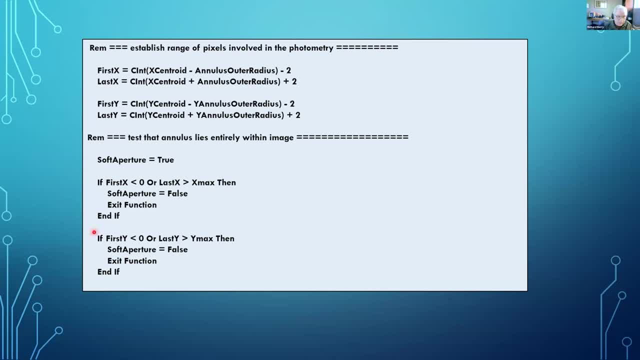 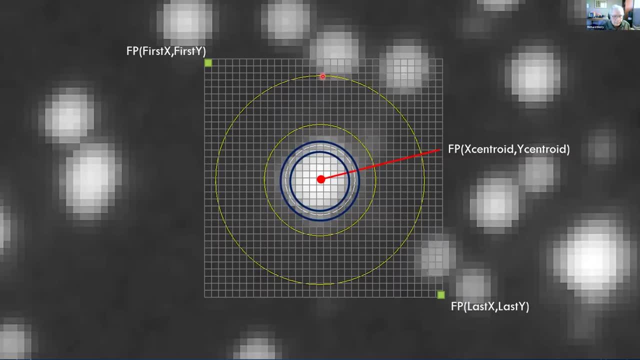 Steven Linthicum A function to true, because we hope it's going to be true and we make sure that it's inside the image: Steven Linthicum A. Now, Steven Linthicum A. In our test Member. we have said, well, okay, we're going to look at this pixel and we're going to say: is it inside this limit limit or is it outside this limit, or is it on the on the fence? well, 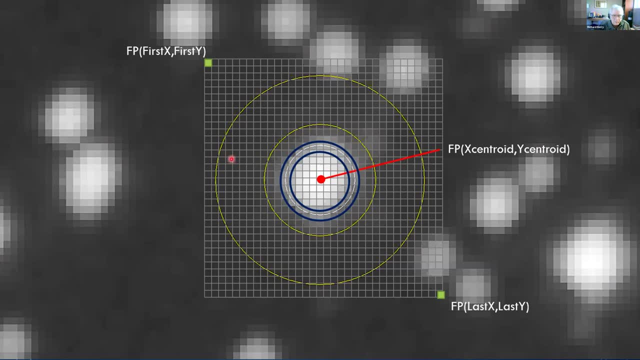 Steven Linthicum A it's. it's going to have to make a decision. so when we look at pixels that are out here in the annual us, we're going to have to make a choice. we're going to end up with jaggy edges. we're going to end up with pixelated edges. 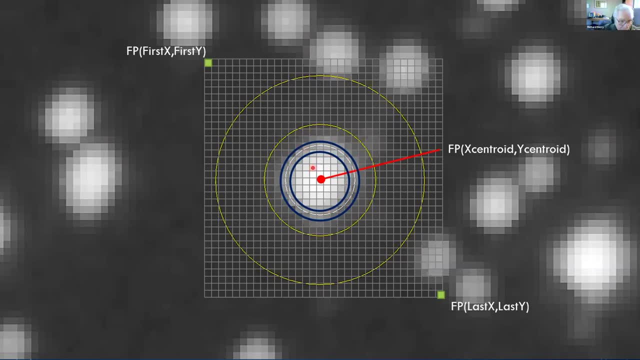 Steven Linthicum A, And we don't want to do that here in the aperture. we want to be able to say: well, if it's inside here, we'll count the whole thing, Steven Linthicum A, As outside here we're going to not counted at all, and if it's here we're going to count part of it. 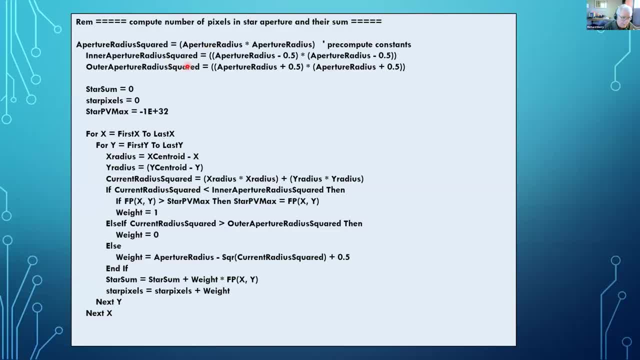 Steven Linthicum A. So here's where that happens. we define some radio I, the inside and aperture radius, and then here's where that happens, Steven Linthicum A. So if it's entirely inside it gets a weight of one. if it's entirely outside it gets a way to zero. if it's in between it gets an interpolated value. and then we're going to add to star some, we're going to add the weight times, that pixel value, and we're going to add a, an amount of a pixel. 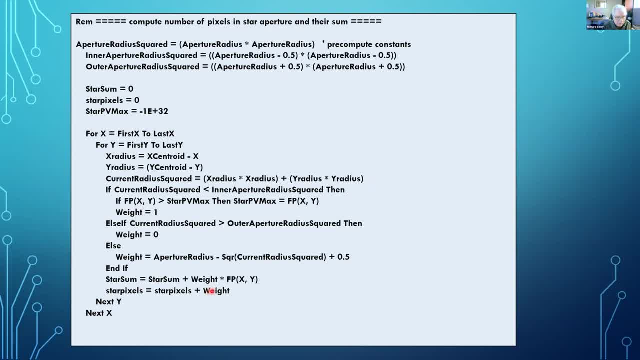 Steven Linthicum A Plus its weight, so you can have a pixel that counts 50%. you can have a Steven Linthicum A pixel that counts Steven Linthicum A 50%, depending on his radial distance from the Center. 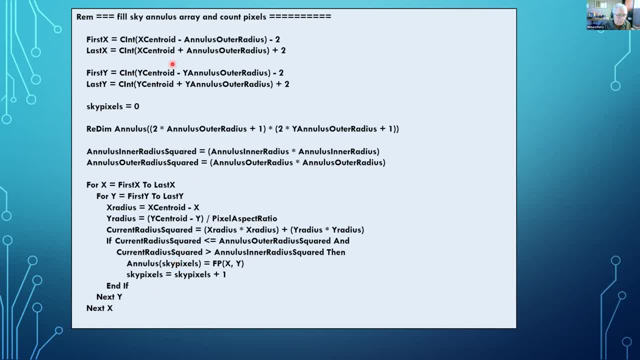 Steven Linthicum A. Okay, and then this similar routine and what we're doing here. we're not going to bother with with Steven Linthicum A, Getting nice tidy edges, because we typically have 200 to 500 star pixels in that outside. we can afford to lose one or two in an insider outside. so we're summing them up. 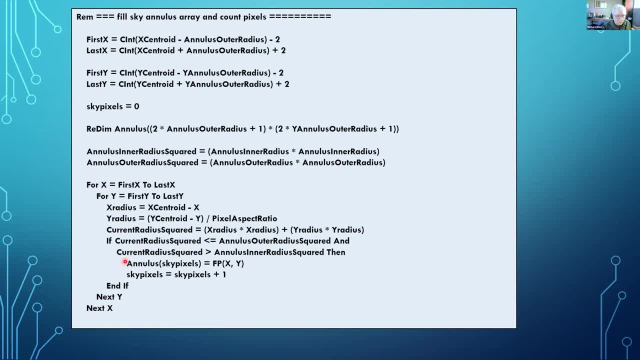 Steven Linthicum A And we're going to put these- not Steven Linthicum A- into a some, but we're going to put them into an array. Okay, so we have an array called annulus Steven Linthicum A And it's indexes sky pixels. we determine it from accounting how many star pixels we're going to have. 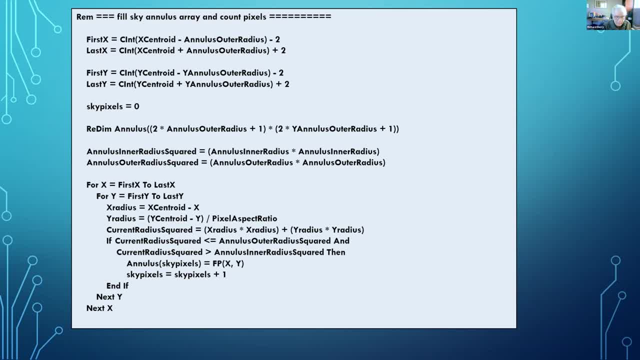 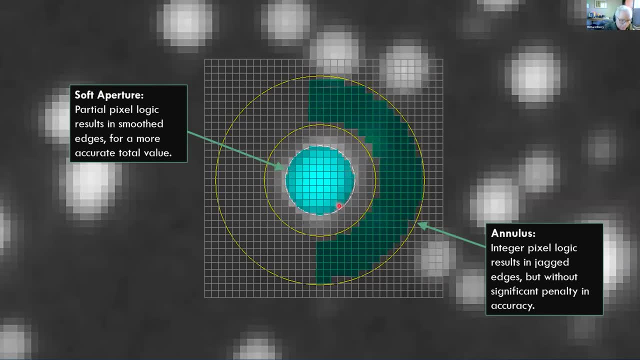 Steven Linthicum A, And we're counting the number that go into that. now here's the graphic that shows what we're talking about. so here, if you have the soft aperture- and we've colored these in by hand, which is really tedious- 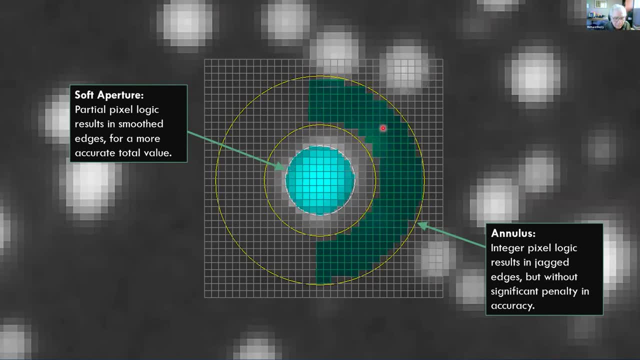 Steven Linthicum A. But you can see, Steven Linthicum A, We have basically it follows quite well- and I hope you can see it- that we have jaggies here, right, jaggy, jaggy, jaggy. okay, Steven Linthicum A, We don't have to work, we could do that, I mean, you know, but it really isn't going to give us a better result, whereas here it's going to make a big difference. now you say, well, that's big enough. you know, few pixels inside. now, 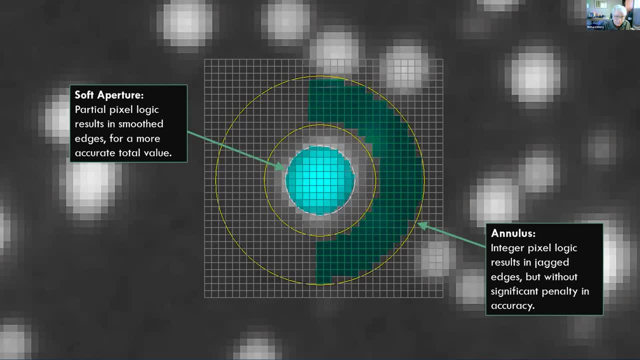 Steven Linthicum A. It actually probably is not necessary with a radius of six, which is the value used in these tests- Steven Linthicum A, or five Steven Linthicum A. Rather it's value Steven Linthicum A. But if you have really small star images, really tight star images, as we did actually when we're early in the days of testing avs or net, 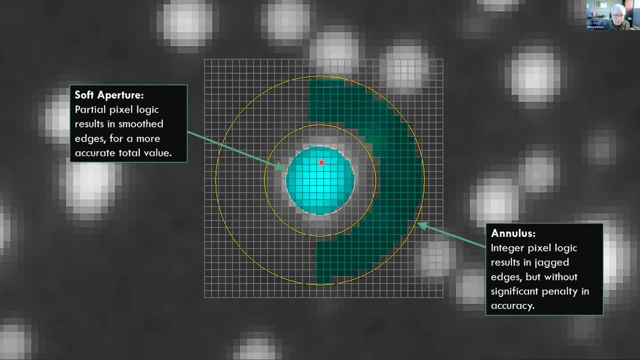 Steven Linthicum A. we're using very sharp little refractors, are using radio of two and three pixels, and it really made a difference as to what was included. now there's one more thing that's going to happen here. Steven Linthicum A, We got background. 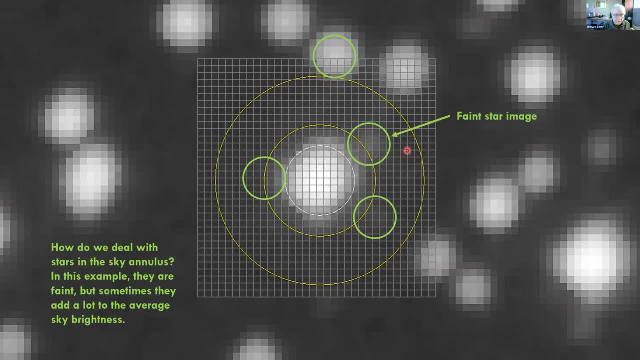 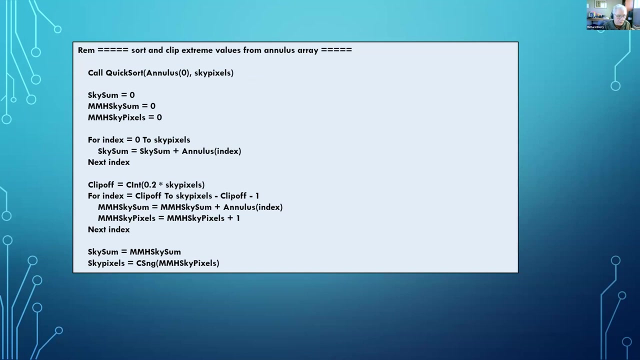 Steven Linthicum A. star images here. this one you can see pretty well if I crank out, and this one is just beginning to impinge here. Steven Linthicum A. How do we deal with these extra stars? Okay, they can. in this case they don't, but sometimes they add a lot of value to the average sky brightness, and what we're going to do is we're going to sort the array of pixels. 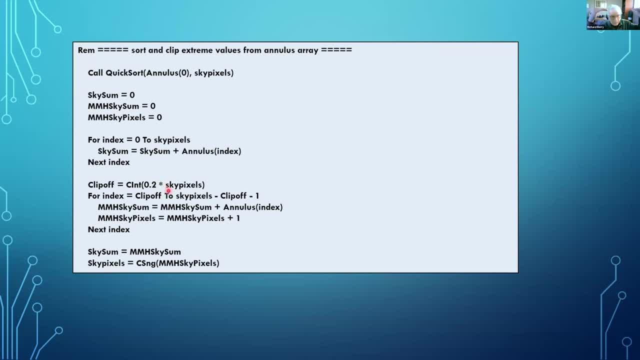 Steven Linthicum A. And then we're going to throw away the Steven Linthicum A. brightest 20% and the dim is 20%. Steven Linthicum A. Okay now, Steven Linthicum A. there's been, over the years, a lot of argument as to how you do this. people take the, the median, they take the mean, they take various statistical measures. 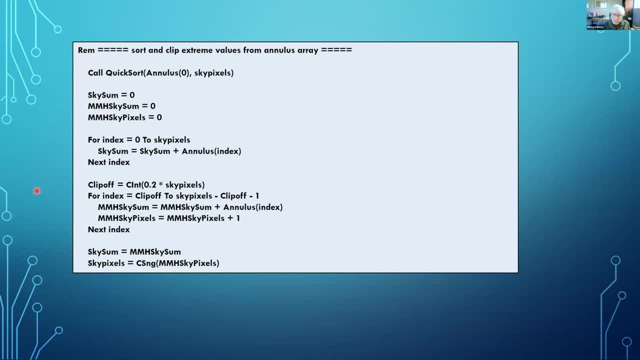 Steven Linthicum A. This one is simply throwing away 20%, the brightest 20%. in order to balance that, we throw off the bottom. Steven Linthicum A. 20%. Steven Linthicum A. You know it's. 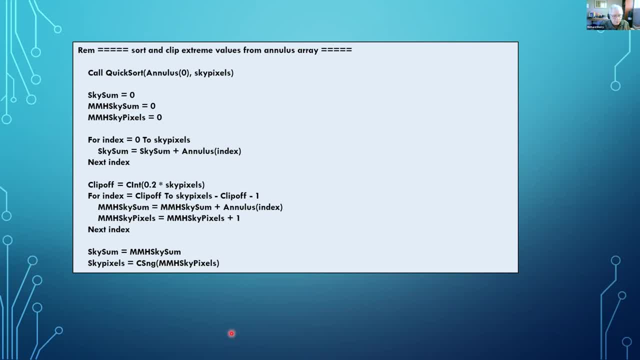 Steven Linthicum A. You can. you can put a lot of effort into trying to improve this, and you probably. Steven Linthicum A. Really, the best answer is: don't work with stars that have significant Steven Linthicum A Other stars near them. Okay, if you can't avoid that, we're taking something that is pretty effective at getting 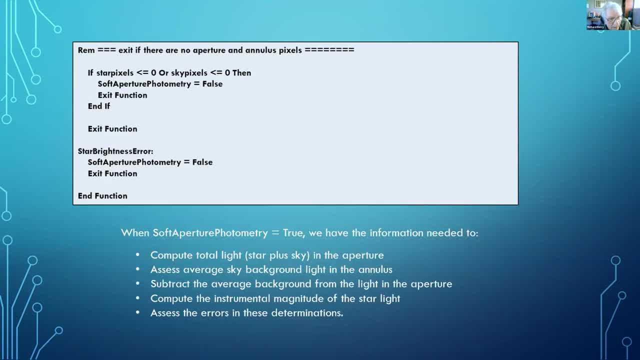 Steven Linthicum A, rid of that extra starlight. Steven Linthicum A And then, as we did before, as we Steven Linthicum A, exit this routine. if there's Steven Linthicum A, If we didn't find any star pixels and if we didn't find any sky pixels, then the soft aperture, photometry and zero and get out of this function and return a value false. it didn't work. 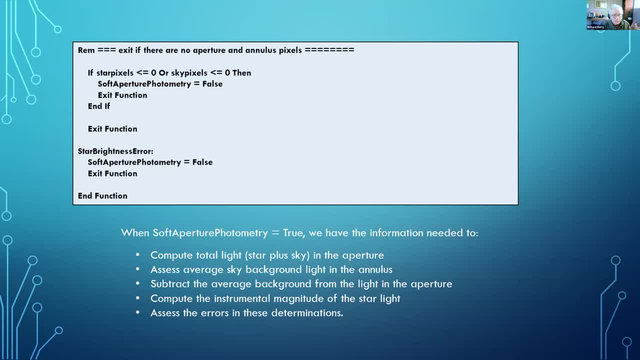 Steven Linthicum A. Okay, having done this, though, when this, when we get up Steven Linthicum A, A very Steven Linthicum A- value of true for this function, we now have all the information we need to. 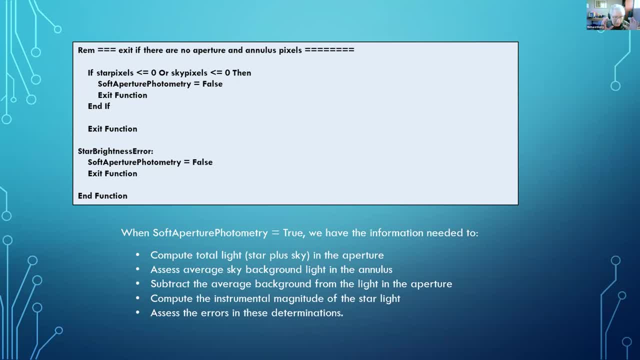 Steven Linthicum A. compute the total light in the star, that is, the star plus the sky. Steven Linthicum A. The average sky background minus impinging stars. subtract the average background from the light and the aperture, okay. compute the instrumental magnitude of the starlight and assess the errors in the determination. 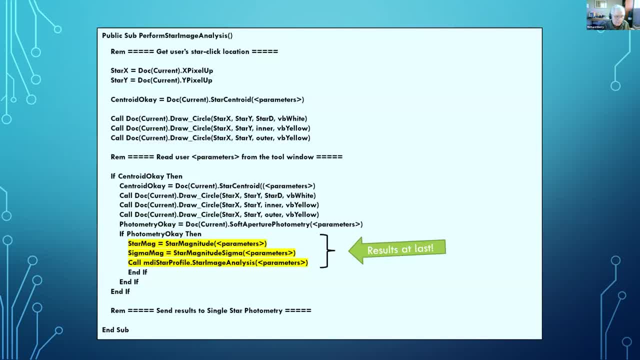 Steven Linthicum A. we've got all these. all these values are come out of here and so now we're going to call a couple okay, if the time entry is okay. so we've gone through this routine. we check. we did a quick check on. 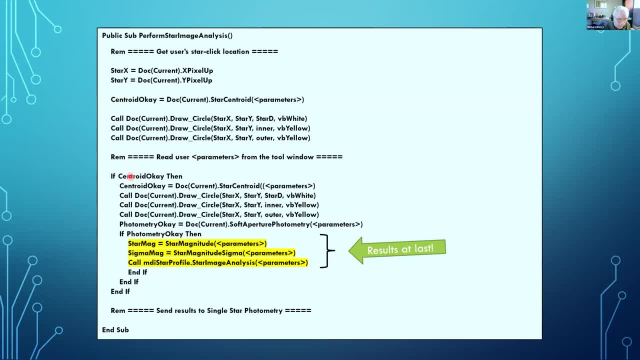 Steven Linthicum A. Can we get a good centroid? yes, can we get another good centroid? yes, can we do photometry and get it okay? and if that's okay, okay, now compute the magnitude. okay, Steven Linthicum A and routines like this. they really hate it when you pass zeros and stuff. 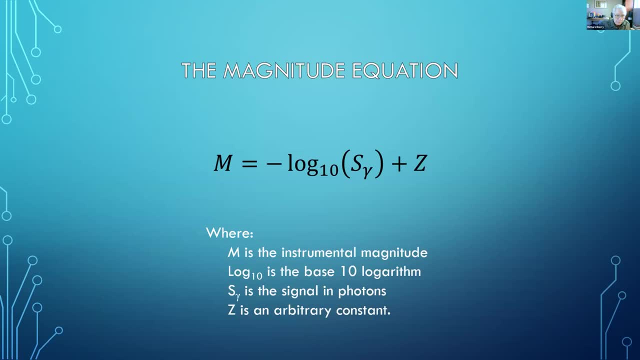 Steven Linthicum A into them, because they crash Steven Linthicum A. So here's the magnitude equation. i'm not going to go into this a whole lot. you, I hope, if you're doing for time it, you understand how magnitude you're computed. okay, here's the magnitude. 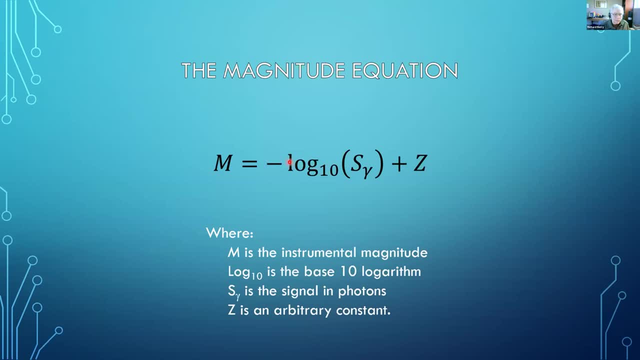 Steven Linthicum A minus log base. there should be minus 2.5. that's a bug in the in the presentation. so it's minus 2.5. log base 10: the signal in photons. Steven Linthicum A Plus an arbitrary constant. 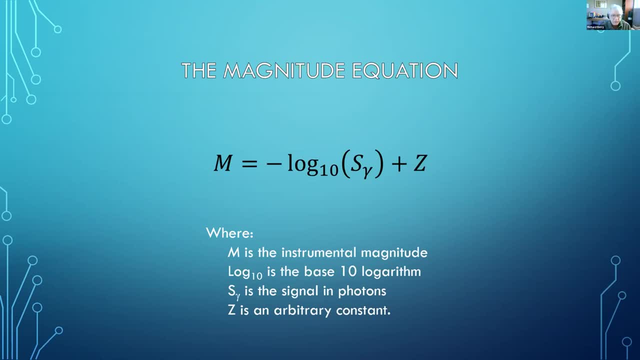 Steven Linthicum A- Z. okay, Steven Linthicum A- Z is the fudge factor, because Steven Linthicum A To it allows us to go from Steven Linthicum A- photons to magnitudes, and Z will typically end up being a value like 22 magnitudes. so, in other words, you just run this, this equation as it looks. 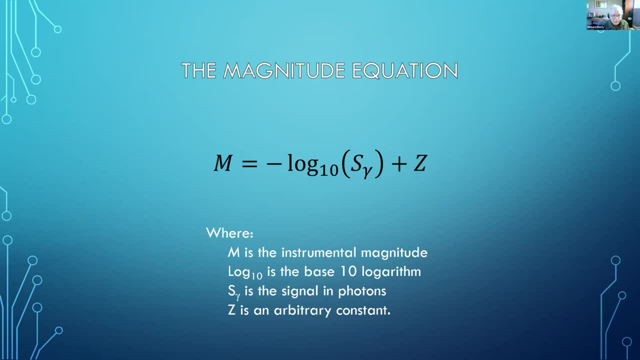 Steven Linthicum A, you'll end up with a minus eight magnitude star, which is Steven Linthicum A, Not you're going to add Steven Linthicum A, A yeah, you're going to add 22 and you're going to come out with a reasonable magnitude like: oh, it's a 13th magnitude star. 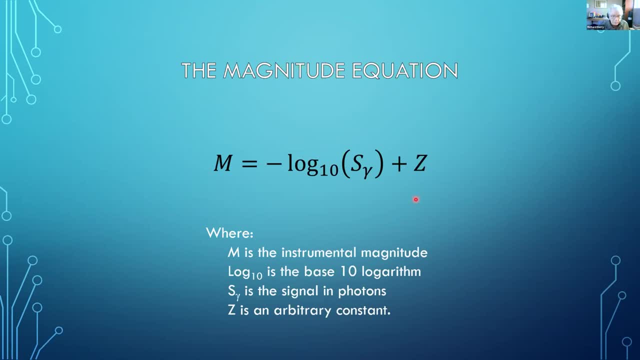 Steven Linthicum A And in the, in the single star photometry, it's important to assess Z carefully. you do that by clicking on a star- Steven Linthicum A- Setting the value of Z to give you the right result. then when you click on other stars, you get the right result. 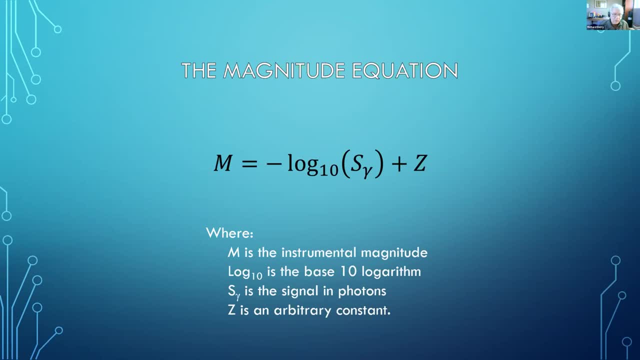 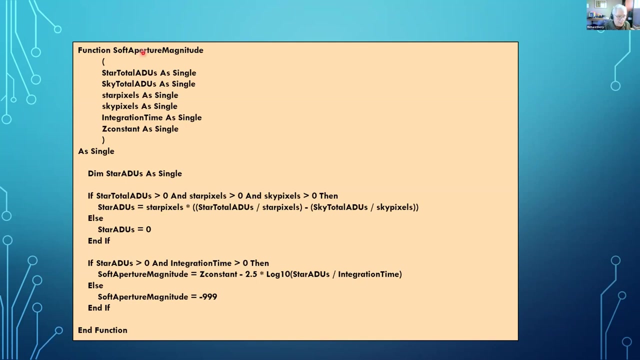 Steven Linthicum A. So Z is your scaling factor, it's your fudge factor and okay, carefully to note, I will change this- it's minus 2.5 log 10. that's just a, the definition of what a magnitude is. okay. so here's the soft aperture magnitude. we're doing the calculation it's basically doing. just see me actually have 2.5 log 10. it's, it's there and we divide. 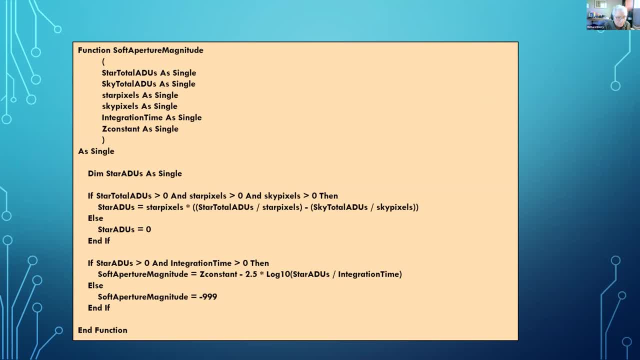 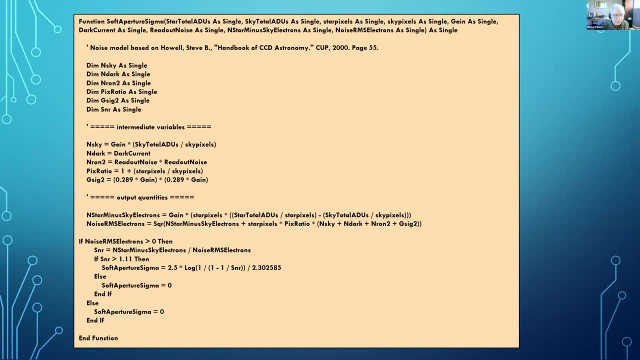 Steven Linthicum A. We normalize this by the Steven Linthicum A- Integrity, Steven Linthicum A, Time, Steven Linthicum A and Steven Linthicum A. Then we're also going to compute the Steven Linthicum A Noise. this I won't get into the equations for doing this there in the handbook of astronomical image processing. 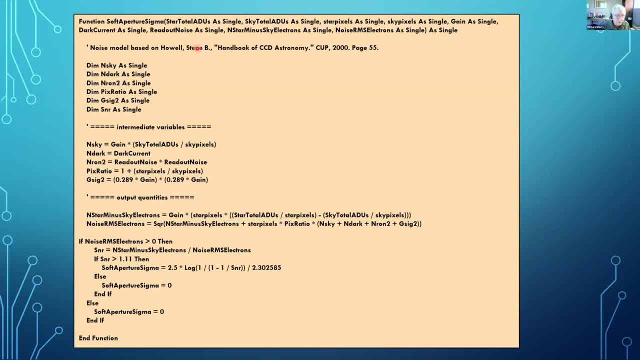 Steven Linthicum A, you'll find a professional reference. and Steve howells book, the handbook of ccds- astronomy, Cambridge university press. Steven Linthicum A, Every Steven Linthicum A, Everybody is using this. it's called the, the ccd equation. 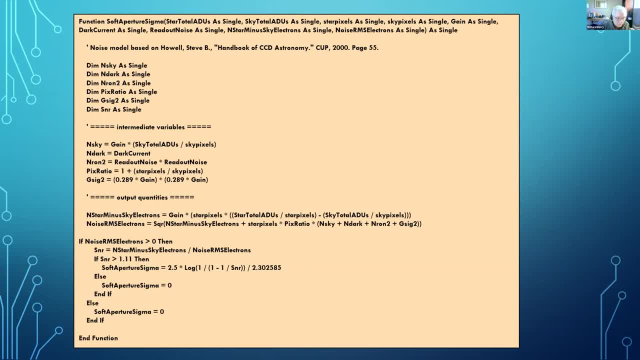 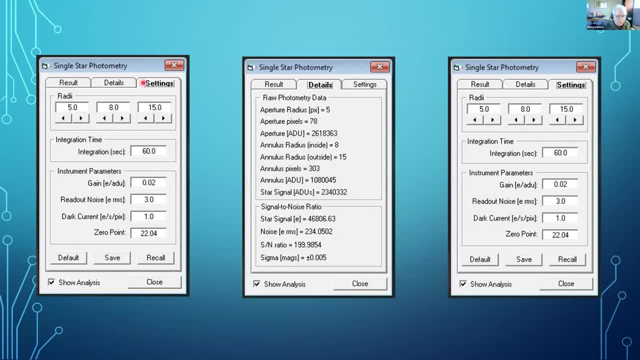 Steven Linthicum A. Okay, so we calculate these values: Steven Linthicum A. So, on the single star photometry tool then okay, here's, here's where, Steven Linthicum A, The settings. here's your radio five 815, which i've been using my integration time. 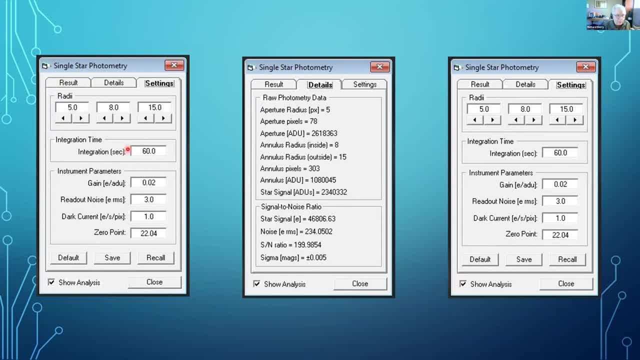 Steven Linthicum A, which is important. Steven Linthicum A, The single star photometry tool, Steven Linthicum A is a relatively dumb tool, so you have to manually set the integration time. you also are setting the gain, which is the 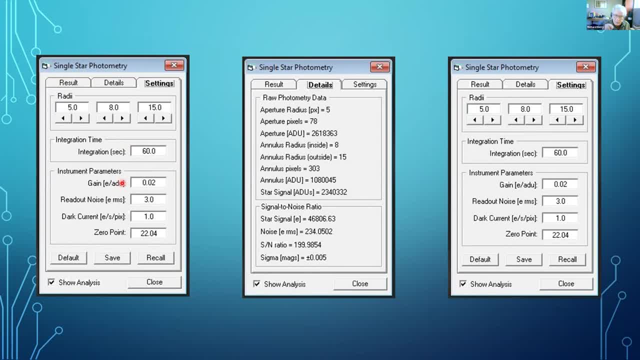 Steven Linthicum, A number of electrons per at you, remember, at us, to the pixel values, the readout, noise, because these are all making your the dark current and finally zero point. So these are key values you're going to set, Steven Linthicum, A um. 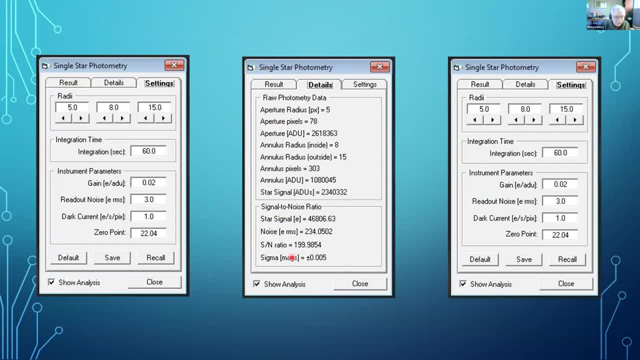 Steven Linthicum A, Then Steven Linthicum A. The result: Steven Linthicum A, The. what you get out of this thing is it gives you all the values that it computed. Okay, so this is your complete readout of the analysis, and then this is the: the. 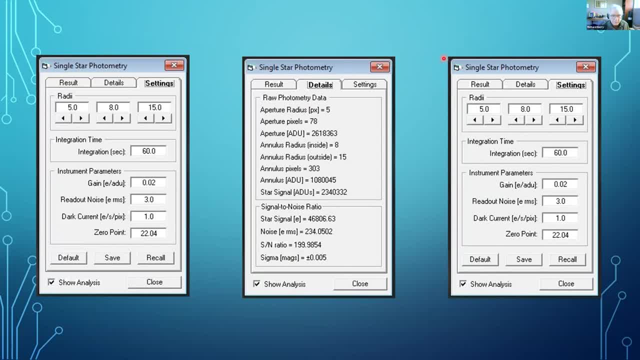 Steven Linthicum A. oops, another bug in the in the presentation, the front and the back of the Steven Linthicum A Of the. this is my settings. I should have had a result. Steven Linthicum A panel there. we'll fix that up and we'll probably do something like. 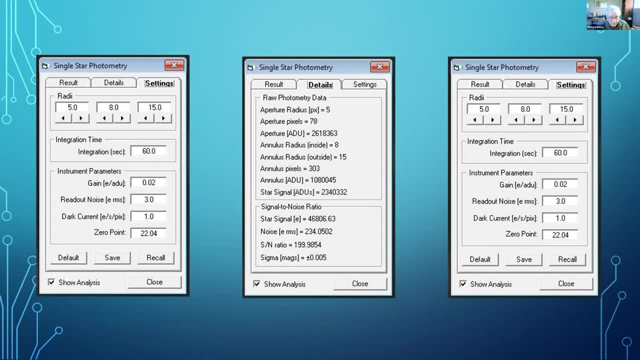 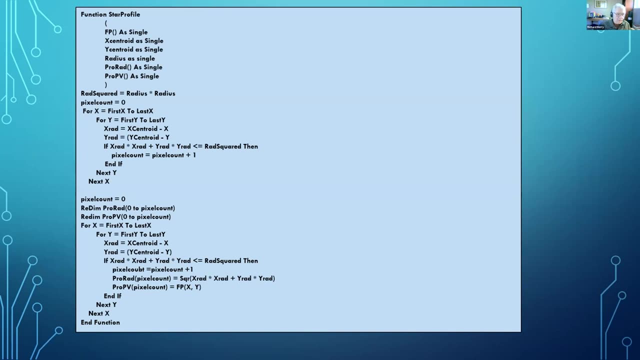 Steven Linthicum A. Oh, at some point, Steven Linthicum A, post them a PDF file of the of the talk, with the bugs corrected. Steven Linthicum A. there's always bugs, anything you do, okay, Steven Linthicum A. Now we've talked about the star profile a number of times. i'm. this is the software, the code that produces the arrays. 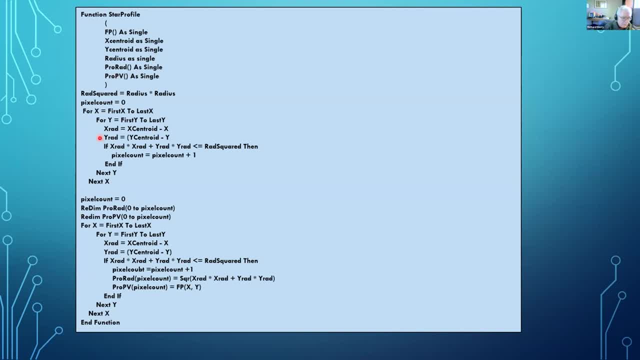 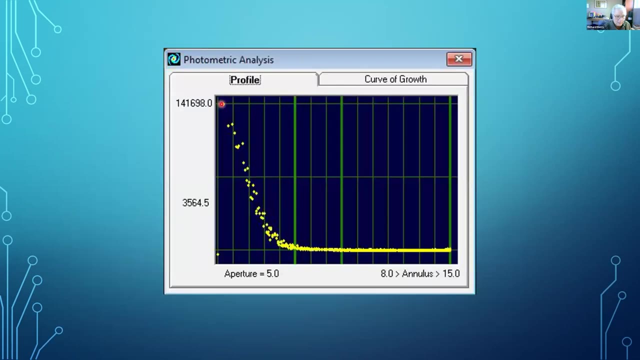 Steven Linthicum A That we're going to plot in the star profile. so we simply find the radial Steven Linthicum A, Distance outward Steven Linthicum A And we produce to raise. one is a radius array and the other is the value pixel value array and we're going to plot those like this and you've seen this a bunch of times already. 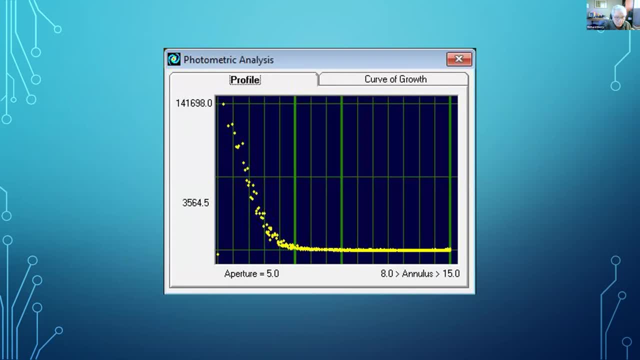 Steven Linthicum A. Now there's one other thing that comes out, a very useful tool, Steven Linthicum A, And this is the curve of growth. Okay, those of you who've been looking at this thing several times, Steven Linthicum A. There were. 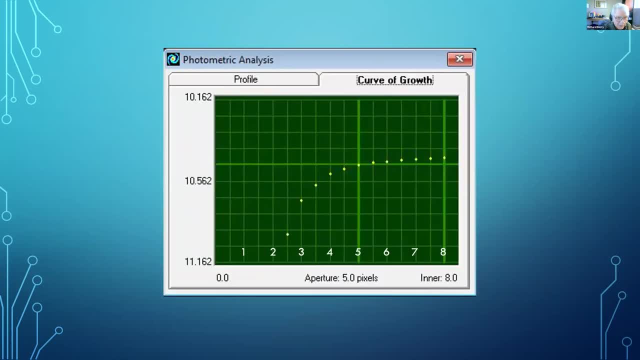 Steven Linthicum. A Wait, a minute. he's hiding something from us. now i'm going to tell you about that. the curve of growth is the Steven Linthicum, A curve that says, well, i'm going to, if I set the aperture to a different value, say, I set the aperture to for what magnitude? what i've got? well, here's the magnitudes you would have gotten, and here they are okay. well, if you have the 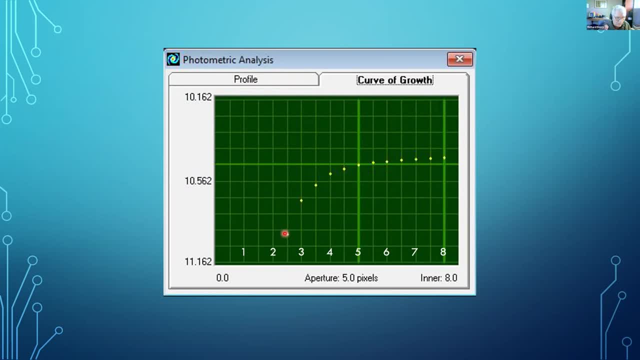 Steven Linthicum, A aperture set for two and a half. you can see you would have left out most of the light. you would have left out Steven Linthicum, A Four tenths of a magnitude to dim. if you'd set it for radius of three, you would have had about two tenths of a magnitude faint. set it for magnitude of three and a half, it would have been. 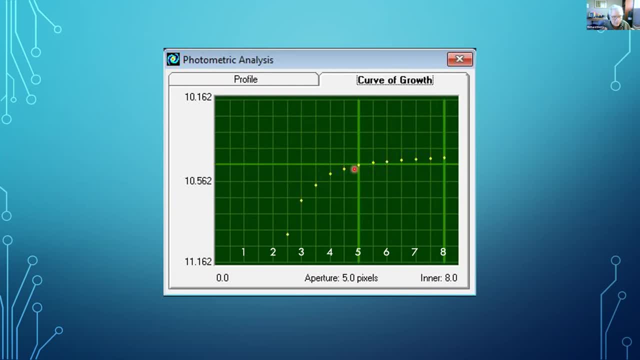 Steven Linthicum A. A tenth of a magnitude too bright and so forth. so here's value of five: Steven Linthicum A. Okay, and then you'll notice, if you keep making the aperture bigger, you're going to get more light. Okay, until you, and it just keeps on going up and it. 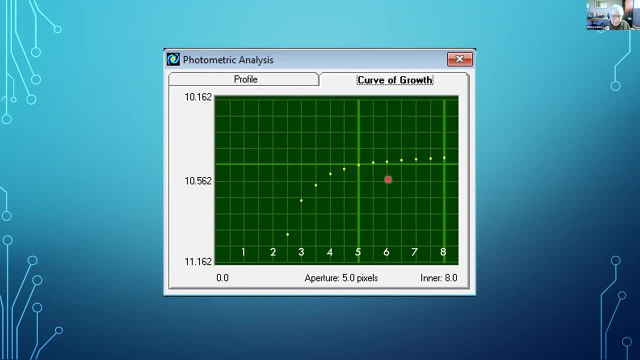 Steven Linthicum A typically does, Steven Linthicum A, But at some point number every star has the same profile. Okay, which means that every star- you do this to the curve of growth- should look the same for every star. it'll be noisy, they'll go up and down. 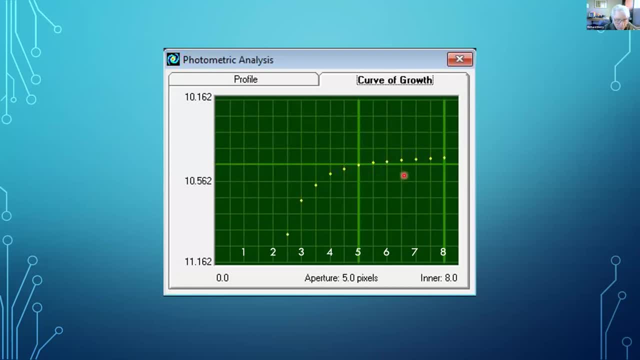 Steven Linthicum A. Now, one of the things you can't see in this graph because they're too small, is that there's a little red error bar, Steven Linthicum A. Now the error bar Steven Linthicum A is: 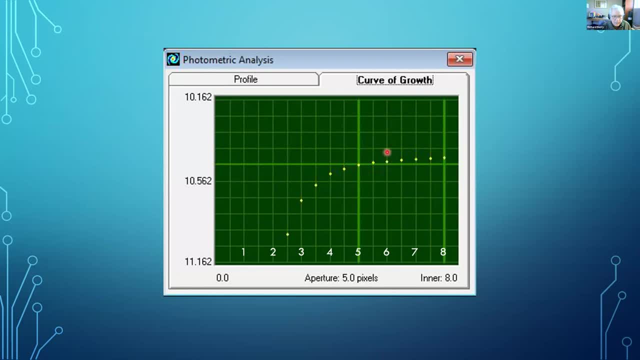 Steven Linthicum A are small at the smaller values, but as this gets bigger, you're now picking up more sky pixels, but you're not picking up much starlight. you can see the stars not getting brighter, but the error bar start to grow. 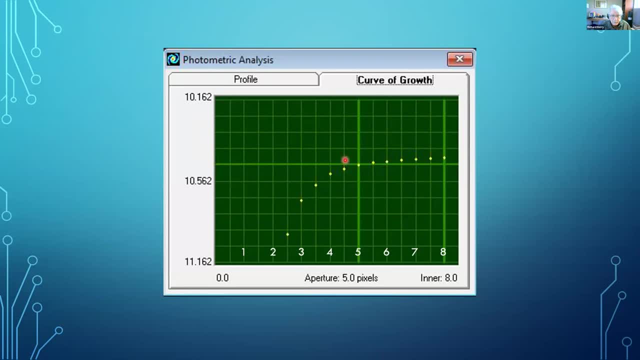 Steven Linthicum A, And what you do is you make a judgment call, really, that five is the value just before it's going asymptotic. Okay, you know this will keep going up forever, potentially, so you're going to pick this value now. Steven Linthicum A. So there's in some of the other photometry tools in ap for when. 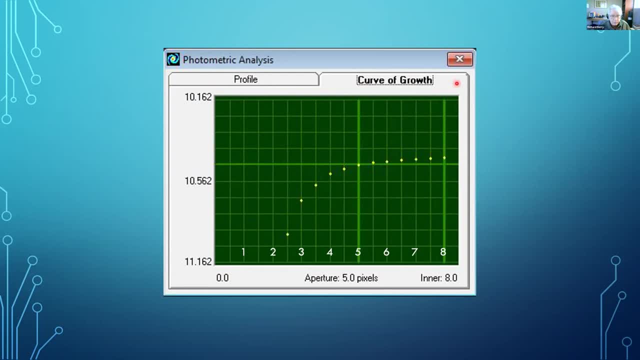 Steven Linthicum A. We also have a signal noise ratio plot and I don't have that, the simple in this in the single star photometry tool. but what you typically see is that signal noise ratio rises Steven Linthicum A And then falls. So if you doing more sophisticated, 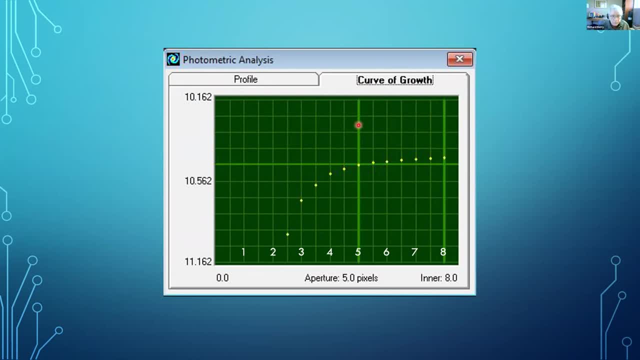 Steven Linthicum, A photometry. you might tune for the Steven Linthicum, A highest signal noise ratio. now, what's scary about that? is the highest signal ratio, as you typically appears at 70 or 80% of the value. where you, it tends to go asymptotic. 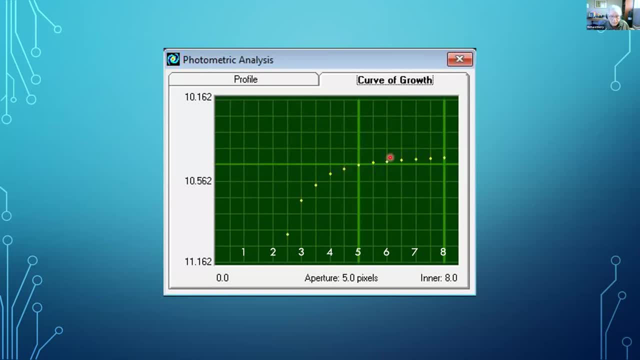 Steven Linthicum A Most people, including me. I go for a slightly lower signal noise ratio. Steven Linthicum A. In order to be assured, Steven Linthicum A, That Steven Linthicum A, i'm going to always get this all of the starlight. 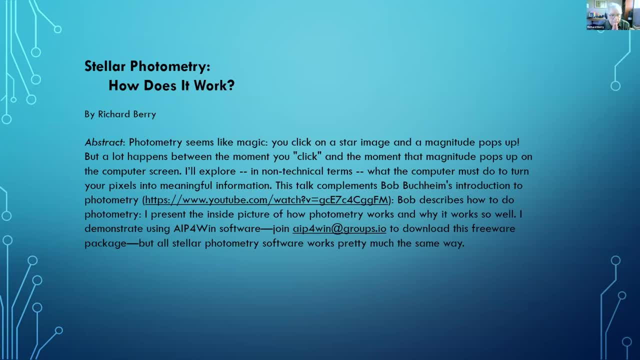 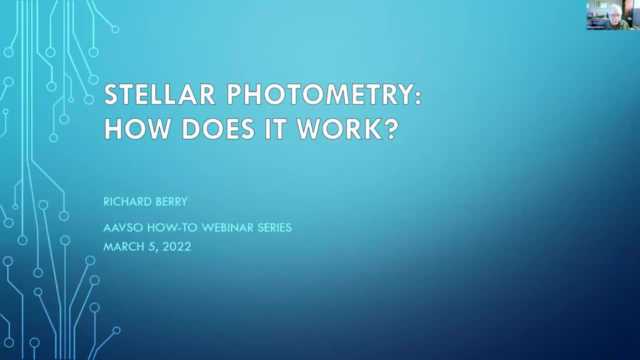 Steven Linthicum A. So that's the Steven Linthicum A, Basically what I have to say. this is the Steven Linthicum A abstract written for it and Steven Linthicum A. we've reached the end of the formal presentation. I hope I haven't run too far over time and I think we're open for questions now. 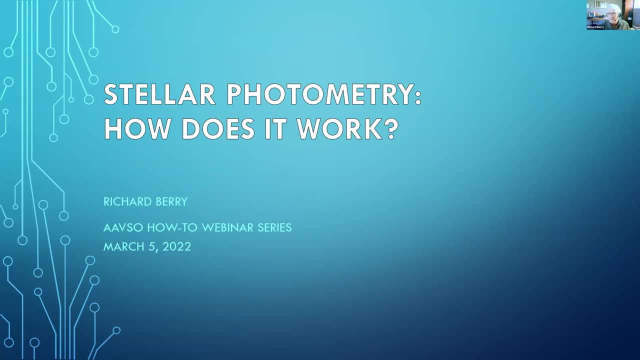 Steven Linthicum A. So there's. there's, lauren. Okay, thank you so much, Mr Barry. that was a fantastic talk. I really am kind of in awe at the amount of hard to find out information that was just shared. Steven Linthicum A. Before we move on to the questions that we have quite a few here, I want to go ahead and 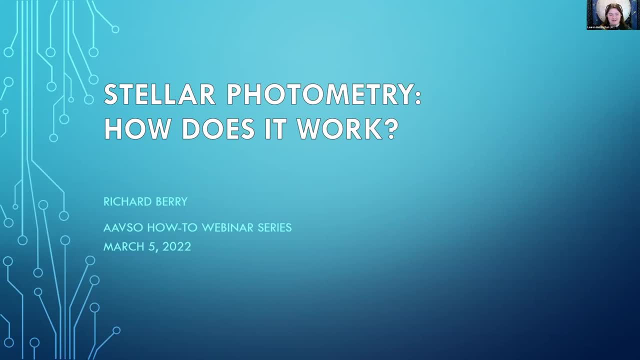 Steven Linthicum A. Make a small announcement, because I did receive a question from, or a comment from someone in the audience who's Steven Linthicum A brand new Steven Linthicum A Photometry and said this is all very intimidating. so I want to make a point that what you just showed is a behind the scenes of software aimed at programmers. 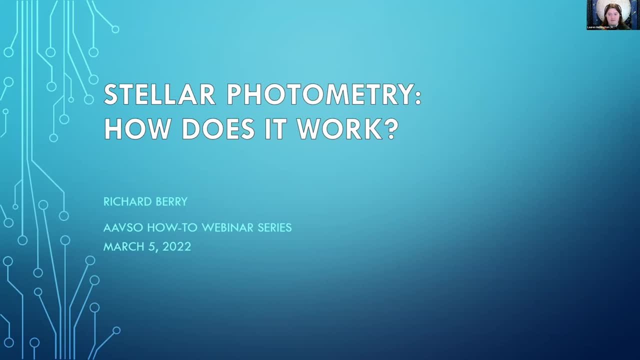 Steven Linthicum A, But it's not how you actually do the photometry. when you're just have an image and you're like: i'm going to go, Steven Linthicum A, find out what magnitude the star is, that procedure is a lot simpler, so don't worry if you're a beginner in the audience. 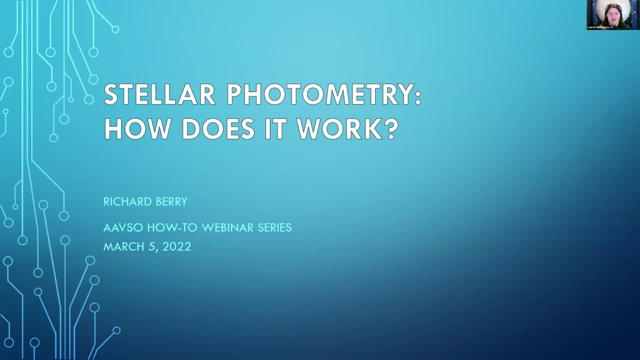 Steven Linthicum A. i'd recommend that you go back and look at our past webinars, like we had one by Bob buckheim on Steven Linthicum A- Getting Steven Linthicum A started with ccd photometry. that showed how you would walk around in a software like Mr berries and. 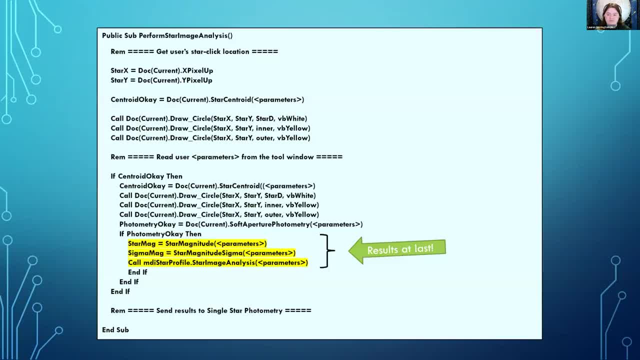 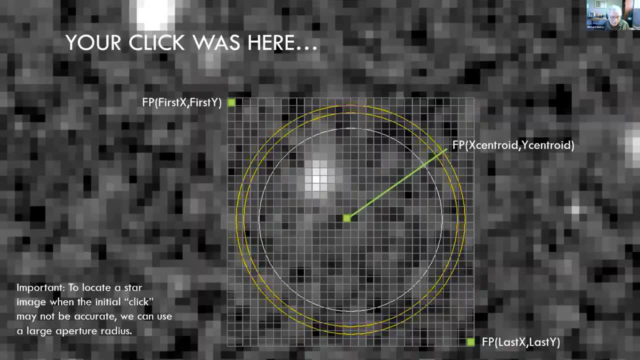 Steven Linthicum A very simply perform the operation of getting your magnitudes For that person. let me go back to the very very beginning, which is When I introduced. it takes a while to get back there. click, click, click, click, click, click, click. 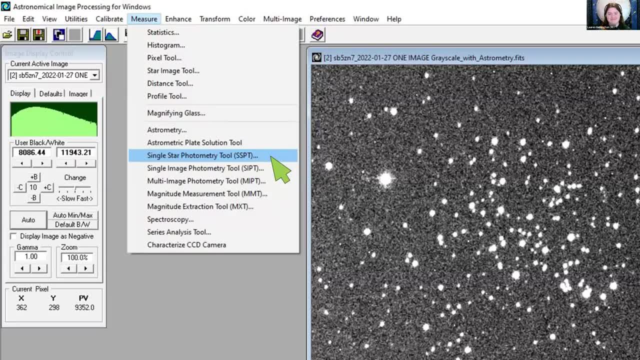 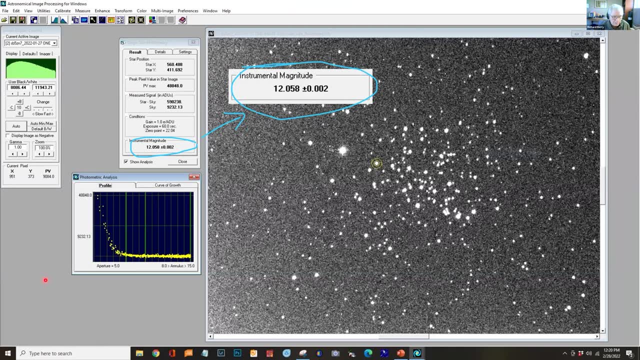 Okay, remember I said: okay, pick the tool. You have the tool comes up, Steven Linthicum A. And then here's the tool up, i've got the, the ratio, and you take your mouse, you over and you click on the star and a number pops up. that's the outside view of what you do when you do photometry. 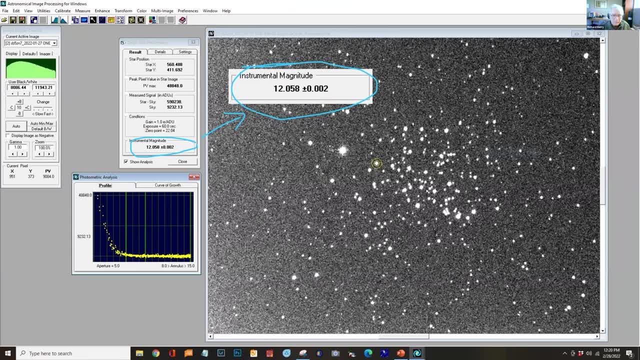 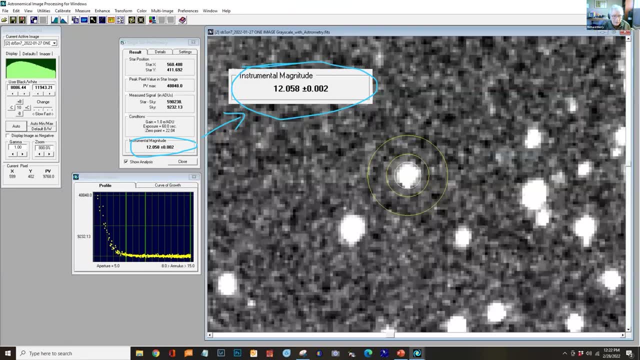 Steven Linthicum A. Okay, right, it's, it's like it's. I mean, it's really fun. Steven Linthicum A. Okay, when I was doing this thing with them. 67.. Steven Linthicum A. I could go click, click, click click. 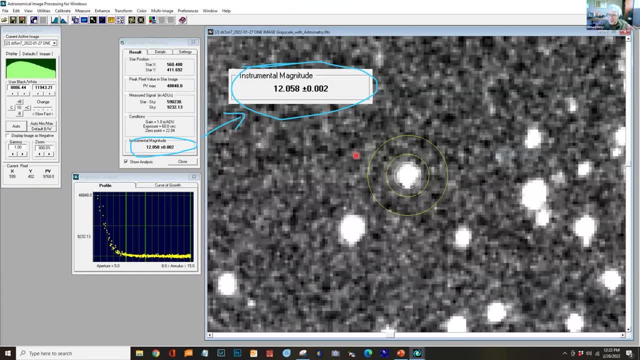 Steven Linthicum A, I get a magnitude for each star. that's. that's the video game part of astronomy, and you don't have to know how this stuff works. however, Steven Linthicum, A Part of what I hope you learn was that if you go and you click on this star, you're in trouble because it's sitting right next to that star. 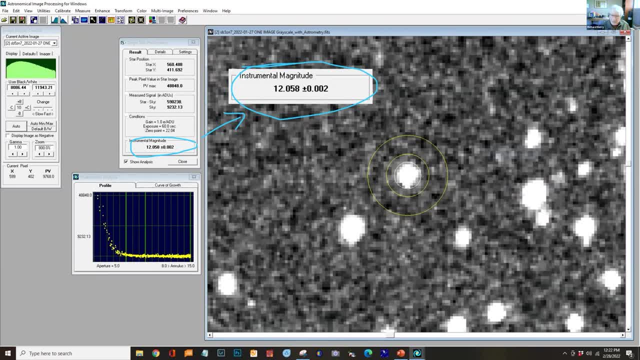 Steven Linthicum A. So it really does it really not normally that complicated, Right, Steven Linthicum A? Right, this is the easy part, this is the fun part. All right, thank you. So now, moving on to some of the questions, let's see, let's, let's take some of the 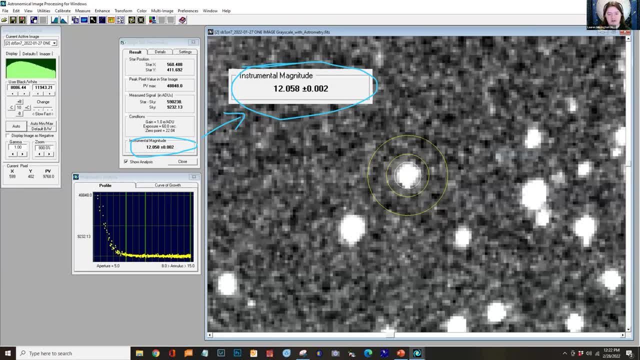 Non programming ones first. so this one comes from Joe for Gola, who asks if, using an ev scope, how do you access the dark frame data in order to do your calibration? and also, I don't think that Steven Linthicum A Maybe scopes can. 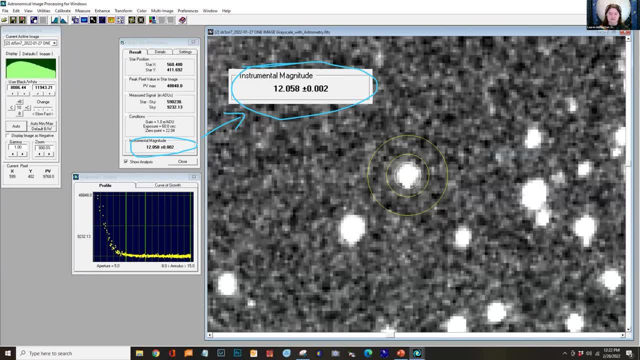 Steven Linthicum A capture flats, just dark frames. do you know anything about that, Steven Linthicum A? They cannot capture flats and it's very frustrating to me. however, the optics are very, very simple. you have a paraboloid focusing on a. 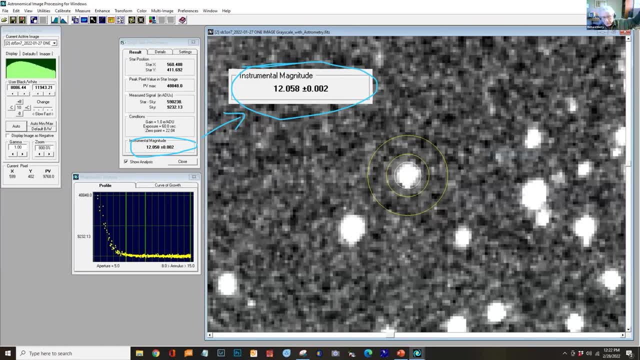 Steven Linthicum A. On the sensor and there's really nothing else in there. there's no diaphragms or anything that might cause vignetting. so, Steven Linthicum A. yeah, flats are an issue. Steven Linthicum A. Okay, 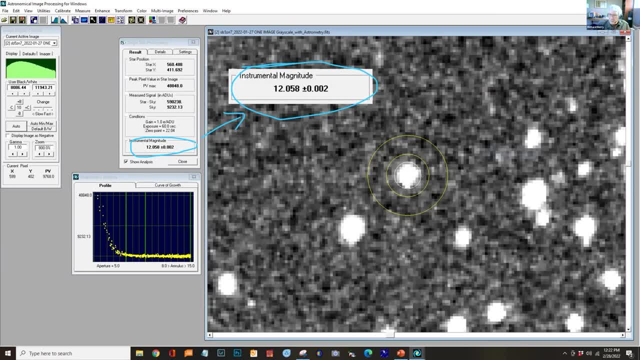 Steven Linthicum A To Steven Linthicum A. With the ev scope, what you do is you write to Steven Linthicum A. You need stellar support, Steven Linthicum A. Okay, first of all, you'll notice that you can upload your images. okay, so first thing you do is you go upload your images. 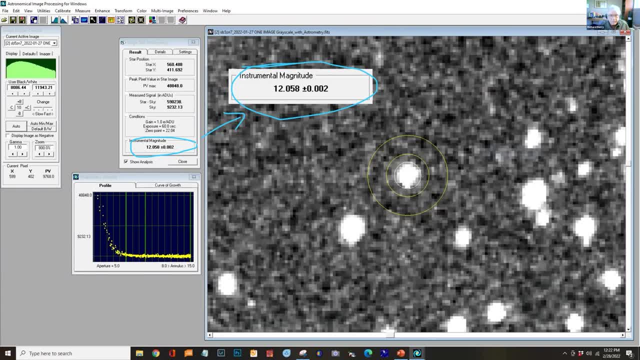 Steven Linthicum A And it's an automatic function ev scope software. then you write to the support people and say I just uploaded a bunch of images from ev scope, blah, blah, blah, blah which has a Steven Linthicum A, It's it's serial number and please send me a link to my images. 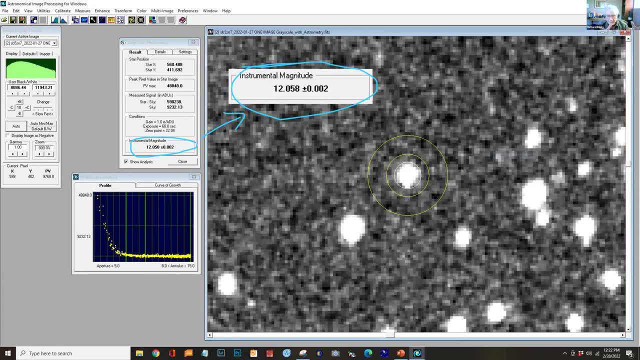 Steven Linthicum A. Two days later, you get back a link which is like 200 characters long- it's got some- and you download Steven Linthicum A Five gigabytes of data, which will consist of typically two or 3000 fits images. 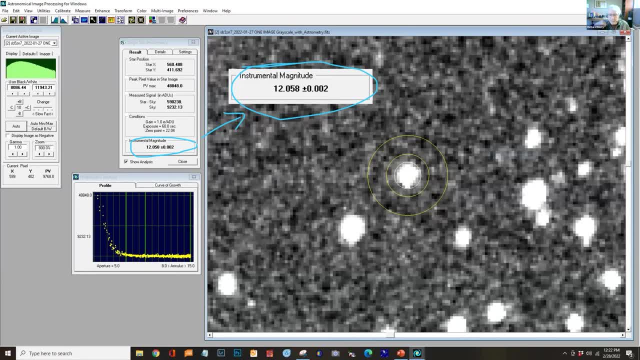 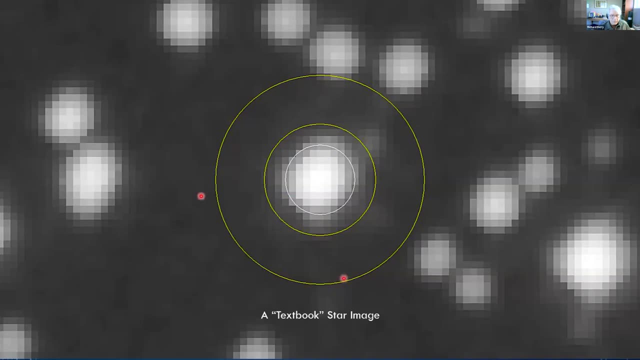 Steven Linthicum A. And it's very nicely organized, Steven Linthicum A, You have the individual images and for each time you did a live stack, they stack all those images together for you. so that's what I was using when I showed the 902nd exposures. that was Okay. this is. this is one of their- their 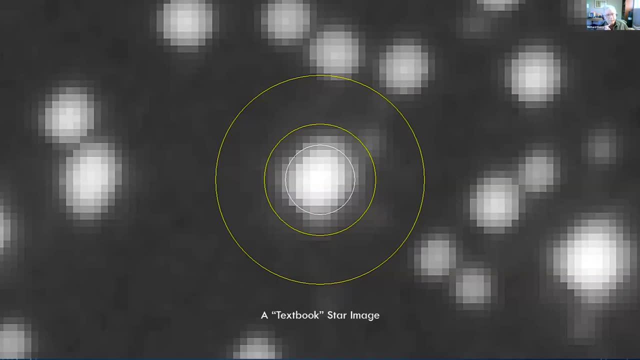 Steven Linthicum A 900. well, what was it? Steven Linthicum A 250. some images average together to get that Steven Linthicum A. I am told that they expect to make it so that you can automatically log on, give a password and download your data, which will be much nicer than having to write to support, but I have to give support. 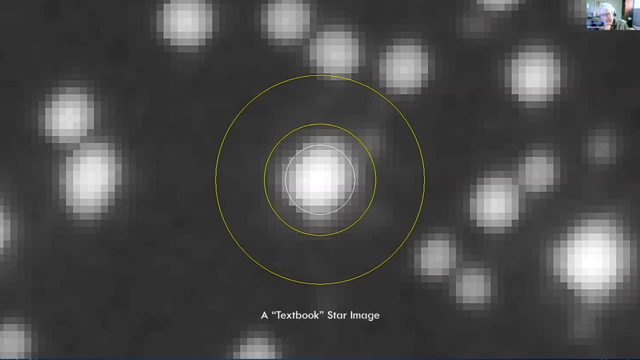 Steven Linthicum A. Great credit at this point. they know me, Steven Linthicum A, To go like: okay, here's, here's your link. Steven Linthicum A, The biggest problem is you always you take you good data. 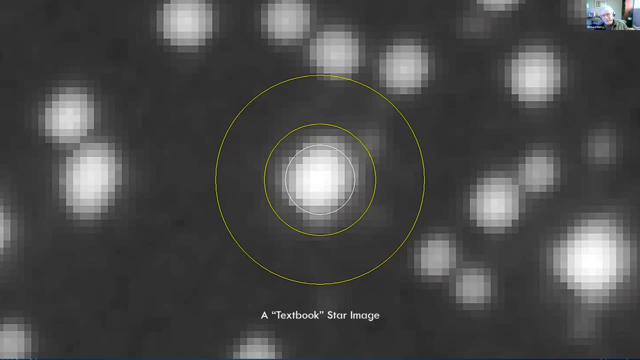 Steven Linthicum A Thursday night. by the time the link gets to them it's Friday evening and they take the weekend off, so they don't get to send you a link until Monday. that's why I say it takes two days to get your data back. typically. 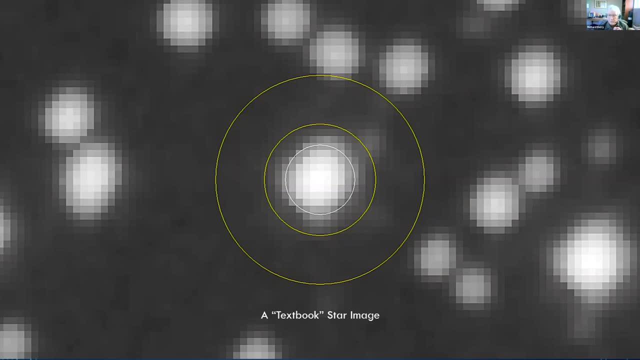 Steven Linthicum A, But I would like to see I think they will automate that at some point and you'll be able to get your data back. That would be great. Okay, The next question here comes from guys string fellow Who says hello and thank you very much for the presentation. can you please explain exactly what encompasses stacking images compared to, for example, media and combining a set of images? 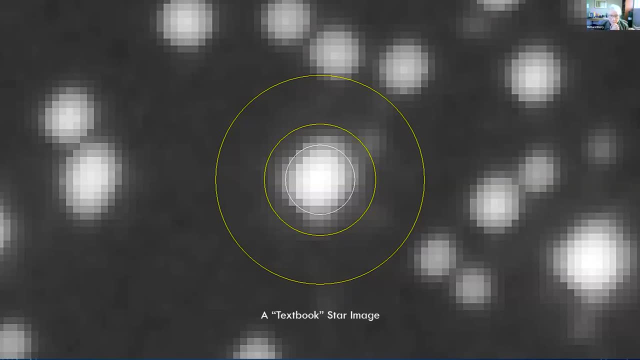 Steven Linthicum A, And this, I think what Steven Linthicum A Well stacking is simply adding them together or taking an average, and either way works. you can add them or you can take an average. if Steven Linthicum A, If you are working with integer software, you add them. 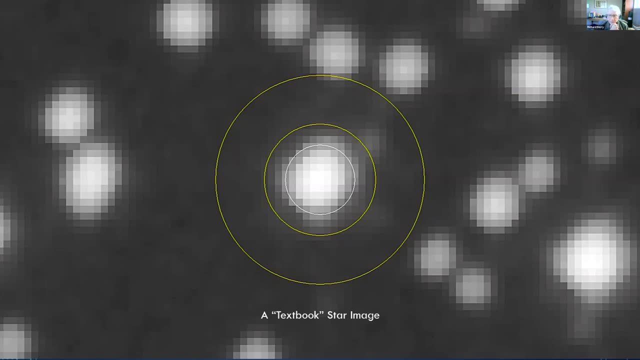 Steven Linthicum A. If you're working with software that uses floating point data, Steven Linthicum A. You would average them Steven Linthicum A, So that you'd have partial pics, or you know you wouldn't have Steven Linthicum A, You wouldn't have integer values, you'd have floating point values. 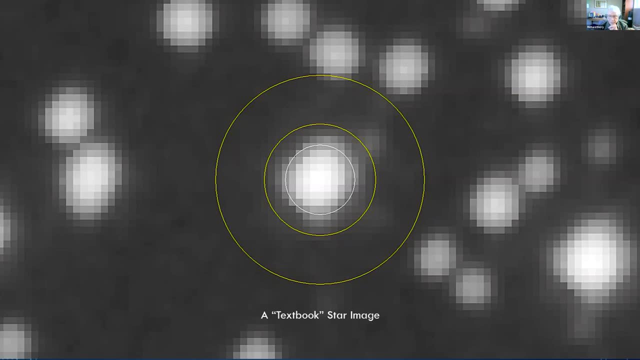 Steven Linthicum A. A IP for windows averages. although you Steven Linthicum A, there's actually an option, Steven Linthicum A, To add them. Steven Linthicum A, You can use the the other routines that he mentioned. 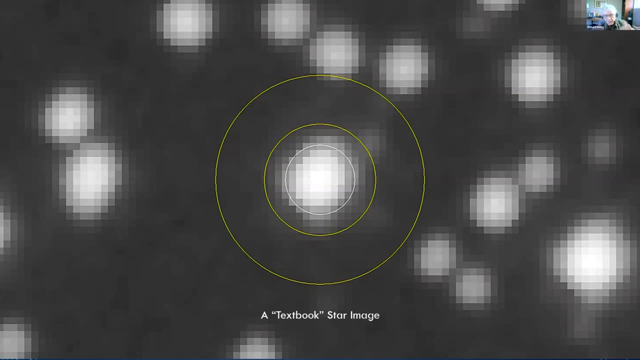 Steven Linthicum A. Compare the pixel in each successive image with the images. all say you have 100 images. okay, for any given pixel you've got 100 different values. in theory, they should be the same, Steven Linthicum A. Okay, but the satellite and airplane went through, so two of those values are just wildly big. Okay, if you use a media, you simply exclude those extreme values. if you use K Sigma, what you do is you compute the median value and then you throw away the ends which are contaminated by passing airplanes and satellites and and. 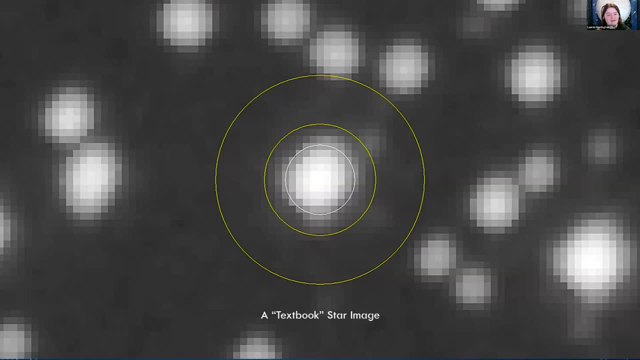 Steven Linthicum A star links Right, okay, thank you, and Steven Linthicum A. Next question. Steven Linthicum A. Here, while we're on the topic of stacking, Jeff meyers asked if there's any reason to measure 10 one minute frames separately versus averaging them together and then analyzing the final SEC. 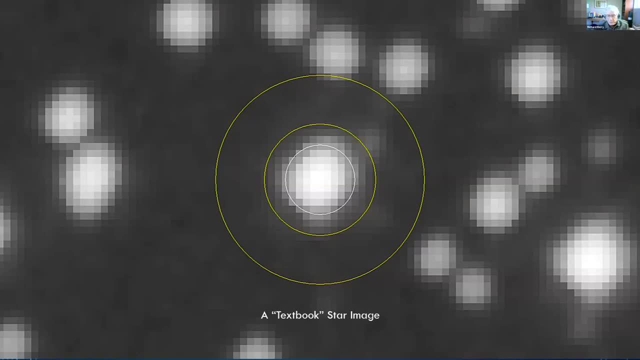 Steven Linthicum A. My preference is actually to have to to measure the 10 of them and and Steven Linthicum A Average, and not only average but also compute the standard deviation, Steven Linthicum A Of the result. 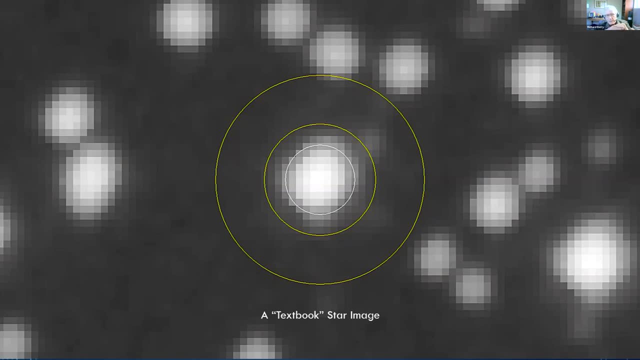 Steven Linthicum A, Because the state: Okay, when you just stack the images together and get a magnitude, you don't know how good that magnitude is. but if you measure the individual ones and you compute the standard deviation, Steven Linthicum A, Then you can say: ah, the magnitude I get is, for you know, 11.25 plus or minus point 003.. 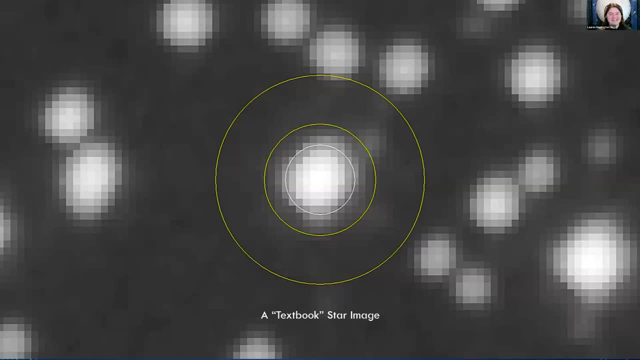 Steven Linthicum A. Well, that would be awfully good. Steven Linthicum A A, point 03. realistically about 3% error. Steven Linthicum A And, and you know, with ordinary photometry you typically looking at a 2%. 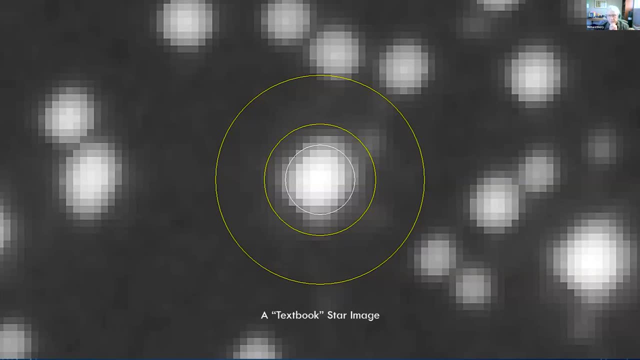 Steven Linthicum A error. Steven Linthicum A, Actually not error. uncertainty in the magnitude. Steven Linthicum A, You know, and I believe avia. so basically would like you not to stack the images. Steven Linthicum A um. 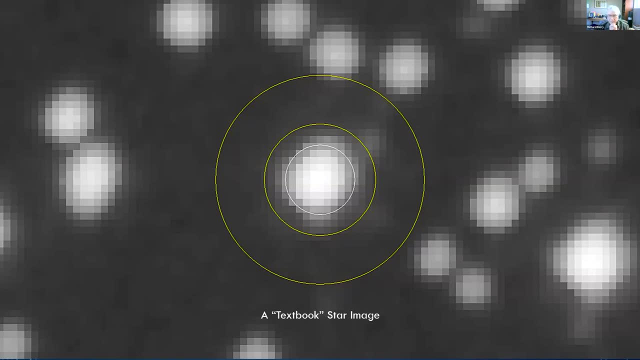 Steven Linthicum A. But when you get down to really really faint stars- Steven Linthicum A, you're starting to deal with, can you get a good centroid and stuff like that? so stack them will give you a better centroid. 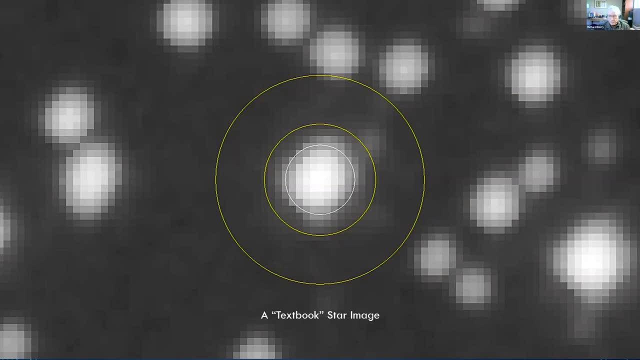 Steven Linthicum A, But it makes it harder to assess whether or not you know that the photometry is good. you simply have a magnitude with no real sense of how good that value. Steven Linthicum A is right and it's an exercise for yourself. do it both ways. 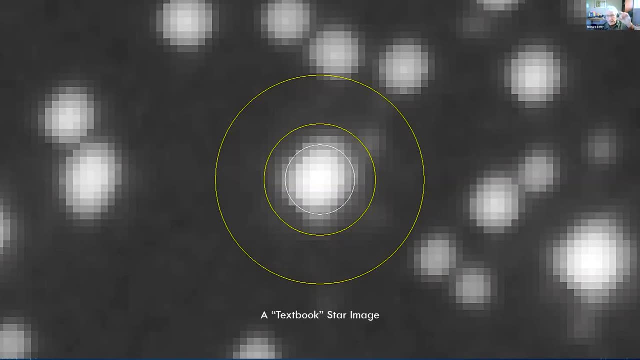 Steven Linthicum A And then compare, compare, Okay, the, the average, the average magnitude by averaging the 10 and the magnitude of the stack should be the same, Steven Linthicum A, And of course they won't be. they'll be slightly different. 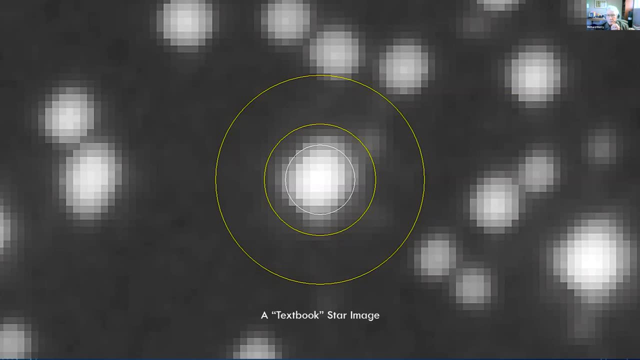 Steven Linthicum A. That doesn't look like a good experiment. Steven Linthicum A, i'll always be willing to do experiments. people, for instance, will ask things like: well, you know, the images of my Steven Linthicum A telescope are a little bit soft on one side and a tiny bit of coma because it's a new Tony and 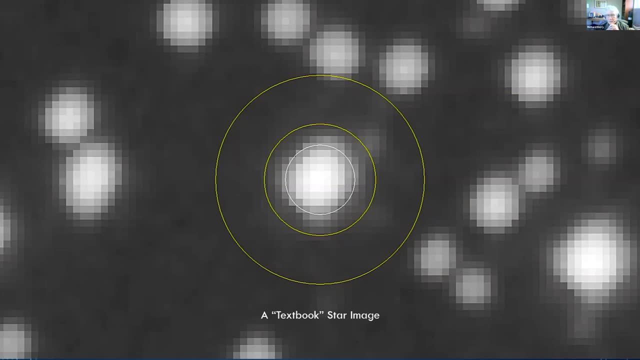 Steven Linthicum A. How does that Steven Linthicum A affect my photometry? Steven Linthicum A And my answer is: Steven Linthicum A. don't Steven Linthicum A. don't go out the cloudy nights and ask someone for for an expert opinion. 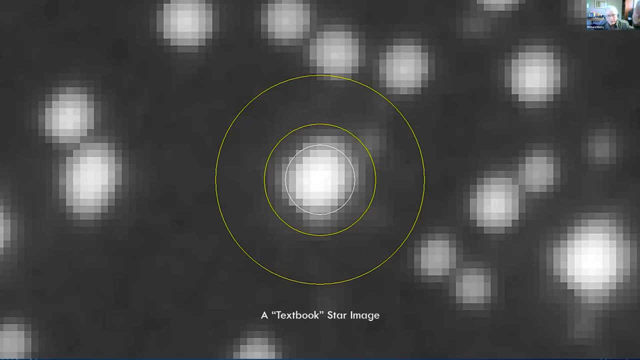 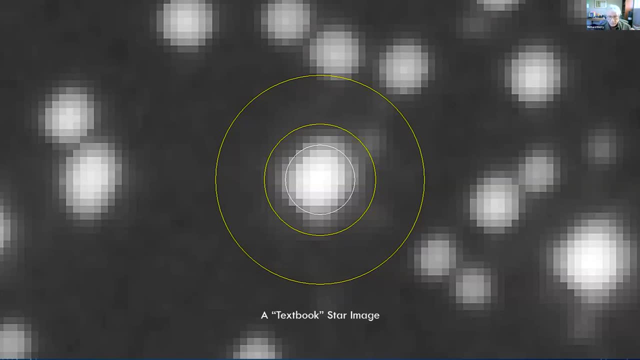 Steven Linthicum A. If there's no problems with the netting and stuff, you should get the same result wherever the star is in the field and if it doesn't, Steven Linthicum A. Now you know that you've got to pay more attention to your flat feeling, or something like that. 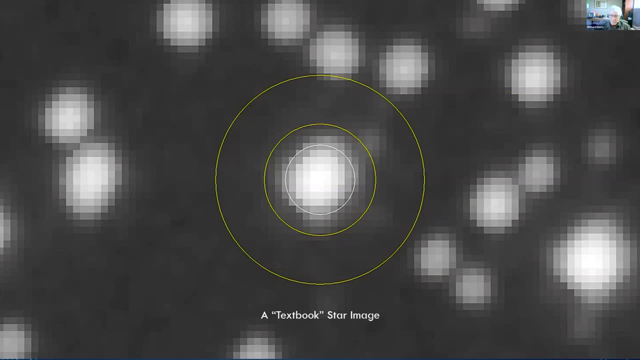 Steven Linthicum A To to get that problem out. Steven Linthicum A. And again, the assumption here, and the assumption we try to make, is that the profile of the star will be the same everywhere in the image. Steven Linthicum A- reality. 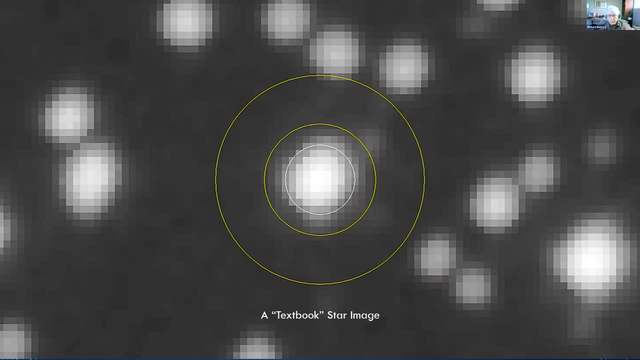 Steven Linthicum A differs slightly. Steven Linthicum A For good, for time it. you really don't want to have your Steven Linthicum A, Your program star in the Center of the field and your your comp stars, often the extreme edges. 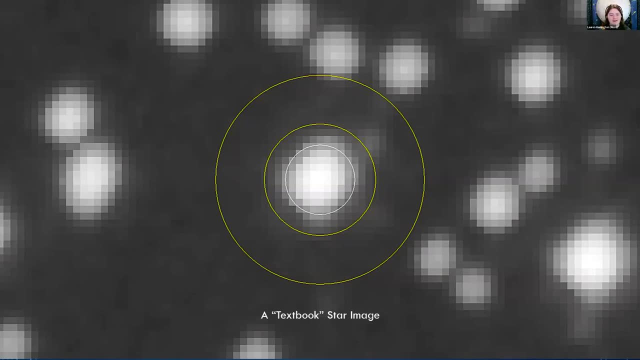 Lauren Ponganen- Right, Lauren Ponganen- Okay. um, the next question here comes from Michael Gardner, who asks: can I do useful photometry in an urban environment? Steven Linthicum A- Oh yeah, Steven Linthicum A stars in, you know, bright city lights and stuff like that. fx stars very, very little compared to how they affect. 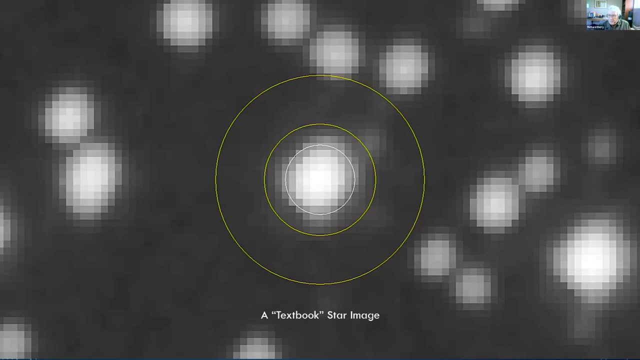 Steven Linthicum A, nebulae and galaxies and stuff like that. Steven Linthicum A, So Steven Linthicum A, yeah, um, so, uh, you know, i mean, i live near a small town, i have about a portal five sky and um. 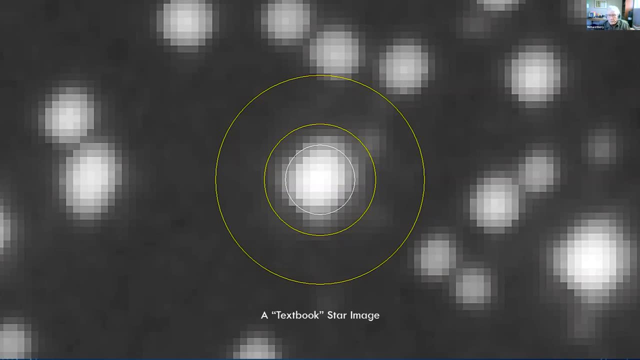 you know i'm reaching 16th magnitude with a small scope, so, um, you can easily do decent photometry. 12, 13, 14, 15 magnitude- well, maybe not 15th, but you know 12, 13, 14 magnitude in a bright sky with 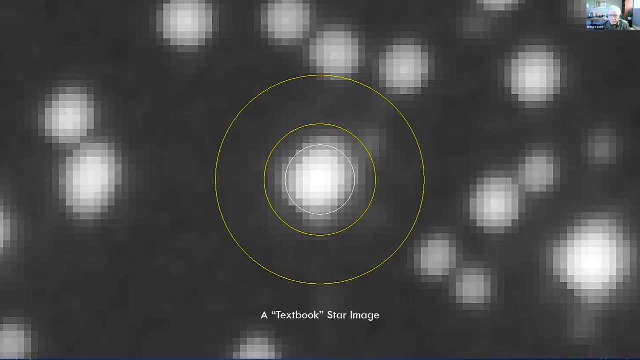 no trouble. and if you have a big scope, um, you know again, the magnitude scale just goes lower. and you've seen, uh, from the images that i showed, um, you know, the we're gonna, we're gonna subtract off the sky background. that's part of what we do. okay, we make it go away. the sky background adds. 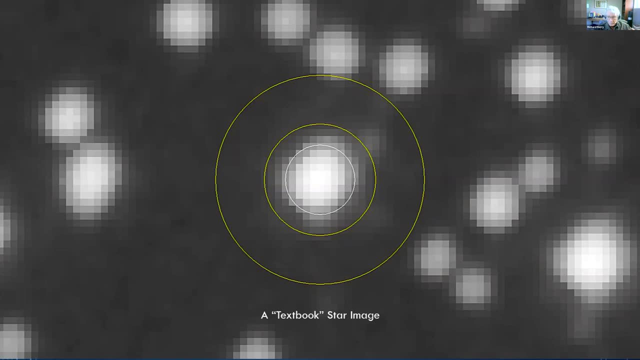 noise okay because of the that random uh fluctuation in the in the signal. um, but if you can see something, you can get photometry off of it. great, thank you. okay, um. next question here from george smythe or smith, who asks um: are professional cameras significantly better? 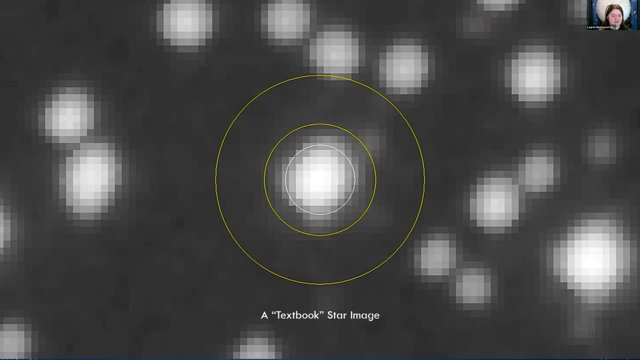 of course they are. i'm not sure quite what you mean by professional, um, if you're talking about astronomical ccd cameras, um, if, if possible, you're looking for, um, well, okay, it's going to be a choice of the, the chip quality, um whether or not the chip has more hot pixels or less hot pixels in a professional camera. 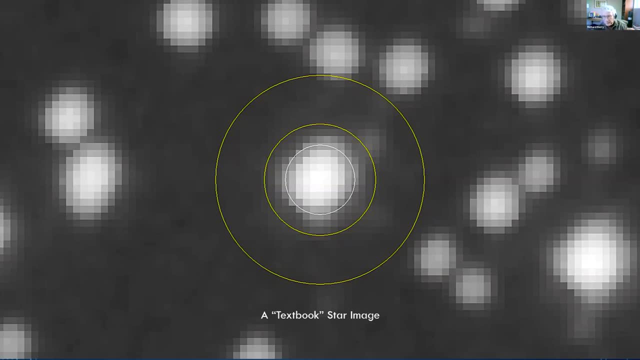 they would probably be using the class a chips or something like that, the chips that have no defective columns, fewer hot pixels and so forth. the quality of the amplifier and how? whether they break the signal into 12 or 14 or 16 bits, um, but if, if, 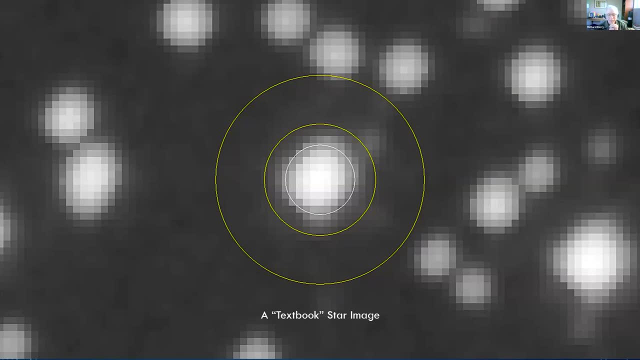 well, if you buy a, if you buy a camera today, your camera is so much better than the camera you would have bought 20 years ago. that, um, uh, you know you, you're going to be able to do good photometry with no problem, because even a cheap 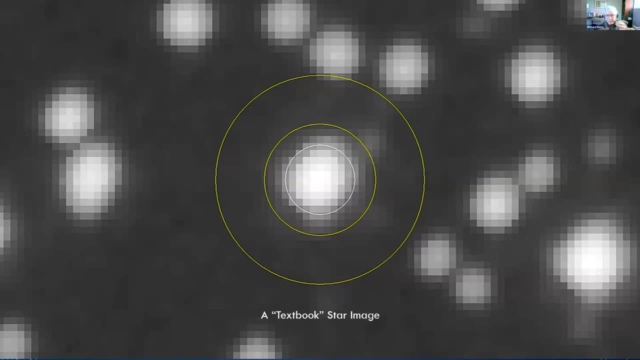 cmos camera. if you use it well, if you stay within the limits of what it does well, you're going to get good results. yeah, that's so true. i mean, the key things are: don't saturate um. the eevee scope, for instance, really can't do good photometry brighter than 11th meter. 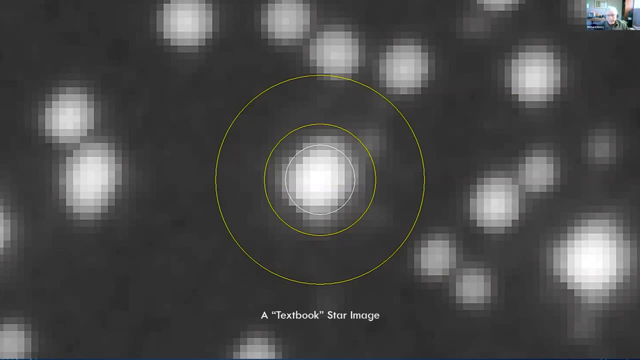 brighter than 11th meter really can't do good photometry brighter than 11th meter. you can't do good photometry brighter than 11th meter because the stars are saturated um and below 15th magnitude it starts to run into um. you know, the results are just too noisy. 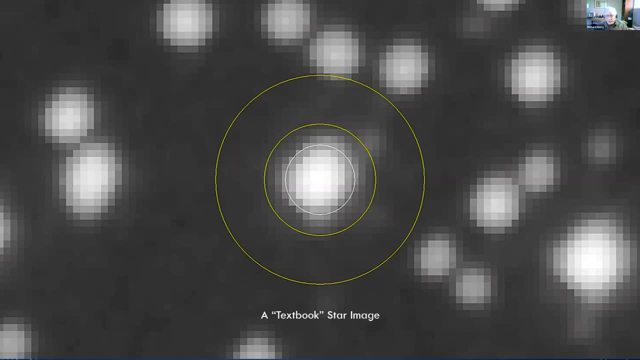 if you push it with a 15 minute exposure you can do 16 magnitude stars, um, but in a four second exposure you're probably limited to about 14th. okay, thank you, um. so just one or two more questions on the topic of general photometry and then we're going to get to. 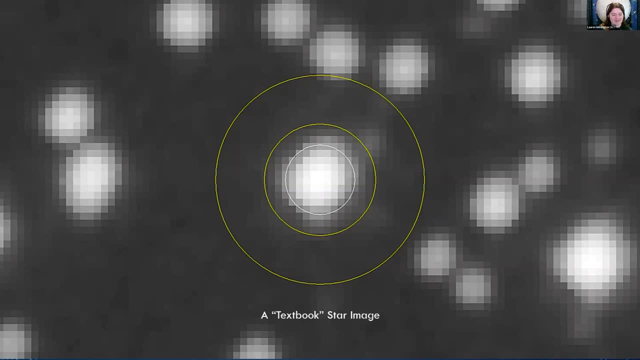 the ones about programming. but uh, real quick, here's one from wayne clark who asks: can you do accurate photometry with elongated star images? um, you can actually, uh, and that is because the the profile of every star in an image is: is, is the same. 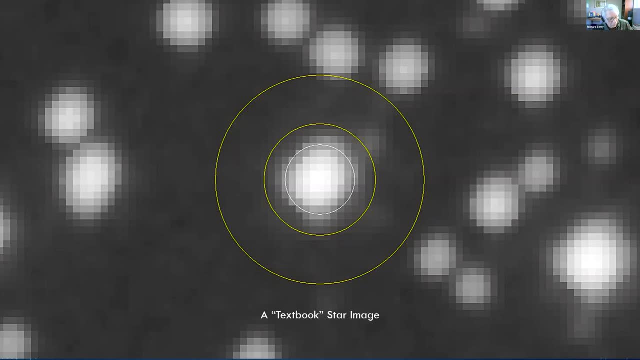 uh, if you do all these final other person of photometry of some star And his mount wasn't tracking well, And the stars were severely chromatic and they were trailed, Okay, so here's, here's Phil's images, and the star goes like boop, boop, boop, boop, boop And then he resets. 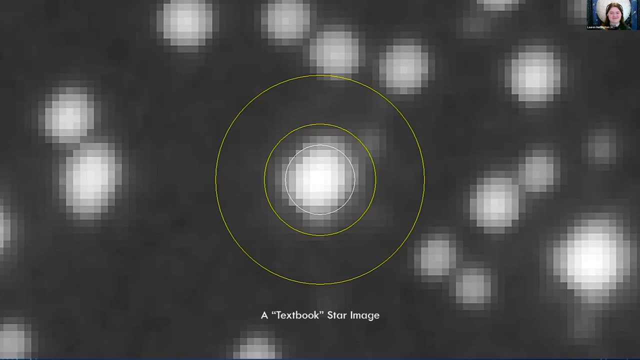 the mountain. So it's trailing along like crazy And it was- I think it was- an eclipsing star. Okay, so you're going to get a late critical stuff. I ran the photometry on it, tried a bunch of stuff And I was amazed he's horrible star images. The 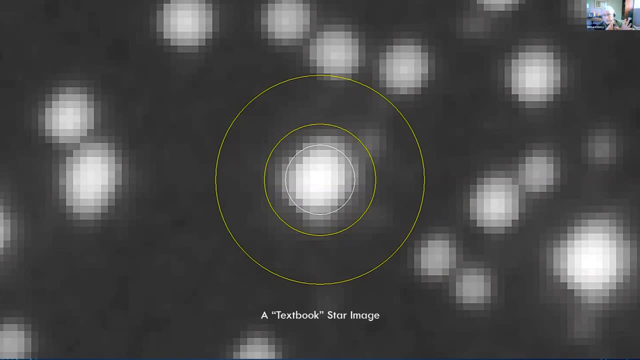 centroid routine is really good at finding the center of light of the star image. Okay, remember, it's a comparison. Okay, you're going to be a comp star and your variable, Okay, and they're going to be affected equally by the trailing, And so 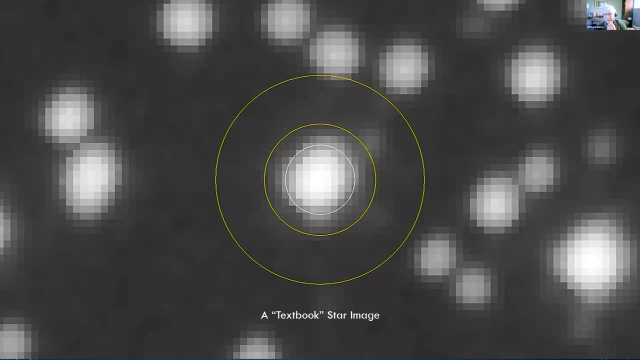 what came out was a very nice eclipse And I went like, wow, I wouldn't have thought it would work so well And the that plot actually shows up in a handbook of astronomical image processing. Now, I would not recommend you use trailed images, But if that's what you, 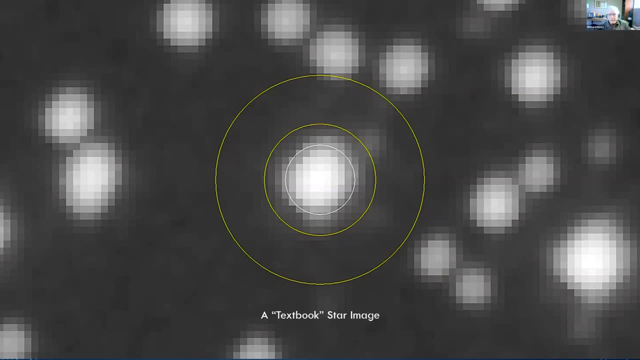 got and you can't improve it. Remember the other thing people do. people do is they say, well, I tried to get my focus absolutely perfect. Well, if you think about getting your focus absolutely perfect, that means you're putting as much light into the smallest thing you can. 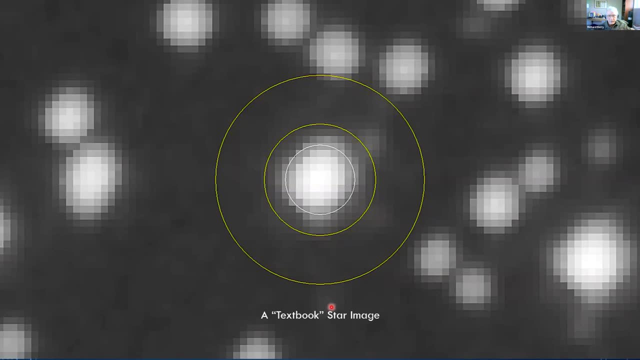 And you're likely to be getting saturated pixels in the centers of brighter stars. So time- a lot of photometry- was smaller than the light, So if you wanted to be able to do this, it would take time before you could do this right. you wouldn't be able to get that. 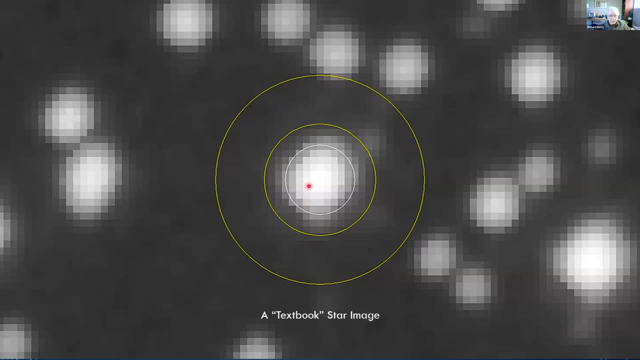 really high of a spot if you were too far from the stars, right. So the use of small telescopes is done, with the telescope slightly out of focus, because then the star image, like this one on a screen, covers more pixels and you don't have a saturated core. 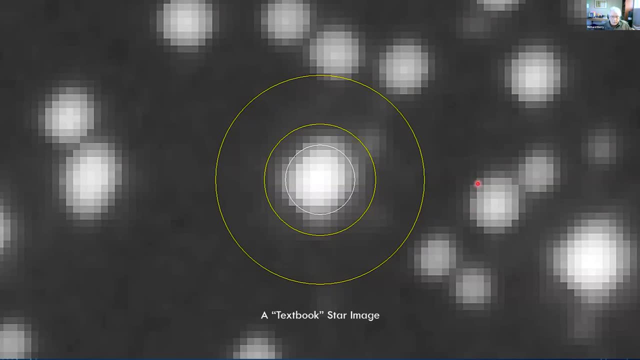 you have a kind of a flat top thing, And with DSLRs it's commonly recommended to be slightly out of matrix, And so you want to make sure that you have the red, green and blue matrices equally sampled. Okay, Thank you, And you actually just touched on one of our next questions. 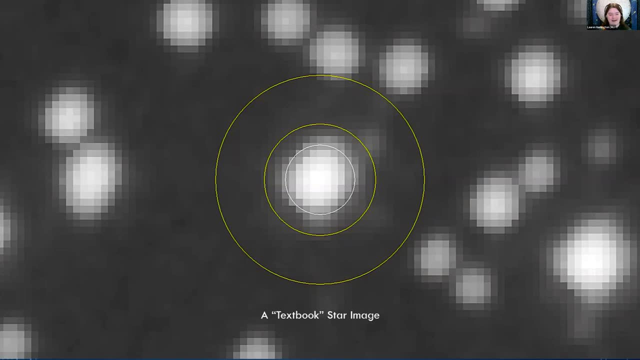 which was about how AIP4Win handles defocused stars. Is it just the same way as in focus? Same way, Yeah. The centroid routine actually works very, very nicely on planet images too. AIP has a planet stacking algorithm. 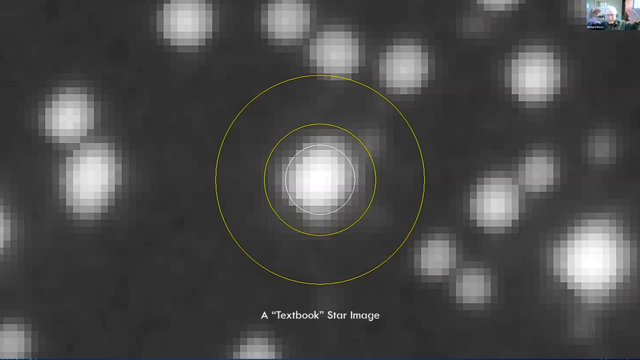 and it just uses a gigantic aperture, 300 pixels in diameter, and it centers an image of Mars or something Like that. It's the nearest tenth of a pixel. I mean, what's amazing is you can centroid it, then centroid it again, centroid it. You keep getting the same result. And in the series of 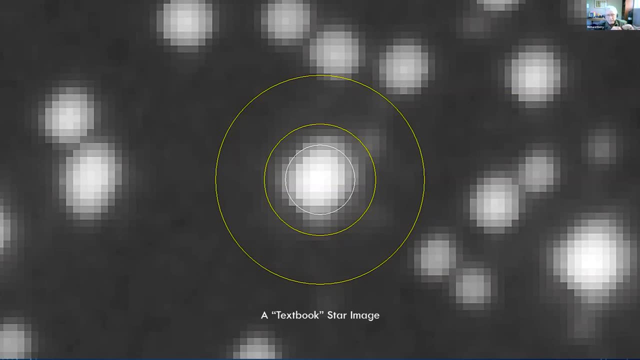 like 200 images. it'll boom, boom, boom. You then make a movie out of it and Mars does not go like this. Mars just sits there and jiggles a tiny bit. That's great. Okay, Thank you. And while 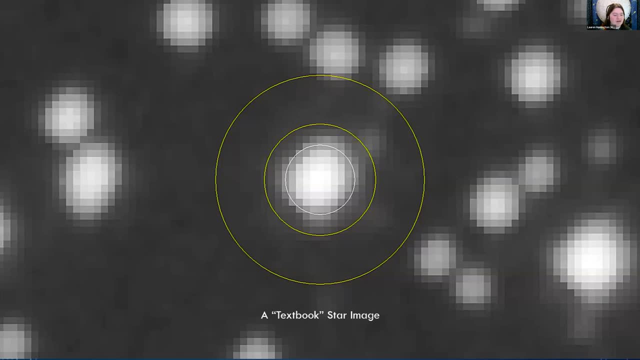 we're on the topic of pixels and how they're handled, Sid, who asked: how does the pixel size affect the end result? You want enough. You want enough pixels in your star image that you're not getting down to using a really 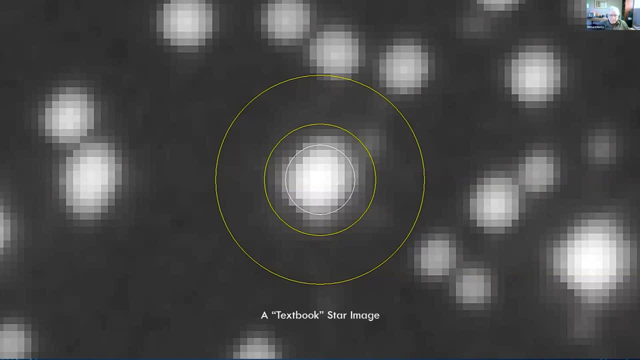 really tiny aperture, Because then you you start to get into that the business of of, um, square edges and is: is any particular pixel included or not? um, i'm not sure exactly what is behind the question. um, if he's thinking, okay, well, let's put it this way: in the olden days, all, all cameras had nine micron pixels. 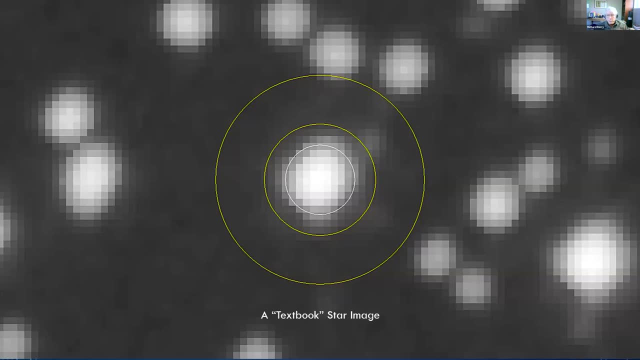 excepting professional cameras, which had 25 micron pixels or 15 micron pixels or 12 micron pixels or nine micron pixels, we typically nowadays we're dealing with 3.75 micron pixels and we're rapidly moving into an era of two and a half micron pixels. 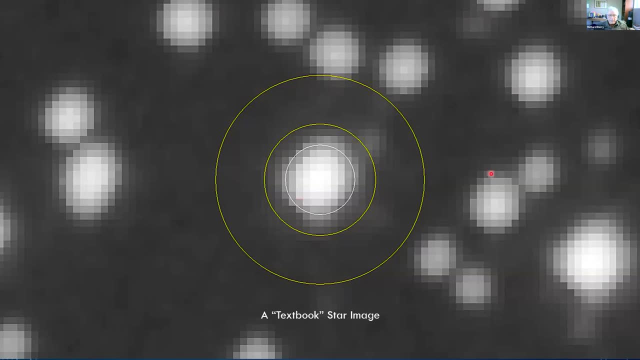 um. the key is: are you sampling the star images adequately? these images are very well sampled. we've got lots and lots of pixels. it's like a hundred, hundred and some pixels in this little box. um and um again, if you're if the brightest pixel value in the image. 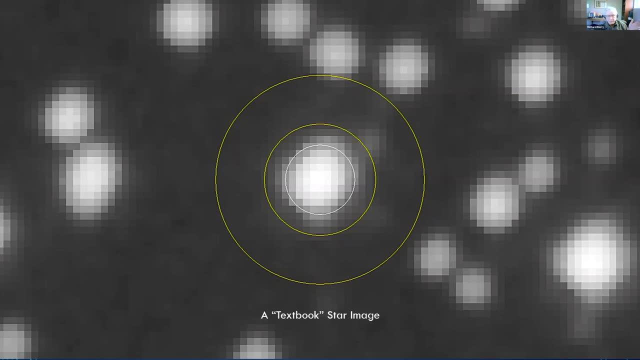 is greater than typically, like 70 or 80 percent of the peak value, you're running a risk of saturating that pixel. when the pixel saturates, you lose light from the total image and that's what happens with with the uh um, with the uh ev scope on bright stars. 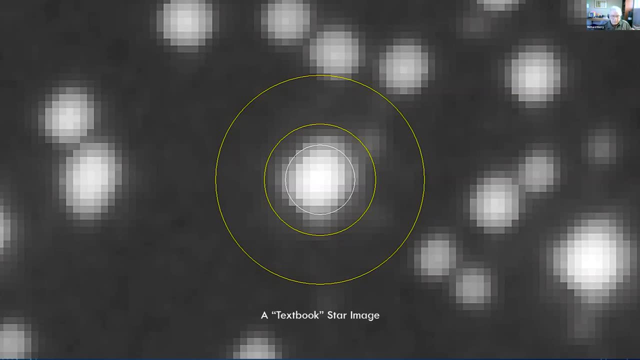 it's, it keeps on recording them because you're looking at the, looking at the light from this outer edges, but this few pixels in the center will be greater than 65 000 and you'll be losing light out of those and when you actually plot that, i actually did a plot, let me. let's see if we can. 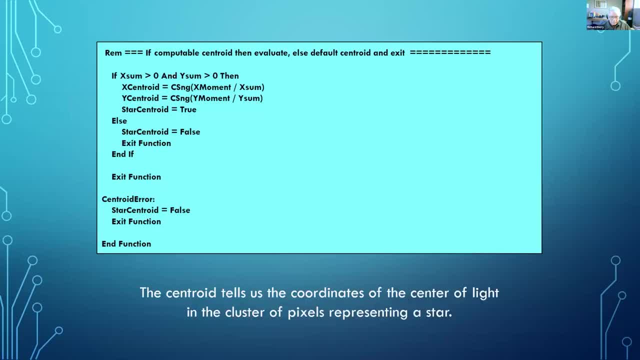 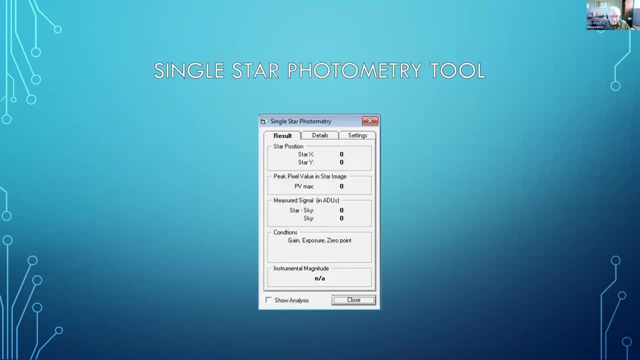 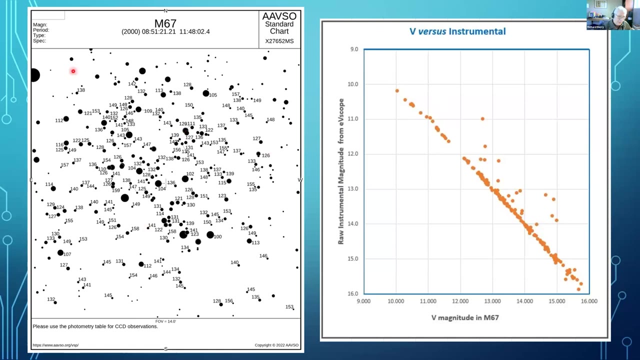 get all the way back to the back end here. um, doesn't go real fast, does it? i had a couple of extra things here. okay, this here here is a plot for m67, which i did using the single pixel tool. okay, and this is the v magnitude, the official standard v magnitude. 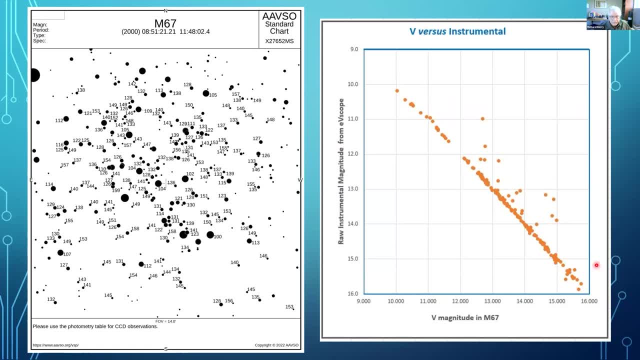 and this is the raw, instrumental magnitude from the ev scope. and you can see like, oh, these follow up so beautifully. and then the curve next over, and because you're losing light now from the ev scope and so it's producing values that are a little low, now you say, well, wait a. 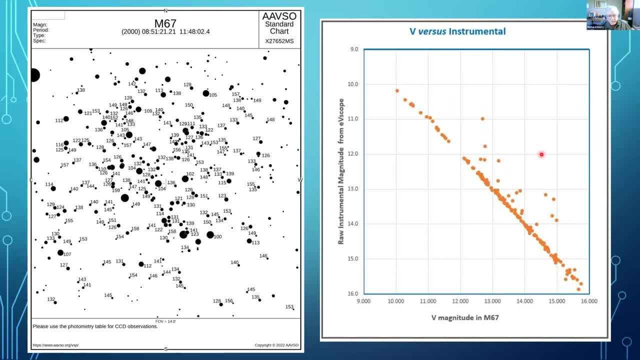 minute. what are all these guys, these? this is m67 is so crowded that it's you often will get light from an adjacent star as you get theater um jumping into it, and so the raw instrumental magnitude will be too bright. you'll notice it never happens the other way, it's always this way. 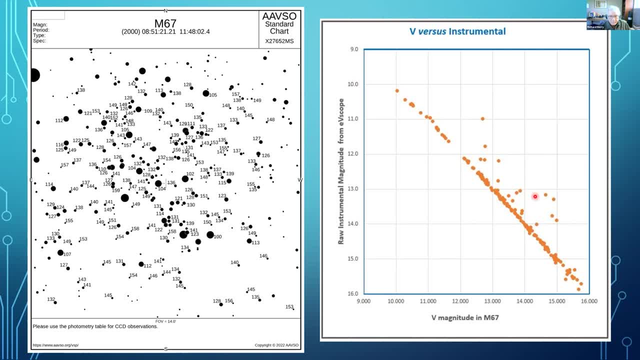 so, um, i mean, i i just wanted to say that. uh, with apologies to visual observers, i tried visual observing and i never could convince myself that when i looked at a star that i could say that is 12.3, i'd look at it and say that's 12, ish, okay, i look at this and say: 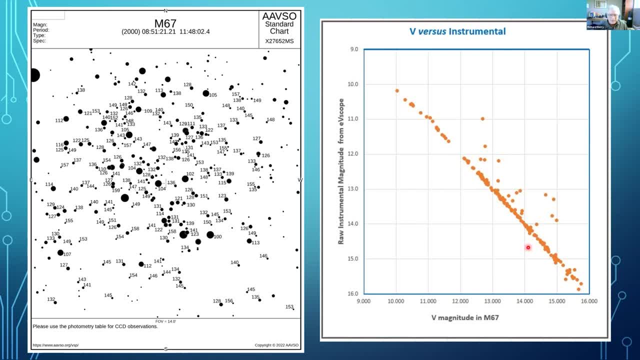 without even you know very, very you can't. you can't do worse than the tenth of a magnitude with with photometry, um, although people do manage to. but if you're careful you can, you should be able to. somebody with a good system should be doing um 10 milli mag. 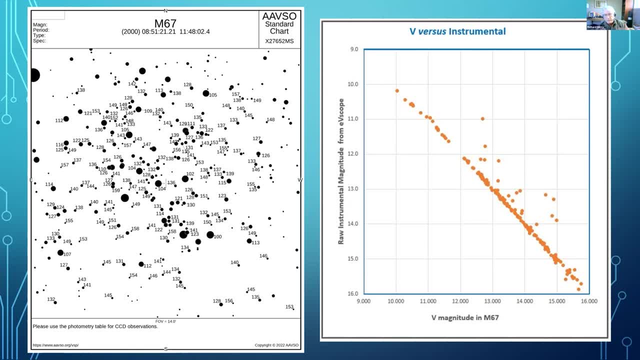 or better, on stars that are not crowded together typically, and, um, i know two or three would be two or three million. two, two or three hundredths of a magnitude, 20 or 30 milli mags would be pretty typical. that's great, okay. um, we have one more question before we get to the 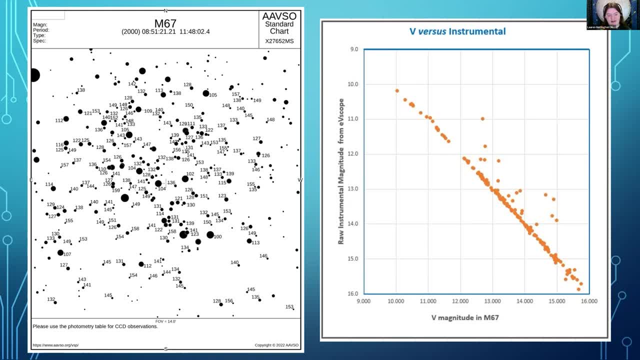 programming questions, and this one comes from paul norris, who asks: uh, will the results of your photometry be different depending on whether you use fits format images or jpeg images? um, yes, because jpeg is a a lossy compression routine. um and um it, jpeg images are carefully designed to look good to the human eye. okay, but they, they throw. 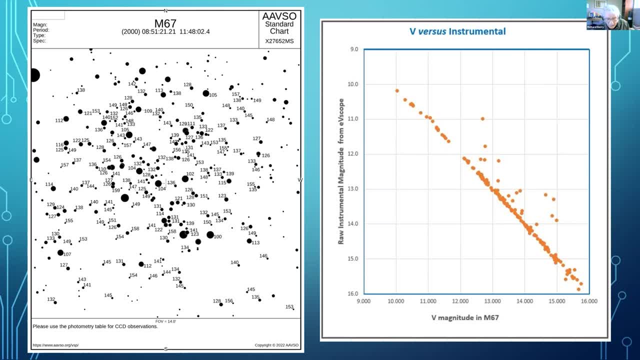 away data, because it's obviously throw away data, because your image is a tenth as big as a, you know, as a tiff image of the same size. um, if you can't avoid using jpeg, then, um, you know, fine, but but, um, it's best not to. um. 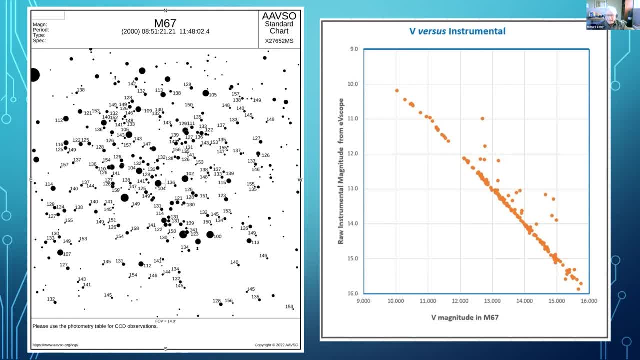 um on. on the other hand, um, i, i'm, i, i like to play and experiment and i mean i'm not a. i mean, one of the things i'd like to do here would be to take my color image that came out of the evs scope and do the same kind of photometry on that, now that data has been very non-linearly scaled. 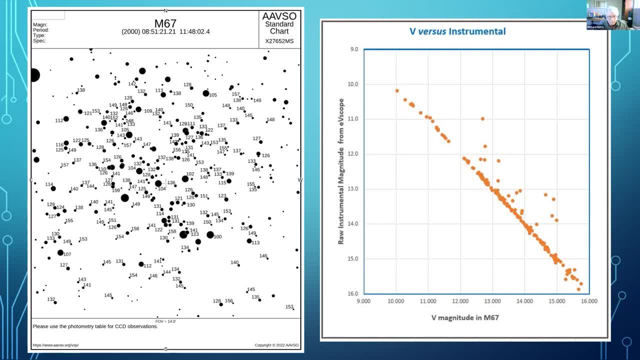 okay because it's been designed to well. it's been processed to look pretty to the human eye, so it would probably be a horrible curve that do something like this and be scattered all over the place fits images by design are that are really important for this thing and you're doing it on the 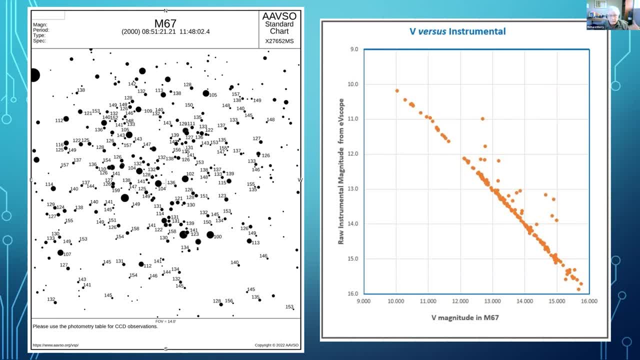 screen and i think it's interesting for us to also know that, um, that fit images, that like fit images. here we can kind of Tingling and all the other things that we can do in terms of that can be pretty. give you back what the sensor saw- JPEG images. give you back what is small and easy to email. 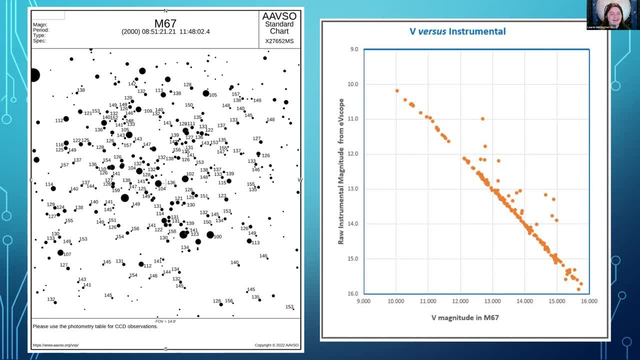 Mm-hmm. Yeah, Okay, Thank you. Now going back over here to some of the questions about AIP4Win and programming. Okay, First of all, we have had a couple questions about what programming language are you using? The program was written in Visual Basic 6,. 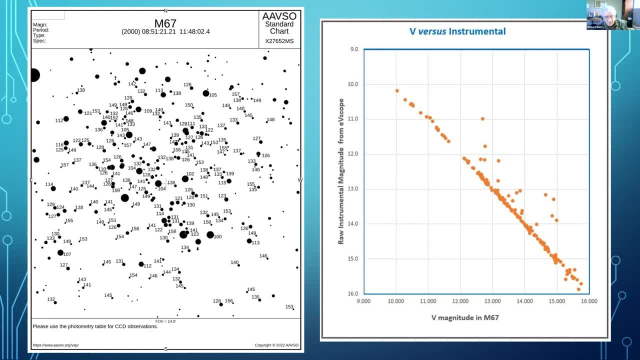 which was the last version of Visual Basic that was not fully OOP, okay object-oriented. It was kind of a mix of somewhat object-oriented, somewhat procedural. It was designed in a way that was not fully OOP. It was designed in a way that was not fully OOP. 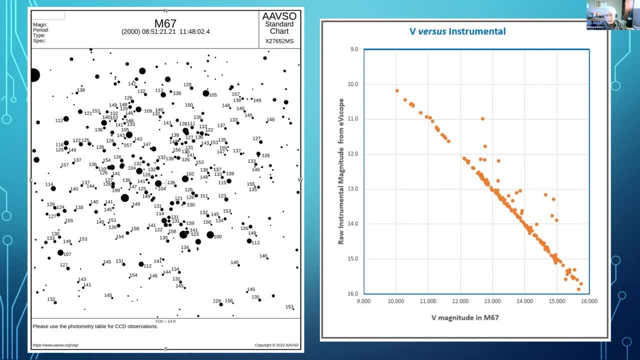 It was designed by Microsoft to be very easy to prototype software. It dates back to about 1995, 1996.. Its problem nowadays is that it's 32-bit code, which means that the program can access about two gigabytes of data. Now, by the time it's done, it's going to be. 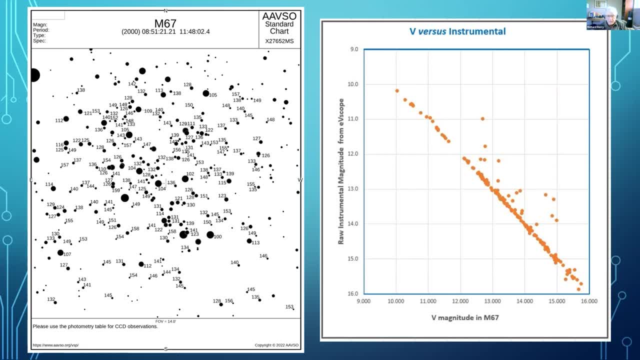 run time, libraries and stuff are loaded. VB6 can access only about 1.3 gigabytes of memory And we use 32-bit floating point data throughout. Okay, So when you have a color image, we have 96 bytes per pixel, Is that right? 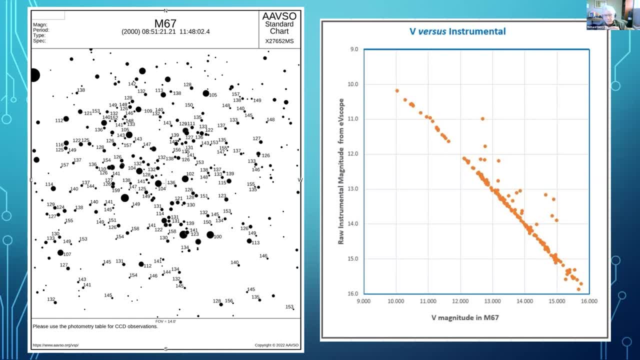 Yeah, no, yeah, And you have a 10-megapixel image. you can suddenly see you're using a good fraction of the memory that's available to you. So AIP4Win can work very nicely with six-megapixel DSLR images, Somewhere around eight or. 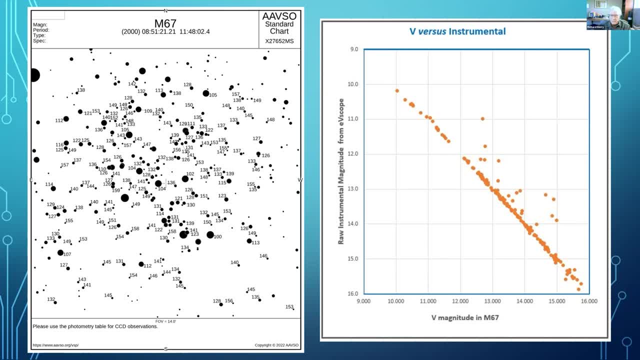 eight to 10 megapixels, you start to have to be very careful how you use your. you know anytime you, if you have three images up on the screen, you're fine. Add the fourth image and you run out of memory. So the the on the other hand, I just the other day. 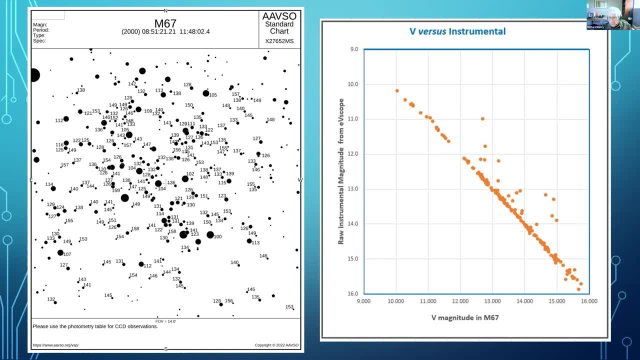 I loaded a monochrome image- okay, which has takes as much from a QHY600 camera, which is 61 megapixels, So it only takes 180 megs in memory. That's easy because we got 1.3 gigs. 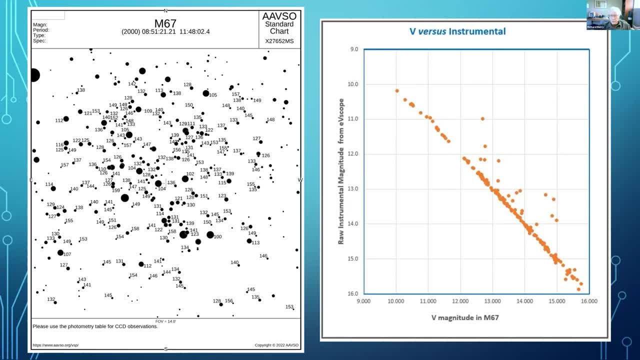 So I can do almost anything I want with these huge 65 or 61 megapixels images from the QHY. But you know, a much, much smaller color image from a DSLR will will leave me with too little memory to work with. 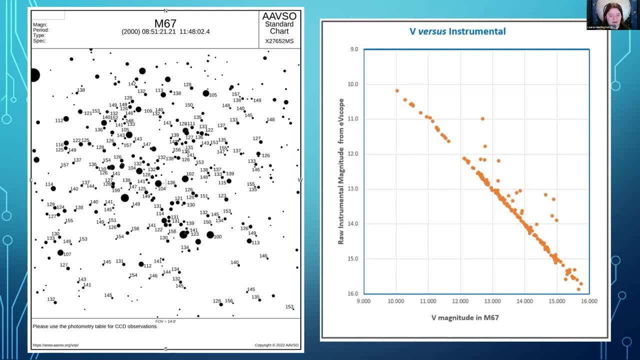 I see Okay On that topic, Wayne Clark had a question. He said when William Wilman Bell was in business there was a list of DSLR cameras that would work with AIP4Win. Is that list still available, Because his DSLR wasn't on the list. Would you like to see the list? No, When Wilman Bell went down, they went down really quickly because of of health issues that Perry and Pat Ramaklis, who were the owners, had, And I don't know exactly what happened, but I don't know, I don't know. 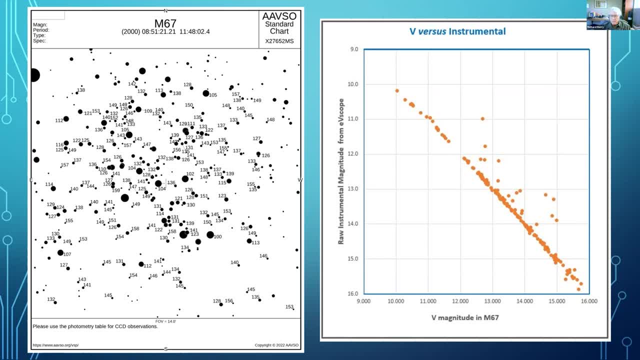 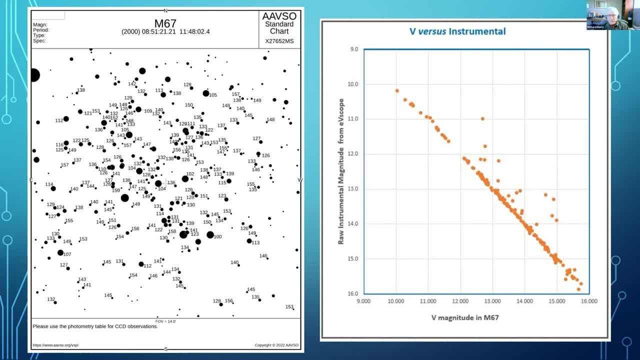 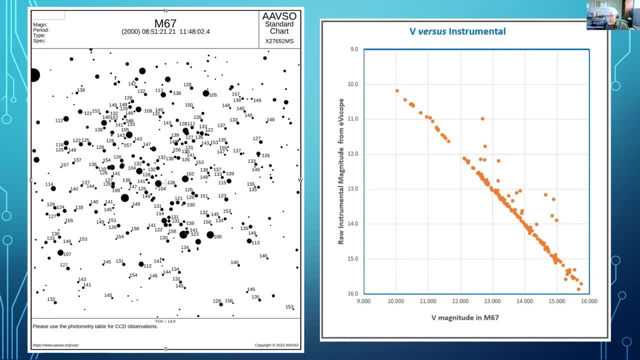 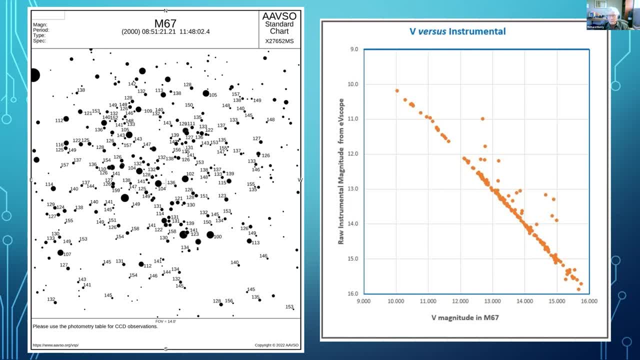 we came. you know that, far from from losing the source code entirely, Wow. Now um, um, um. When I realized that the software would have no support unless we did something about it, I called up my buddy, Jim Burnell, who was the co-author of the book and worked with 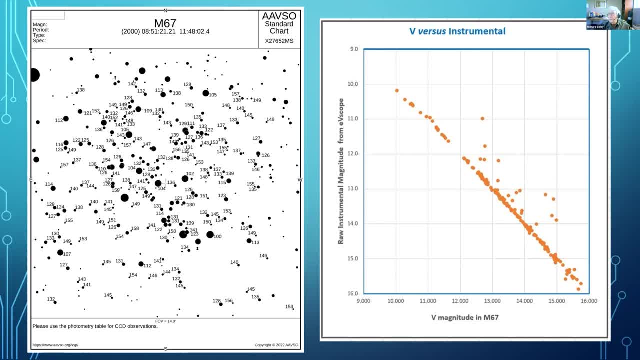 me for years on the software and he had an old Windows 7 machine that he was using to make the distribution packages. So he shipped that to me by FedEx and I set it up and that's how we built the distribution for the new code. 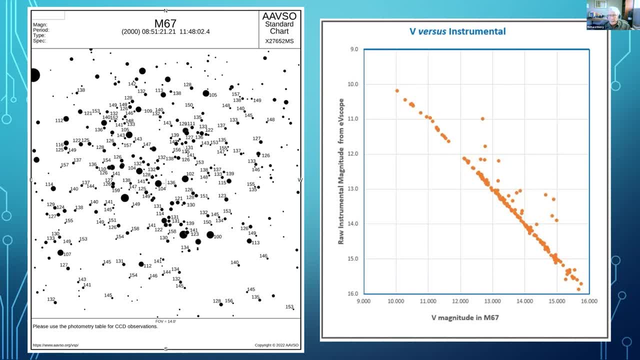 And 2.4.10 had in it a bunch of diagnostic code for me as a programmer. So everybody who runs this thing, they run into these things where you get these development messages, And I did not have time to find them all. 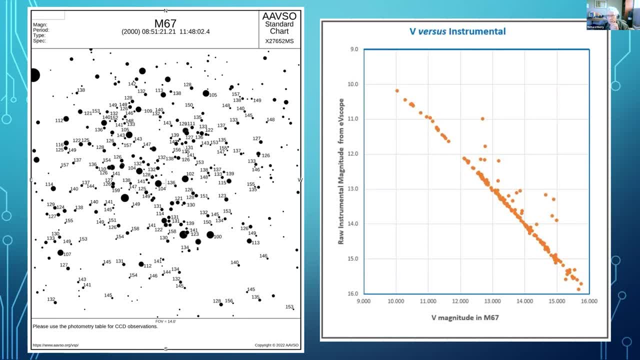 So there's some residual bugs in the software that's available to people And what the Groupsio people do, which is, I totally appreciate, the community there. they will answer a lot of questions that come in from new users, So I'm going to show you some examples. 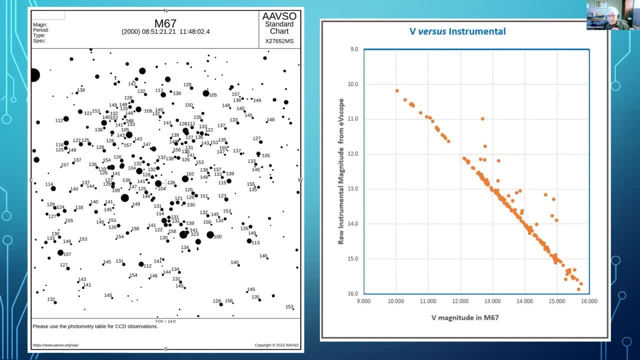 And I'm dealing right now with a question that's up on the site of a guy who has installed it and it's running just fine on his computer. but he has a couple of students and it won't run properly on their computer. I wrote him and I said I think what's going on is they have school computers. 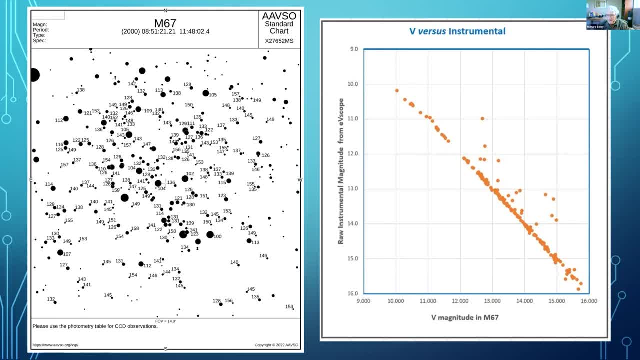 And the computer is not working. And I wrote him and I said: I think what's going on is they have school computers And the computer is not working. I wrote him and I said: I think what's going on is they have school computers. 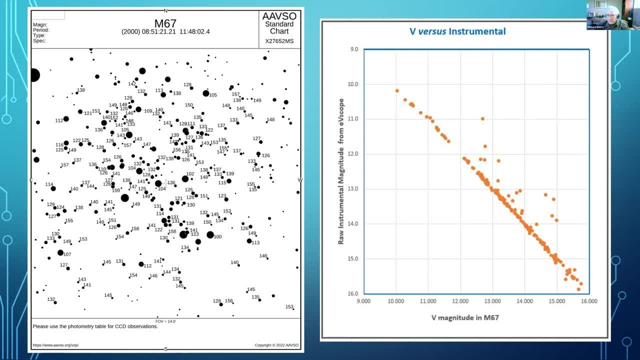 And he replied: I think it's a pretty bad nightmare. I said: well, I'm not going to run it. I said I don't want to run it And he said: no, you can do it. I said, no, you can do it. 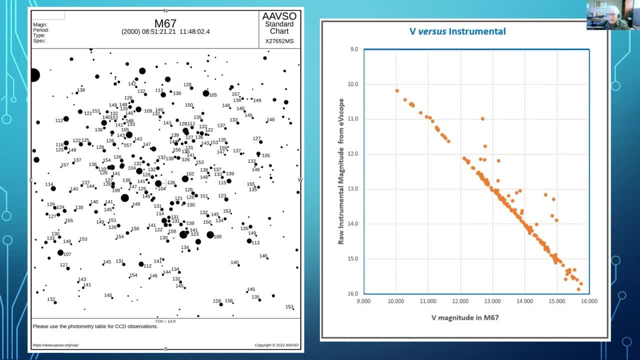 And he said there's software on the school computers. It says if something doesn't say Microsoft, you can't, you can't run it, or something like that. So we're. every time you have to diagnose a problem in a individual's computer, you're. 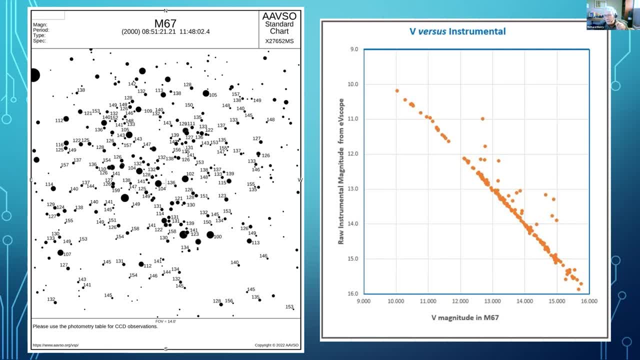 dealing with a computer that's like no computer I own, Because- and, by the way, I've just installed AIP for Windows on Windows 11. And it runs just fine. runs just fine and allegedly windows 11 fixes a lot of problems that windows 10 had okay. 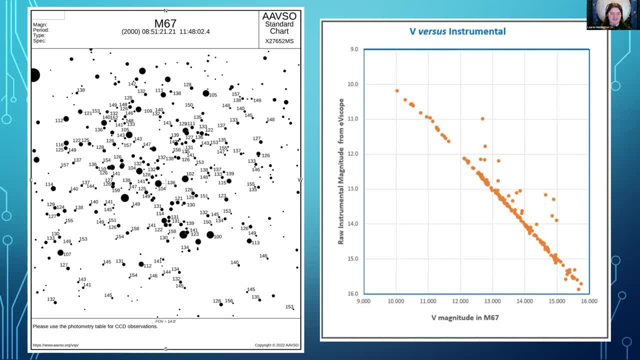 hopefully. probably my computer's going to update without my will one night and i'll find out then. no, you can tell it not to. so, um, oh, where did the next question go? i've got quite a queue here. um, um, okay, oh, yes, so on on the topic um of development of aip for when? 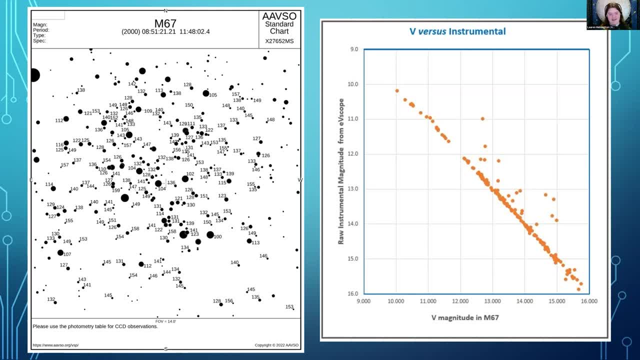 um, we had a couple of related questions. one was: will the existing um aip for when bugs be corrected in sometime in the near future? and the other was, more generally, what is the what is the future of aip for when? look like right now, um, what i want: the future of aip for when. 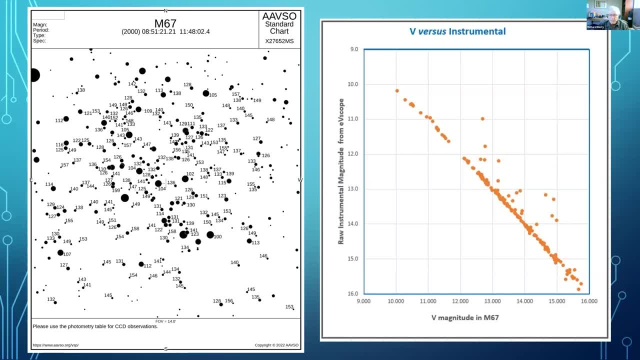 look like: um. what i want the future of aip for when to be, is to move into a different programming platform And that supports 64 bit code. Okay, then we the limitations will go away. I see absolutely no sense in playing around with. 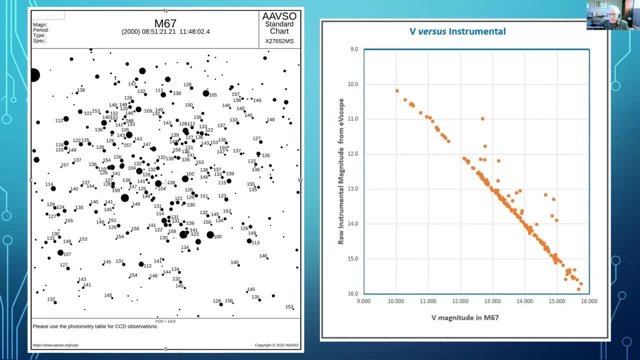 code that makes pretty pictures anymore. There's already lots of other expensive ware out there for handling DSLR pictures And it's getting. you know. I mean even Photoshop and some of the other software out there is doing a great job with pretty pictures. 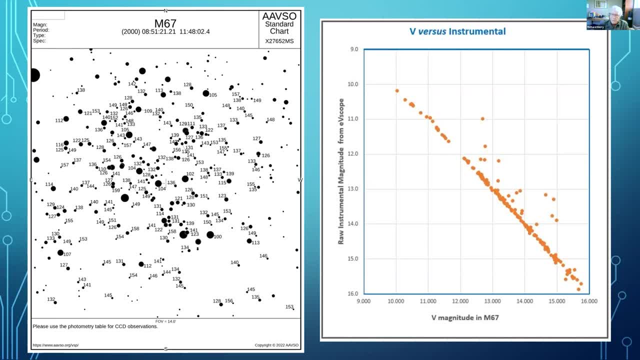 So I intend to focus on science applications And we are looking at, you know, greatly improving that way around, I think, And it's it's a tremendous output over time, But we're hoping that it's what we're looking for. So we're working on a two dot four, dot 50.. 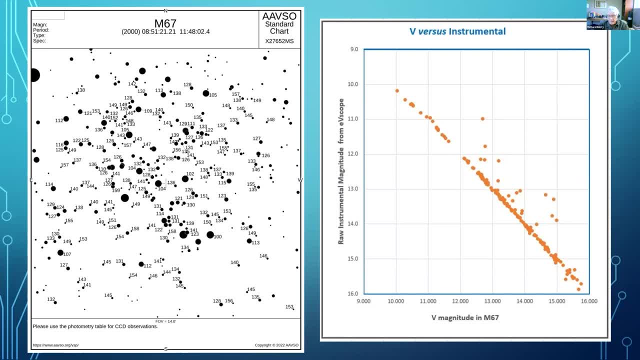 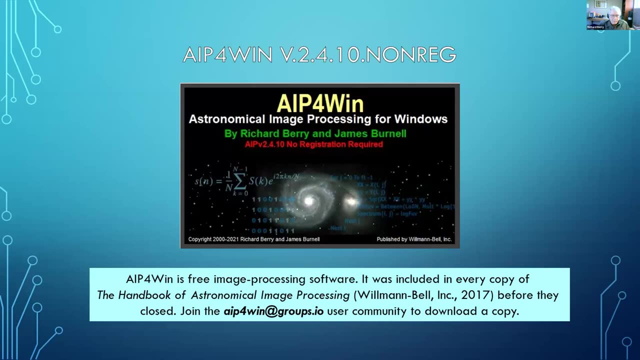 So in the visual basic six routine it's handling of astrometry. In the Visual Basic Six routine my last working version was twofor that 50. Okay, so I had done a long. So if you have a working version of 2.4.8, and you simply take the executable 2.4.8, the two executables can sit side-by-side in the same directory and Windows doesn't know which one of them is running. So you can fake out Windows. The major difference between the two things was that 8 requires registration, 10 does not, And that, well, I keep saying no registration required, but you pay a price. The number of complaints of stuff that doesn't work have actually been amazingly small. 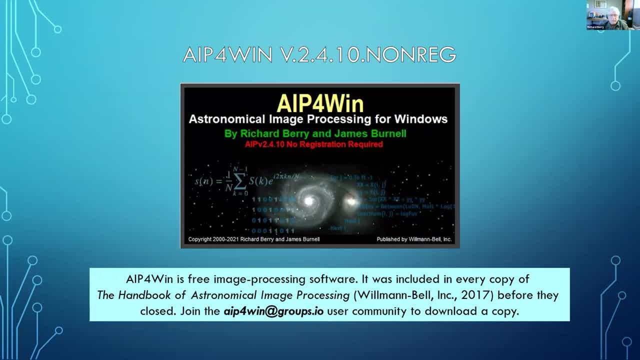 Mostly you have to put up with Windows that every time you save an image it says it just goes through a bunch of checks that I put in to make sure I was saving properly, for example, Right, Okay, Next question here About when you were showing the procedure where it was calculating the magnitude and just displaying it, you were showing how simple it can be in video game-like. 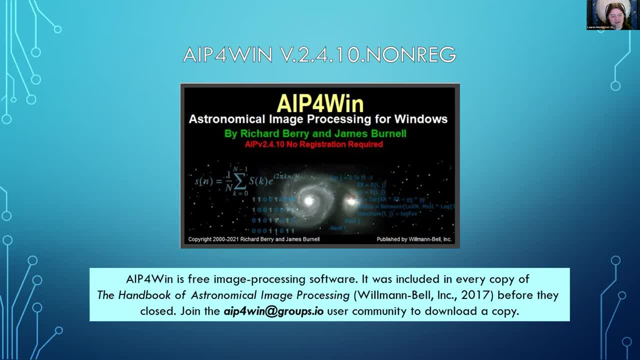 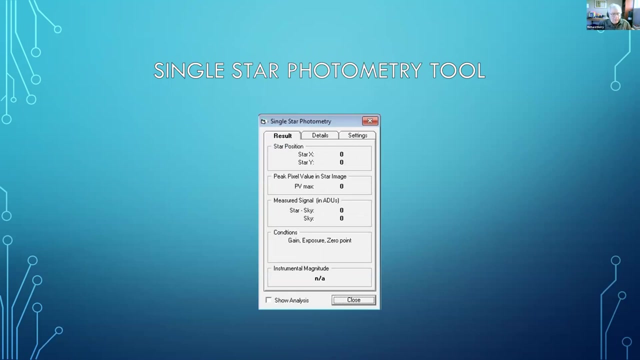 We had a question come in then that said: wow, so the target star magnitude is computed without needing to select a comparison star. Ah, okay, Yes and no. Okay, There are six. I think it's six- photometry tools in AIP4Win. 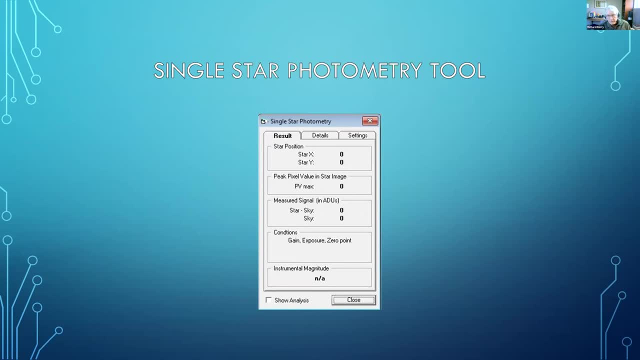 What I was showing you was the single star photometry tool. Okay, When we wrote the software and we wrote the book, we were thinking of educators a lot. Okay, And a single star photometry tool is nice because you can go into an image like the one of M67 and you can click on different stars and you get magnitudes. 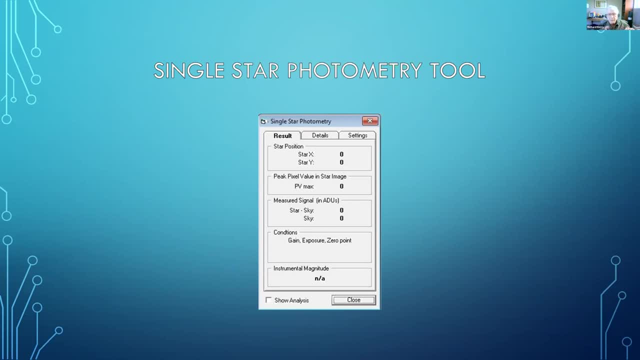 But then you have to realize you have to set that zero point. So you go to something like M67 and you have the list of the magnitudes of all the stars And you click on a star with a known magnitude And then you go into the settings tab, which would be here. 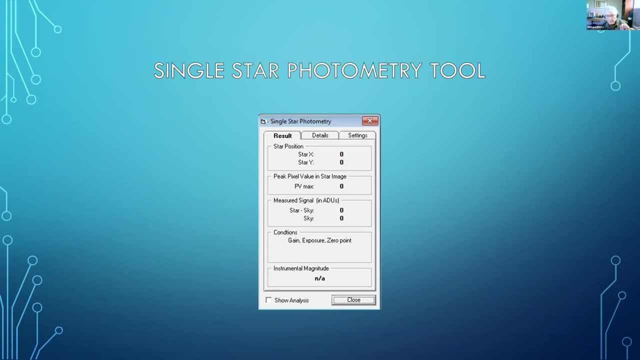 And you set the value of Z to be a value that gives you back the catalog value. Now you go click on other stars and bingo, they give you back the catalog values with small uncertainties. Okay, Now, This was to show you in terms of an educational thing. 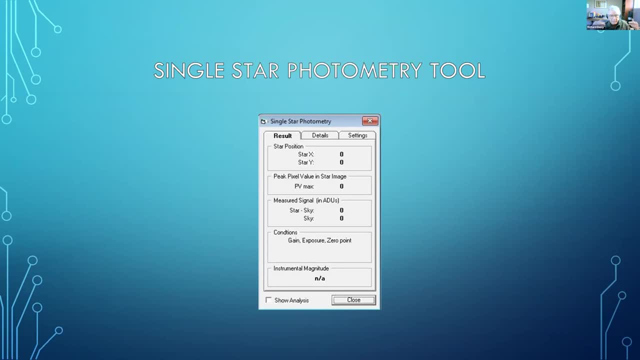 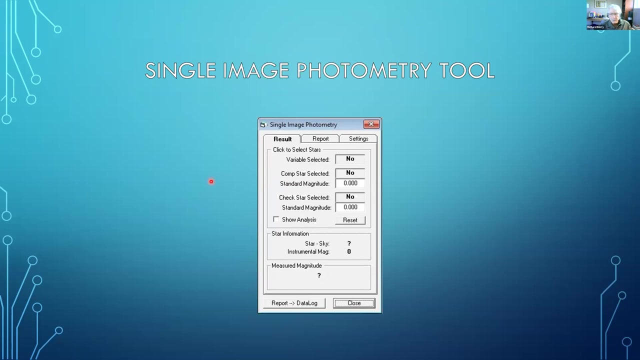 It showed you that a raw, instrumental magnitude is a magnitude that is unanchored, because Z is something that you choose. Okay. The next is the single image photometry tool. Okay, And here it expects you to click on three stars, It expects you to go over and you click on the variable, and this will then turn up. 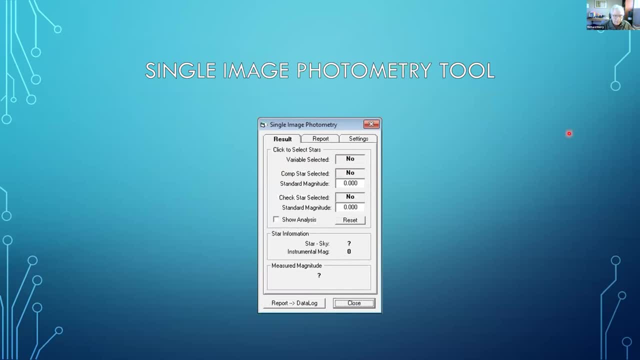 It will say yes, Click on your comp star, and it will click on the comp star and it will put a C next to it. Then click on your check star and it will put a K next to it, And then you enter the standard. 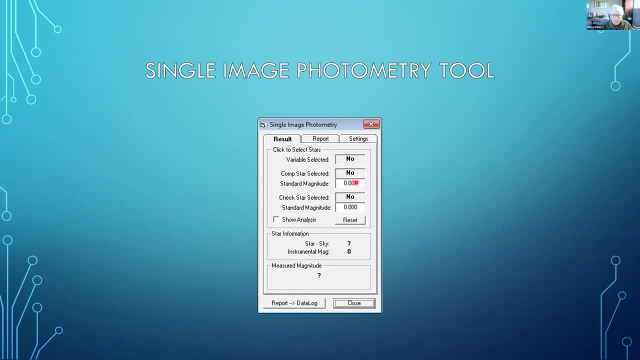 Well, okay, Then you enter the comp star's magnitude. Okay, So it's a you know 11.25 magnitude. You put this number in when you click Rather Yeah. As soon as you finish that, it will give you back. 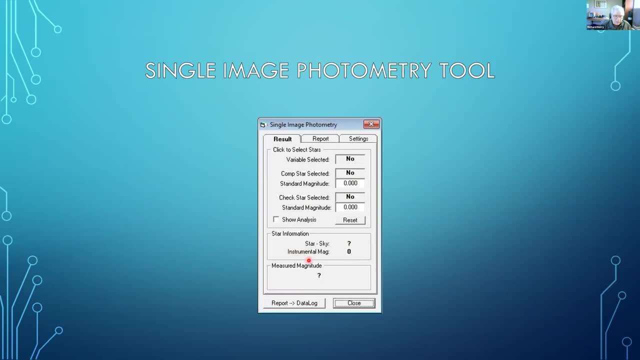 Okay, The star minus magnitude, star minus guy and instrumental magnitude. So there's your magnitude And then it will measure them, Give you the measured magnitude, And now it's making a comparison between the comp and the variable And it will also tell you what the 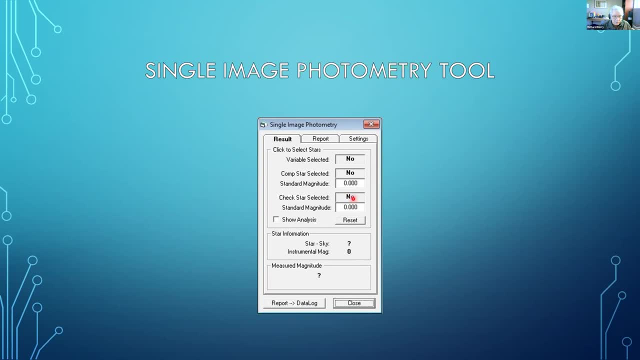 Computed magnitude for your check star is. So you should get that. when you click on that, Those three stars, You'll get back The magnitude of the, the unknown magnitude, And you also get back to magnitude of the check. Okay, 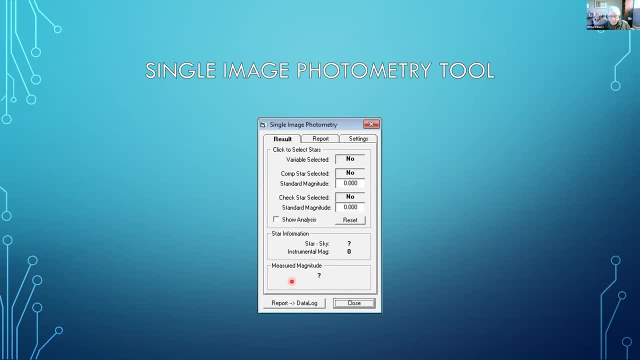 And then visually you go like: okay, The check star matches the Book value And the magnitude of the check. Okay. And then visually you go like: okay, The check star matches the Book value And the magnitude of the check. star matches the. 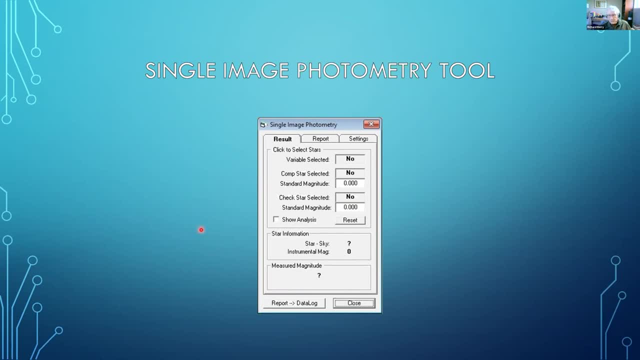 Book value And the magnitude of the check star matches the Book value. I'm okay, And this is again Thought of as a teaching tool. Okay, So you can have students and they can go through and they can begin to understand. 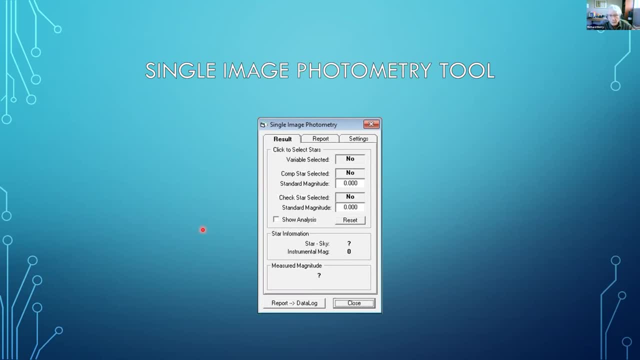 That all magnitude calculations are differential Between a known comp And an unknown. And then you've got to check, Because who knows that the standard That your comp stock Is Okay. So it's, it's, it's, it's intended for teaching. 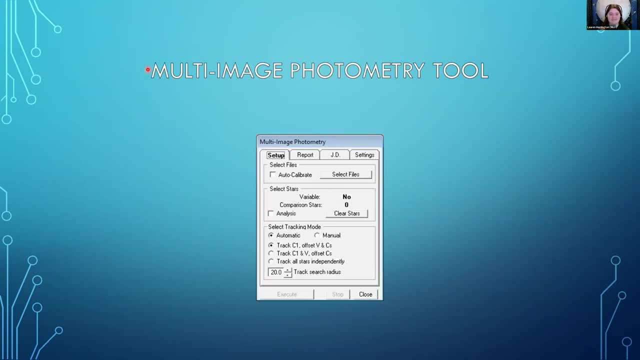 Great Multi-image photometry tool Does Almost exactly the same thing As the single image Photometry tool. that expects you to pick three stars, But you can Put in a list of like 500 stars And you select on the first one. 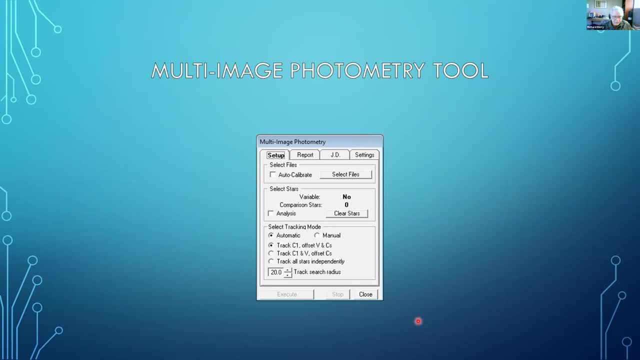 And you click, click, Click, use the stars I want. And then you click Do it, And it Loads each one of those 500 images And runs the time: Bang, bang, bang, bang bang. And it's really cool because it'd be going like: 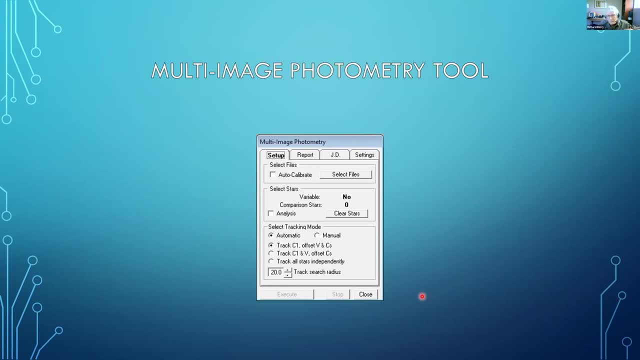 Two or three images a second, That's great. Think about doing that manually, Basically, By the time it was done, Right, Okay, And when it And It's now, I consider it out of date. How do you do that? 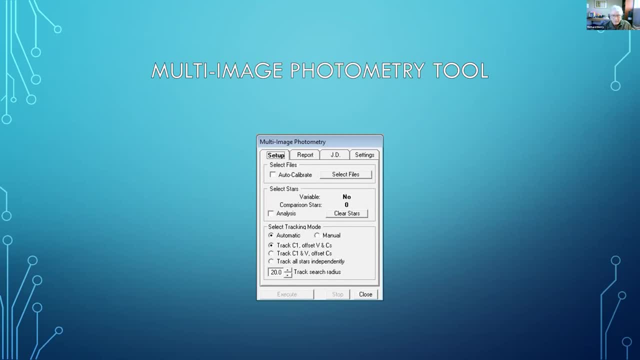 How do you do that? How do you? How do you Do that? Yeah, So You can do that By Using the data. However, it works really well And we have observers. I've been using it for years. 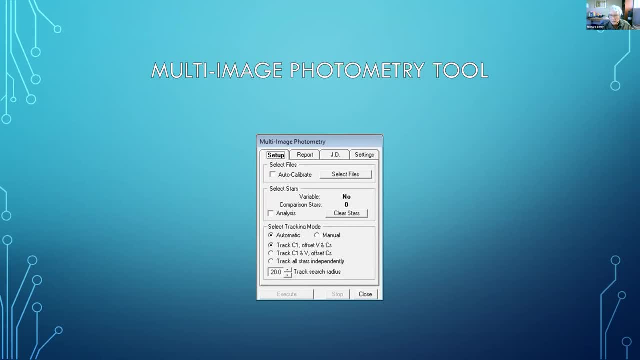 And to keep their results consistent, They keep using it So that there's there's no changes in their techniques. Okay, So that's internal consistency of your work. V- Yeah, And it does things. It does nice things, like it computes the Julian day. 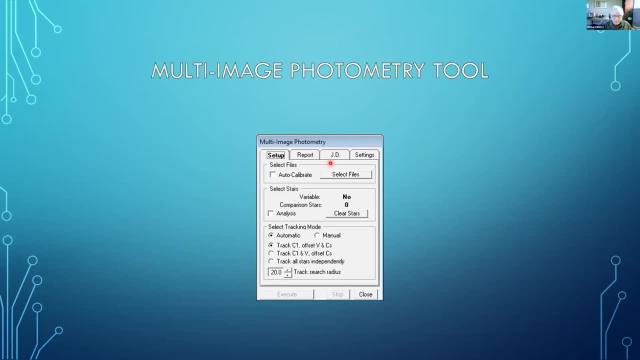 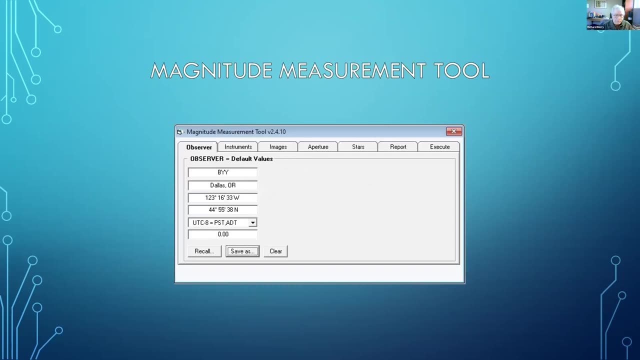 And stuff like that. So it's producing um output. the next tool is the one that i want people to use, because it is the most sophisticated um and this is be. this is designed for production photometry, so i can fill in, for instance, my observer value, my latitude, my longitude, all the values that i 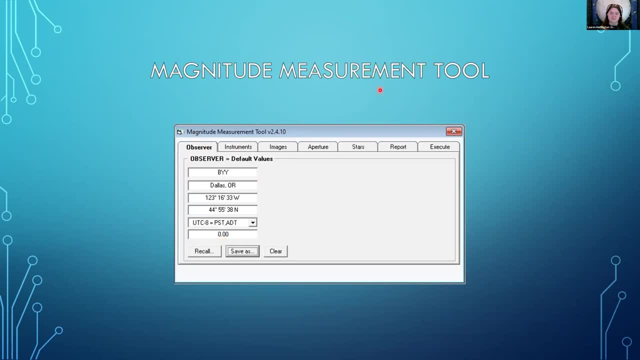 need to produce a complete report and avso report is one of the formats. center for backyard astrophysics is another format um and there's there's, there's also a dump, every bit of data you ever get uh format um, but so my observer, i set my observer and it loads my observer thing. 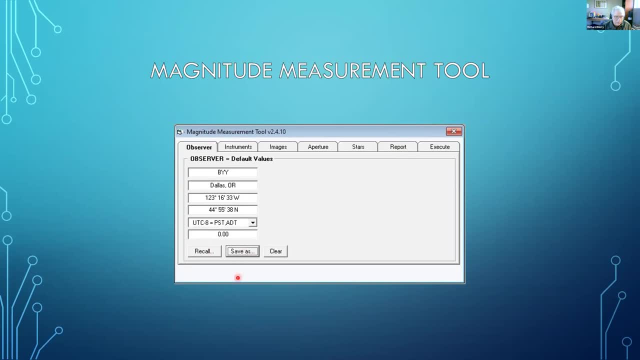 i can recall that, um, i can save that. i can also recall my observer format for my old house, where the byy was the same but it was in a different location, okay, or if somebody sends me some files to look at, i can load in that observer's stuff. then there's the instrument thing which lets me 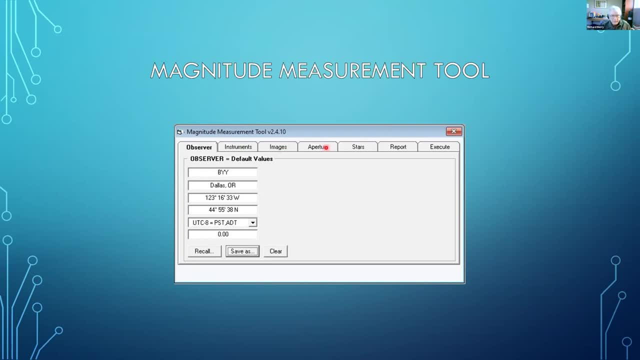 put in the telescope data, then i can make a list of the images, then i pick my aperture, then i can pick up all the stuff for a star, like you know, i can have dozens and dozens of little star files and they will fill in all the data i need for the check and multiple comps and then i can do. 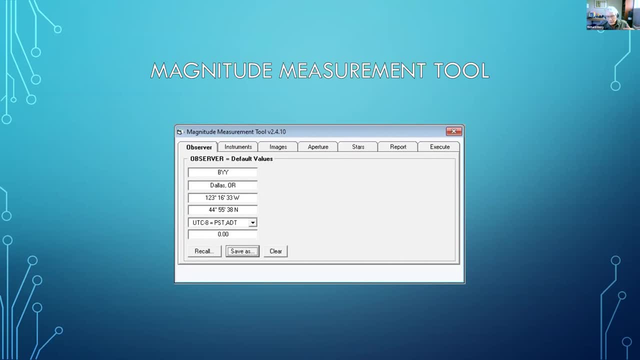 different. and then, finally, we have the execute thing, which also has a, a star, that um, you're now dealing with things like um, asteroids that are moving through the field of view, but you have to keep the stuff. you know it's designed for heavy duty production stuff. and then, finally, 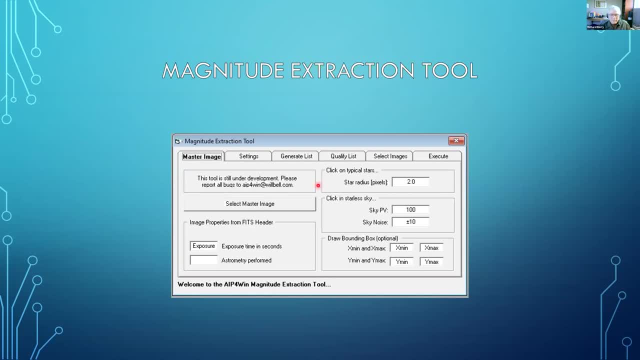 there's a magnitude extraction tool which is designed to find every photometric star in the image, and i've done some uh stuff with with globular clusters, where i've gotten 8 000 stars out of the red, green and blue images. then you can plot it and show it to your computer and then like the with the global structures. 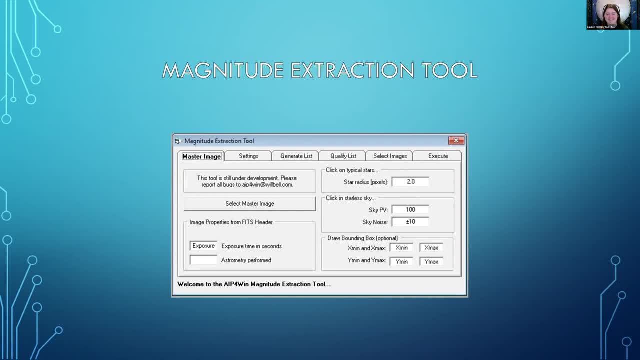 then you can plot it and show it to your computer. and then you can plot it and show it to your computer. hr diagram- whoa, that sounds really cool. so i mean, you know, as as years went by, we developed these different tools to do different jobs, and the magnitude extraction tool, um, you know after, 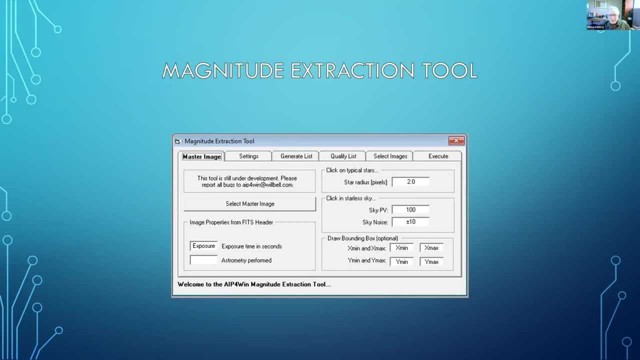 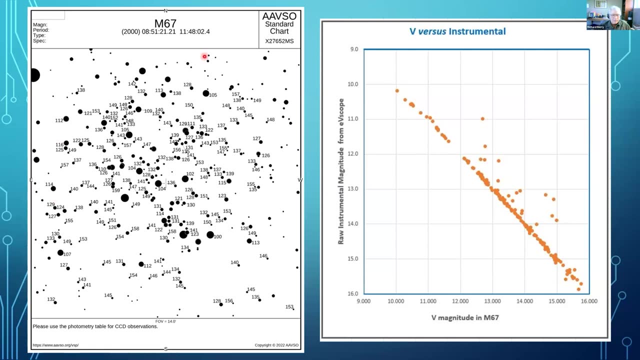 after spending like three days manually doing m67. uh, okay, with the single star. uh, i went into the magnitude extraction tool and, um, like in three seconds it did all the stars. wow, that's wonderful. okay, i'm definitely going to be looking into that. um next question here comes from ari sequeria, who asks if there is an updated tutorial available. 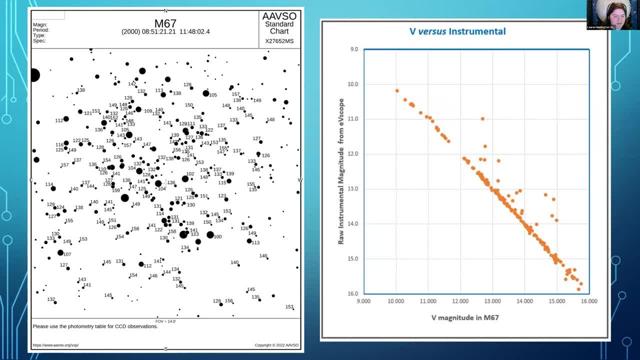 for aip for windows. um ari says they have the book, the uh original cds and version 2.4.10 running. okay, but appendix c tutorial does not always seem to match up with the actual software. um, no, it doesn't. um as a, as a programmer and a book author. 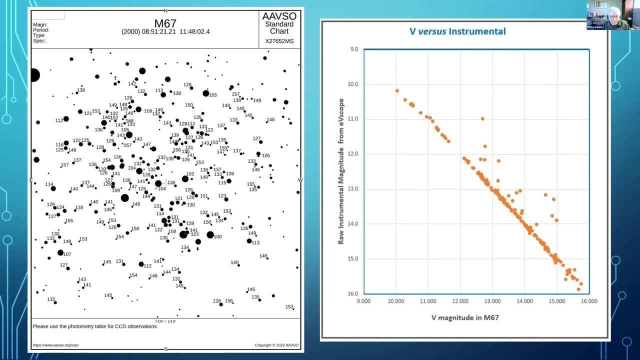 and stuff. i have to say that programming is very fast compared to documenting mm-hmm okay and um uh, keeping a book which gets printed every two or three years and keeping software which you can go through in the earlier days of aip for windows. um, i tried to release a new update. 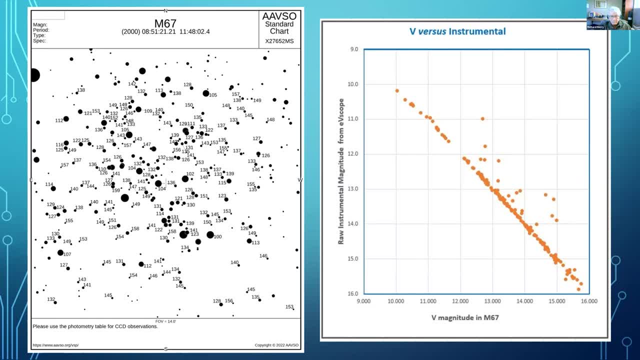 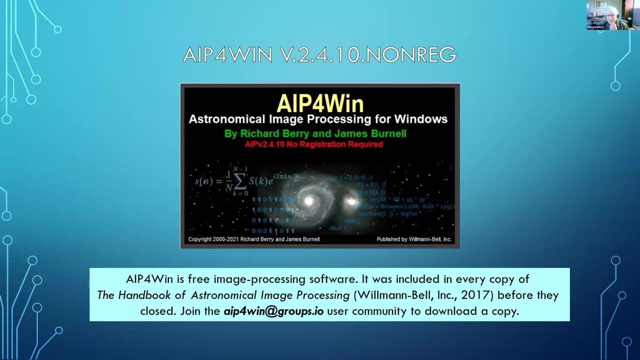 every two or three months. um, because we kept getting a lot of bugs and we we kept getting user requests and we kept getting bug fixes and so we just kept the software moving forward. um after after. uh, my partner in in crime, jim vernell, got a promotion at work and suddenly got more pay and more work. 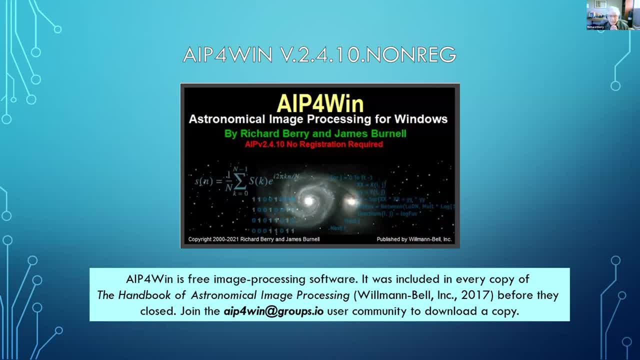 and less time in his life. um, i didn't have enough time to keep up all of the stuff that i worked at. it should have been done. then, of course, after, after your house burns down- you don't have- you're doing things like we're buying chairs and beds and realizing you don't own any books. 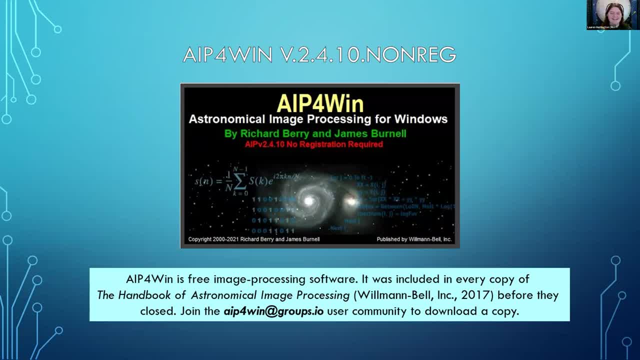 anymore at all, oh man. so yeah, you don't want to do this in your life. if you, if you want to simplify your life, burning down your house, does not do it. but, as you can see, i now have a, a nice office, and over there in the corner is my ev? scope, which, for quite some time, was the. 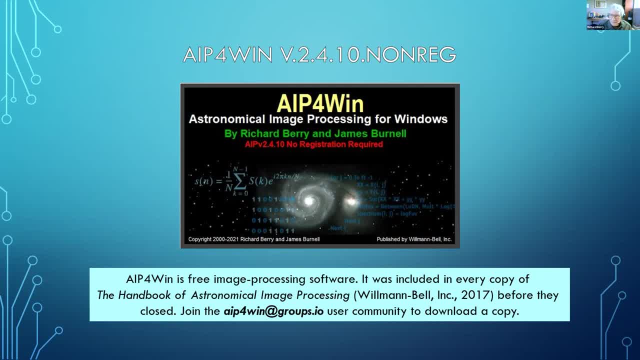 only telescope i had, because all my other ones burned up. oh no gosh, i can't even imagine um you get to do some interesting things with with um, the insurance company, because you have to list everything that burned up. oh, wow, yeah, yeah, what do you do? 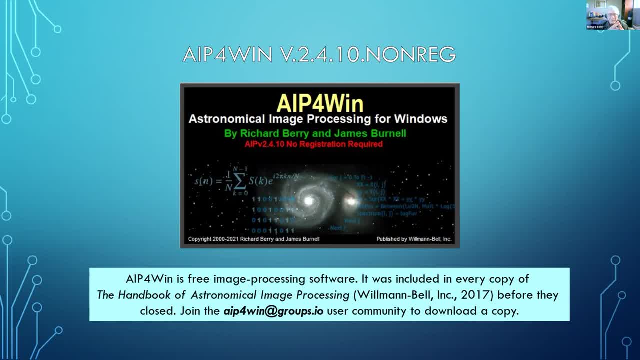 uh, i, i had some interesting negotiations with the, the people because the the insurance people, because i said, well, you know, i have about. i had about four huge library style book cases covered with books and they were famous. them are big academic books and you know, this is the kind of book that costs between 60 and 120. 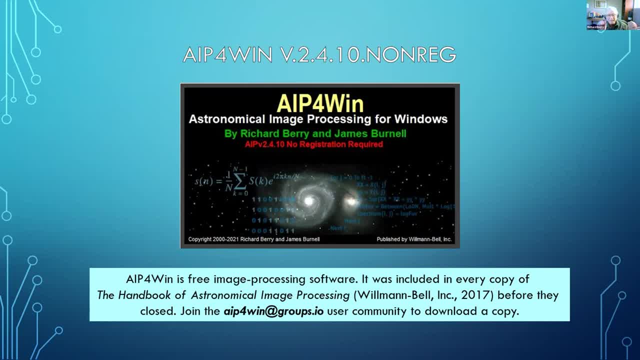 120 and we agreed to make it simple to compute that. um, we would. we would put a value of like 500 on each shelf foot of books. we just calculated shelf feet so i didn't have to give all the titles. but yeah, it's crazy, yeah, for sure, wow. 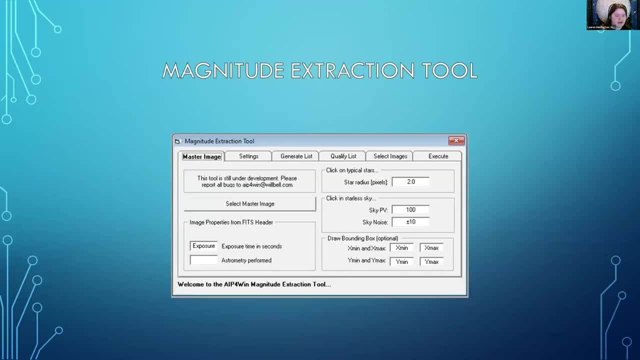 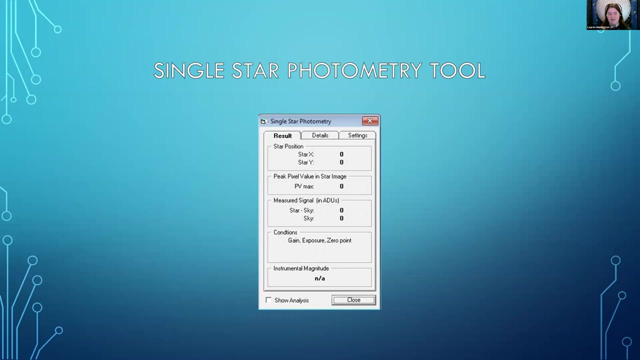 okay, um, so our our next question. actually, we have um two questions here which are related to something you were talking about earlier: the uh zero point. um. first, we had a question asking if you could say why is the zero point in the magnitude equation uh important and 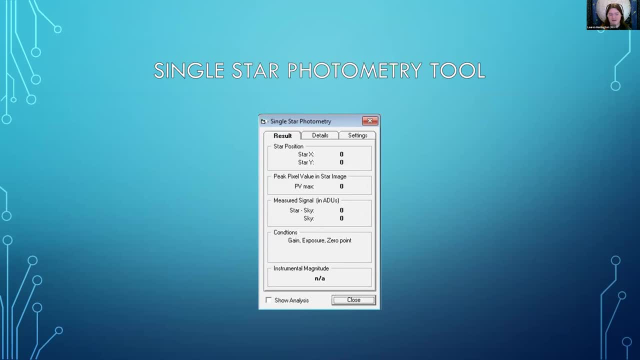 the other question asked: if you don't set the zero point, then does aip for win just use a fixed zero point for each frame? it uses a default value of 25, i think, um, and 25 for back when we wrote the software, 25 gave you something that was within. 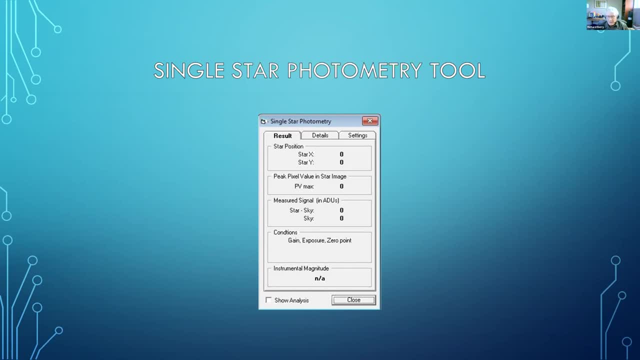 typically within a magnitude or so of of of the right answer. can we use a fixed zero point or is it about the same as the zero point and the error is? is it about the same as the zero point or is it the right answer? it's very important to understand that magnitudes. 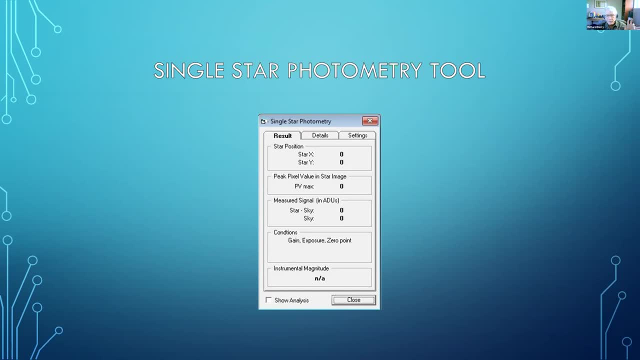 um, magnitudes are always comparisons between a standard in the sky and your unknown, okay, and all we do, all all zero, cranking it down to something which is realistic. Now, as they've developed the science, there's a number of different ways of doing magnitudes. 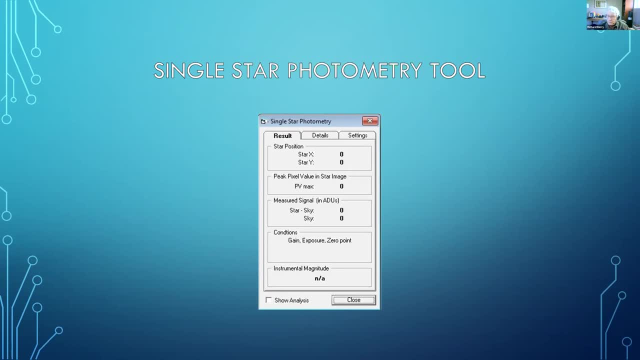 And if you want to, if you want to get really confused, you can go. you can Google how are magnitudes determined and then look for the more the university level lecture series. You'll find PowerPoints out there describing Vega mags and AB mags and different magnitude systems. 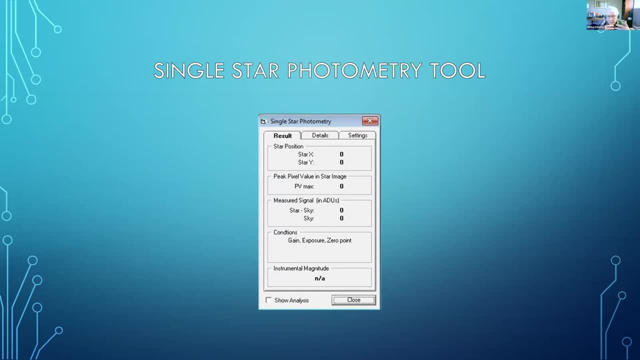 And they're all based on a standard or a group of standards. in the AVSO universe We use magnitudes in the Landolt system, where Arlo Landolt, who passed away recently, determined not sure how many. there are something like 60 standard fields. 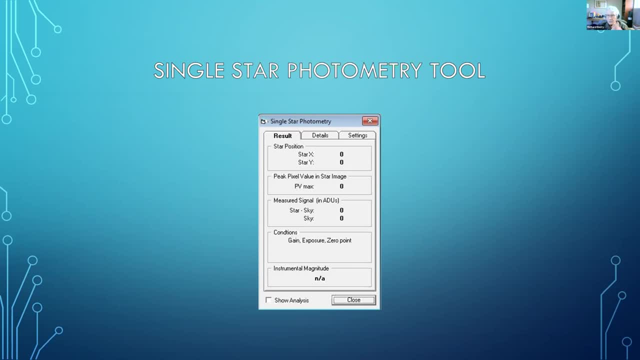 located around the the celestial equator. Each one of these things has a bunch of stars. Those stars were very carefully and meticulously standardized against the master list of ten stars that were used to standardize the Johnson Cousins UBV system. Okay, it was originally the Johnson system. 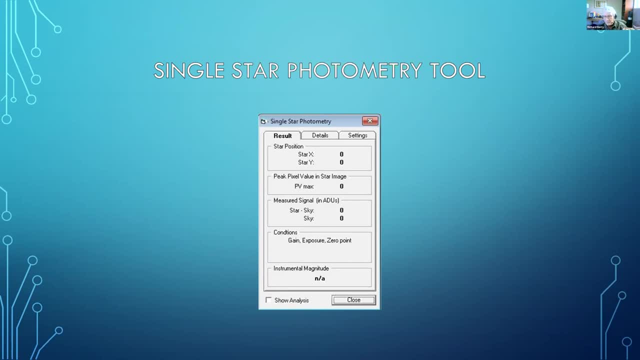 and it was expanded to Johnson Cousins And they added the R and the I filters. So the Landolt fields are your primary. Well, they're actually secondary standards, but people use them as as the primary standards. So if you want to calibrate your data, 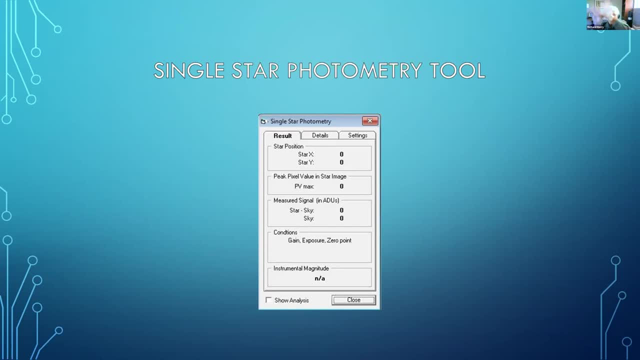 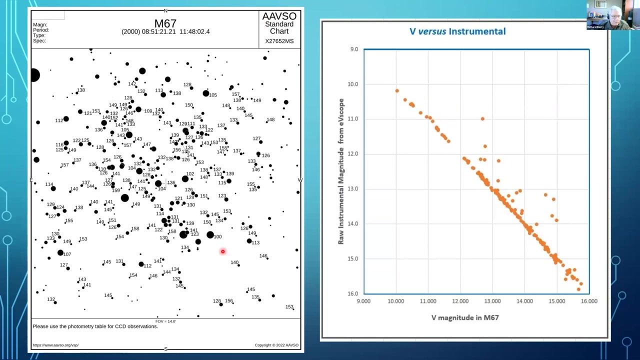 calibrate your system. you go and you do photometry on Landolt fields and you get to, and then we have things like M67.. Let me, oops, Yeah, here's, here's OK, And this is. this is a standard chart- M67. 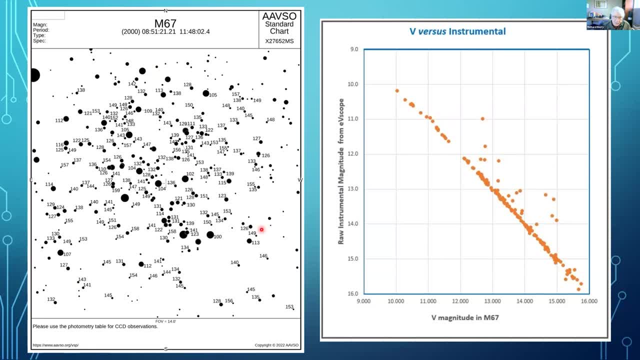 I hope it's big enough for people to see, but a lot of stars and there's a visual magnetism And you can get a magnitude or a star number for each one of those And then there's a list of there's about 250 stars there. 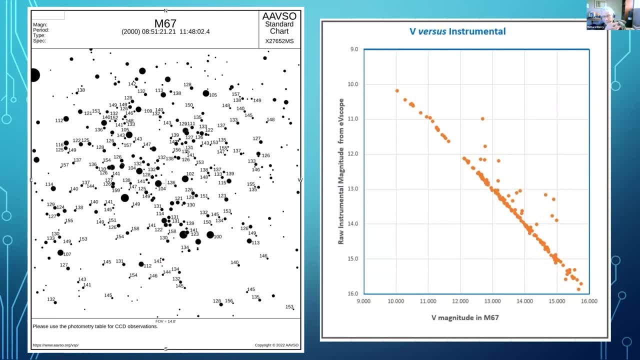 And you can get UBVRI magnitudes for every one of those stars. Those have been meticulously done And that's how I plotted this when I wanted to check. So M67 is now, you know, near the meridian And at midnight now. 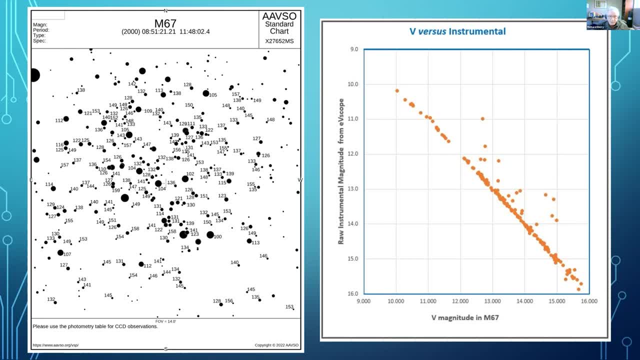 So you know, shoot a picture of M67 or a bunch of pictures of M67.. Get the standard chart and you know, start doing, start Figuring out how photometry works with standards. Now what the chart team does at AAVSO. 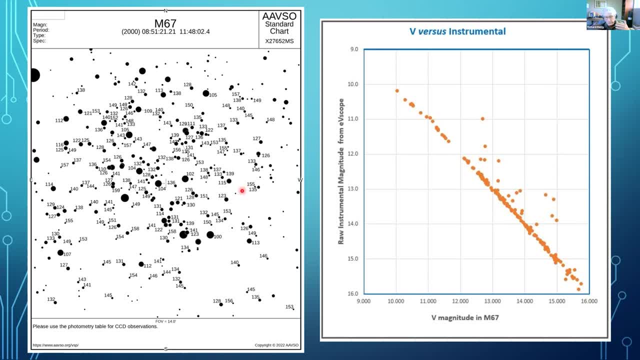 is that they go to the field of your, of your star. you want a photometer and they've created, they've standardized comp stars. OK, so your field will have comp stars in it that have been carefully standardized against Landolt standards and standards like this. 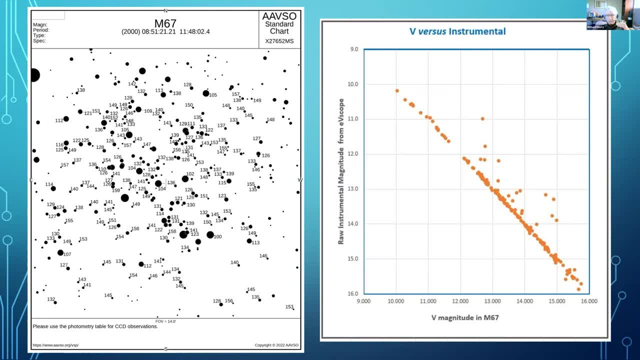 OK, so your comp stars are basically an extension of the standard magnitude system, But you know there's a lot of work that goes into into this, And so we've got the chart And then Arnie Hendon's APAS thing where he photometer the entire sky. it was an AAVSO project- typically to about 20 milli mags accuracy. 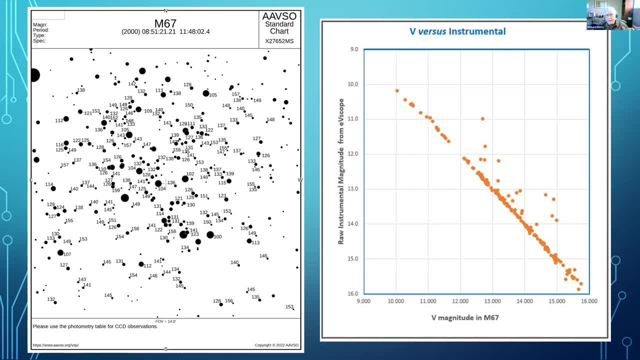 And APAS. I think the whole database is available online. I'm not, I'm not sure. But basically you can get And then what you can do is you on the AAVSO website. I can't give you a link. 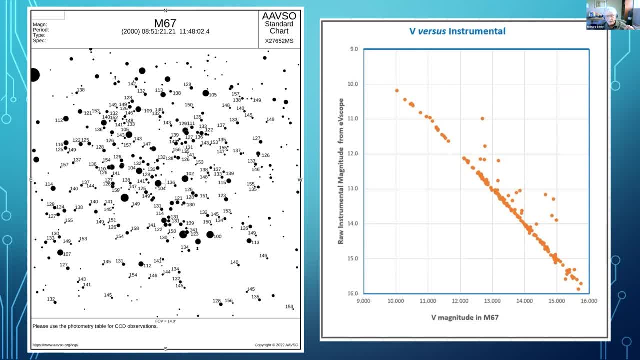 but you can ask for all the APAS stars within a given distance of any spot on the sky And there's a few tiny holes, It will give you back the magnitudes that their system has determined. That's a great resource, Good to know. 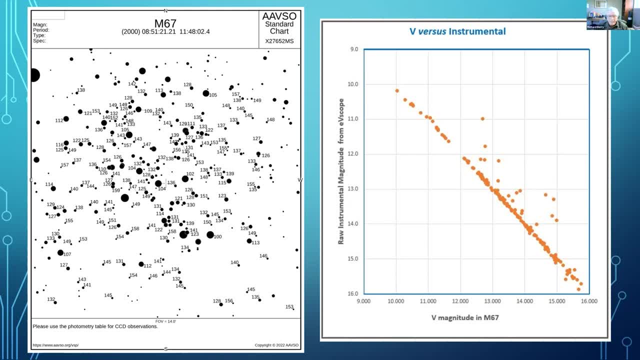 Thank you. AAVSO website has many, many secrets hidden away. Not the world's best interface, And if you can find them, there is really good stuff there. You do have to search. The biggest problem, I think with the website is you have to know what you're looking for before you can search for it. 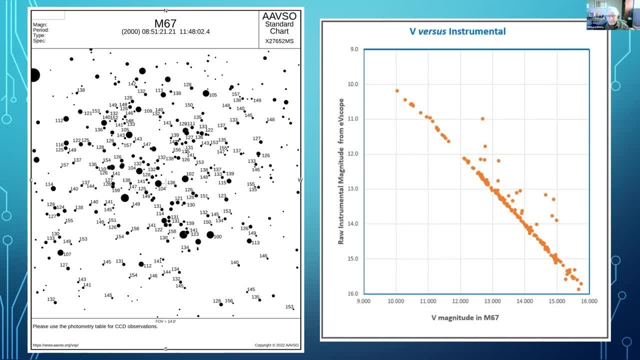 Yeah, OK, if you know what you're looking for, you can find it. If you don't know what you're looking for, you can't figure out what the keyword is. Yeah, Yeah, We've been discussing better ways to structure it. 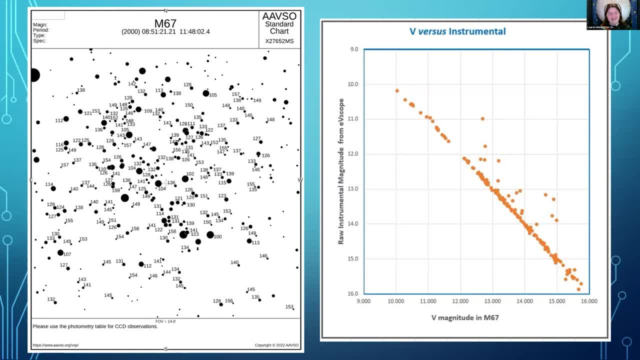 but it's because there's so much good stuff on the website. it's going to have to be a big effort. You know it's a. it's a huge. it's a huge job either. It is a very, very rich resource, Yeah. 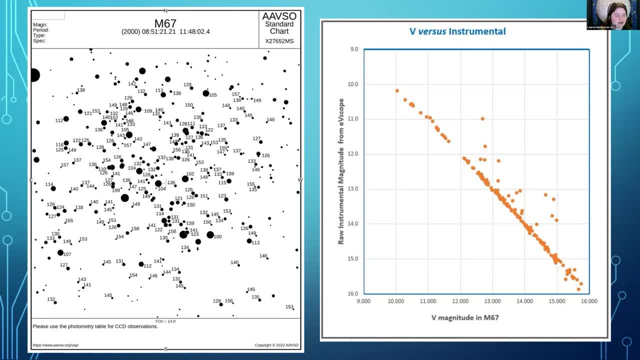 OK, next question here This one comes from. actually, multiple attendees have asked about this one. The basic Question is: since there's been a change up in the availability of photometric filters and the new ones have slightly different spectral responses, do you know if the AVSO has published any information about how suitable 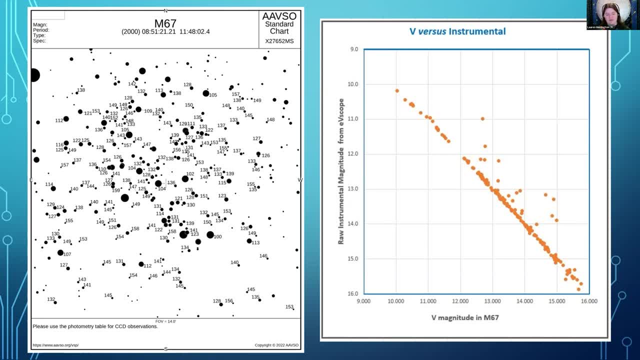 these filters are and can. can we use these new filters for photometry? The answer is complicated. I've been Involved with some of the discussion groups about this stuff And basically COVID slowed down and complicated Everything with with getting filters, The classic Bessel filters which are made by 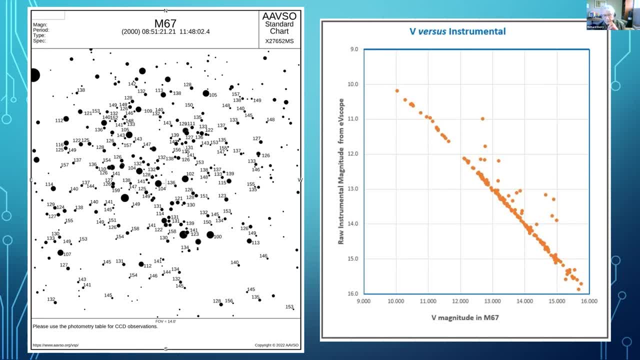 dyed glass Are complicated and labor intensive and I suspect- but I don't know it for a fact- that it became hard to get those types of glass from Corning and Schott. This is specialty, specialty stuff And I've made filters using this. 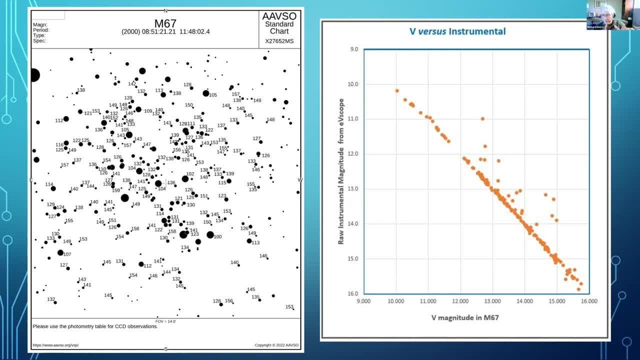 You have to. the raw blanks that come from the companies that make them are not flat, OK. so first you have to put them in a polishing machine and polish The surface is flat, Then they have to be Right. If you want a circular filter, a square filter, it has to be cut, size the edges. 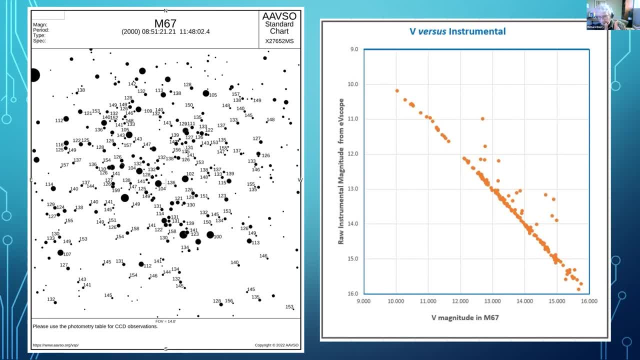 Then they have to put it in a coating machine, probably, and get it clean. Then, because they're round, you have to cut them out with abrasive and then you have to assemble them into a little filter and glue them together and stuff They, However, interference filters, which you I mean in the simple way they put the. they put the, the, the substrate glass, into a machine. series of coatings are put on to it according to a formula and then the interference filter has the right spectral shape. 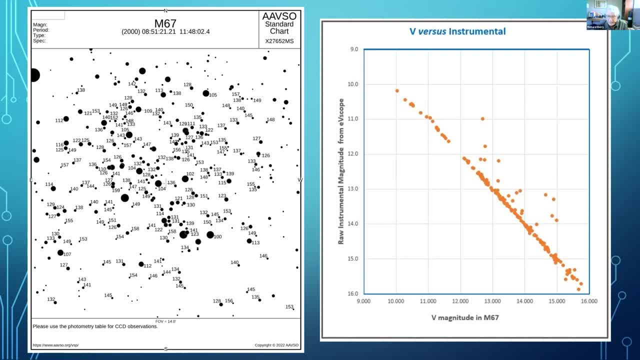 Again, that stuff was probably delayed. A because everybody wants to buy narrow band filters- OK, for for pretty picture photometry, and Only a fairly small number of people are looking for filters for doing photometry. So you know, if you're a manufacturer and you have a choice between making something that a lot of people want, making something a few people, you make the stuff that people. OK, but they are. 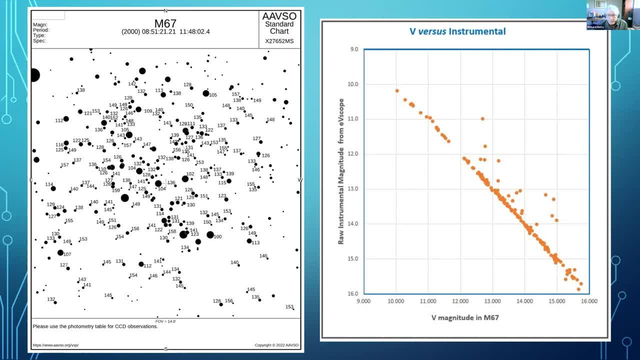 The companies are become very, very serious now about picking up, now that the COVID era is looking like it's ramping down, And I know that at least one company, and probably many companies, Are Working on getting their Formulas made so that the 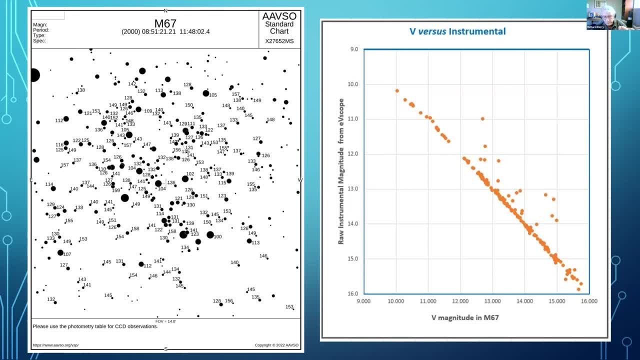 Half band shape of the interference filters match The classic glass dyed glass filter profiles. And the reason is not that you don't get good photometry OK with the the. the argument is that the, The It's- let's put it this way- it's. 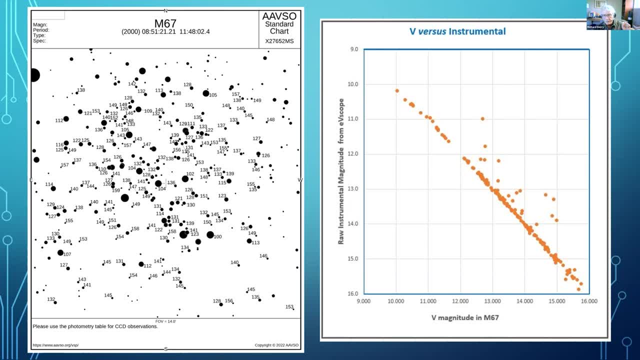 The people that make these filters are very good at making what are called bandpass filters. that is, they present, Transmit nothing. Then the filter comes on, they transmit as close to 100 percent, then they're flat topped and they come back down again to have a 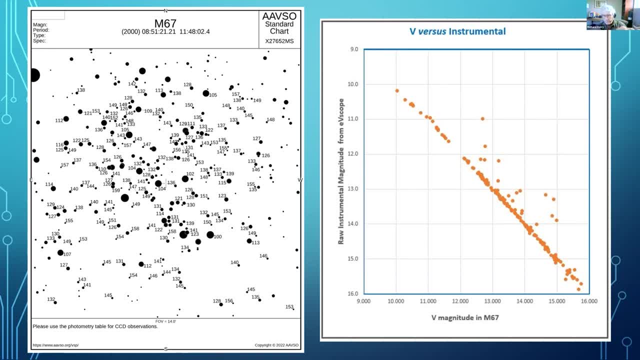 Transmission band which is sharply defined and for almost every technical purpose. This is what people who buy filters want, Accepting astronomers and astronomers want in order to maximize the value of, you know, 75 years of Photometry done with Dye glass filters which have these sloppy bandpasses. 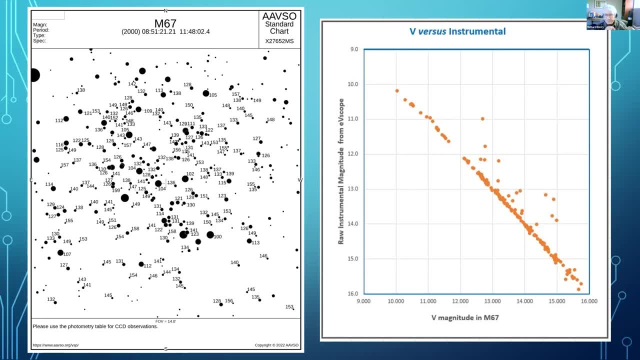 They can make them, But you have to. It's only now that they're beginning to realize that It's critical that the photometry we do now matches the photometry has been done for the last 75 years, So we're in a transition period. 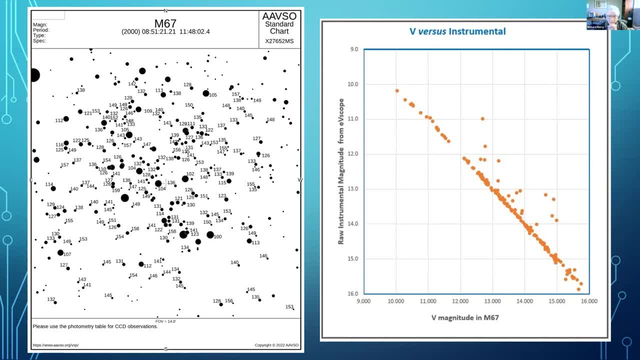 I expect Expecting Okay. the other thing is that photometry done with the square filters can be transformed Into the standard system, but it's an extra step. Okay, now, ideally Okay, because The bandpasses is right, it's centered on the right thing and it's it's, but it's, it's shape is different. 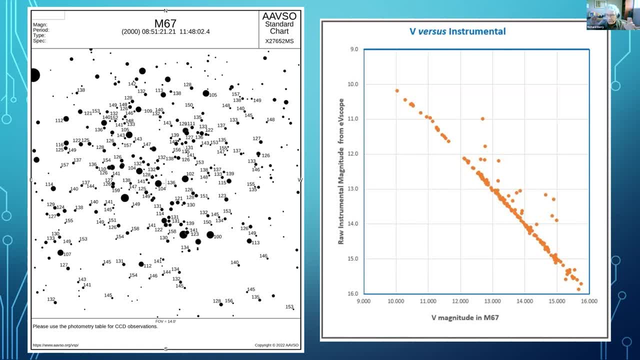 And for a Nice ordinary sun type star you're going to get the same result basically with the, With the, The die glass, the filter and the square bandpass the filter, If the stars really really read. Okay, I remember be minus fee for red stars. every key mobile magnitudes. 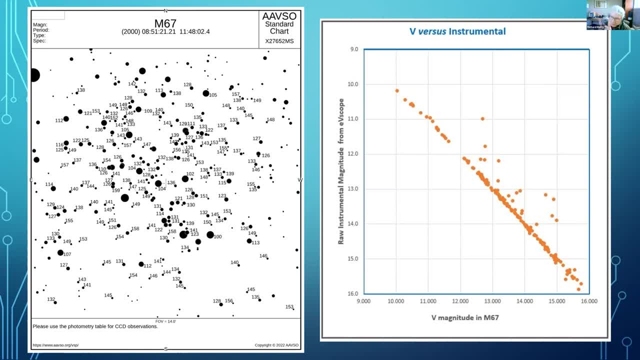 Then this sloppy bandpass is going to pick Up extra red light at this end and your star is going to come out too bright. Okay, but if you know the color of the star, you can then transform by applying a small correction that takes that extra bit out. and that's what transformation does: it takes the raw results you get with your instrumental filters and 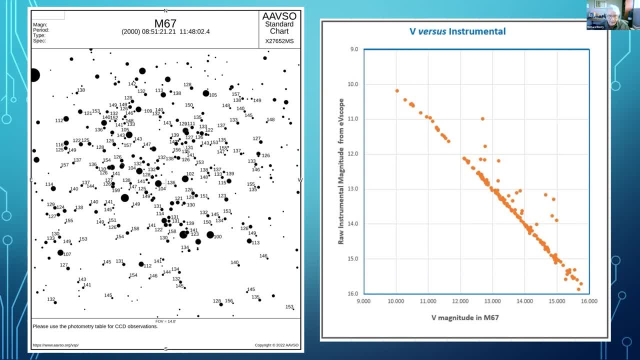 force fits it back to being standard things. And again, what you do Then is you take your filters and you do photometry on object, like i'm 67. And then you run this through the right math and it says: oh, list star comes out your. 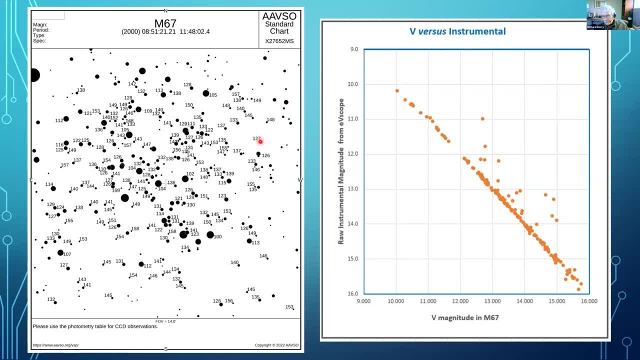 You be your bv. our magnitudes can be crunched over by applying this math to them to produce a standard bv, our filter. There should probably be a webinar on on doing transformation, if there hasn't been already. I have some great news. Yes, we've actually just scheduled a webinar all about doing transformations. that one will be the June- how to our, and Tom calderwood will be the presenter for that. 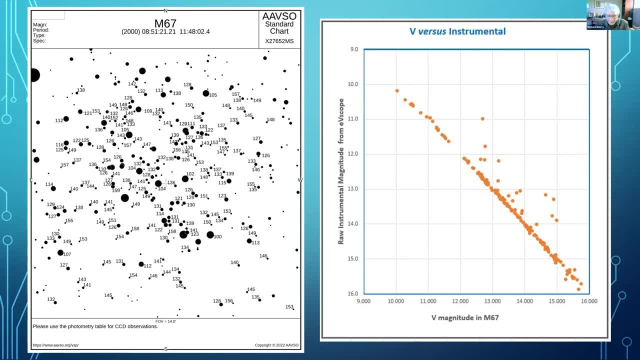 Oh, very good, I know time, he's another Oregonian and The standardization is is the key right now. something like 10% of the people doing submitting photometry are not doing transforms Because you know you have to spend a couple nights figuring out the transform coefficients. 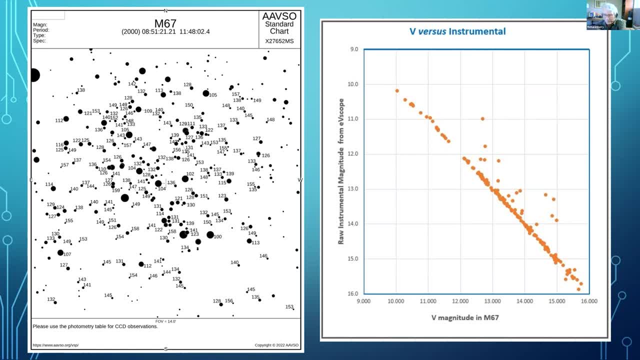 You know you think, oh wait a minute, I only get so many clear nights, I just want to shoot my my stars and send in my results untransformed. So, Tom, I think we'll probably make an excellent plea to learn how to do transformations and do them, because then your, your filter types, become much less critical, because whatever filter you're you're starting with, you should be able to produce standardized results. 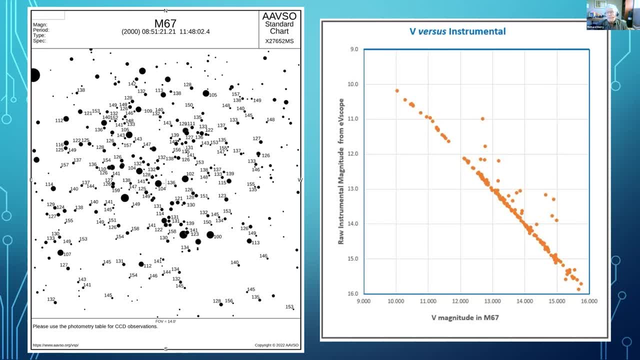 So it will be less, but I think the message is good. Good, new matching filters Are in the pipeline and I think arnie hand and has filters network right now which is testing to verify that they work correctly- Great, okay, so, um, we still have probably about a dozen open questions, but we are now at the two hour mark. want to give you an option on whether you want to try and answer a couple of the last questions or if you want to go ahead and start finding things down. 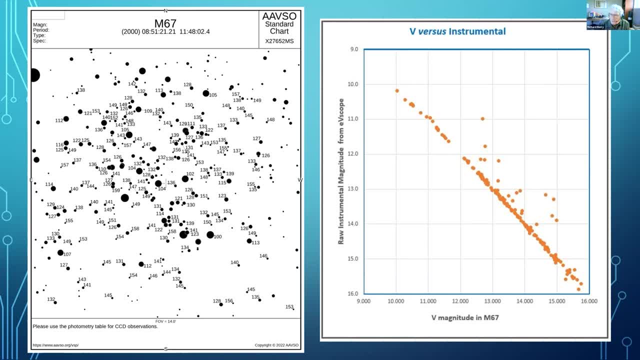 i'm real quick. What kind of questions are they? um, we have Another question about filters. what about the 245 cookbook camera? What about the difference between CCD cameras or CMOS cameras? what about the EV scope? what about astro image J? so it's kind of all over the map here. 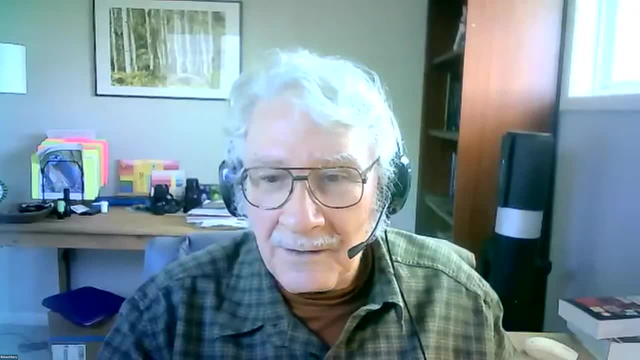 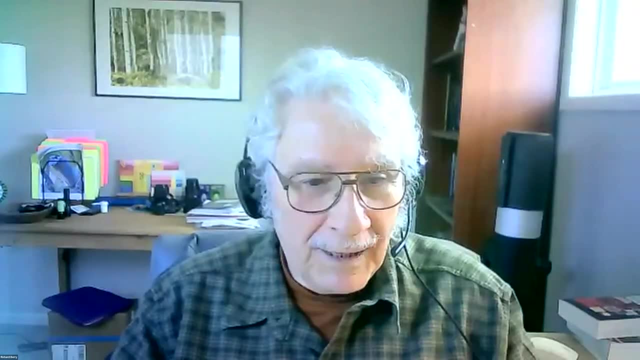 there's like i'm going to stop sharing because it doesn't sound like any of those needs sharing. why don't we try to get pretty quick answers for them? All right, let's round then. yeah, we'll just sort of whip through them and see if we can't. 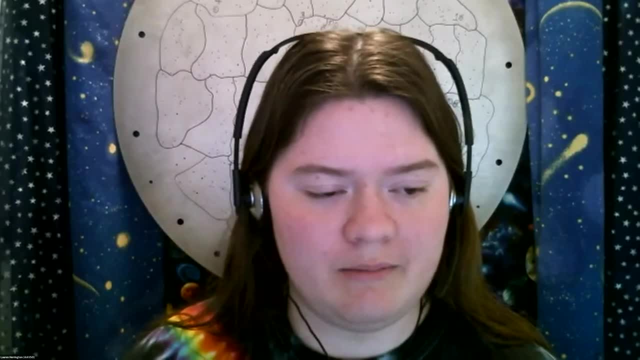 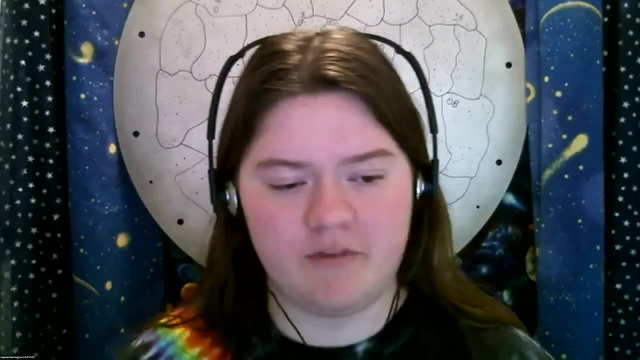 Okay so, um, one quick comment here was submitted by mark but rough, who he had a reference for a paper on transformations from Johnson magnitudes to sloan magnitudes. in case you have the sloan filters, i'm going to copy his comment over to the chat. 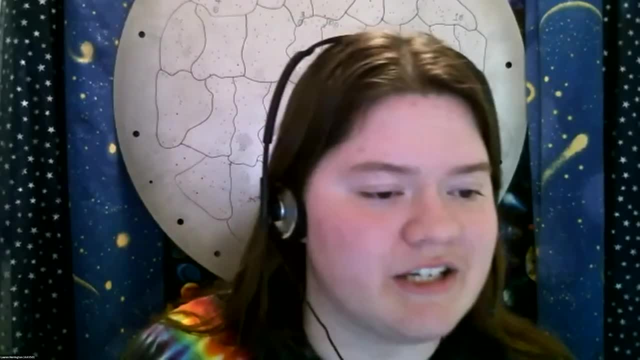 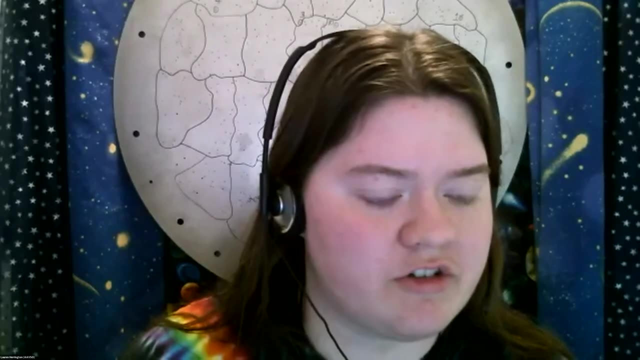 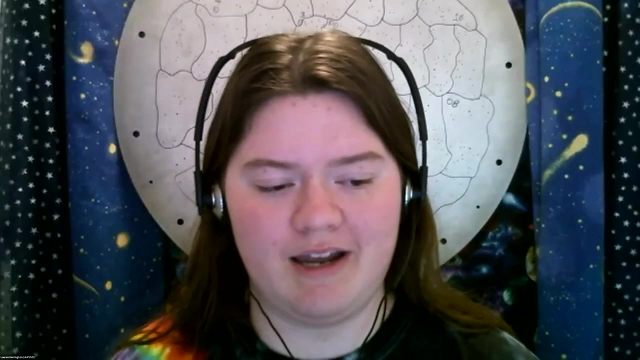 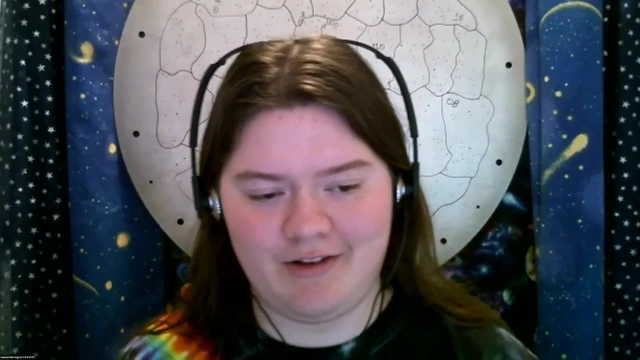 And All right. next question, let's go to. How about George smith's question on how accurate in terms of percentage of intensity, can you measure a stars brightness with amateur quality cameras? He gave an example of a 10th magnitude star with an eight inch F 10 scope and one minute exposure. 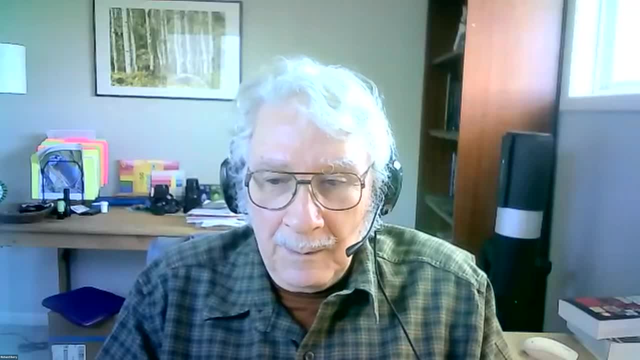 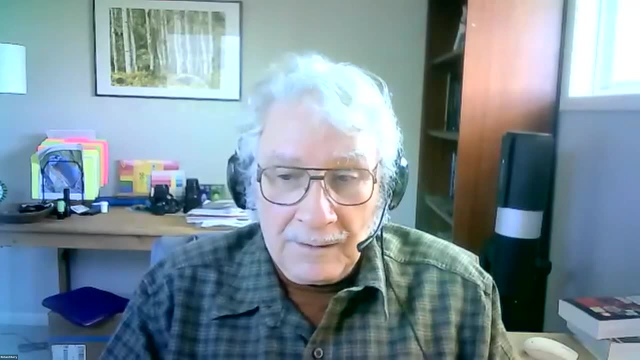 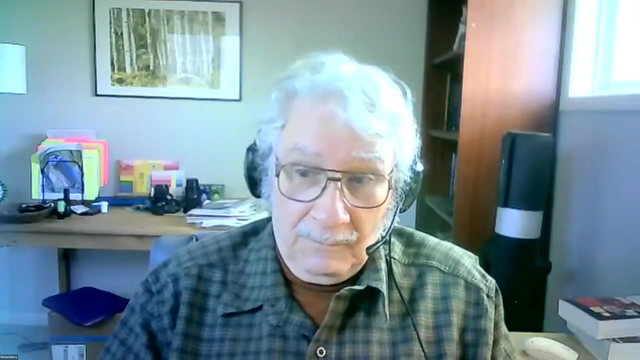 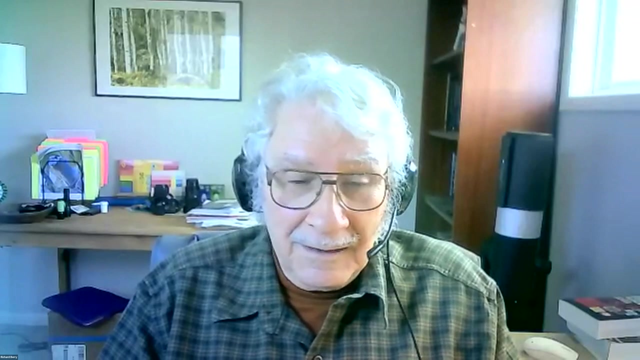 um, You should be able to get some about 5 million X under good conditions. It, you know, any scope is a- is a quite decent sized scope. 10th magnitude star is, You know, today's universe, a really bright star. And, yeah, you should be able to do. 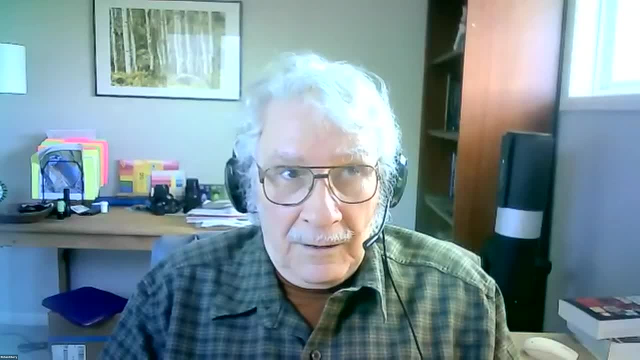 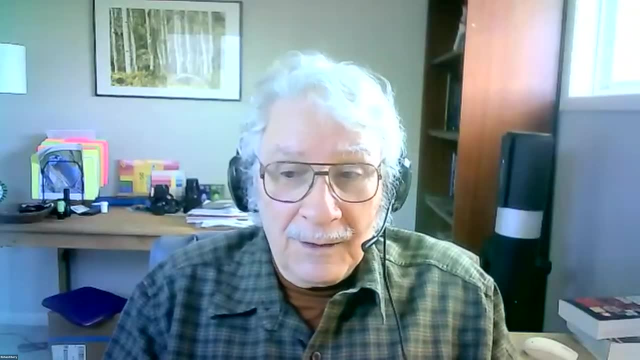 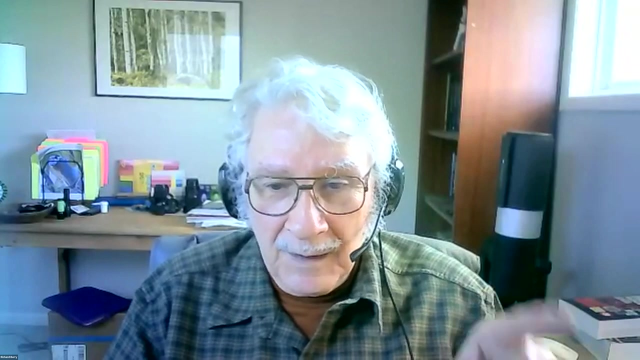 You know um At at that level- let's put it this way you may you're. when you look it up on the photometry table, you'll probably find that the comp stars are given magnitude of like 10, point. you know, 500 plus or minus 20 million bags. 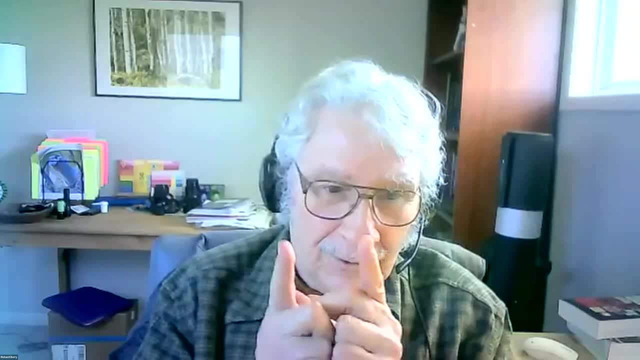 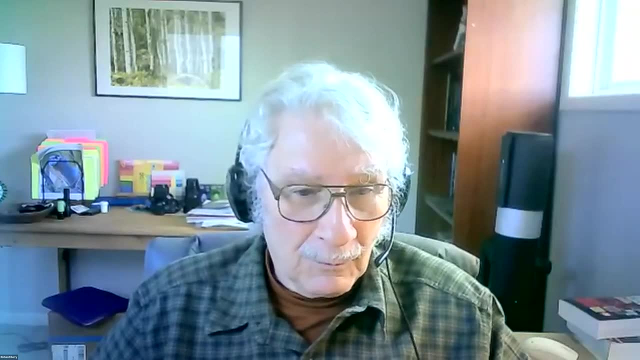 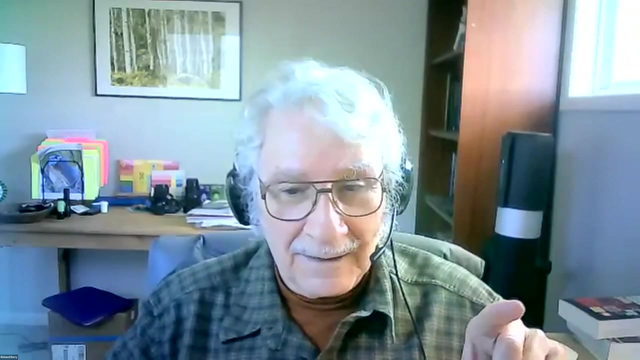 Okay, you may be able to get a differential magnitude that's good to five million bags, But your result is going to be constrained by the fact that you're Comp. stars are not known well. Now, the avso reporting format. When you report that, the, the, that 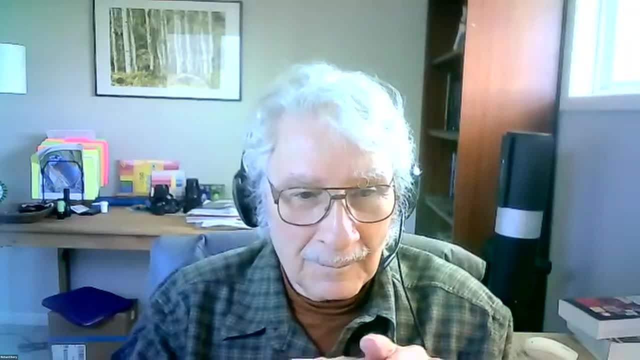 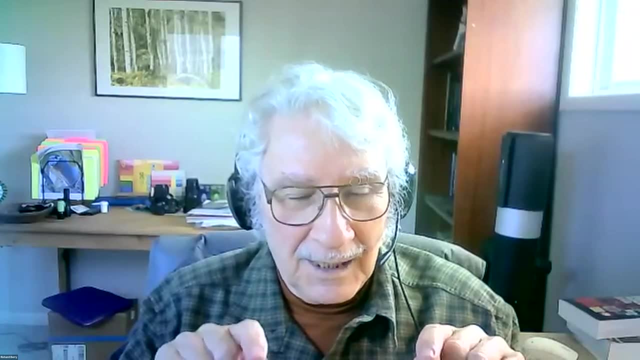 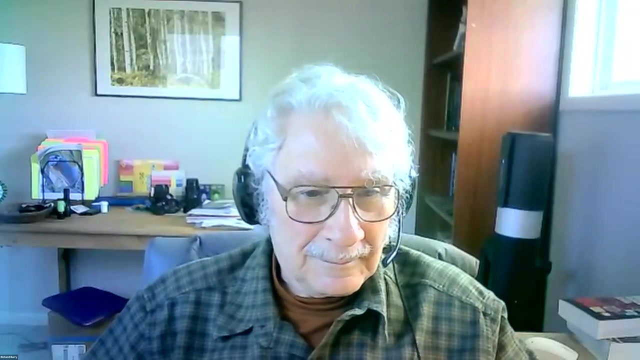 Nine character star number. If we get more accurate values for that, your your data submission can be re computed to be as accurate as the new comp star magnitude is known. Okay, thank you, And we're thinking ahead. when they did that, yeah. 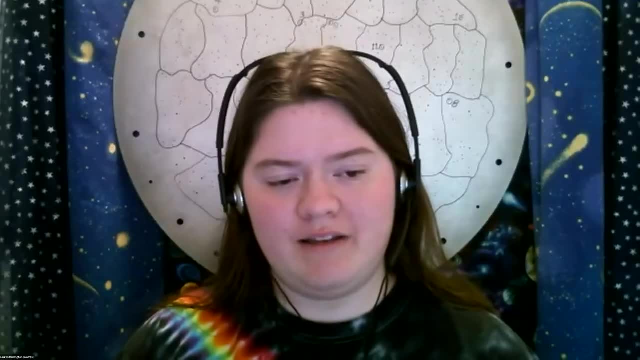 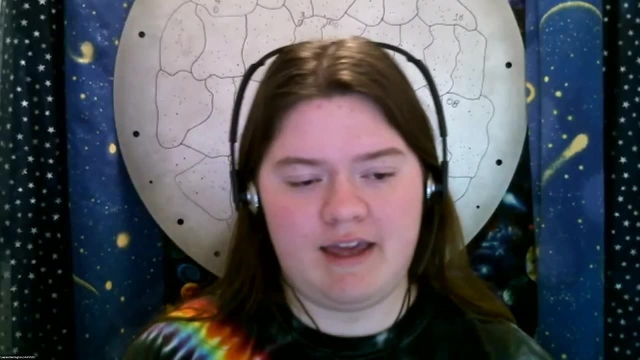 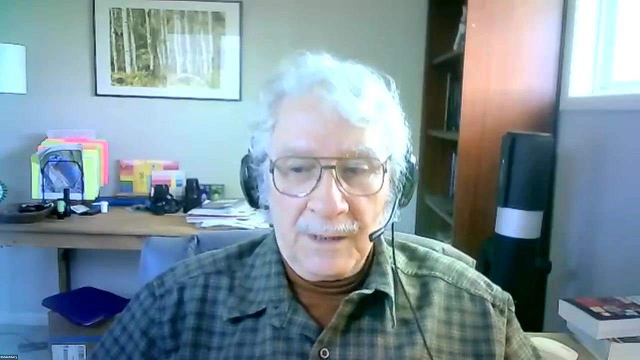 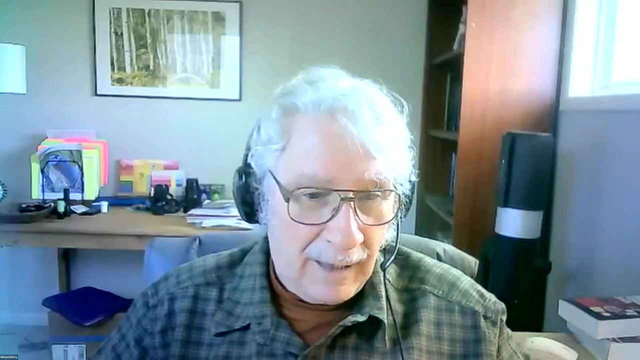 All right. next question here: does a IP for when take the average or the median of the background pixels when it's sampling using the outer annulus? and if it does take the average, does it perform any outlier tests on the pixels? from that It does not perform a test. what it does, it takes the average but then it discards. it basically takes what I call the mean of the median half. 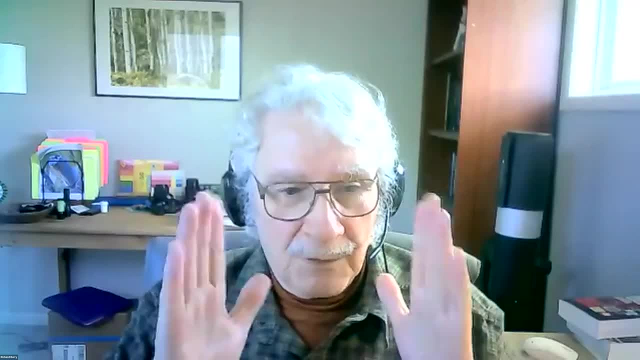 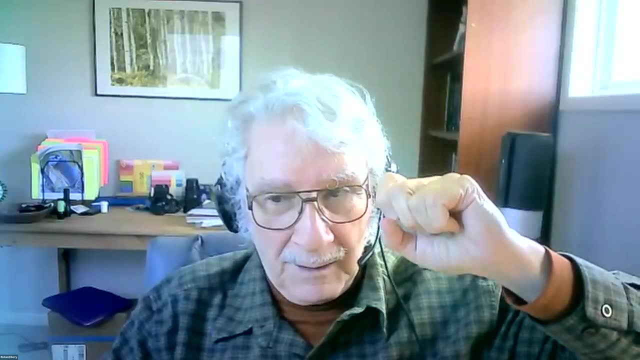 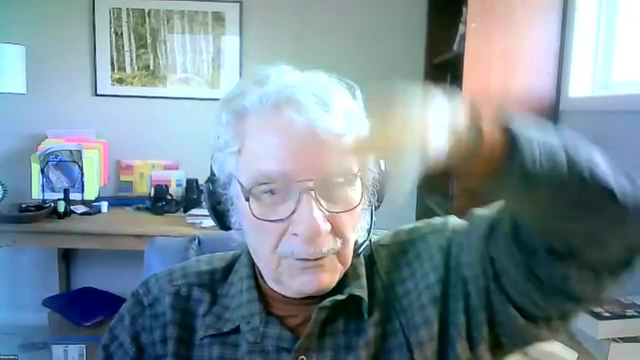 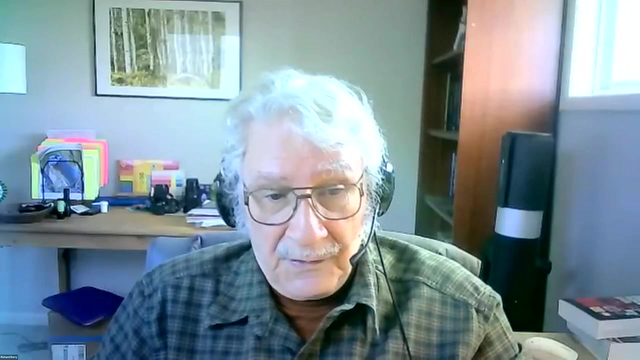 In other words, we take the middle 60% of the stars and we average them. So You may- you might have missed it in the in the- what the software does is sorts them from bright to dim and throws away the brightest, throws away the dimmest and averages the middle one. so it's basically does the same thing as a case Sigma or a median. 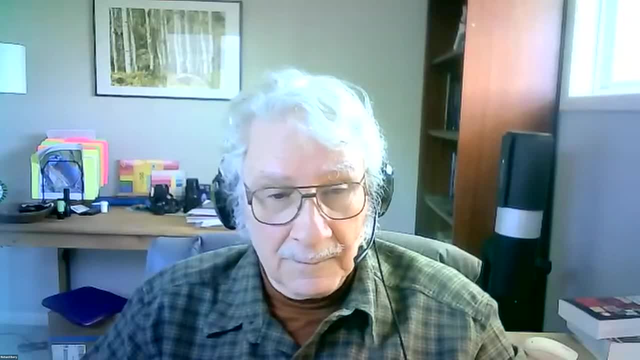 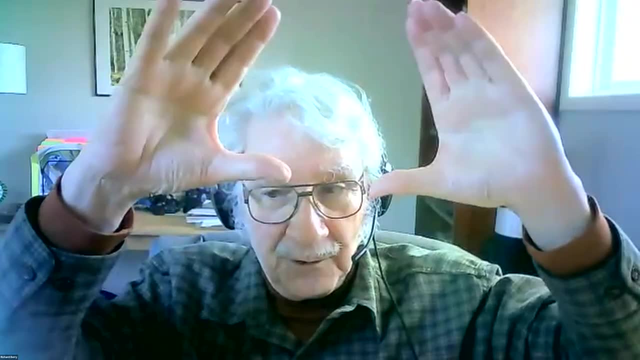 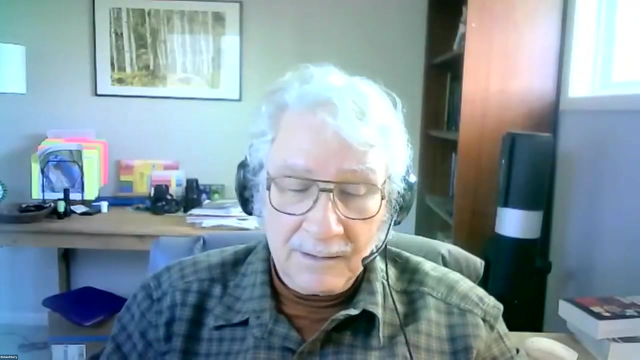 But it's actually more violent because it throws away The top 20%. So if you have a star and pinching on your star that fills more than 20% of that radius, you'll begin to get parasitic light. but it, it, it's, it's actually very efficient. 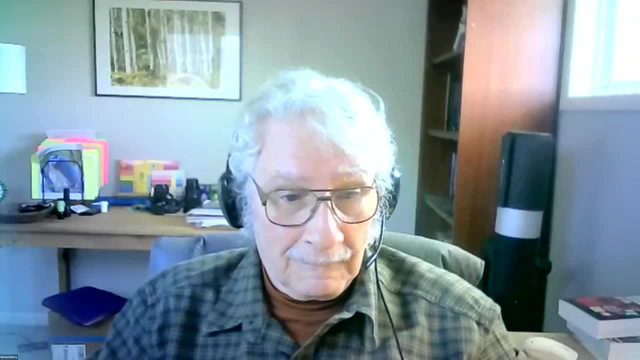 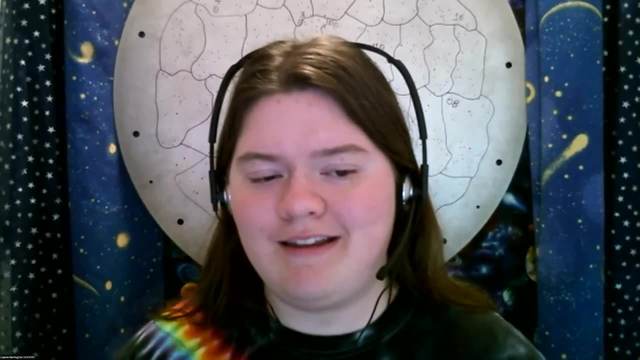 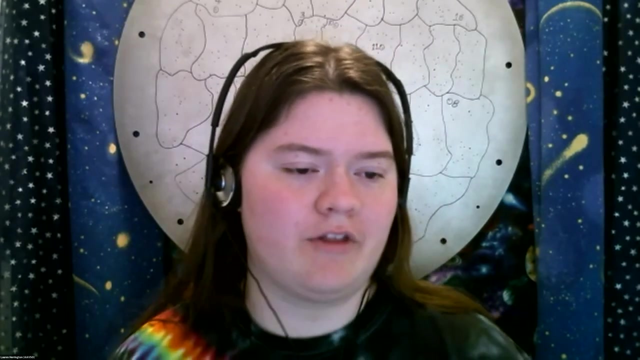 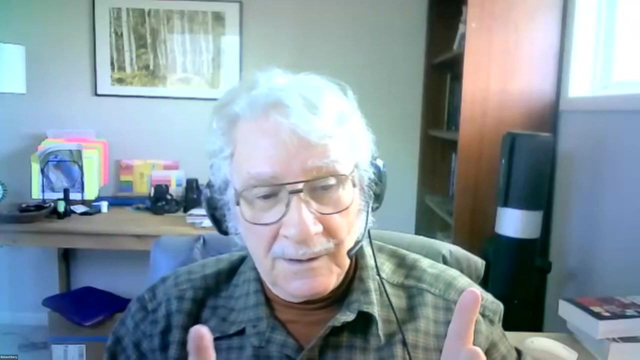 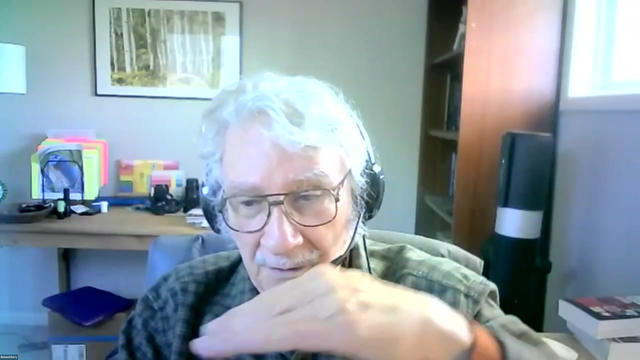 In getting rid of parasitic light nearby stars. Great, good to know. Next question is about: is there a quantitative criteria for deciding how big your photometry annualized should be the radius for the star and the sky background? If you, you, if you use the profile tool and you you can set it, you want to set it so that this star is. 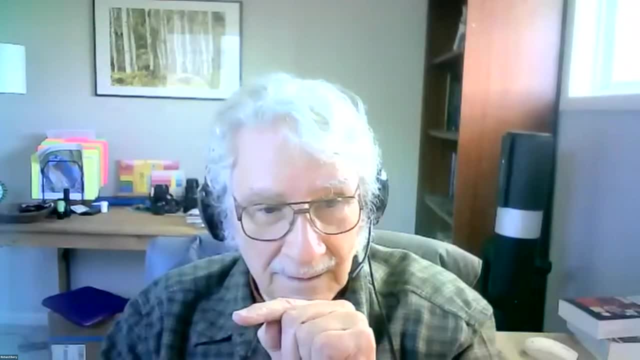 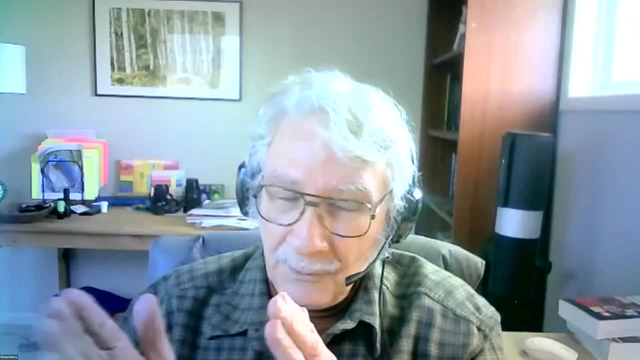 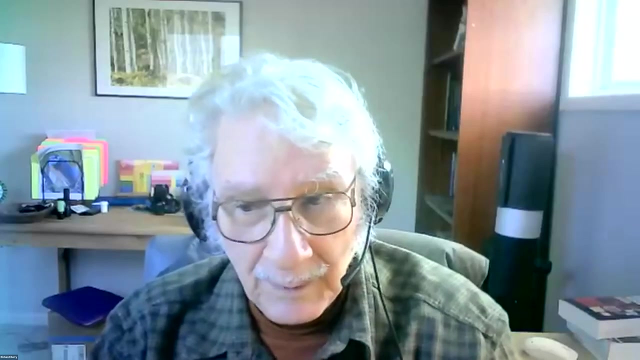 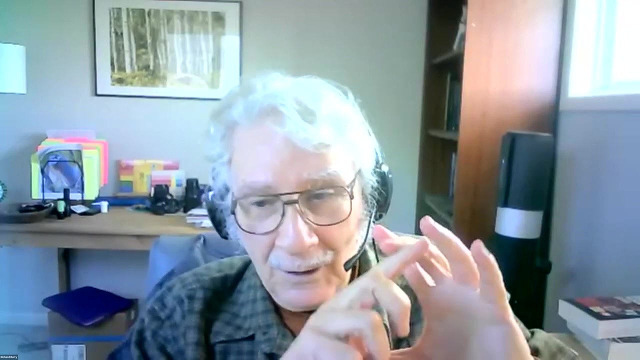 Almost going level but not quite, because your highest signal noise ratio will occur when you're cutting off About 20% of the stars light Interesting. If you go strictly by the highest signal noise ratio, it will make you nervous because you're cutting off more. you're cutting off a bunch of light and you're going like: can I really get away with this? 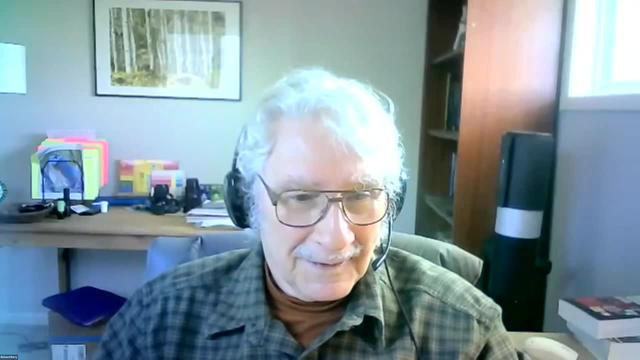 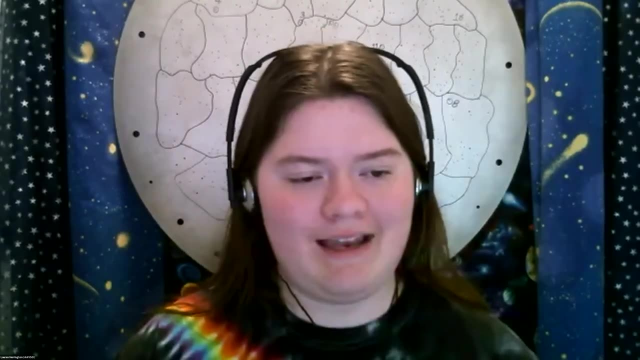 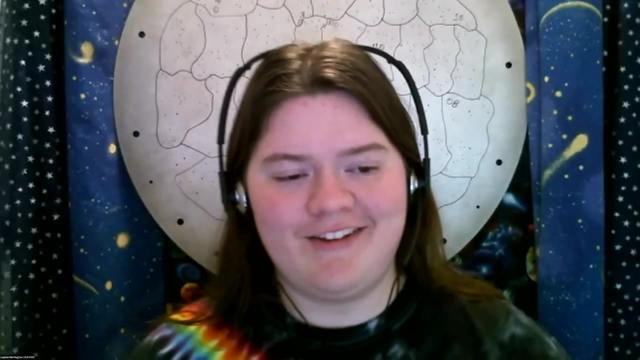 The answer is yes, you can, but it makes me nervous, right, Okay, thank you. Next question: if your cameras gain is 16 electrons per ADU but your camera is a 12 bit, your software saving the images 16 bit. do you need to divide the gain? 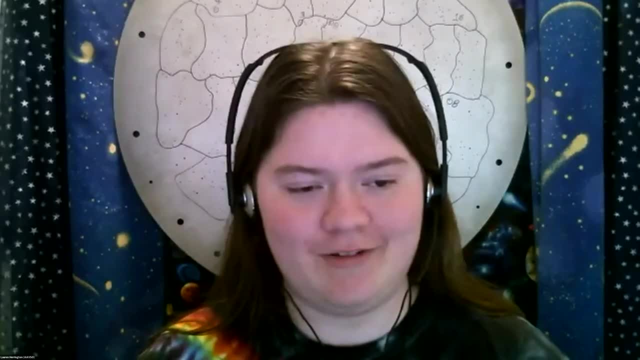 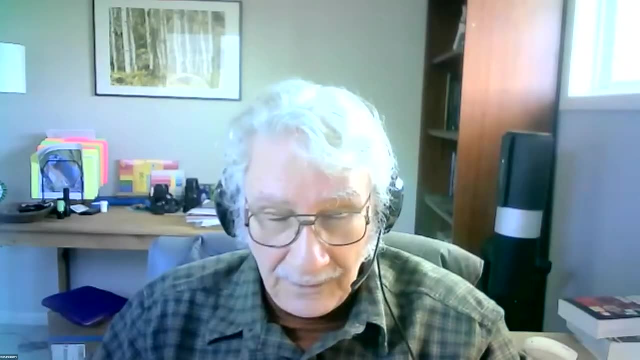 At 12 bits by 16. so that's the conversion from six, 12 to 16 bit, And then just set the input parameter gain at one electron per ADU. I think that's true. yes, Okay, okay, handling questions like this verbally. 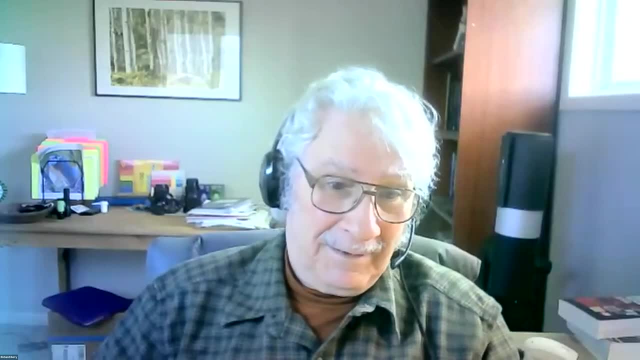 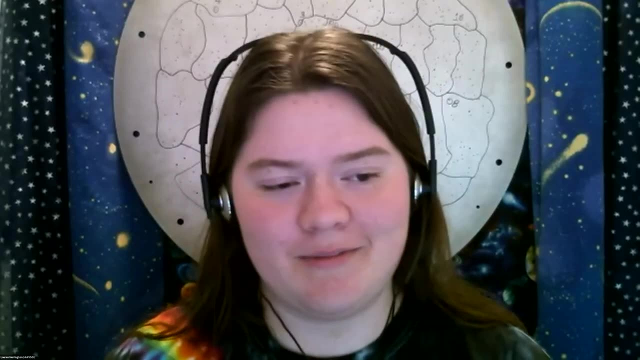 I know it's in the Q&A box. I think he's right, Okay. Okay, thank you. Is there some sort of set procedure? I assume the number 16 and 12 aren't too special there. what's the, what's the goal of that conversion there? 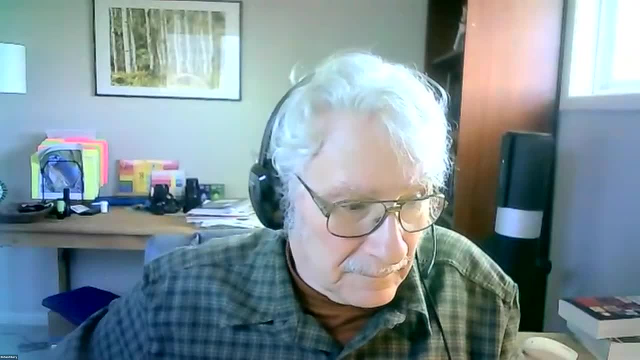 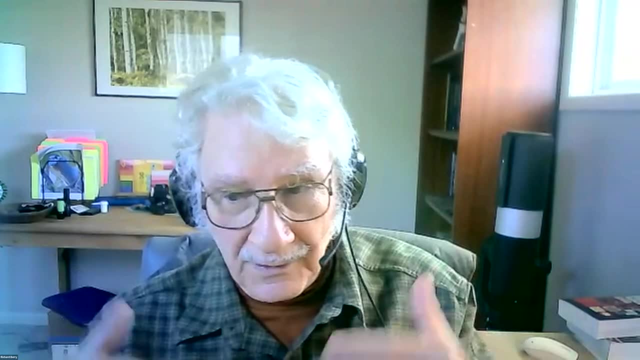 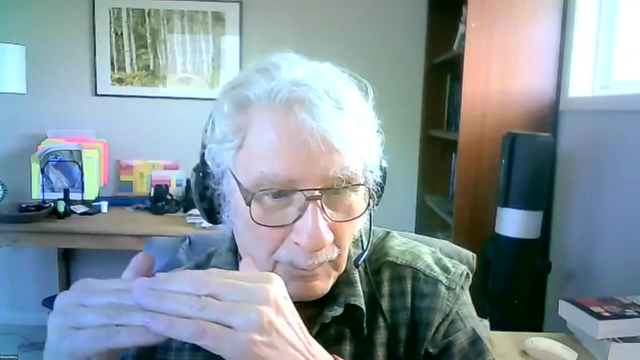 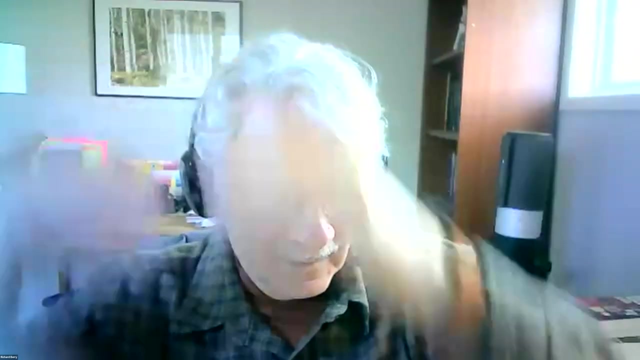 Oh well, The gain is simply the number of electrons in each ADU, When the camera is actually taking 12 bit data. but then you just both play everything by 16 to make it into 16 data. you've you've diluted that by a factor of 16, and 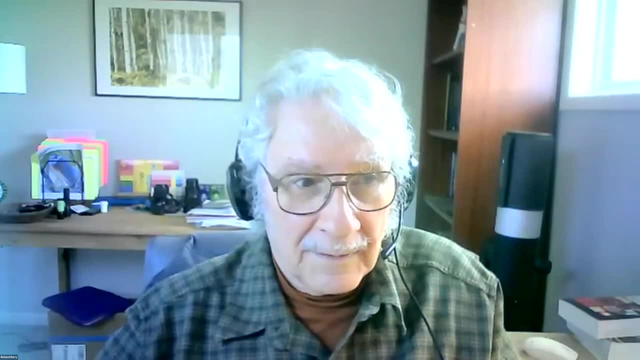 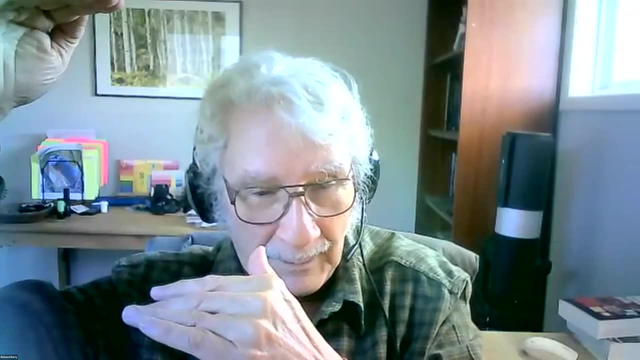 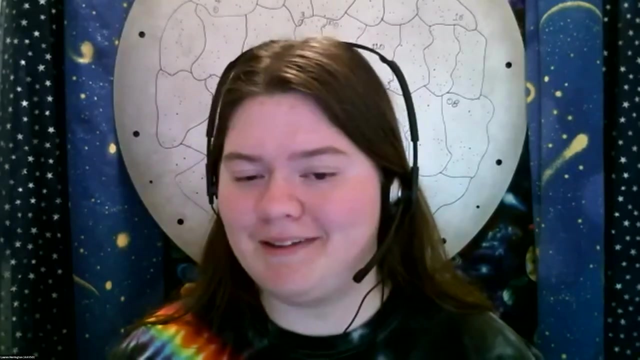 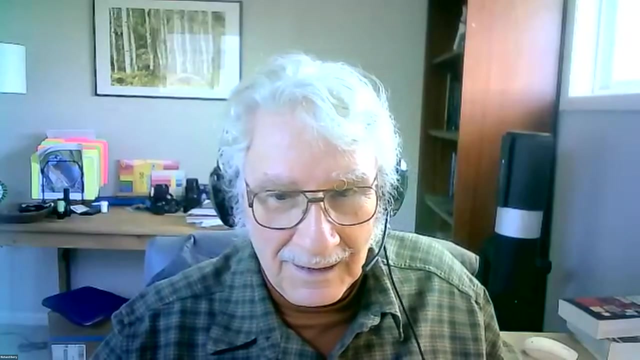 then the number of electrons per ADU would drop. Uh-oh, Can you still hear me, Mr Berry? You froze up. Oh, I'm sorry. Oh, now you're back, Great, Okay. Oh, it says my internet connection is unstable. 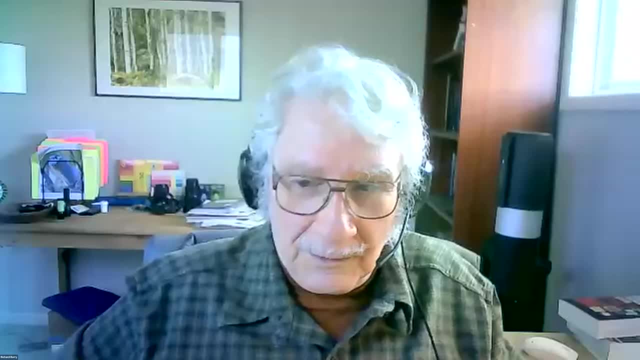 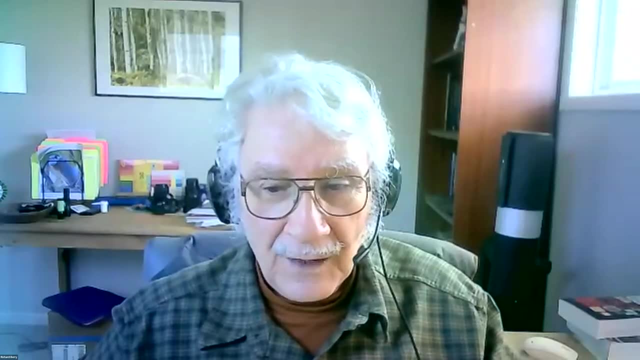 Okay, Well, all the more reason for a blitz round, I guess. Okay, So, so, um, just be If you, as long as you got it. I think he's what he said is correct. I think it's one electron per ADU. 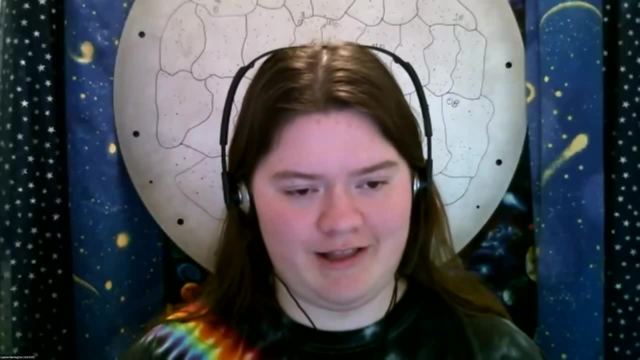 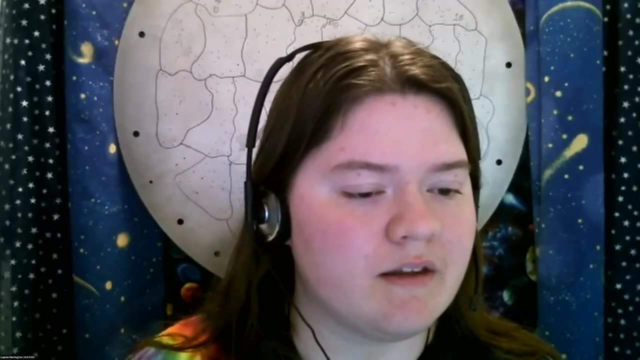 And I understand more now because of what you said about why you're doing that division, Cause you're trying to get back to the one ADU mark, Okay, So, um, next question here. Uh Oh, this one's a little bit ironic, and I'll say why in just a moment. 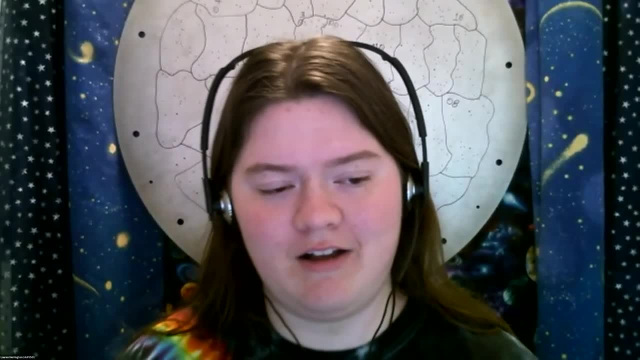 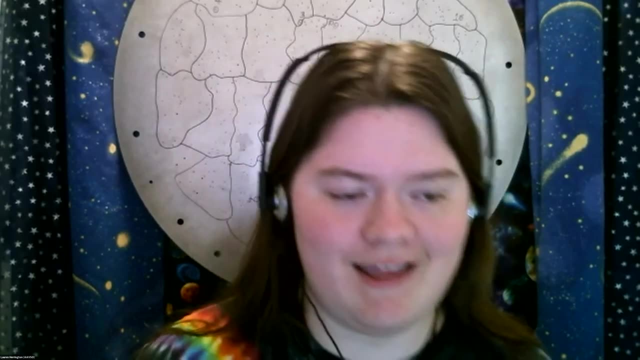 but um, Ron has asked if you can comment on astro image J and its photometric applications for photometry of exoplanets specifically. And um, before you answer that one, I'm going to say the reason I said it was ironic is because it appears. 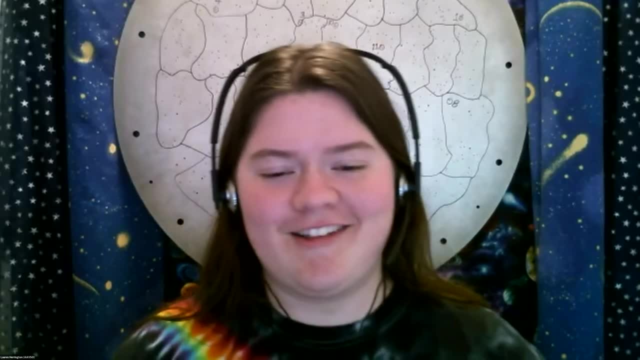 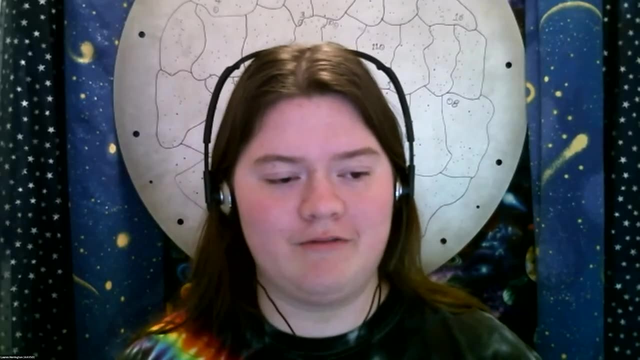 directly above a question from Dennis Conti, who is our resident expert on using astro shape for exoplanet photometry, And he did have a webinar on that last year. So, Ron, I would recommend that you go look at that And then Mr Berry, um. 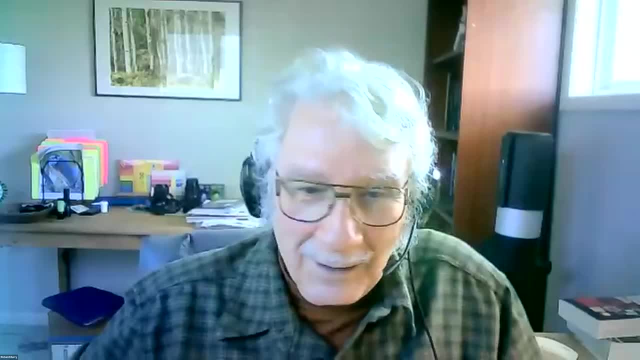 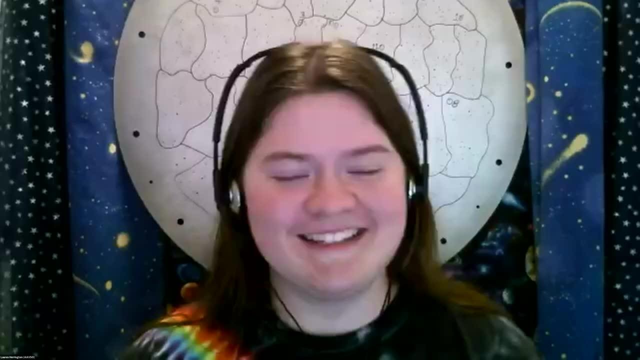 if you want to Add anything, Yeah, Well, I I I know both Ron and and and Dennis, Um, so I could let them Duke it out. Uh, for, for, for, for doing, um, exoplanet stuff. 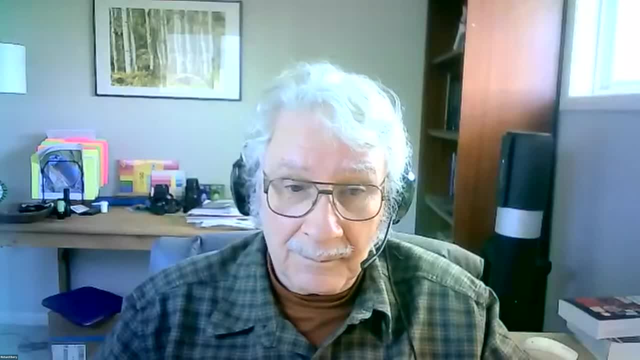 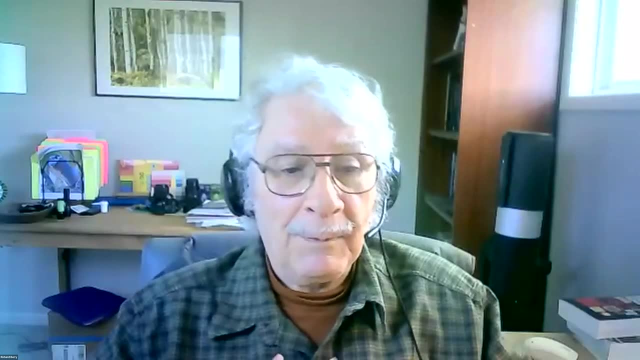 Astro image is a great sore, Uh, great, Um, uh uh. You know it's probably the way to go Because it's so many people are using it as a standard. Um, In terms of putting together this talk, 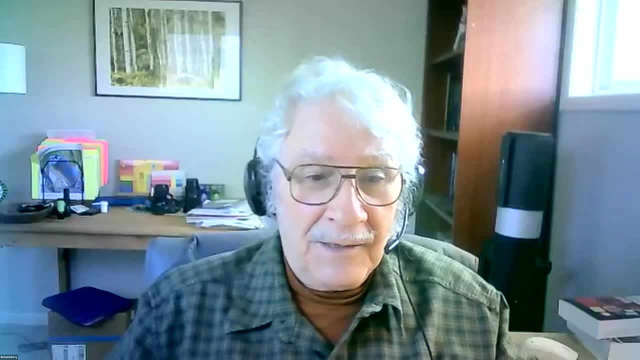 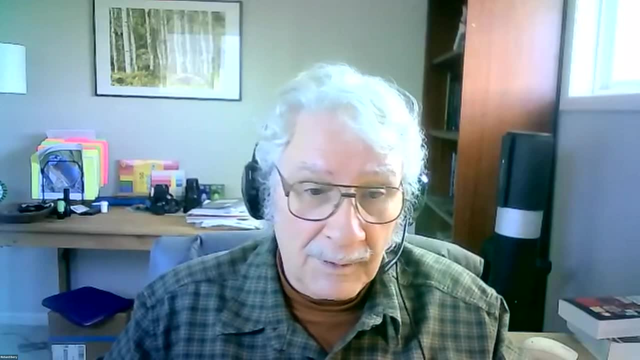 Um, You know, I don't have an inside line on how astro image J does its computations. I think it's, I think it's, I think the code is publicly available. Um, But I wanted to talk about something where I knew exactly how the thing 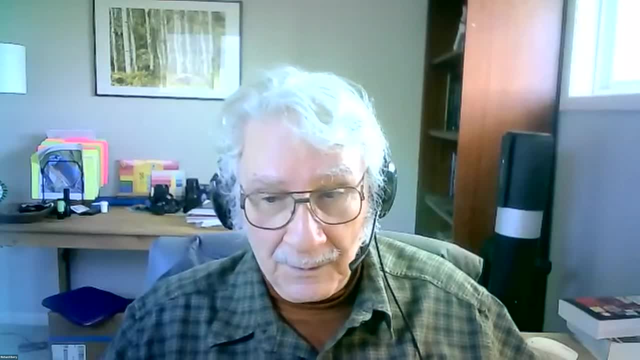 works Right. But as I said at the beginning, You know there's only so many ways to do this. I mean, you're going to have to slice and dice the image certain ways, You're going to have to do certain things. 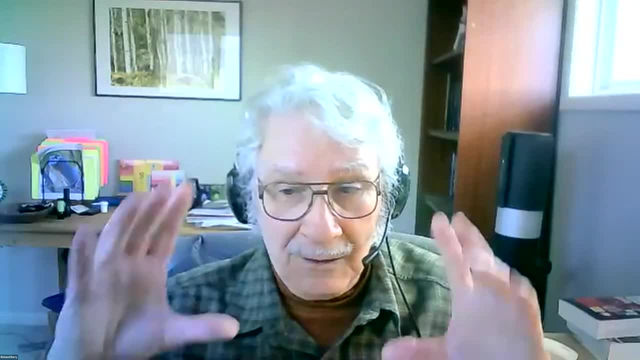 No matter what you're doing, You're going to have to do certain things. You're going to have to do certain things. You're going to have to slice and dice the image certain ways. You're going to have to do certain things. 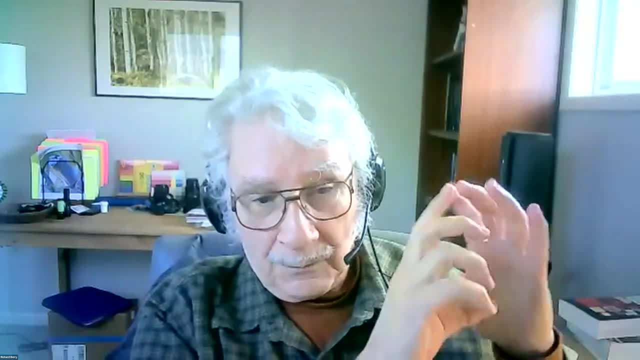 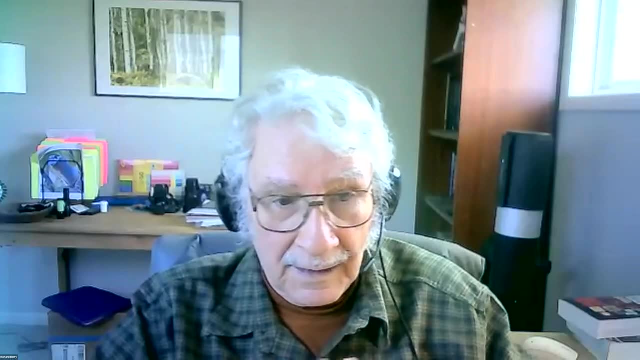 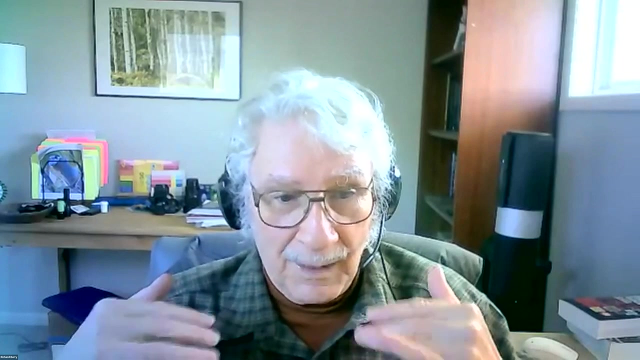 No matter what, you're going to try to Try to capture what's in the central area. You're going to try to accurately handle the sky And you know you can debate from now Until doomsday As to what is the exact best way. 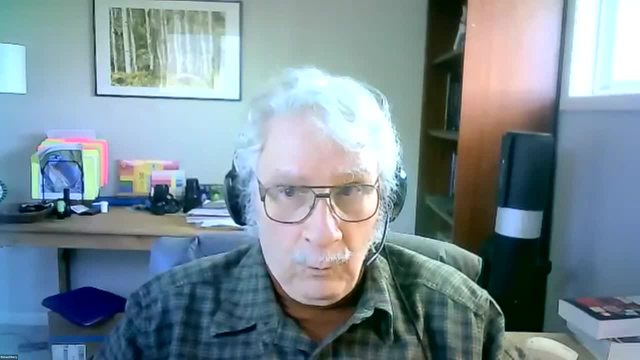 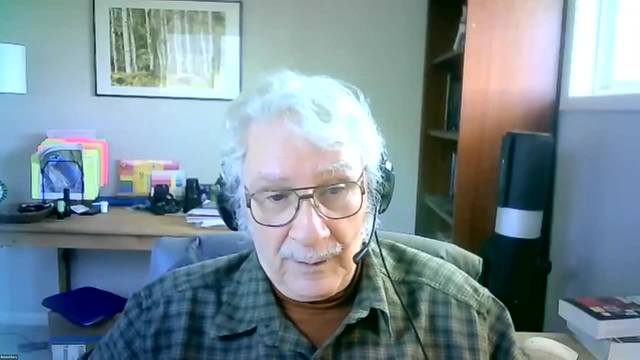 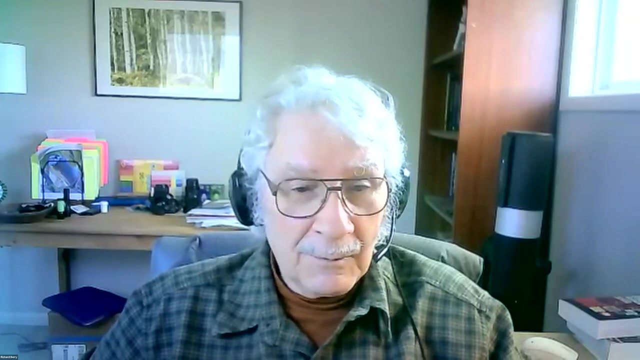 Um. One of the things that AIP for when has in it Um is the ability to make Synthetic star images. Okay, It's, it's one of those, relatively, I think it's in the edit Menu, But you can make a synthetic star. 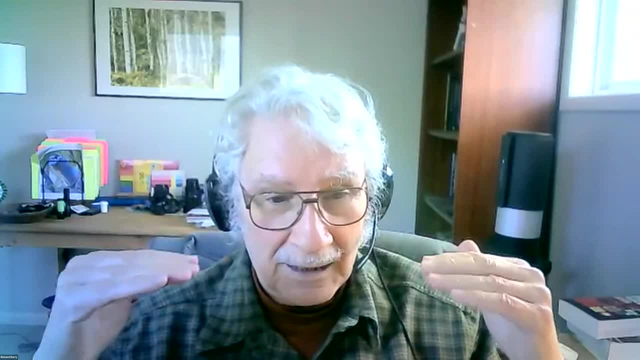 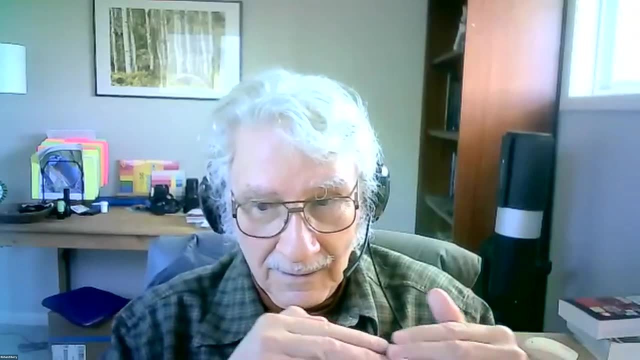 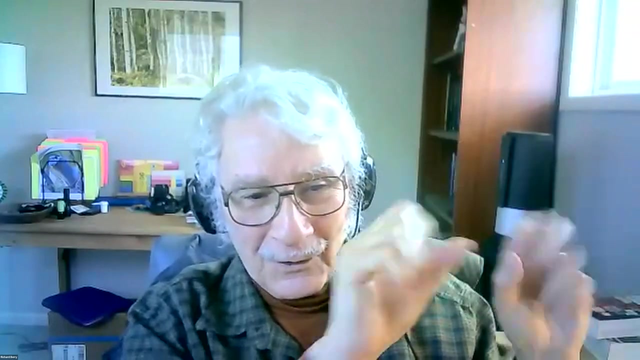 The, you know, has exactly 10,000 ADUs in it, And then you can run your photometry on it. And this is how I validated The routines that I have. Yeah, I built Artificial stars and then tested against the artificial stars. 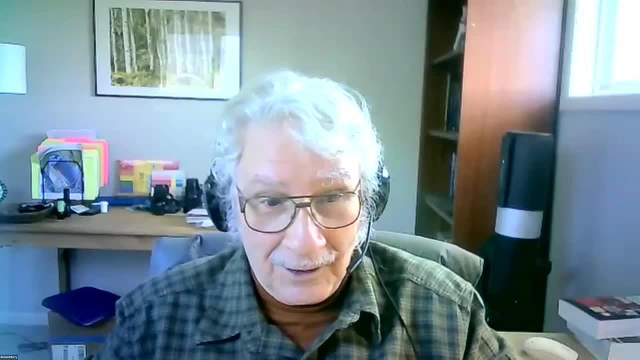 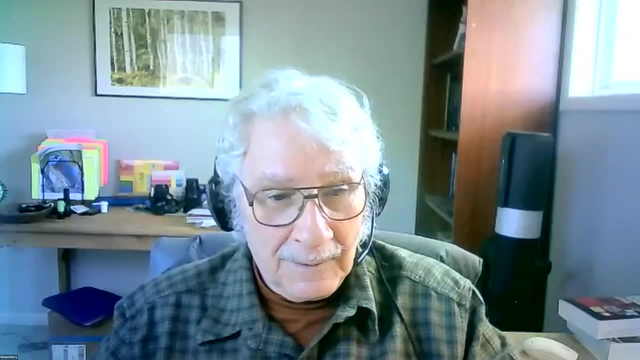 Now you say, well, wait a minute, Maybe you made errors in writing that code. Um, that's true, Um. but you know how do you validate stuff? Um, you, you test, and then you test it against what you think is working. 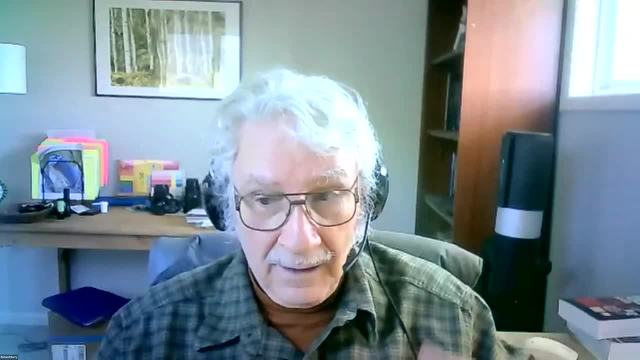 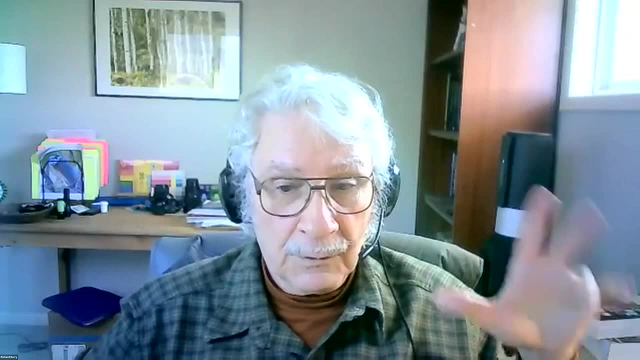 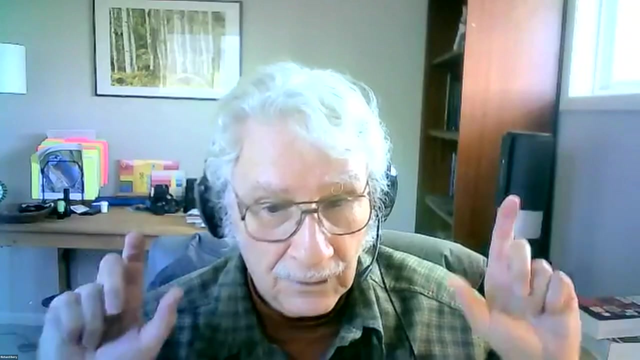 Right, Um, and to go back again, This, this particular code, the way that I showed you, Is not efficiently written code. It was written to be Very clear, Very testable. Okay, You can look at that code and you can in your mind say: how does that work? 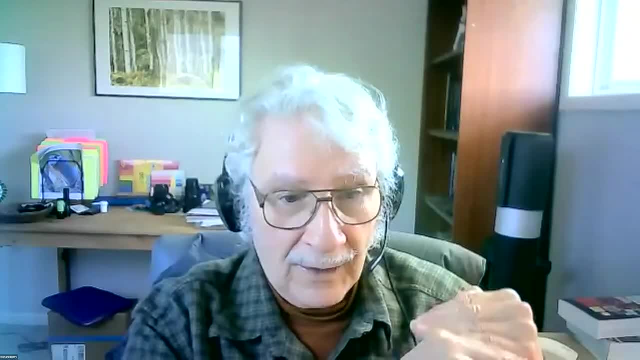 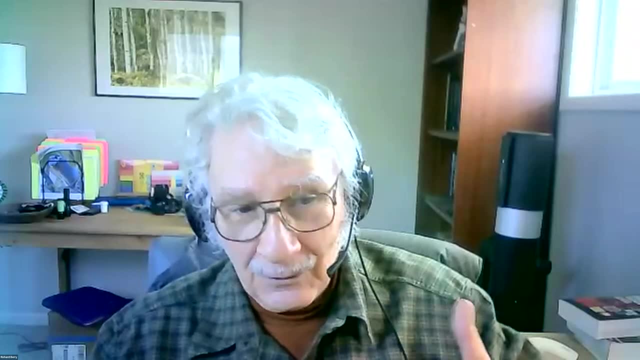 Is he? is it doing exactly what I think it does. When, as a programmer, when you're, You like to be clever, Okay, You like to do things very efficiently, All that thing where we go through and we sort through the, the, the. 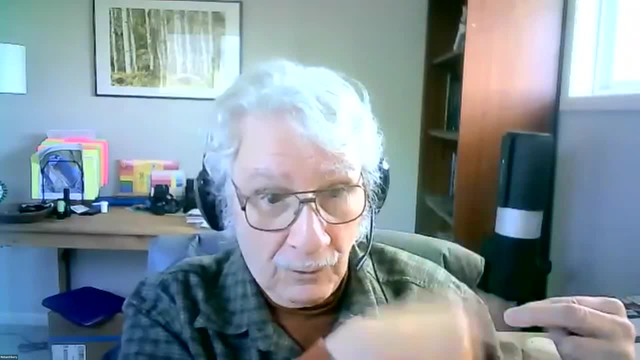 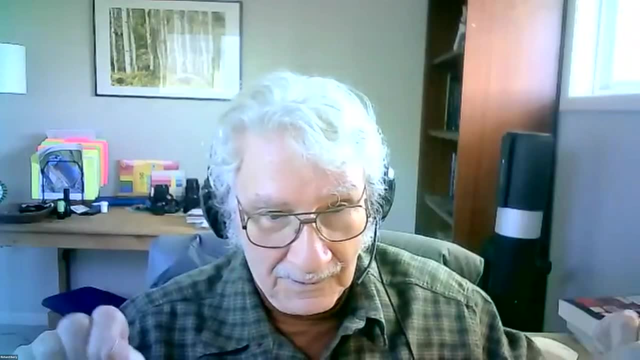 Individual pixels. We do the same thing over and, over, and over again. You don't have to do it all over again. We could have Stripped these, these things out. We could have put them into other arrays. We could have. 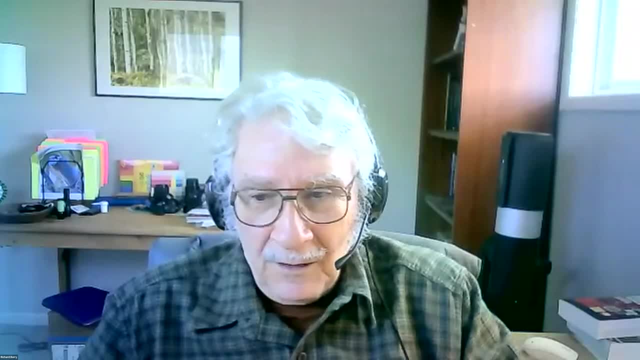 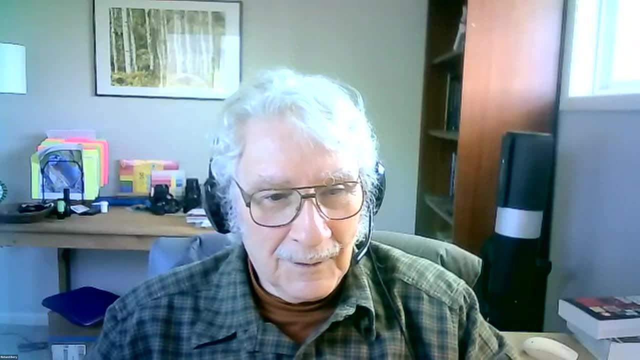 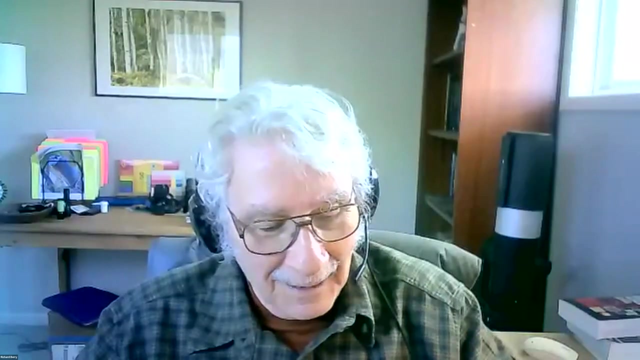 Cut the amount of computation, But when you figure that Your, your computer, is capable of doing like a million operations, A second Of the sort, You still, You still can't see. usually, Between the time you hit the click And the time it appears on the screen, you can't see. 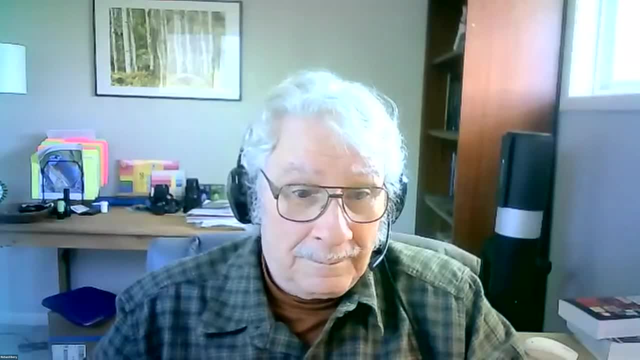 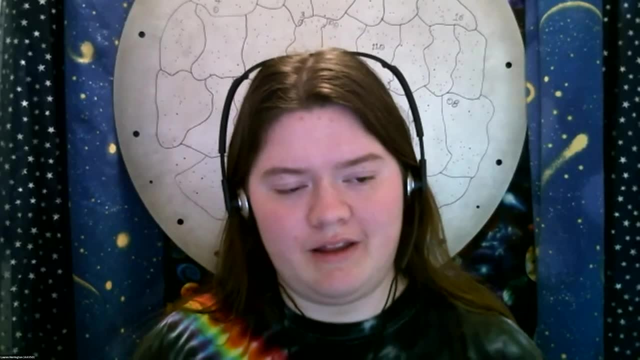 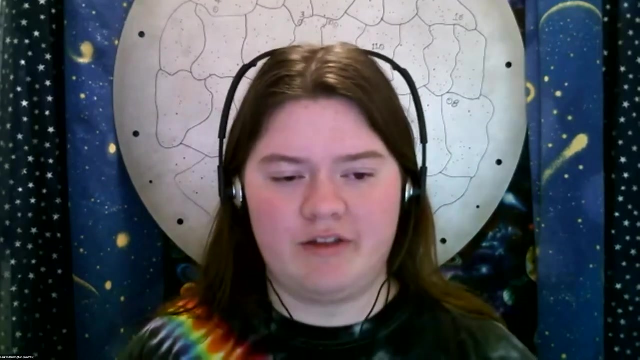 Those processes happen. Yeah, All right, Thank you. Let's go to the question from Dennis Conti, Which was: since the EV scope uses an Altasmith mount And there's therefore image rotation, Are there significant systematics introduced from this image rotation? 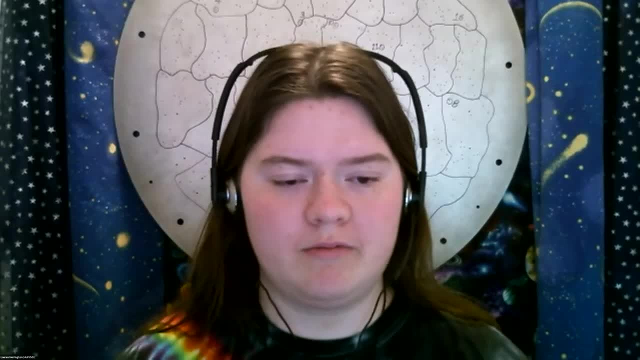 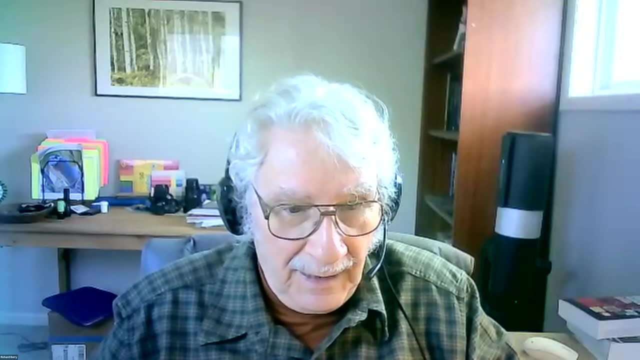 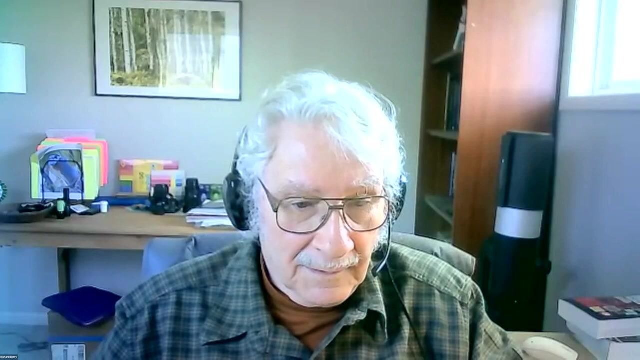 when you're doing long stacks with the EV scope. I have not done a Careful test of that. It's a good question, As, But What I've- let's put it this way, What I've done with the EV scope. 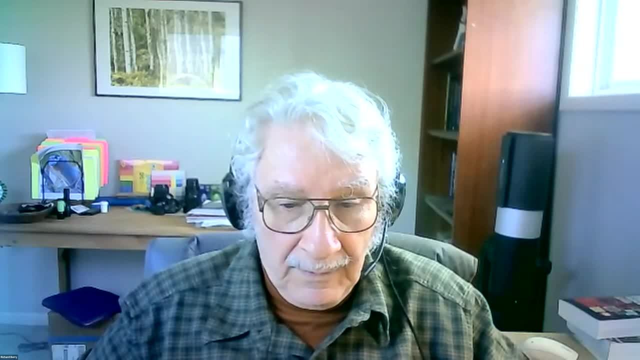 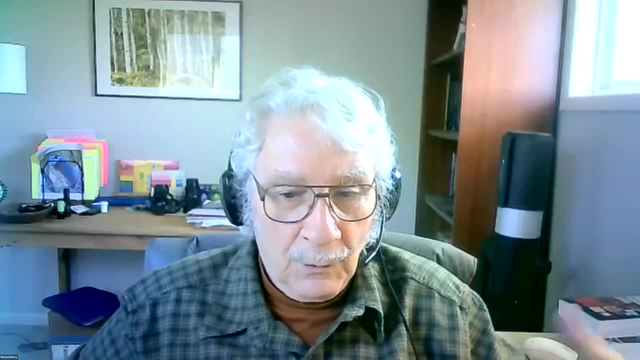 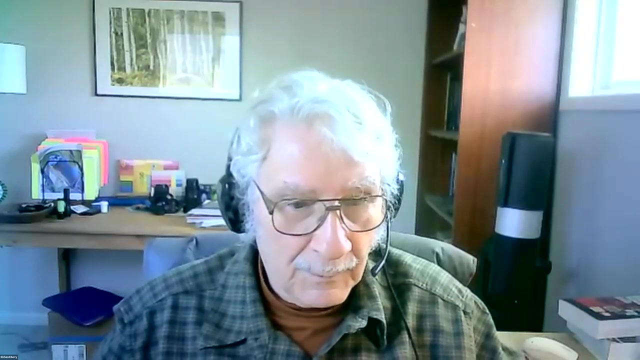 Is. I am using their stacked images here for illustration purposes. When I've done photometry, I've gone back to the individual Frames And done The Photometry on them, And my code Knows how to. Okay. 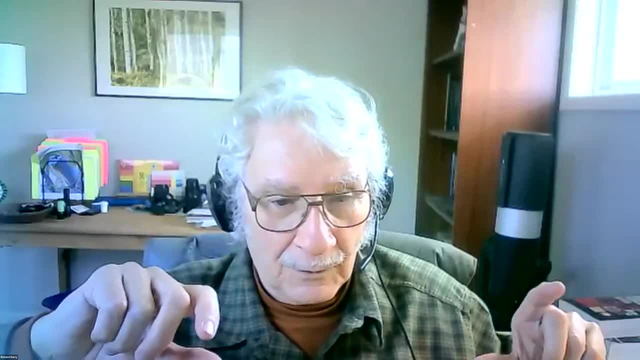 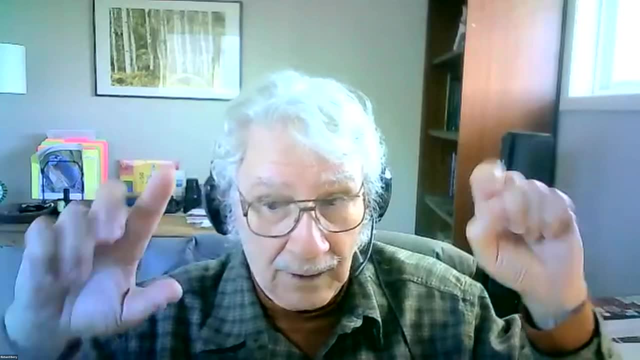 Not not in the, not in the single star photometry tool, But in the other. It has what I call a track star or a guide star. You designate the guide star actually to guide stars And it will follow And as the frames rotate, 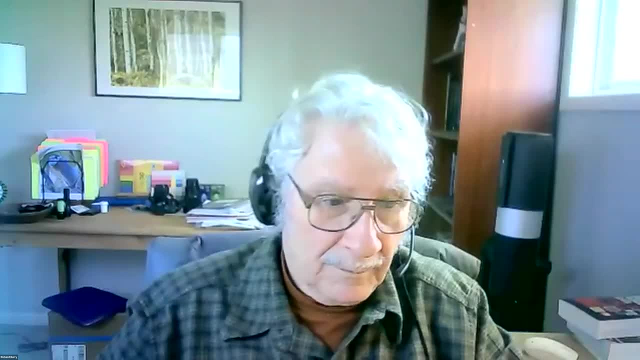 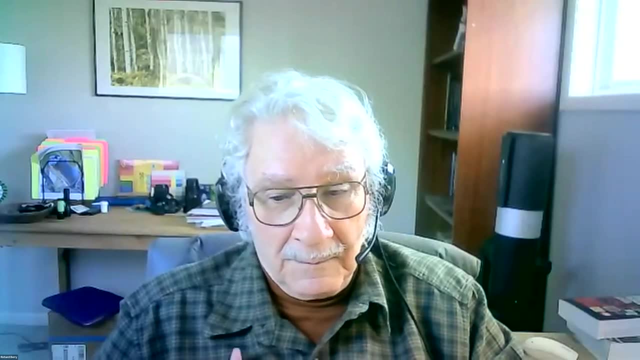 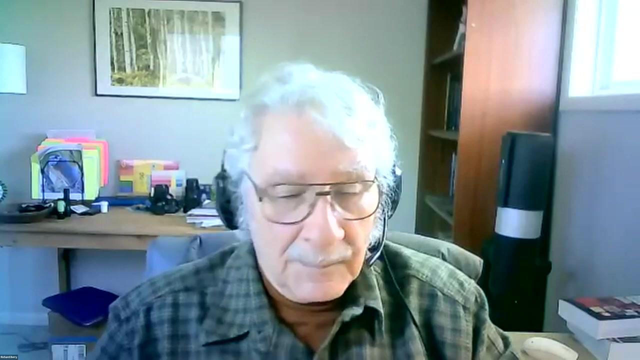 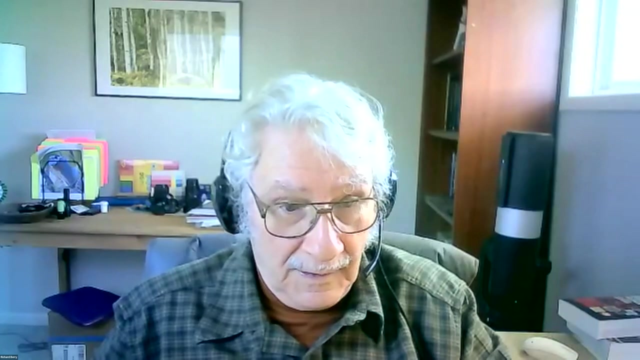 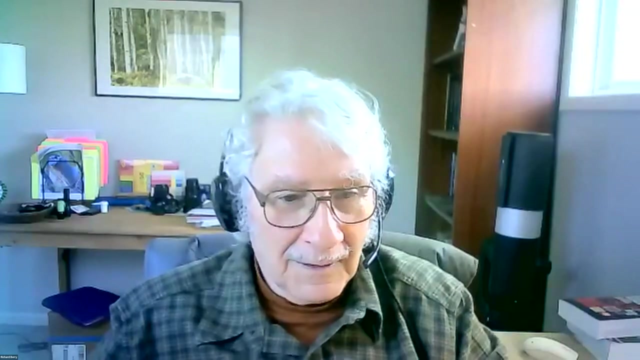 It will centroid And follow The, The stars of interest. So But I mean I could, I could pull up Photometry Run. I did on Star XX, For example. We're shooting one frame, maybe four seconds for for four hours. 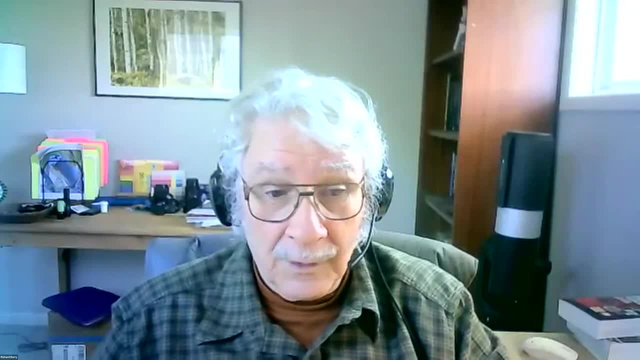 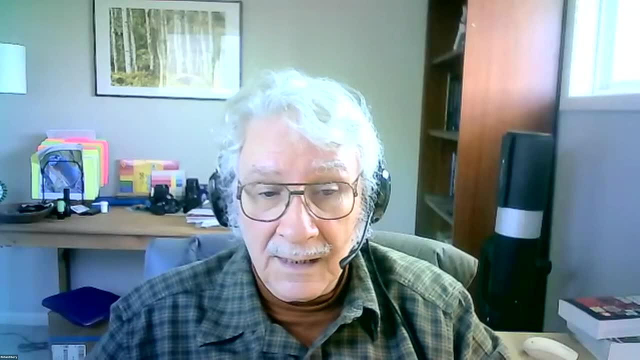 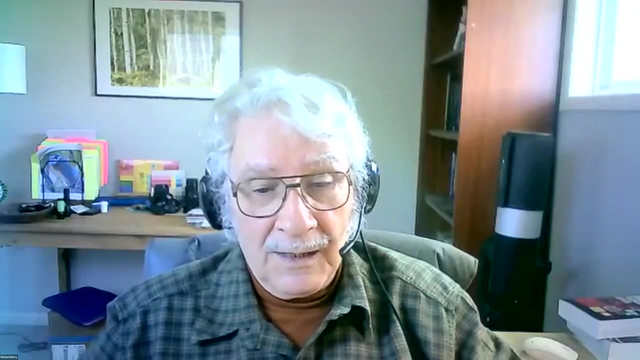 You get 3,600 data points And It's noisy data because they're short. The star was fairly dim, but But I don't see any systematic things happening. What the what? The weirdest? The trick with the AV scope. 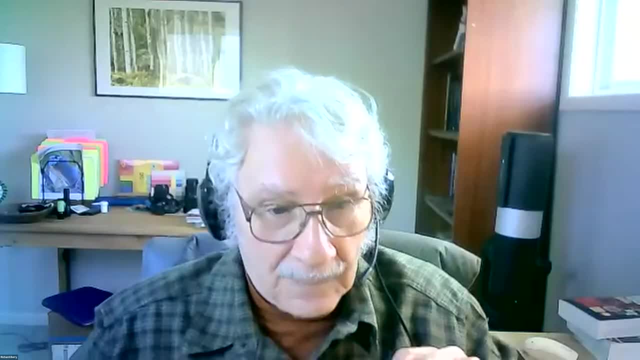 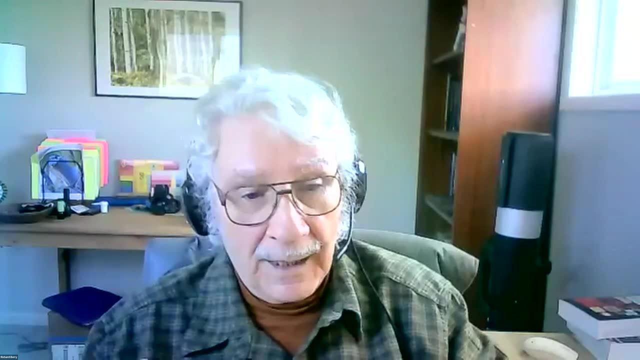 Is. it's a Bayer array filter. Okay, So it's already. it's a color. It's a color camera. In the images I've shown, I have debayered, Using equal weights on the red, green and blue. 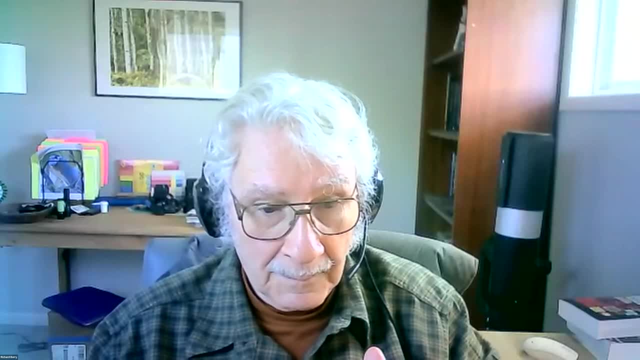 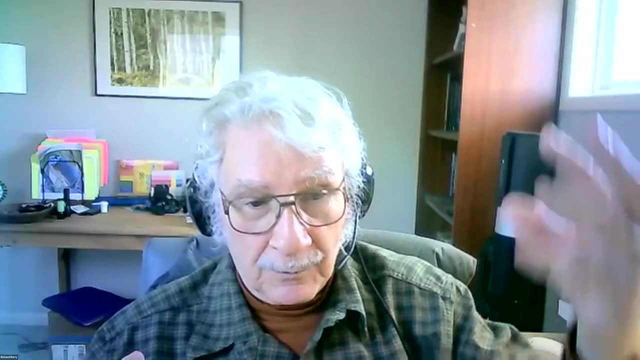 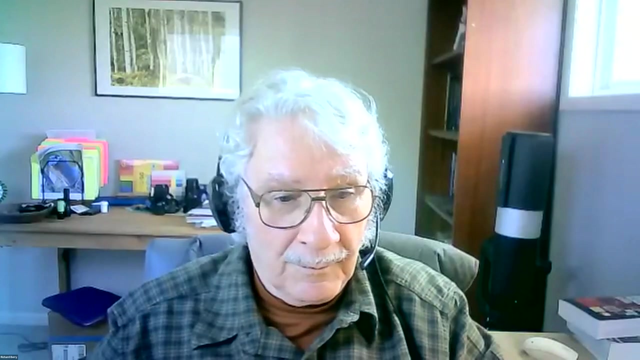 Channels. I haven't yet done the thing where I've split The images into red, green and blue images And then carried out Photometry separately on them. I remember Dr Harris talked about that method and her DSLR talk last year. 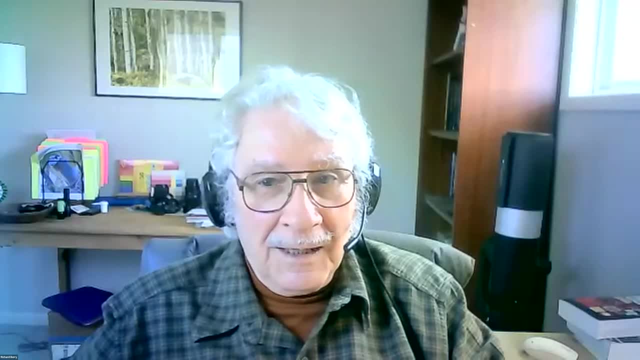 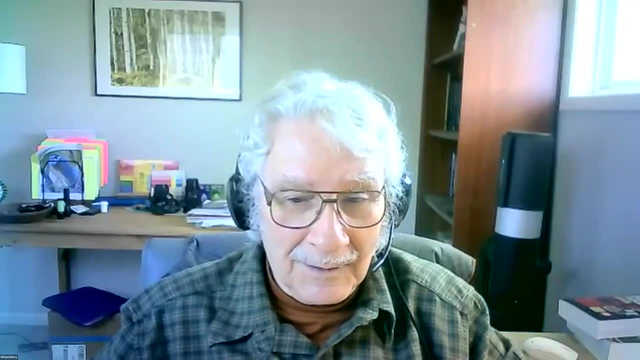 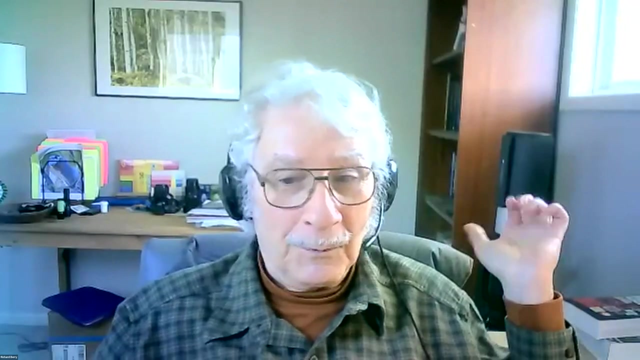 Yeah, I mean this. This stuff gets Complicated. Let's put it this way You can. you want to use a monochrome filter? I mean a monochrome camera With filters. If you have The EV scope as the scope, you've got. 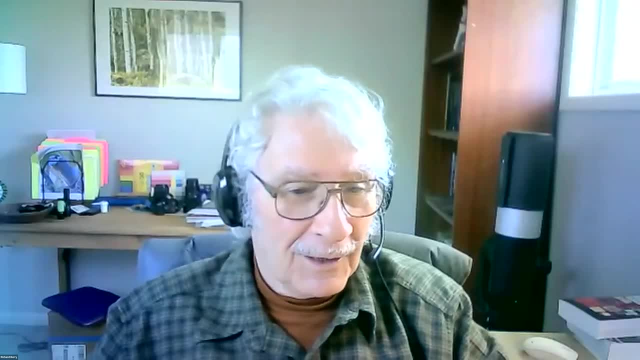 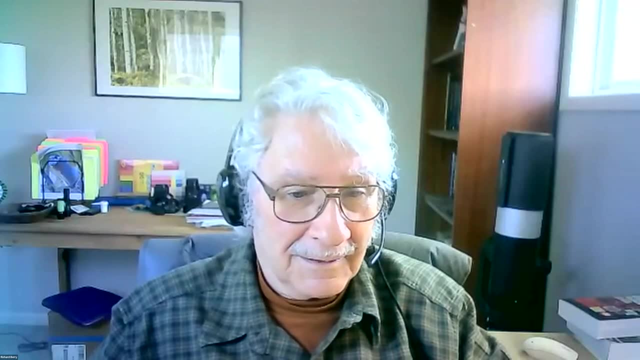 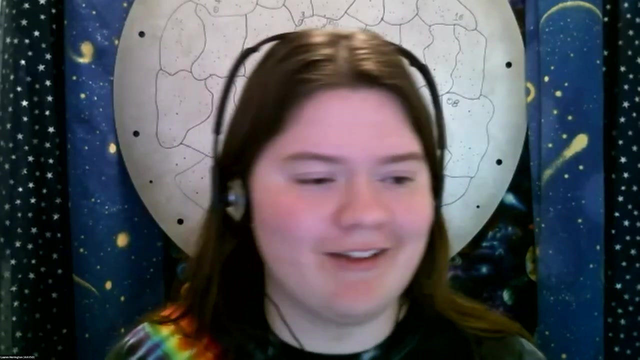 You, You know, being a curious person, you figure out what the heck the thing can do. I've been Surprised at how good it is. Okay, We have time for just a couple more Questions, Probably about five minutes or so, So let's try and. 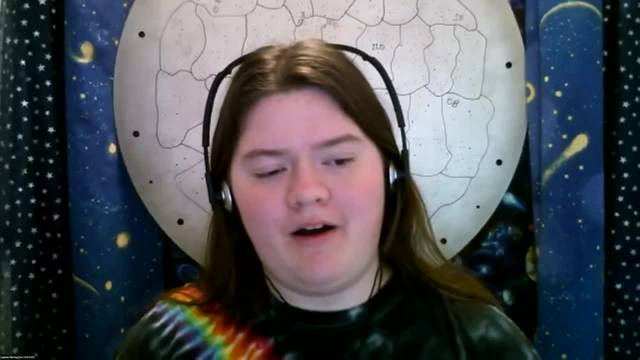 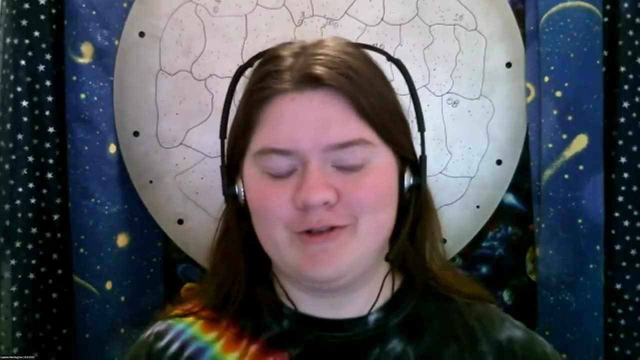 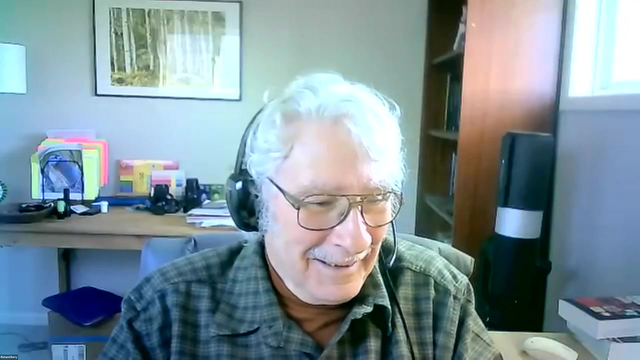 Okay, Let's do these. So one of these is: Are you self-taught in programming And, if so, What learning material did you use And or would you recommend? I'm so old that I learned how to program with alcohol. 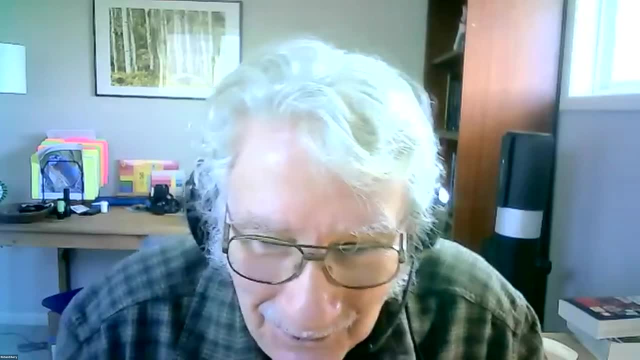 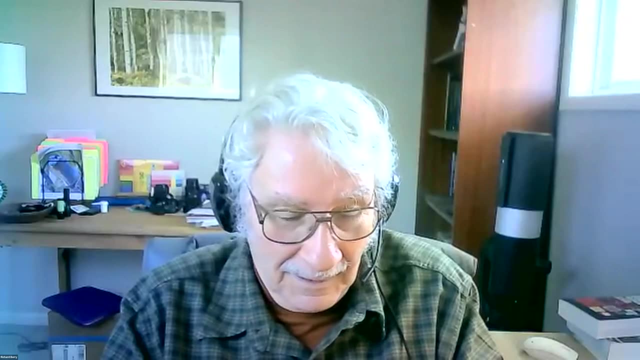 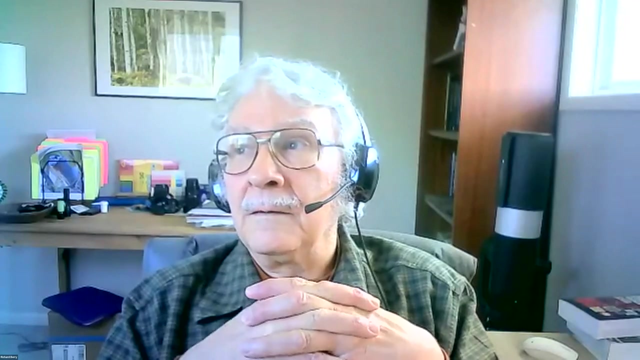 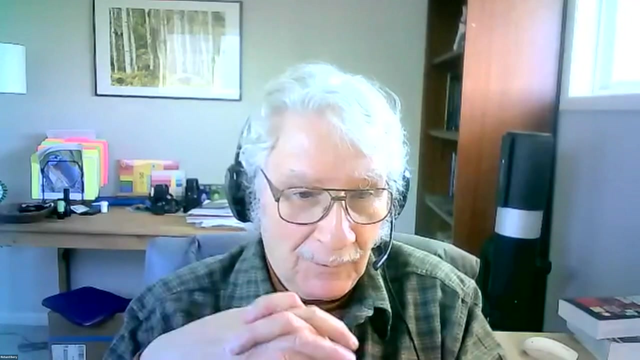 60 on a mainframe computer. Okay, So Yeah, And alcohol 60 is remarkably similar to Basic, or at least at the level I I understood it. I got MS basic five For a CPM computer And that was my first experiences writing. 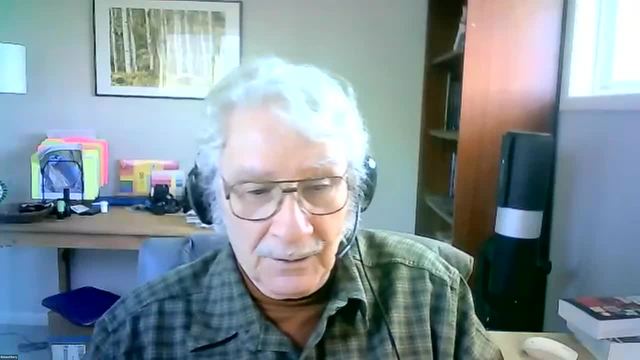 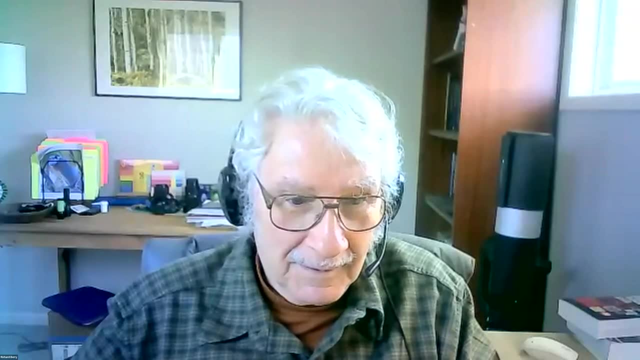 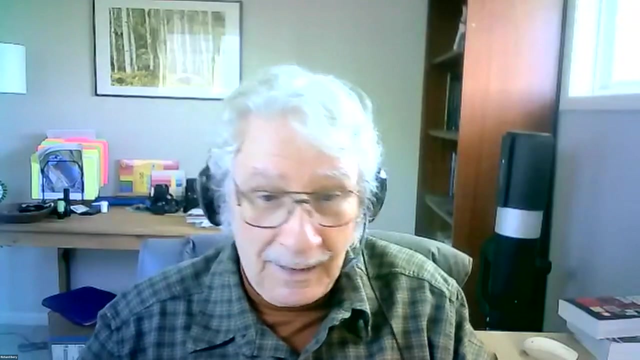 Well, actually Actually learn. my first computing with a mini computer With 4k of memory. 4k of memory Was a Hewlett Packard, I think it was 11,000 or something. It had 4k of memory. 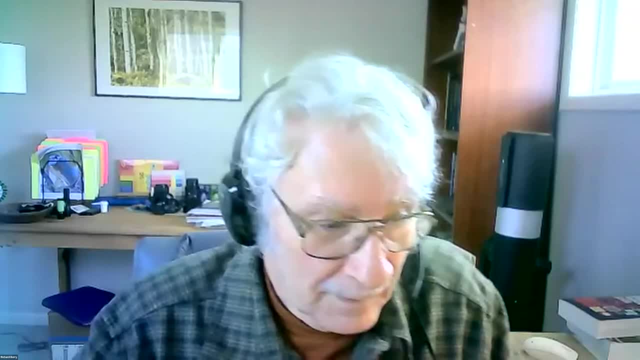 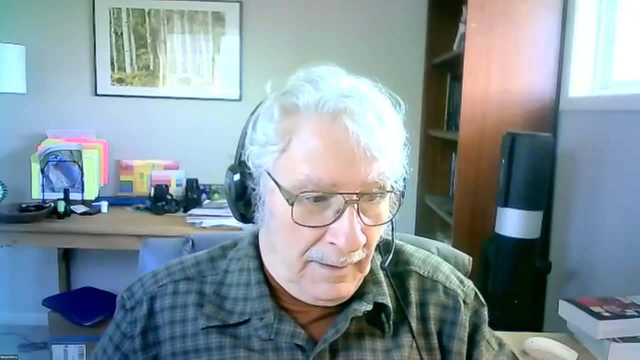 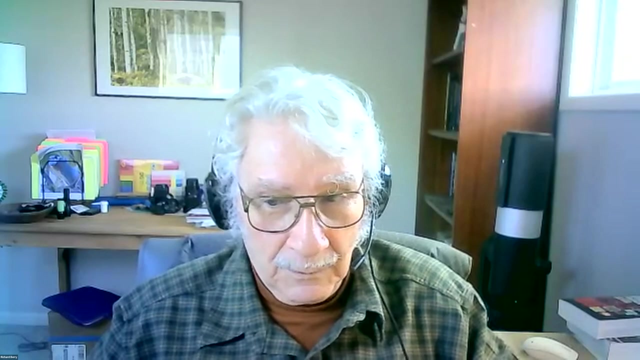 He's a teletype writer And I wrote software for reducing photo metric results, Done with the photo multiplier too, And yet Teletype Terminal to communicate with the machine. Then It was a program called turbo Pascal, And it was the first. 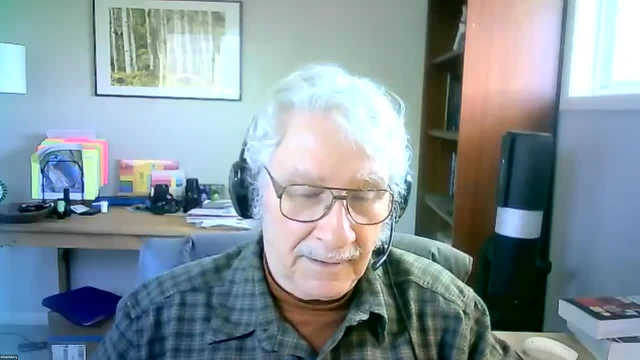 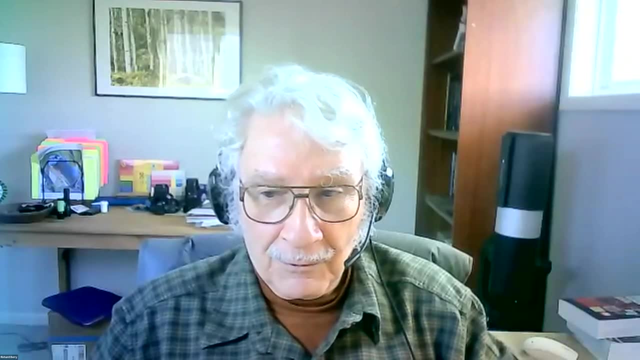 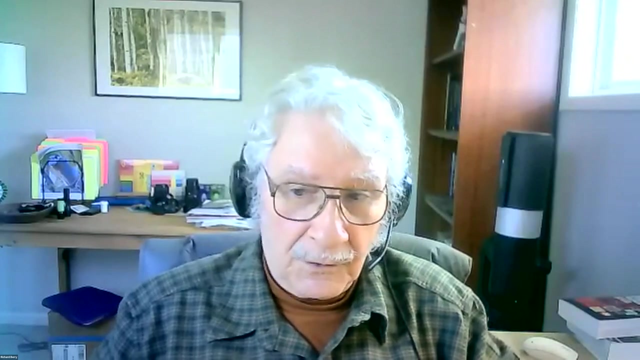 Structured Programming I did, And so I bought turbo Pascal for 80 bucks, or whatever it costs, And learned how to program, You know, in turbo Pascal. Then Microsoft introduced quick basic, which was structured Basic. So I went back to basic. 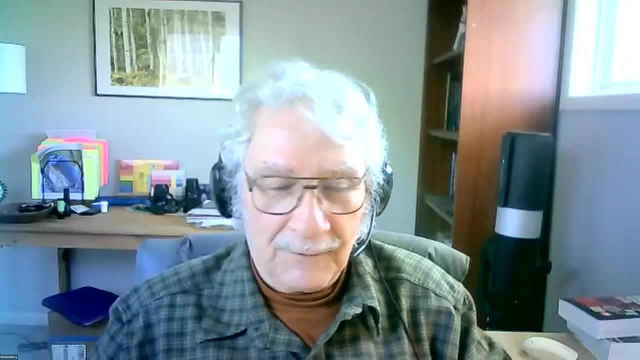 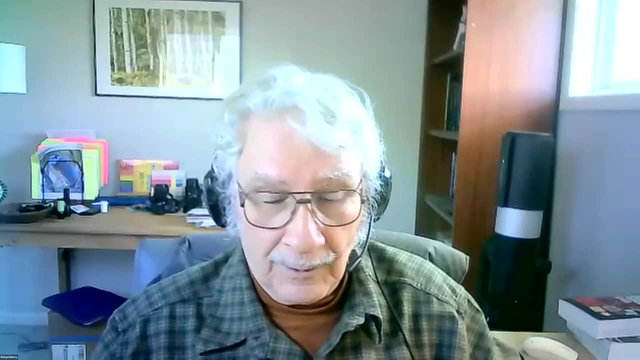 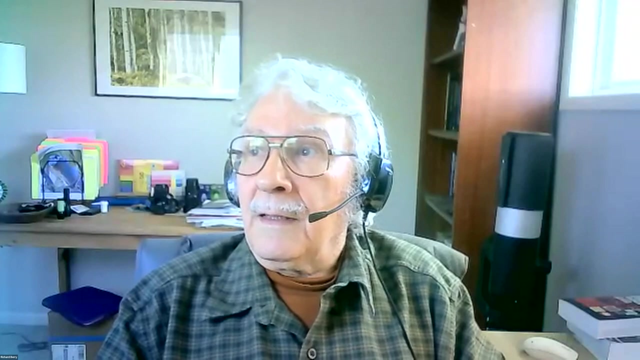 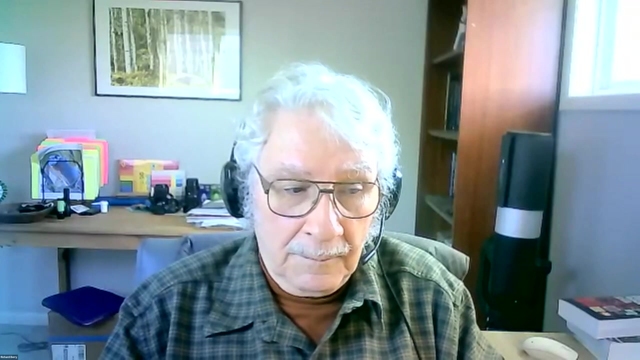 Then I switched into visual Basic for DOS And I wrote a lot of software for doing photometry And image sharpening and stuff like that And visual basic for DOS And the first Stuff I did with photometry was probably done in that code. 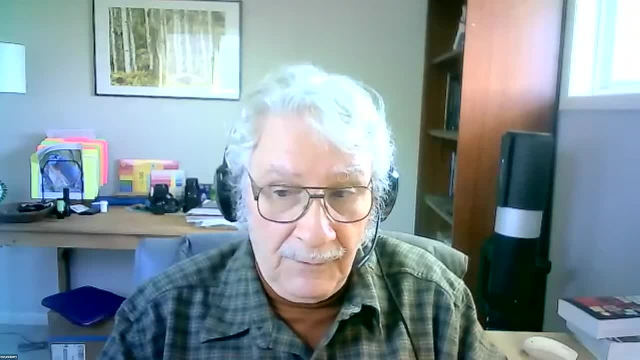 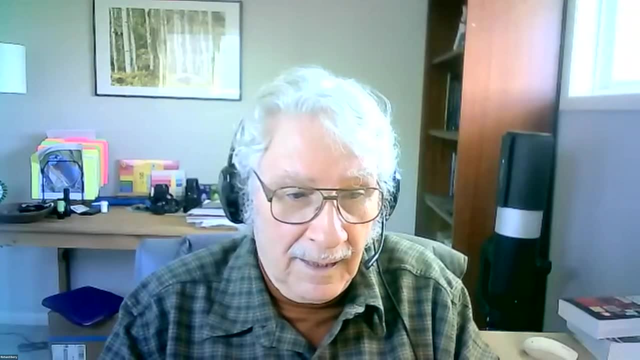 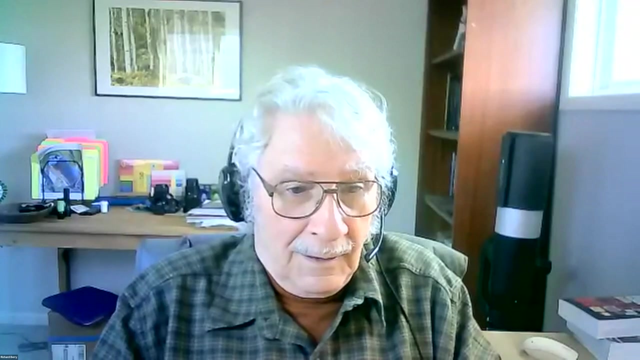 And I think people like Phil Sullivan Probably were relatively early adopters Of photo mat And astro mat, which were Programs for doing photometry with Images. That goes way back. So I think the answer is yeah, I'm self-taught. 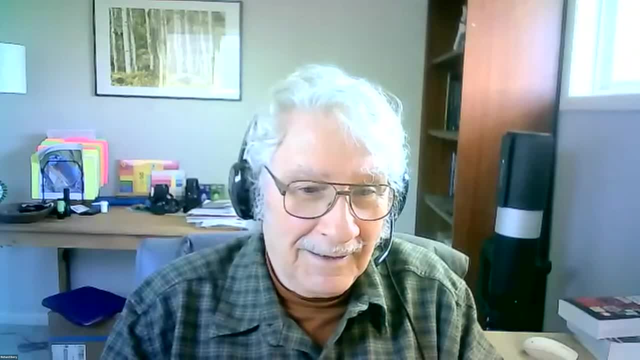 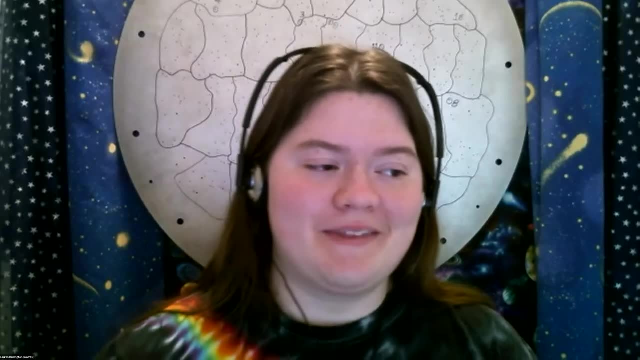 There was no classes in programming Back then. Wow, That's. that's an impressive history For sure. If you'll allow me to put in a little bit of a plug here, at the end of this year we have scheduled for how? two hours. 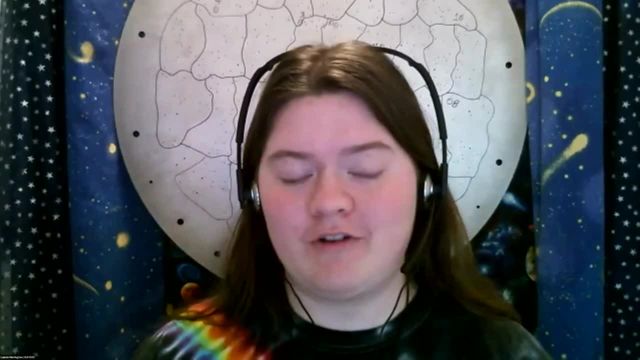 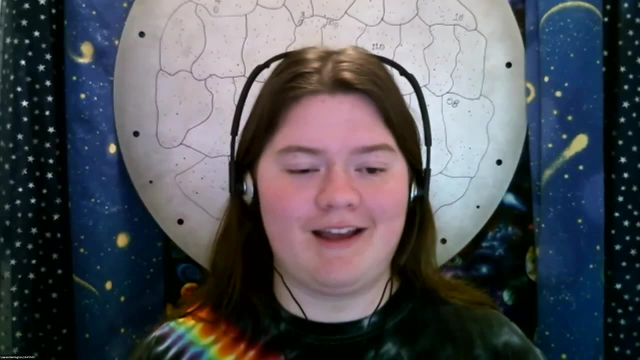 which will be focused on Teaching people how to program in Python For the purposes of manipulating astronomy data. So to the person who asked that question, Make sure that you come back later this year. We're going to be starting with the basics and going up through some. 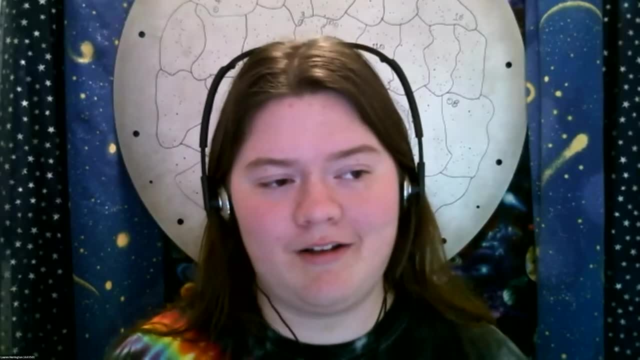 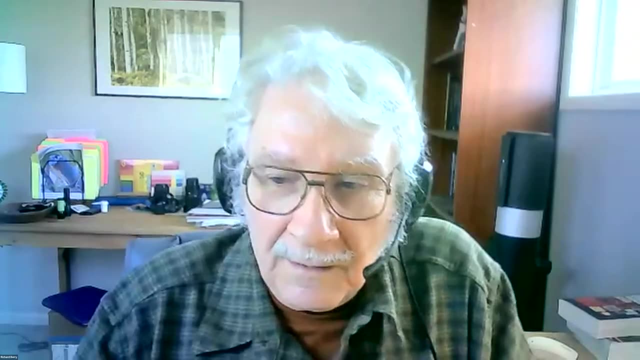 really cool data visualization stuff Using Python as a language, Yeah, And I think that's a really good question. I think that's a really good question. I think that's a really good question. Yeah, And I think If I were going to do one thing, probably 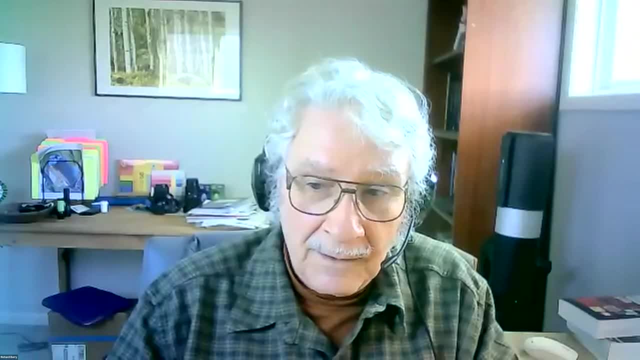 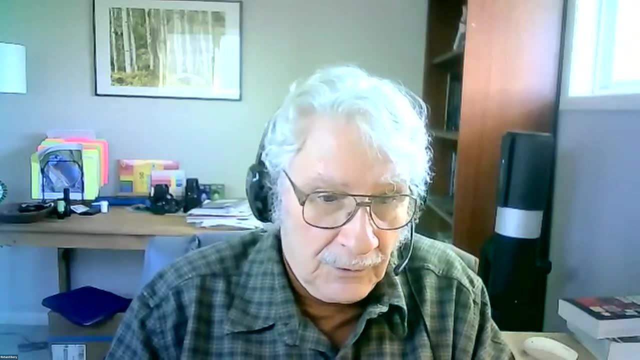 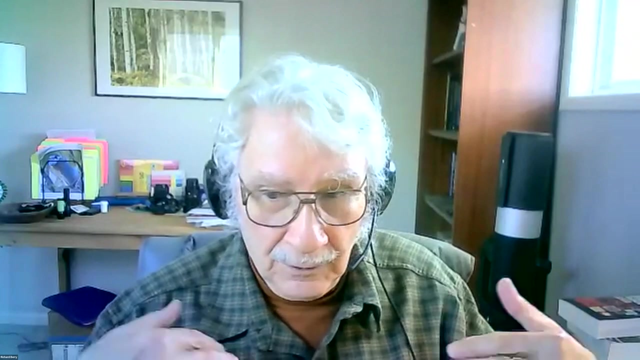 In a new clean release of AIP, It would be to put out CSV files instead of of photometry, So that you would be able to run your photometry In In AIP but then Do your analysis any way you wanted to. 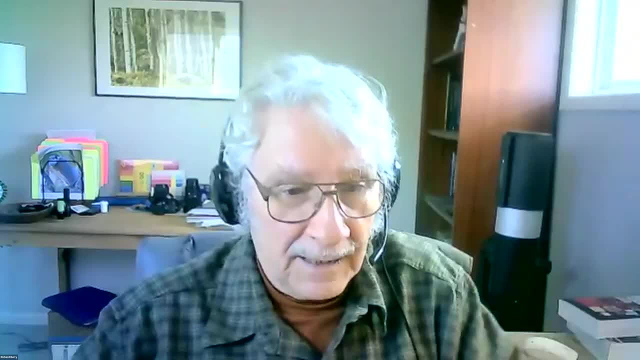 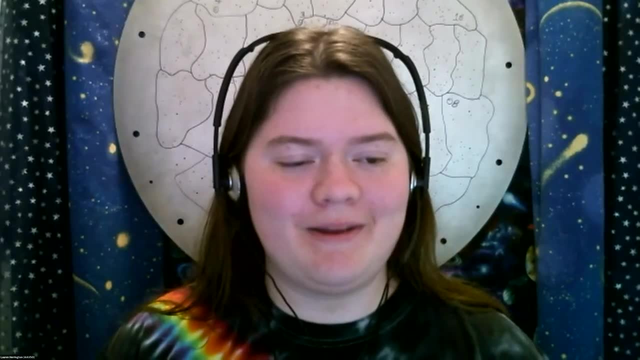 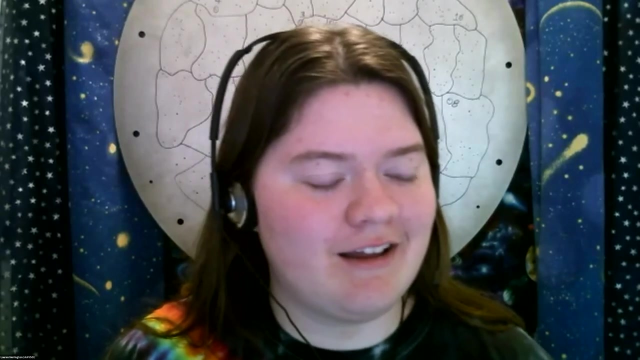 By using By using pandas to suck in the data And then doing the photometry, Writing the code. Yeah, Yeah, that would be convenient to have it be portable in that way. Okay, We have time for exactly one more question. 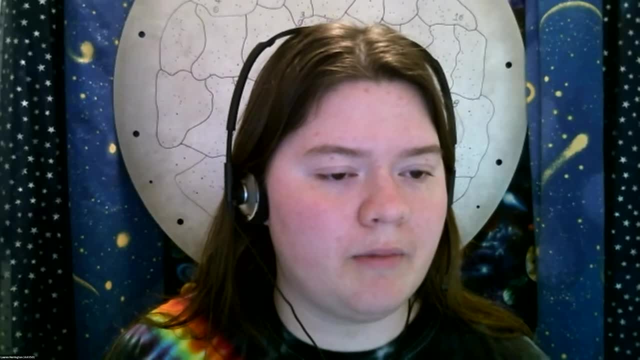 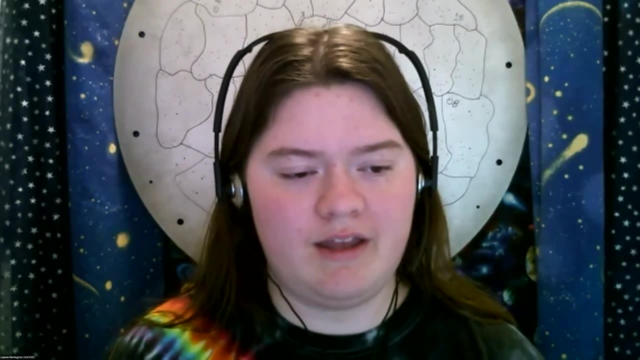 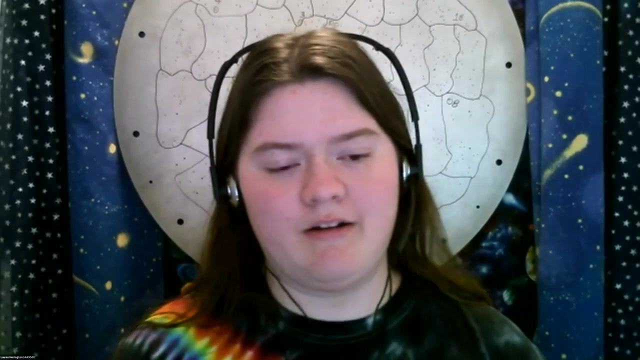 We're going to take this one from Mark, Who asked: is there a way to use AIP for when To get the numerical Pixel values in a subset of an image? The scenario is that If I have a star On the background of a nebula, 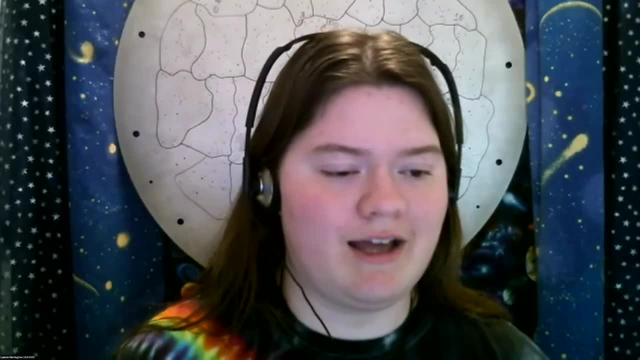 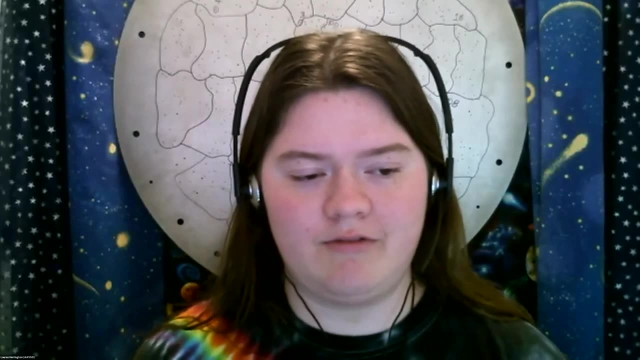 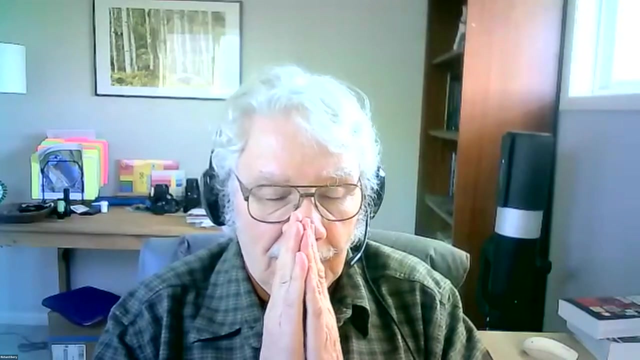 Or maybe a Active galactic nuclei and a galaxy. I'm going to need to be able to do some additional math in order to get Good PSF. On the point, like object, I'm trying to remember whether it's an export function for. 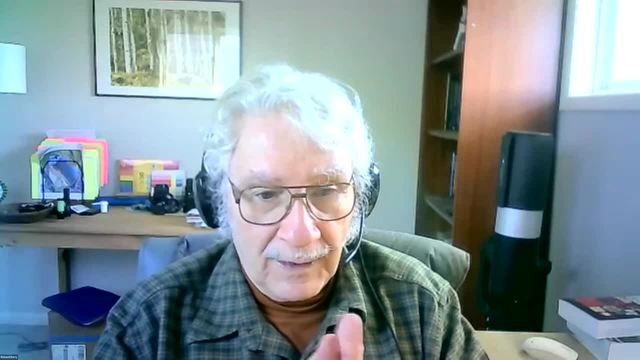 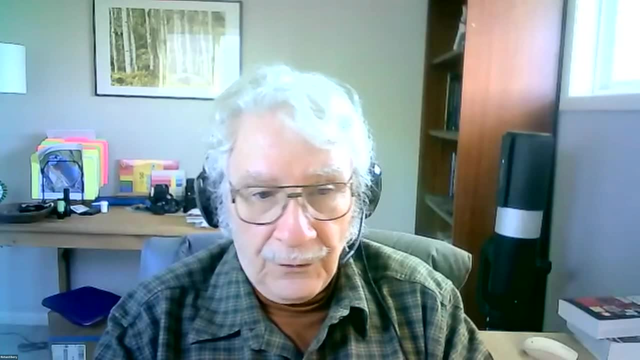 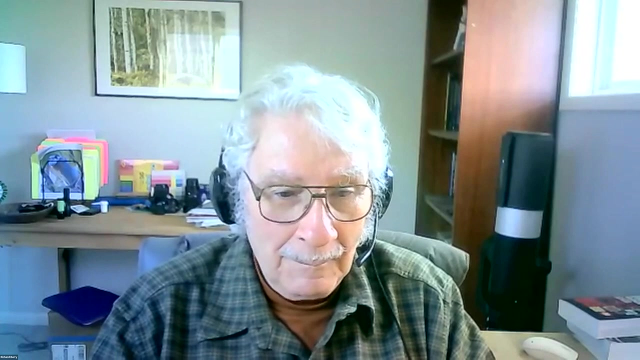 For for Putting out array values? I don't think so, But I'm not a hundred percent sure. There's stuff buried in the code that is, You know, Try every, every Dig into the menus and see if you can find it. 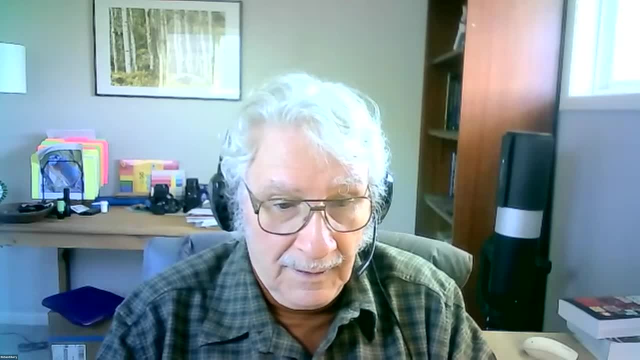 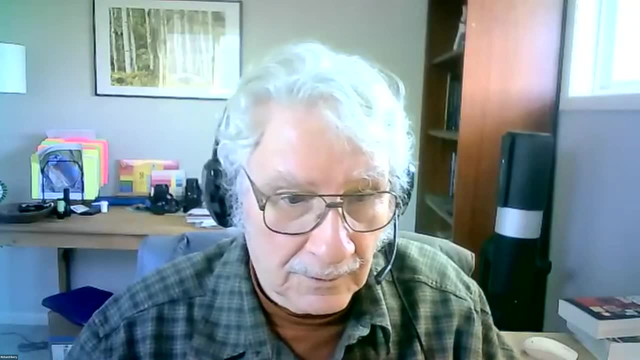 It should be there. It would have been There In the earlier code As a, As a teaching tool And basically, You know, in this box, Dump the data into, You know an Excel Type format, Right. 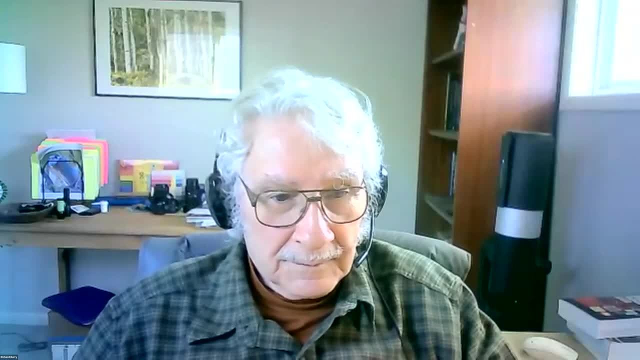 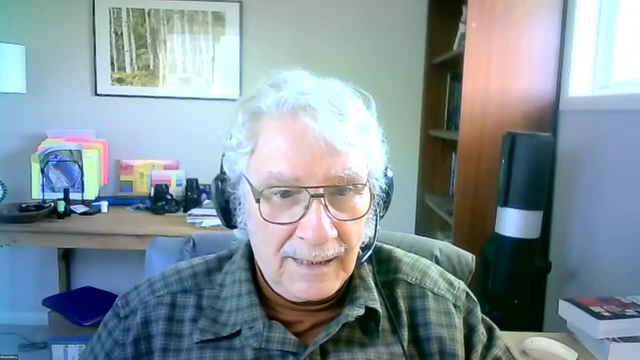 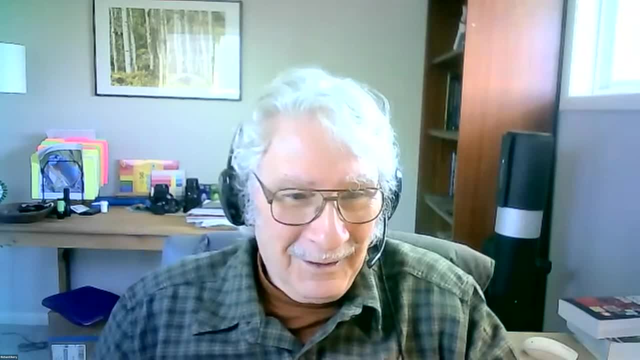 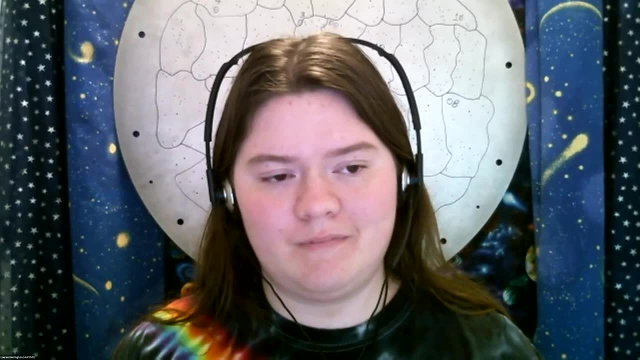 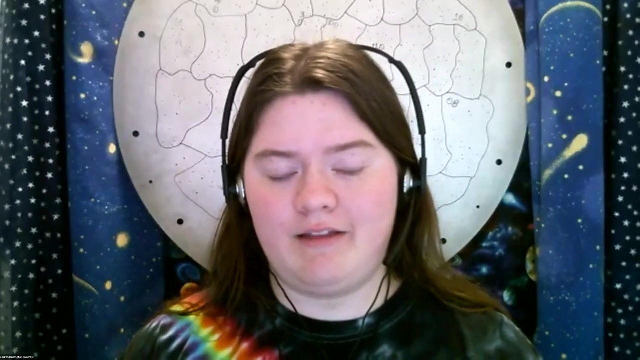 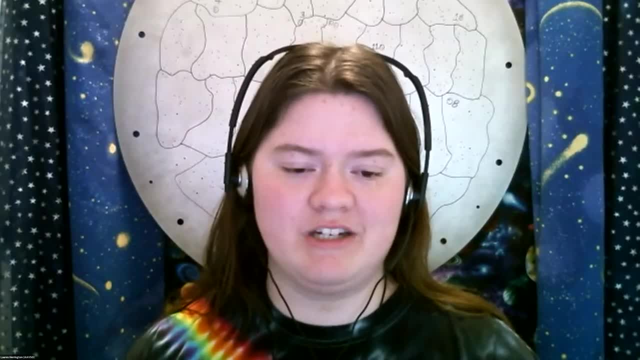 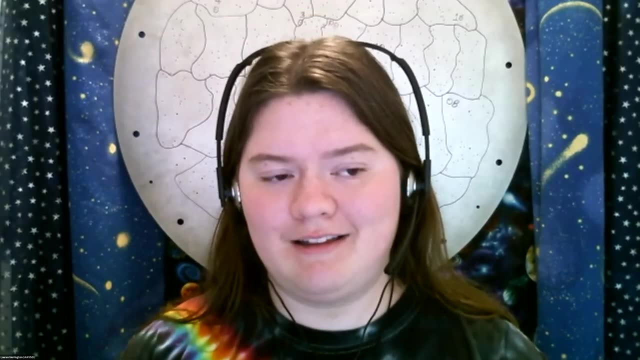 That would be something that would be very simple to do with Python. So I suggest you look into using Python and then The package called Astro Pi. with just a couple short lines, Using Astro Pi, You can load an image And then export the Pixel values for a subset of that image. 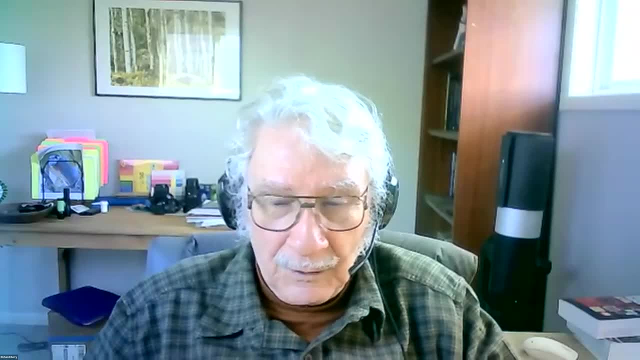 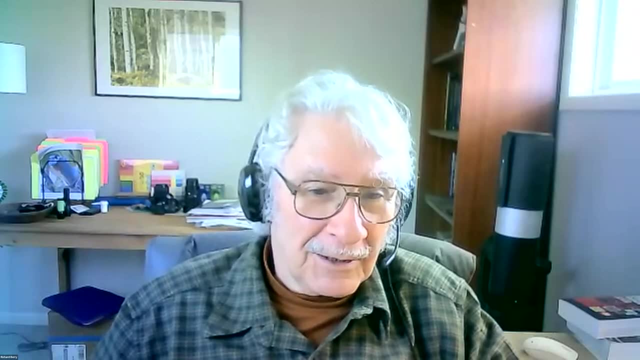 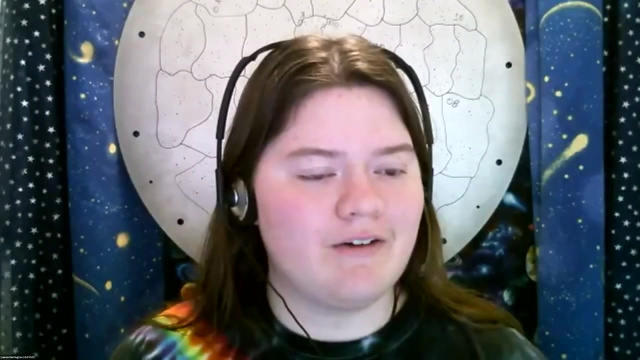 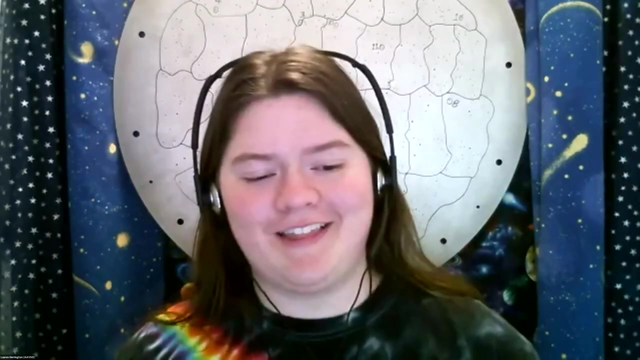 And so look into it yourself. And then AstroPie has very good documentation and there's probably a Jupiter notebook or a Jupiter notebook with examples already written in it. Yeah, I believe so. Okay, now most of what's left in the Q&A box is comments from people saying, wow, thanks so much for this wonderful presentation.